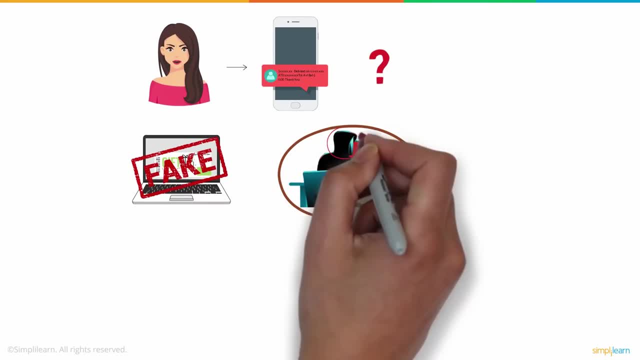 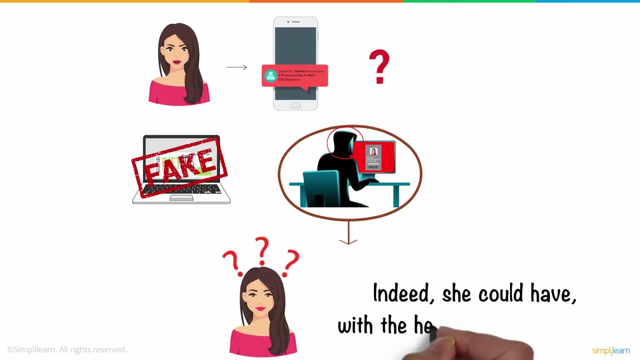 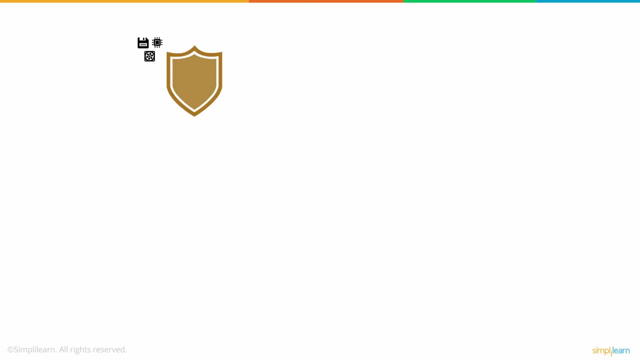 This type of attack is known as a cyberattack, and the person who carries it out is called a hacker. Could Anne have prevented this attack? Indeed, she could have with the help of cybersecurity. Cybersecurity involves techniques that help in securing various digital components, networks. 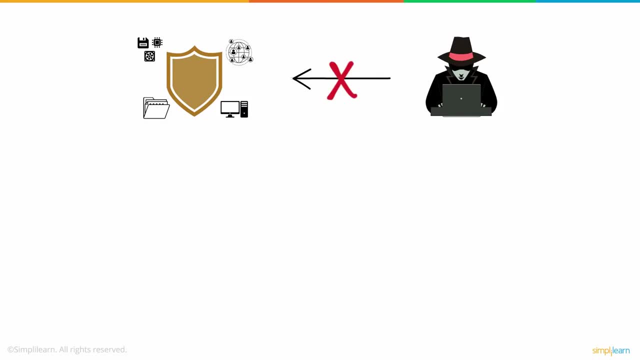 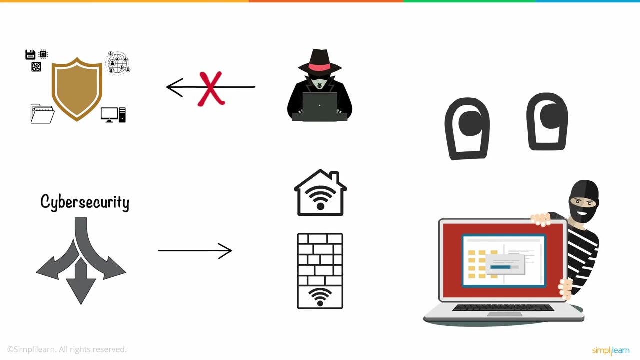 data and computer systems from unauthorized digital access. There are multiple ways to implement cybersecurity, depending on the kind of network you are connected to and the type of cyber attacks you are prone to. So let's take a look at the various cyber attacks that Anne could have been exposed to. 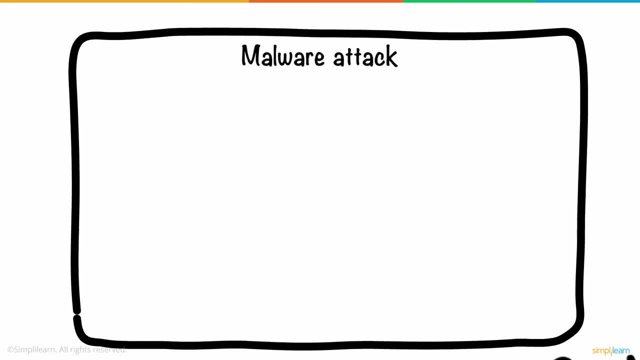 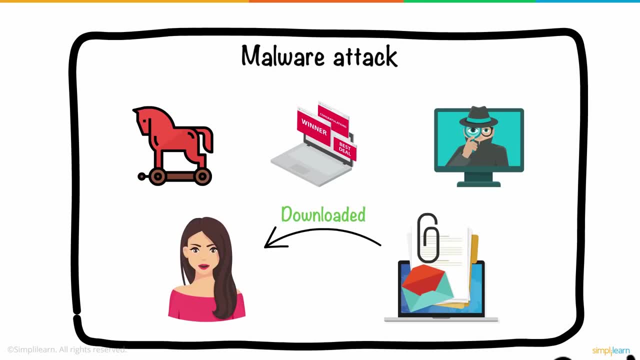 One of the most common types of cyber attacks is a malware attack like trojan, adware and spyware, to name a few. Had Anne downloaded any suspicious attachments online, her system could have gotten corrupted by certain malicious viruses embedded within the attachments. 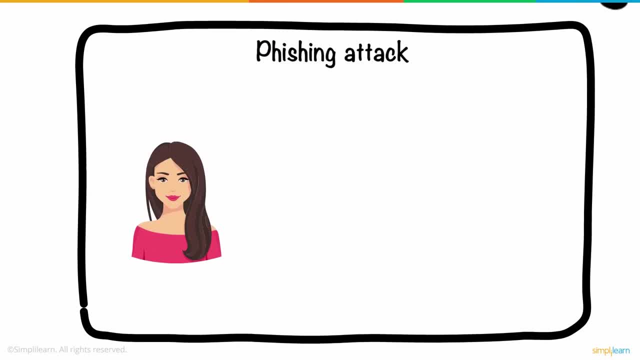 How did she get caught? Next is a phishing. This is a type of cyber attack which Anne experienced Here. the hacker usually sends fraudulent emails which appear to be coming from a legitimate source. This is done to install malware or to steal sensitive data. 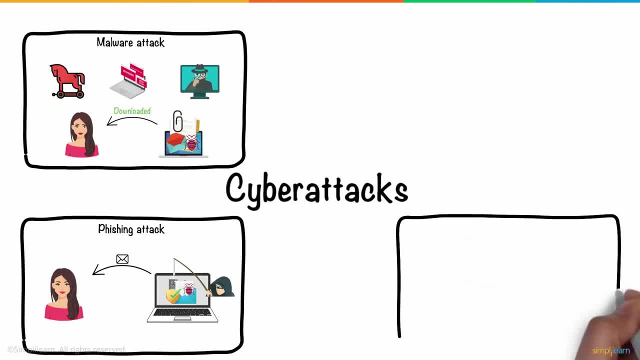 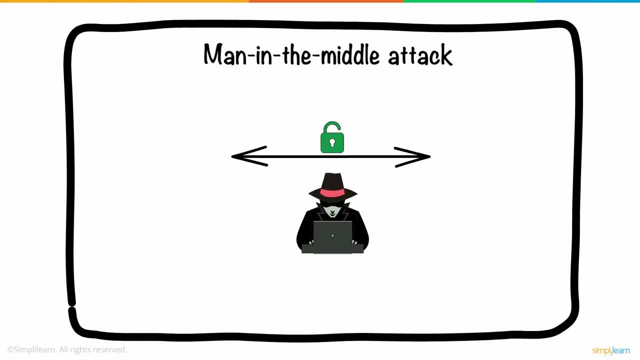 like credit card information and login credentials. Another type of attack is the man-in-the-middle attack. Here the hacker gains access to the information path between Anne's device and the website's server. The hacker's computer takes over Anne's IP address. 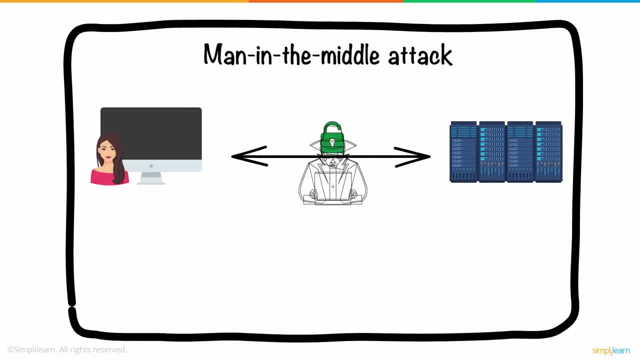 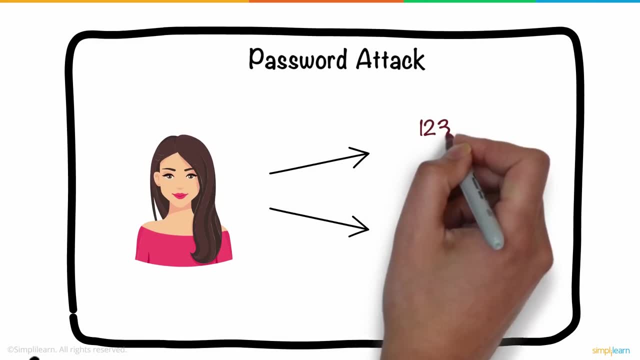 By doing so, the communication line between Anne and the website is secretly intercepted. This commonly happens with unsecured Wi-Fi networks and also through malware. Password attack is one of the easiest ways to hack a system. Here, Anne's password could have been cracked by using either common passwords. 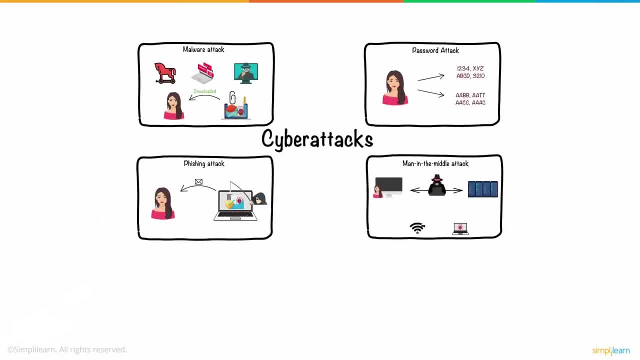 or trying all possible alphabetical combinations, To prevent future cyber attacks. Anne sought to implement a few cybersecurity practices. First, she installed a web-based cyber attack on her computer. She installed a web-based cyber attack on her computer. She installed a web-based cyber attack on her computer. 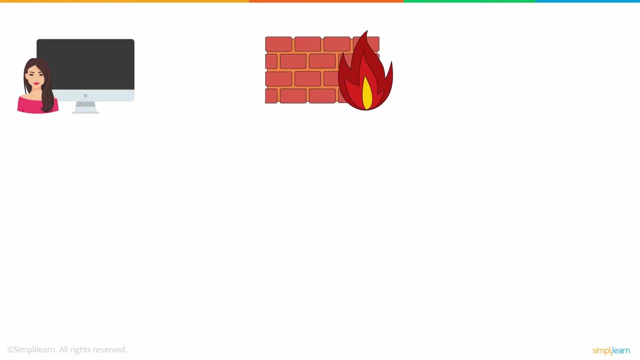 Second, she installed a firewall. As the name suggests, it is a virtual wall between Anne's computer and the internet. Firewalls filter the incoming and outgoing traffic from your device to safeguard your network, and they can either be software applications or hardware reinforcements. 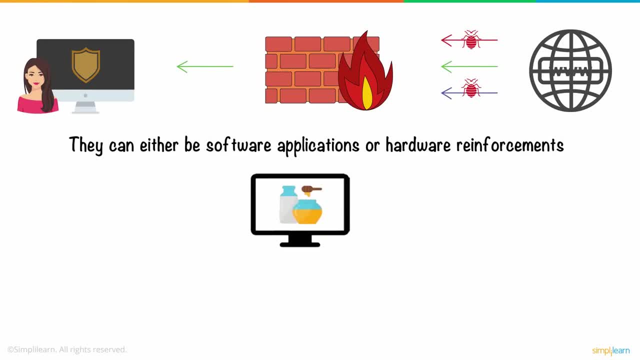 Secondly, Anne implemented honeypots. Just like how flowers attract bees, dummy computer systems called honeypots are used to attract attackers. These systems are made to look vulnerable in order to deceive attackers, and this is how they work, And this, in turn, defends the real system. 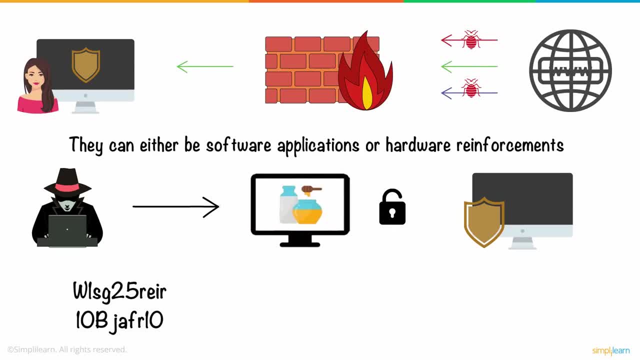 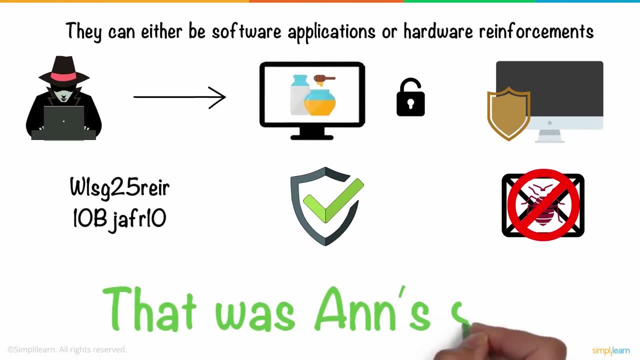 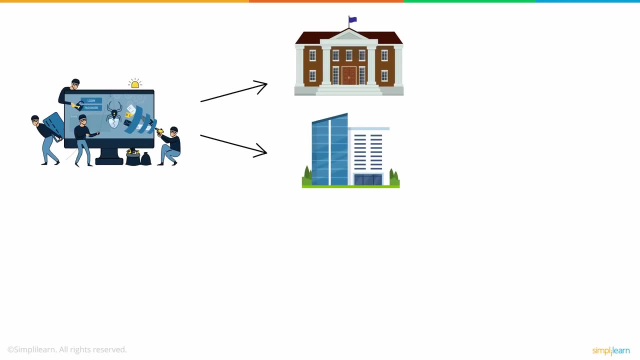 In addition to these, she also decided to use unique alphanumeric passwords, antivirus software, and started avoiding mails from unknown senders. That was Anne's story. Cyber attacks are not just confined to individuals, but also to public and private organizations. The cyber attacks carried out in such places are more deadly and they result in colossal losses. 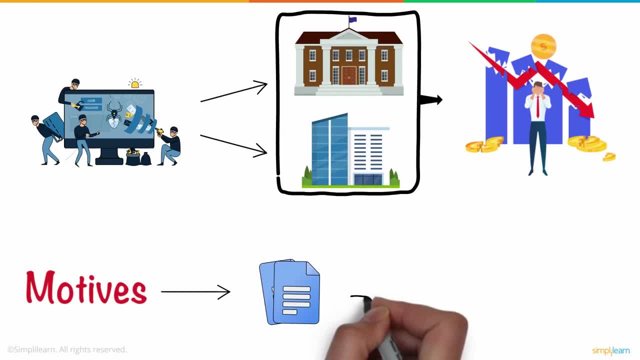 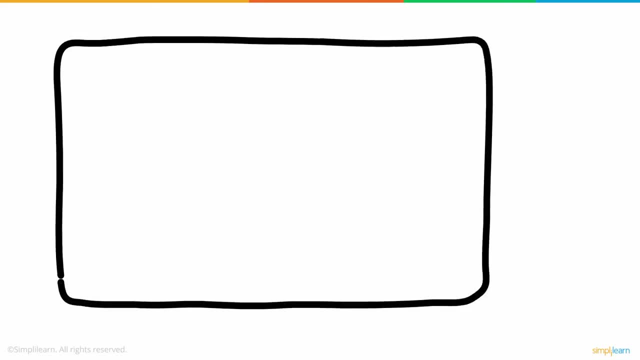 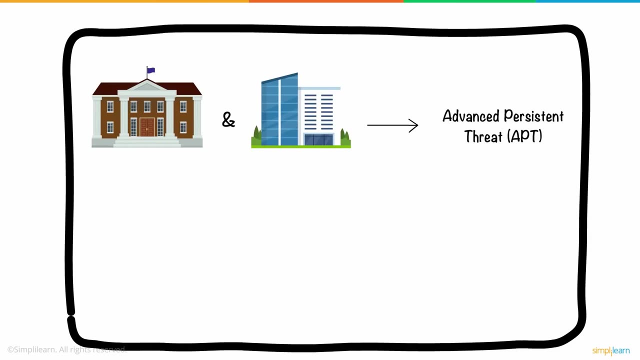 Motives of such attacks are many, Starting from tampering with crucial data to monetary gains. Let's have a look at a few of the cyber attacks that companies are subjected to. Various public sector organizations and large corporations face the Advanced, Persistent Threat In this form of attack. hackers gain access to networks for a prolonged period. 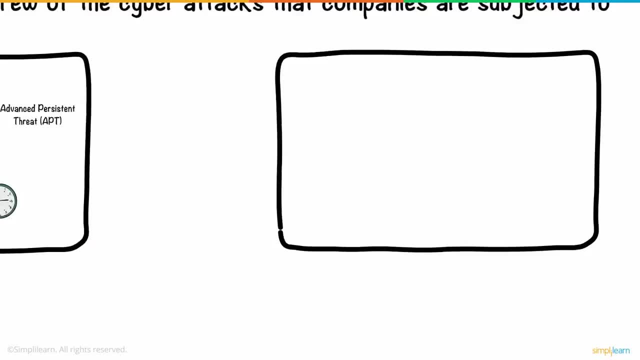 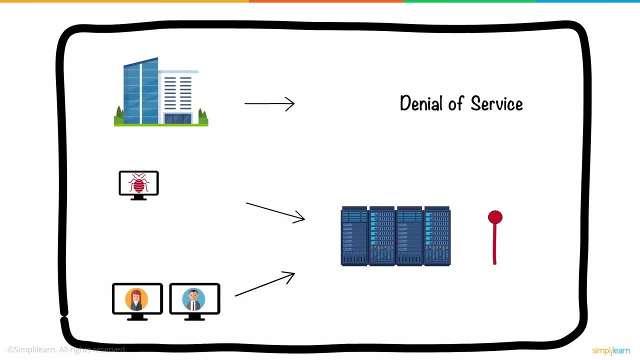 in order to continuously gain confidential information. Companies also witness the denial-of-service attack, where networks are flooded with traffic which in turn lead to the death of their customers. This in turn, leaves legitimate service requests unattended. A variant of this is the distributed denial-of-service attack. 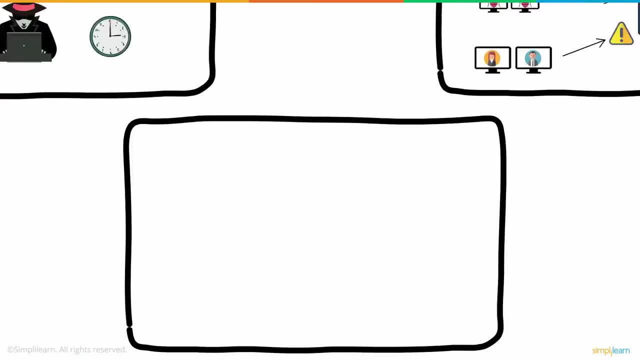 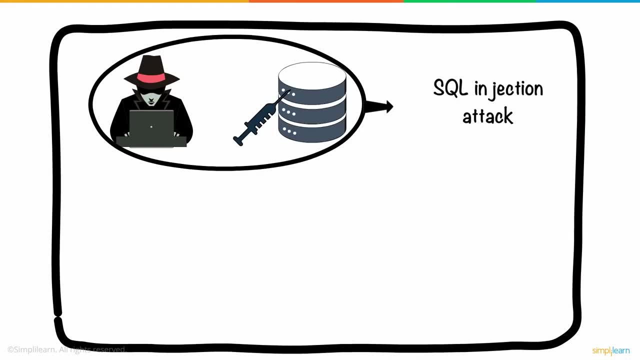 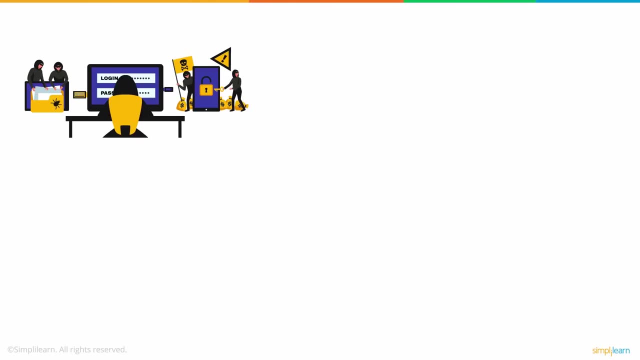 when multiple systems are used to launch the attack. When a hacker manipulates a standard SQL query in a database-driven website, it is known as a SQL injection attack. By doing so, hackers can view, edit and delete tables from databases. Amidst a plethora of cyber attacks, it is indeed a challenge for organizations with several networks in front of them. 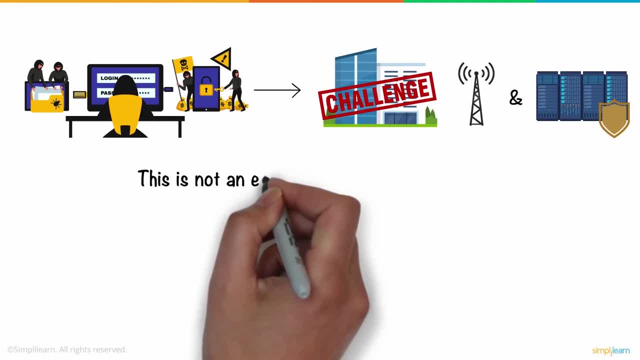 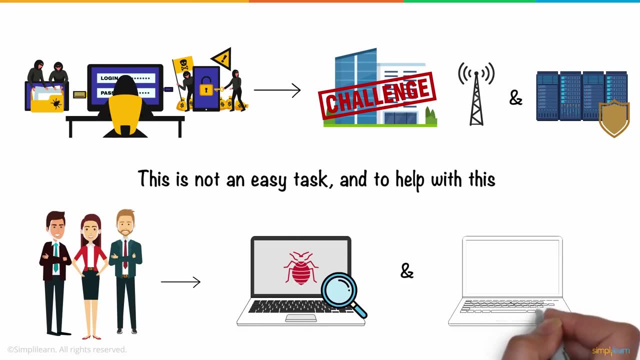 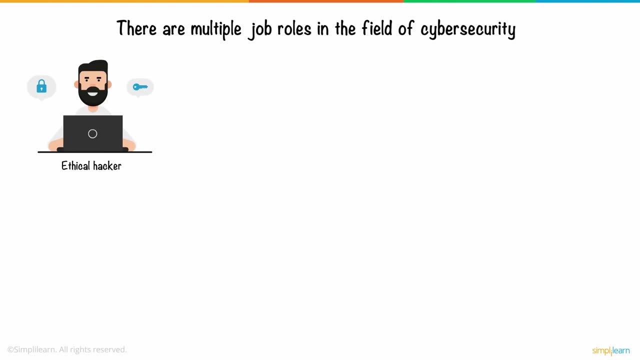 This is not an easy task, and to help with this, cybersecurity professionals are hired to work on identifying cyber threats and securing a company's network. There are multiple job roles in the field of cybersecurity. If hacking fascinates you, then the role of an ethical hacker is something to be explored. 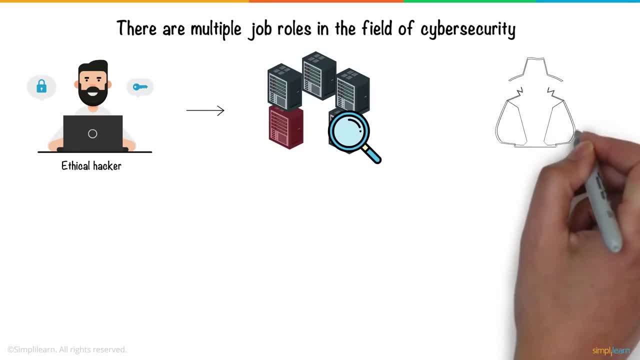 Such professionals try to explore a network's vulnerabilities just like how a hacker would do, but only to identify those vulnerabilities and resolve them. If you are looking for protection against an actual cyber attack, but if you are looking to design robust security structures, 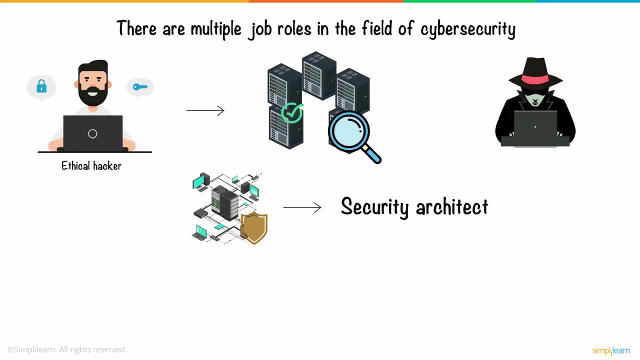 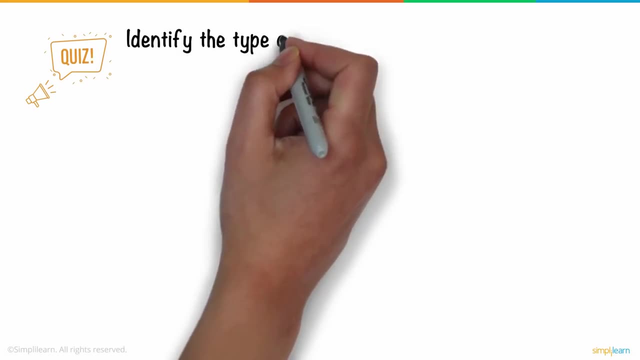 then the role of a security architect is more apt. A chief information security officer plays a crucial role in enterprise security and is entrusted with the overall safety of the information in an organization. So here's a question for you: Identify the type of cyber attack where the hacker's system takes over the client's IP address? 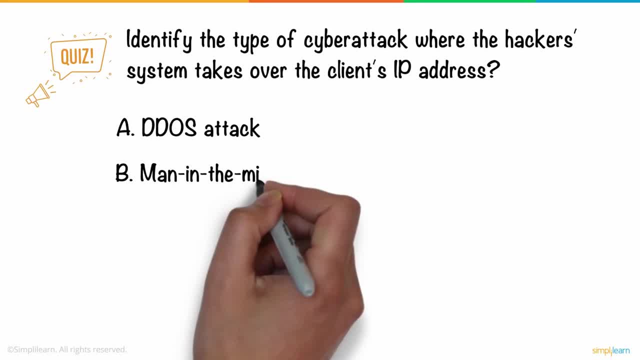 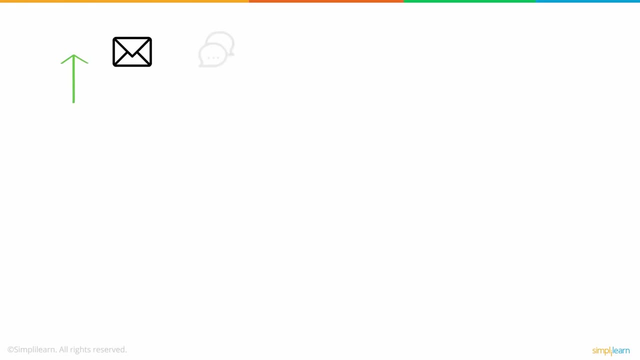 A- DDoS attack. B- Man-in-the-middle attack. C- Phishing attack. D- Password attack. Give it a thought and leave your answers in the comments section below. Three lucky winners will receive Amazon gift vouchers. With the increase in the production of global digital data, 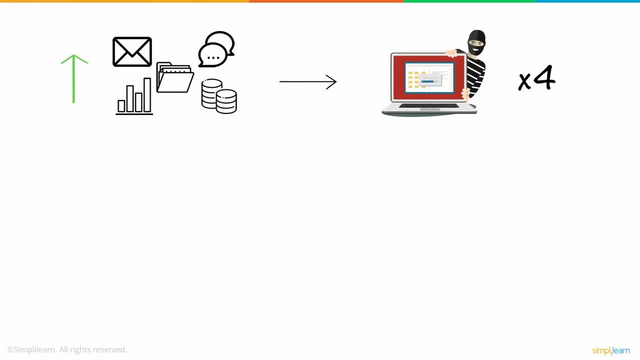 it is anticipated that cyber attacks will quadruple in the near future. Organizations are going to need cybersecurity professionals who can prevent these attacks. A career in the field of cybersecurity is lucrative and a very smart decision for professionals now. So what are you waiting for? 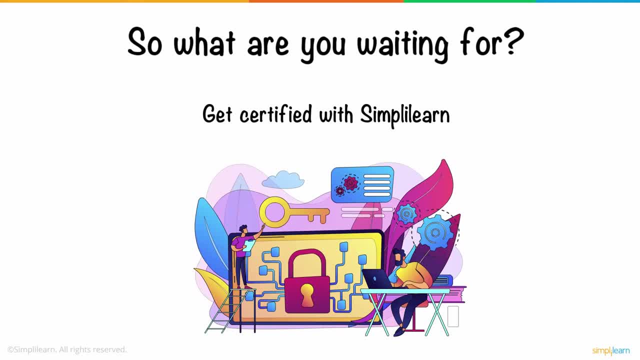 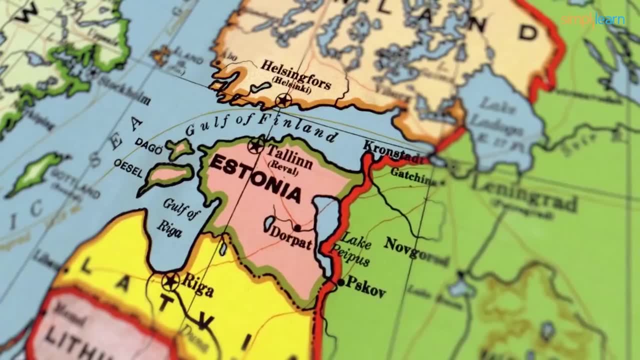 Get certified with SimplyLearn and become a cybersecurity expert. In this video, we bring you the top 10 computer hacks of all time. Let's see what we have at number 10.. From April 27, 2007,: Estonia, the European country. 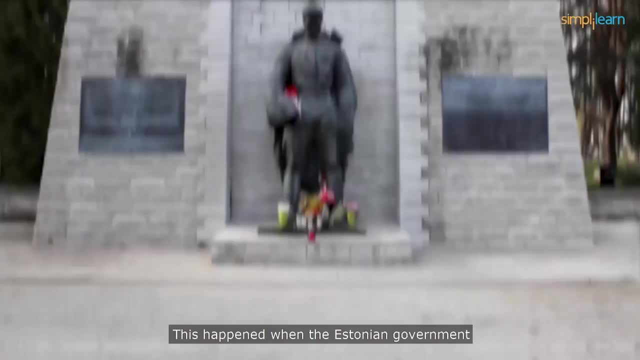 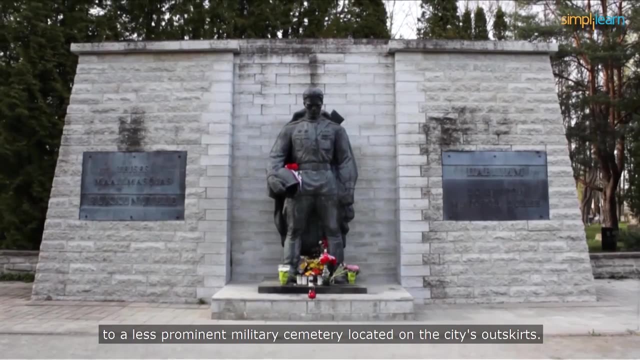 faced a series of cyber attacks that lasted for weeks. This happened when the Estonian governor Mendesaiter to move the bronze soldier from Tallinn Center to a less prominent military cemetery located on the city's outskirts. Unprecedented levels of internet traffic took down Estonian. 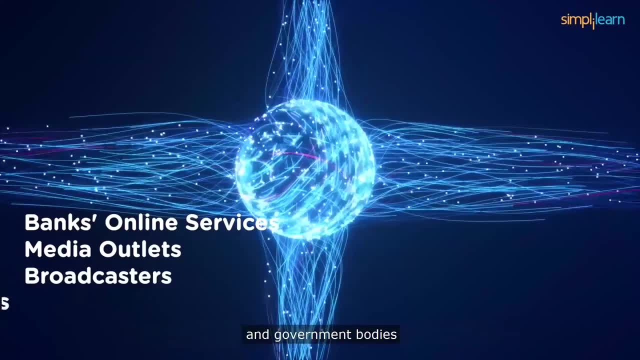 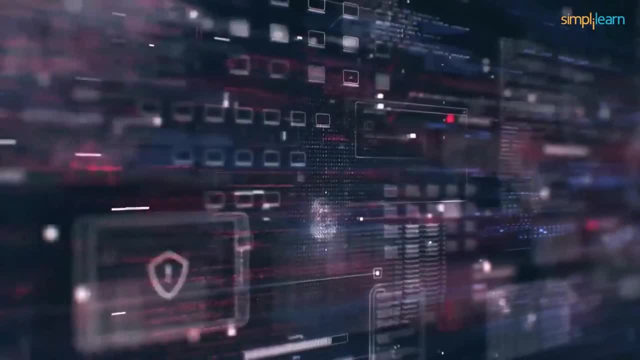 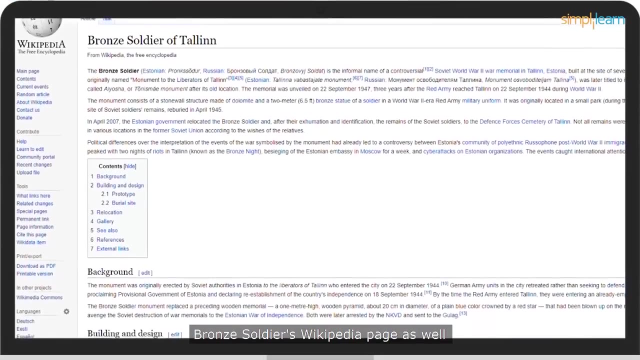 banks' online services, media outlets, broadcasters and government bodies. Botnet sent massive waves of spam and vast amounts of automated online requests. According to researchers, the public faced DDoS attacks. There were conflicts to edit the English-language version of the bronze soldier's Wikipedia page as well, Although there is no confirmation, Russia is believed to be behind these cyber attacks that largely crippled the Estonian society. Let's now move on to the next attack. On December 23, 2015,, several parts of Ukraine witnessed a power outage. 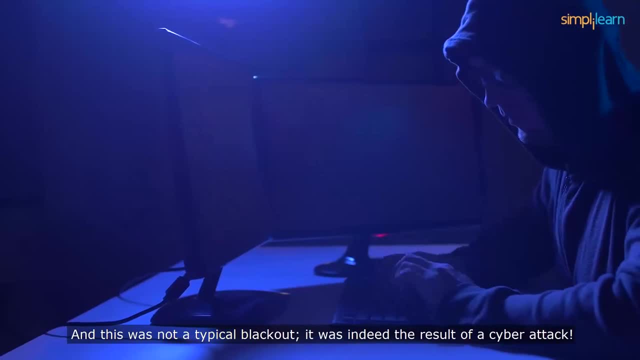 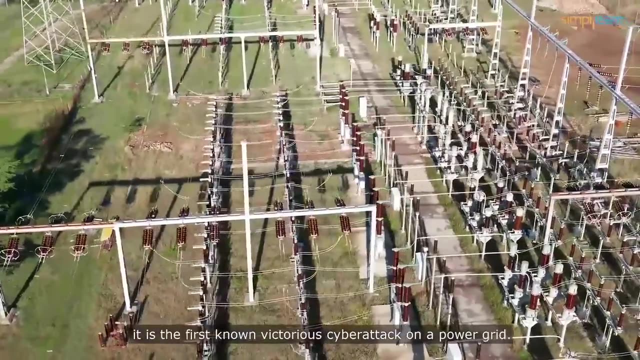 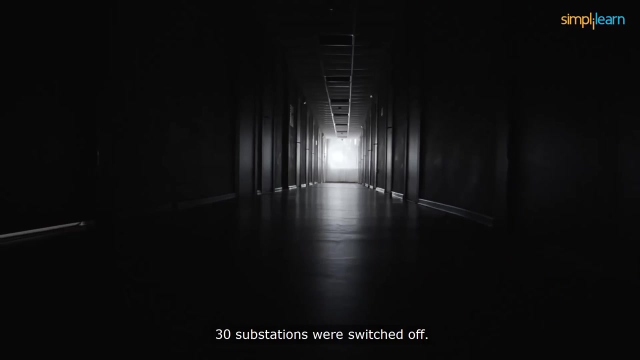 And this was not a typical blackout. It was indeed the result of a cyber attack. Information systems of three energy distribution companies in Ukraine were compromised. It is the first known victorious cyber attack on a power grid. Russia sent out phishing emails to the power companies. 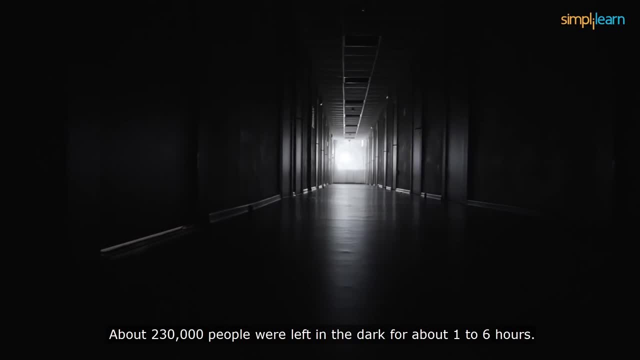 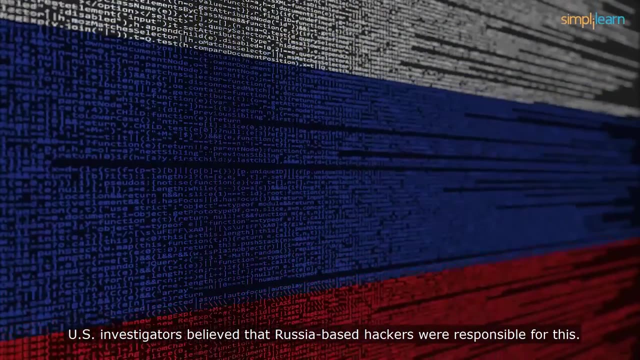 30 substations were switched off and about 230,000 people were left in the dark for about 1-6 hours. US investigators believed that Russia-based hackers were responsible for this. Experts have warned that other countries could also be vulnerable to such attacks. 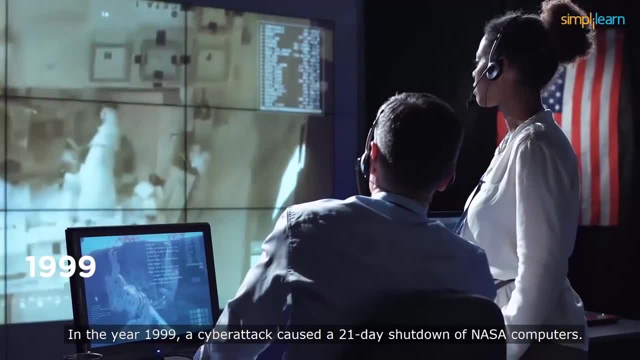 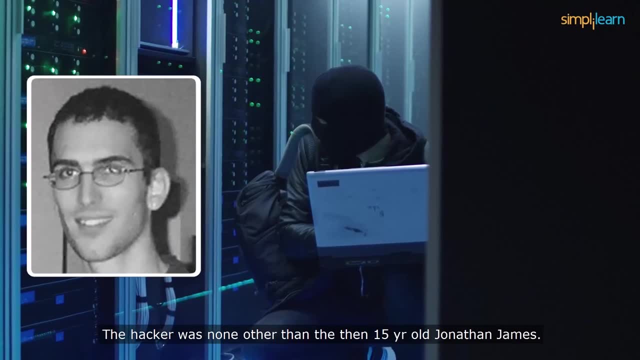 Let's see what we have at number 8.. In the year 1999, a cyber attack caused a 21-day shutdown of NASA computers. Unbelievable, isn't it? There was none other than the then-15-year-old Jonathan James. 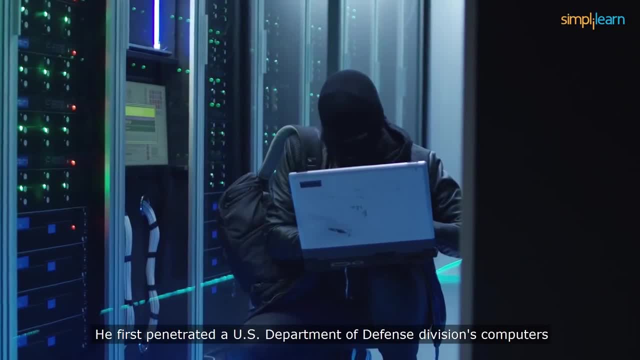 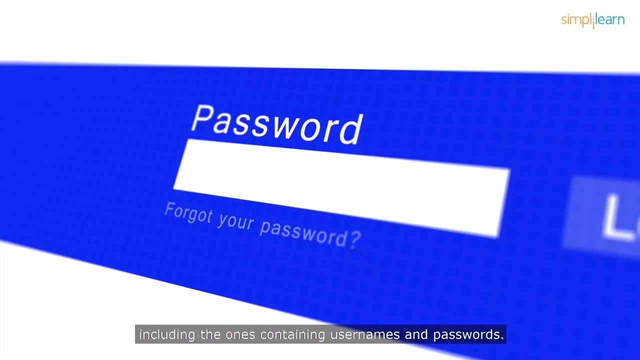 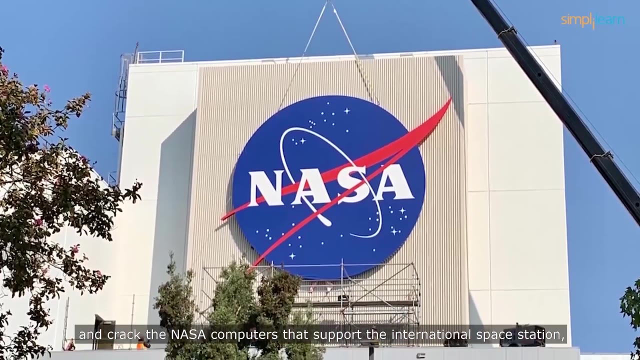 He first penetrated US Department of Defense Division's computers and installed a backdoor on its servers. This allowed him to intercept more than 1,000 government emails, including the ones containing usernames and passwords. This helped James steal a piece of NASA software and crack the NASA computers that support the International Space Station. which cost the space exploration agencies $41,000,, and he was the first person to carry out a computer hack against the American Space Agency. Let's now move on to the next attack. In late November 2014,, there was a leak of confidential data from the film studio of Sony Pictures. 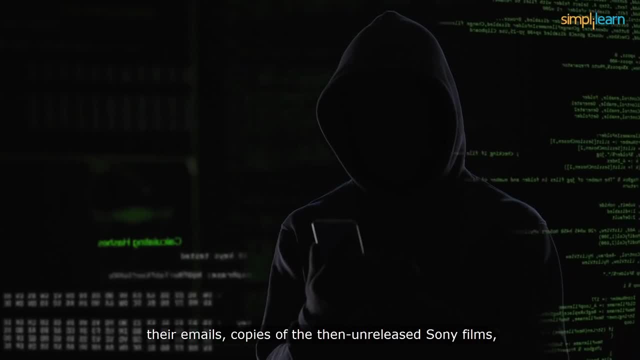 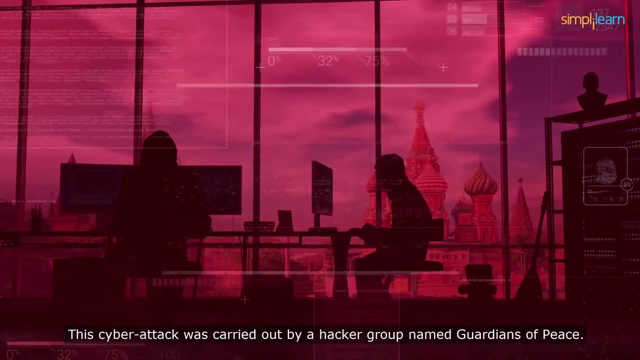 Information about Sony Pictures' employees, their emails, copies of the then-unreleased Sony films, future propositions and other crucial data were leaked. This cyber attack was carried out by a hacker group named Guardians of Peace. So what did the hackers want? 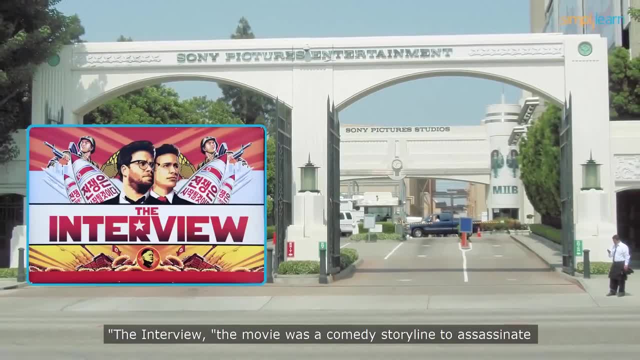 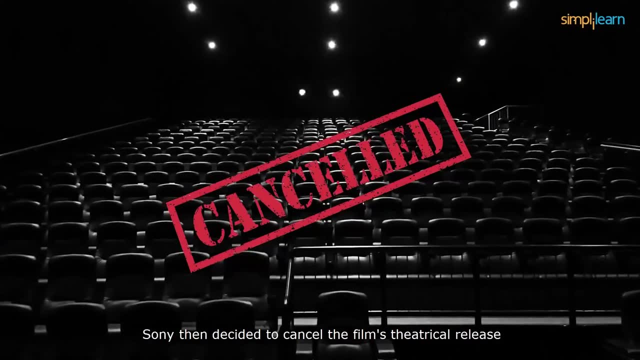 Well, they demanded that Sony withdraw its then-upcoming movie, The Interview. This movie was a comedy storyline to assassinate the North Korean leader, Kim Jong-un. Sony then decided to cancel the film's theatrical release due to the threats at cinema screening the movie. 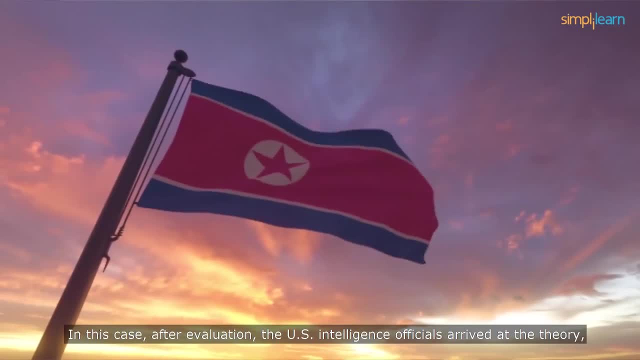 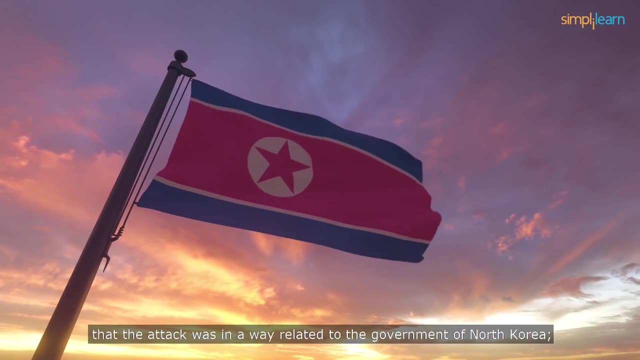 It is indeed hard to trace the roots of a cyber attack. In this case, after evaluation, the US intelligence officials arrived at the theory that the attack was in a way related to the government of North Korea. However, North Korea had denied the same. 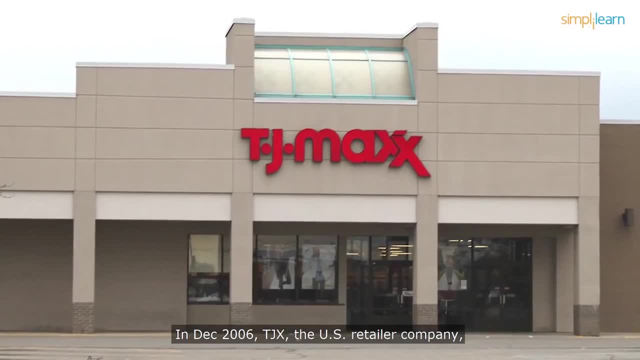 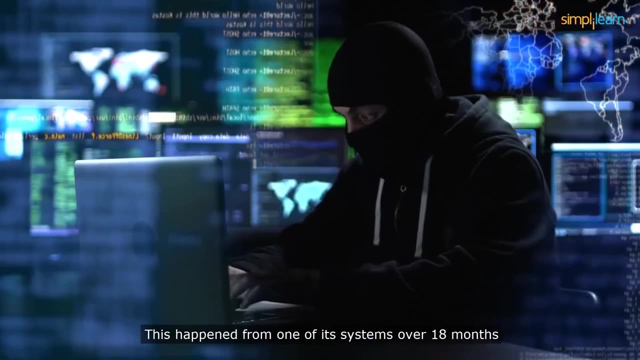 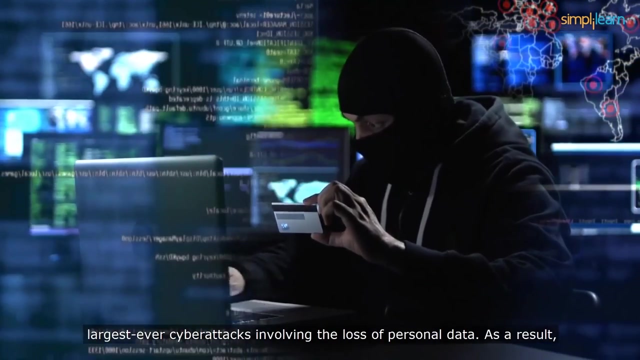 In December 2006, TJX, the US retailer company, identified that 45.6 million debit and credit card details were stolen. This happened from one of its systems over 18 months by an unknown number of intruders. It was one of the first largest-ever cyber attacks involving the loss of personal data. As a result, banks in the affected regions had to reissue and block thousands of payment cards. A group of hackers did this, Albert Gonzalez being the mastermind. The group was from Miami, the place where the TJX heist was believed to have originated. 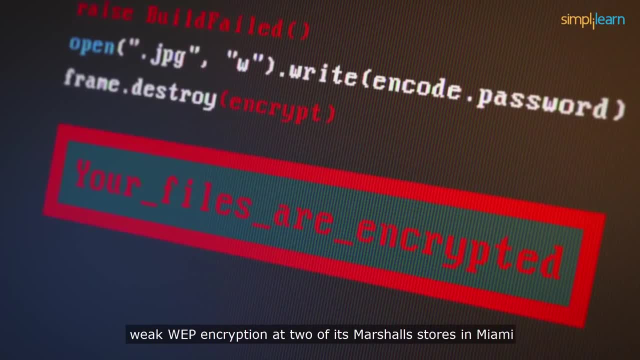 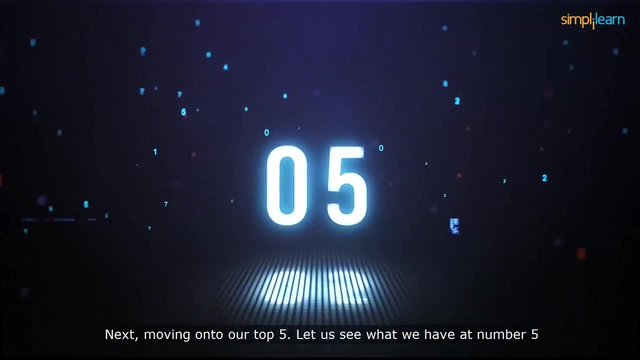 Reports said that the TJX data breach occurred because of weak web encryption at two of its martial stores in Miami. Next, moving on to our top five, let us see what we have at number five. The year 2010 witnessed the discovery of the deadly computer worm Stuxnet. 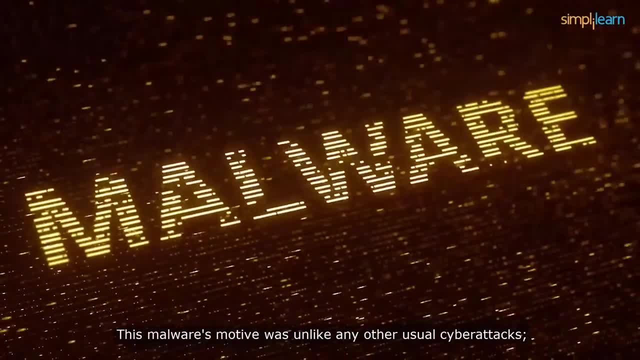 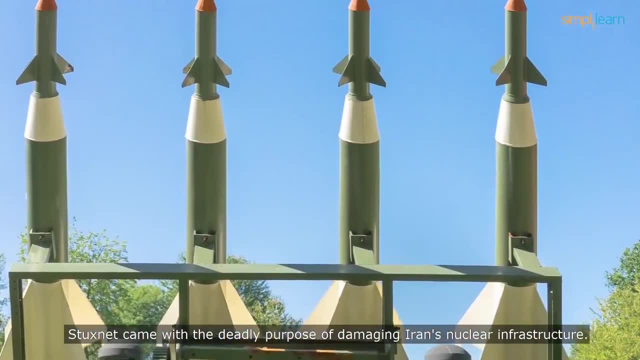 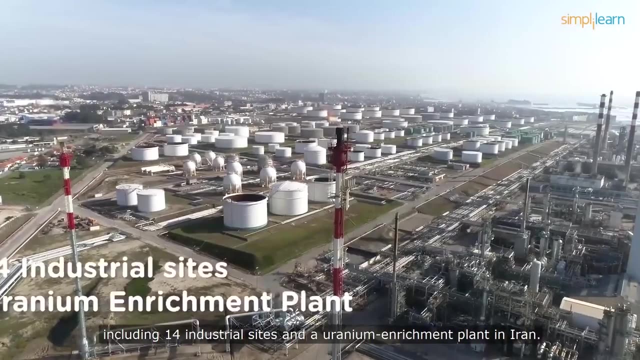 This malware's motive was unlike any other usual cyber attacks. It aimed at destructing the equipment the computer used. computers controlled Stuxnet came with the deadly purpose of damaging Iran's nuclear infrastructure. It infected more than 200,000 computers, including 14 industrial sites and 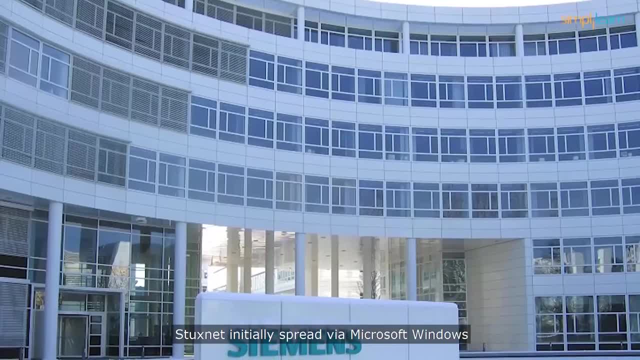 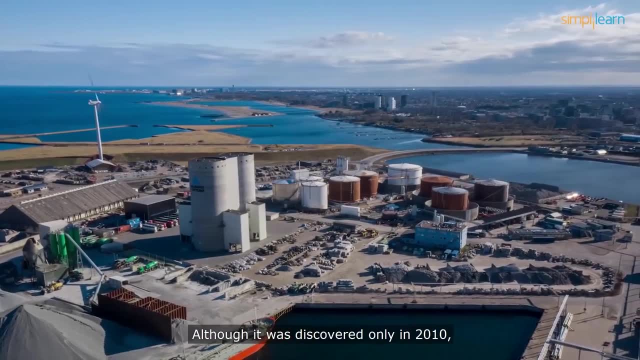 a uranium enrichment plant in Iran. Stuxnet initially spread via Microsoft Windows and targeted Siemens' industrial control systems. Although it was discovered only in 2010,, it is believed to have been silently sabotaging Iran's nuclear facilities. It was one of 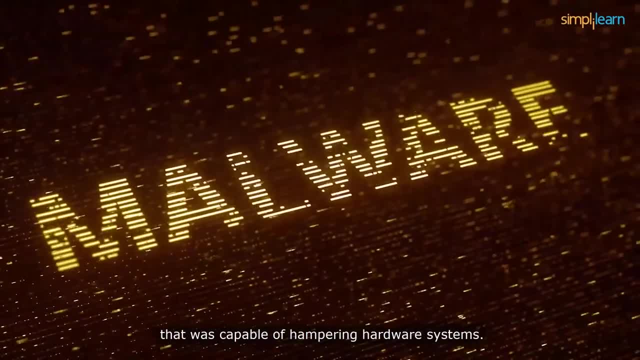 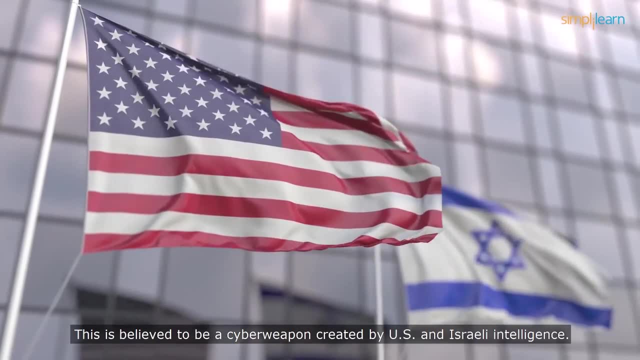 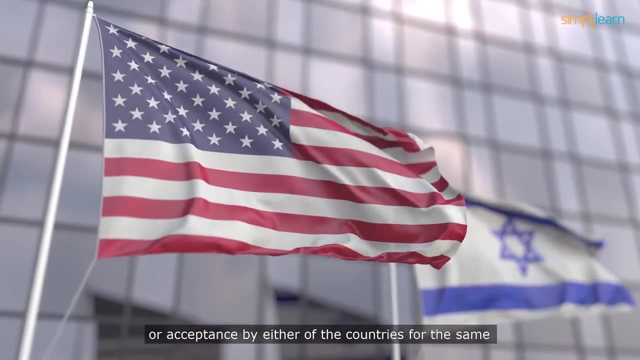 the first discovered malware that was capable of hampering hardware systems. It largely damaged the centrifuges of the Iranian reactors. This is believed to be a cyber weapon created by the US and the Israeli intelligence, although there is no documented evidence or acceptance by either of the countries for the same. Moving on to number 4.. In the year 2014,, Home Depot was the victim of one of the deadliest cyber attacks: 56 million payment cards were compromised, along with 53 million customer emails. This security breach happened from April to September 2014.. Criminals were believed. 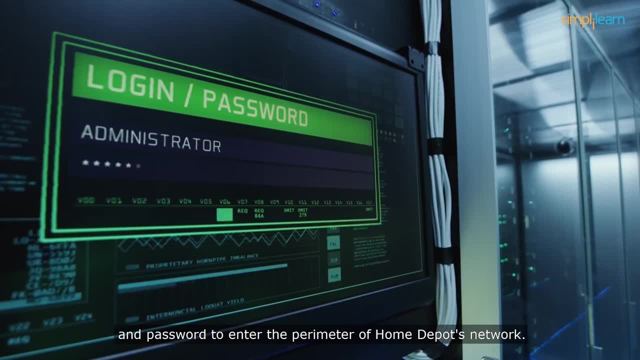 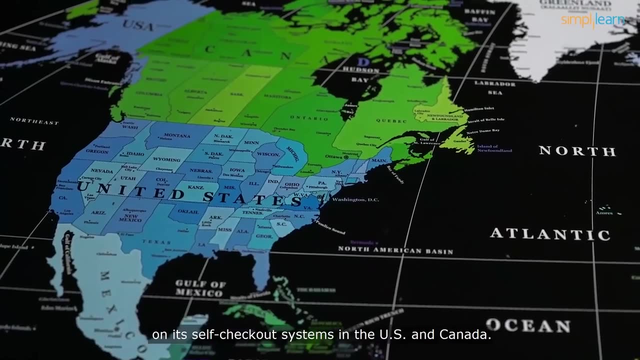 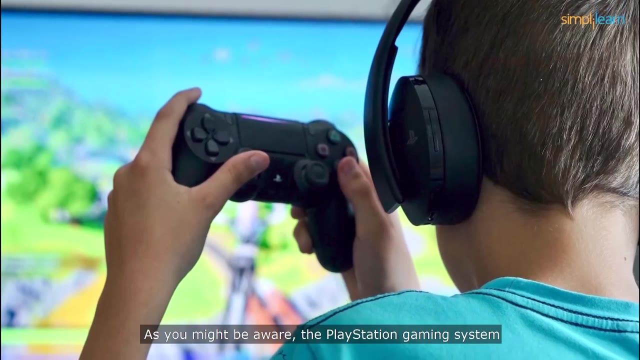 to have used a third-party vendor's username and password to enter the perimeter of Home Depot's network. The attackers were then able to deploy custom-built malware on its self-checkout systems in the US and Canada. Moving on to our top 3.. As you might be aware, the PlayStation gaming 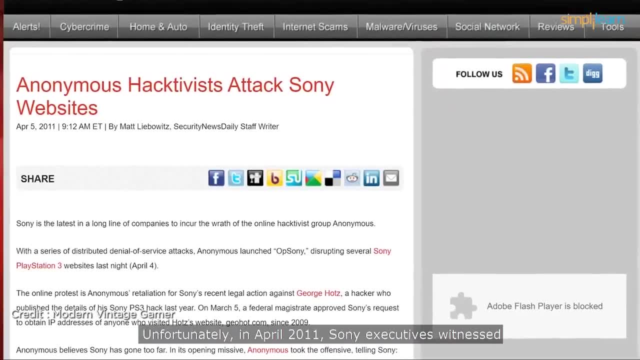 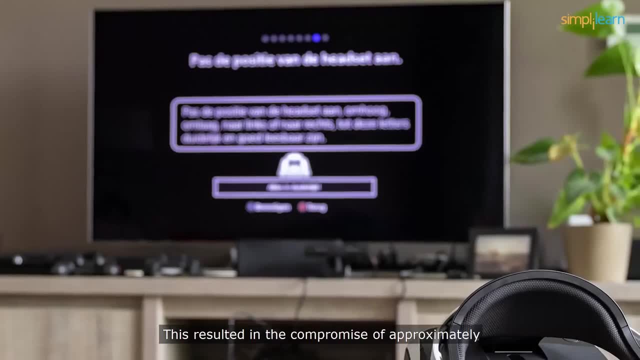 system is one of Sony's most popular products. Unfortunately, in April 2011,, the PlayStation games were banned from the PlayStation Network. However, in July 2011,, Sony executives witnessed abnormal activity on the PlayStation Network. This resulted in the compromise of approximately. 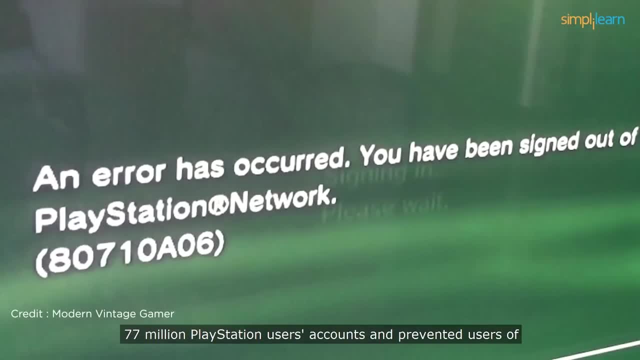 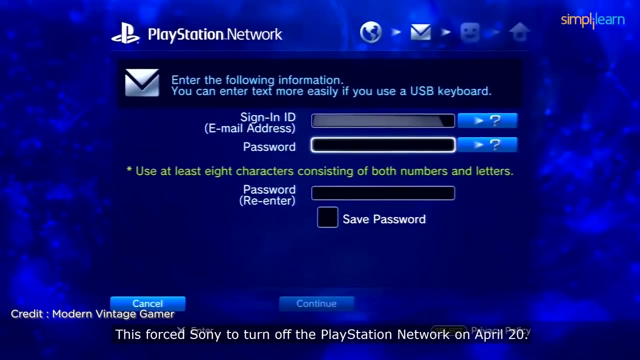 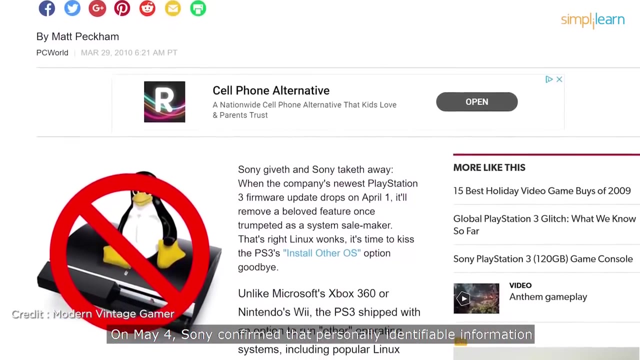 77 million PlayStation users' accounts and prevented users of PlayStation 3 and PlayStation Portable consoles from accessing the service. This forced Sony to turn off the PlayStation Network on April 20.. On May 4,, Sony confirmed that personally identifiable information from each of the 77 million accounts had been exposed. The outage of the PlayStation Network on May 4 was found to be the result of the PlayStation games being banned from PlayStation 3 and PlayStation Portable consoles. On May 4, Sony confirmed that personally identifiable information from each of the 77 million accounts had been exposed. 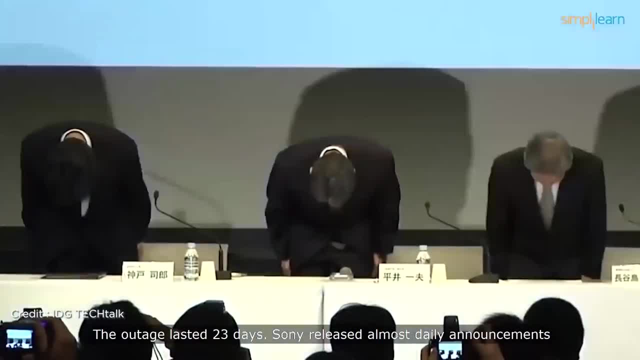 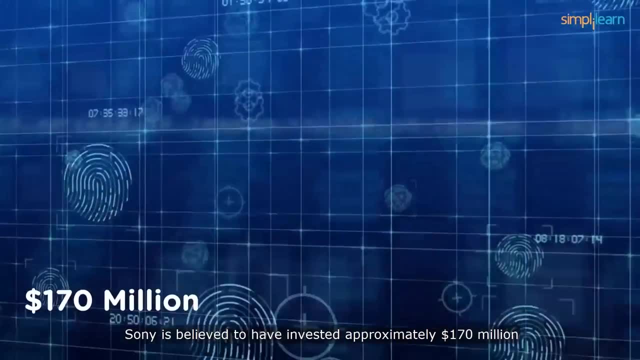 The usage lasted for 23 days. Sony released almost daily announcements concerning the system outage. In the end, Sony is believed to have invested approximately $170 million to improve the network's security, to investigate the attack and to cover the expenses of caring for the 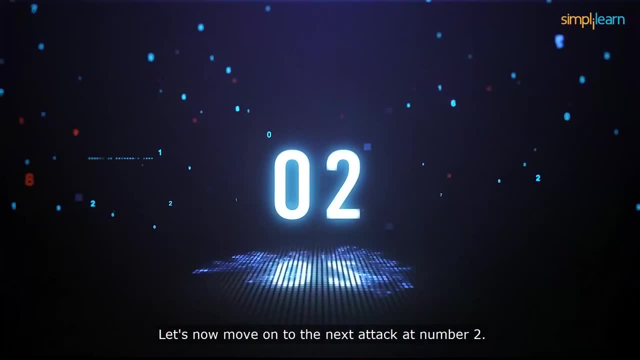 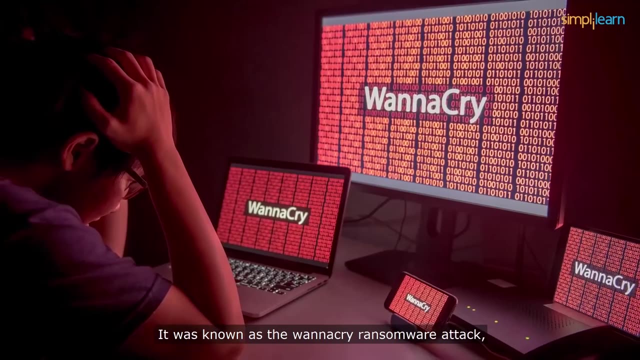 consumers that had been affected. Let's now move on to the next attack, at number 2.. In May 2017, one of the most dangerous cyberattacks took place. It was known as the WannaCry ransomware attack, caused by the WannaCry cryptoworm. 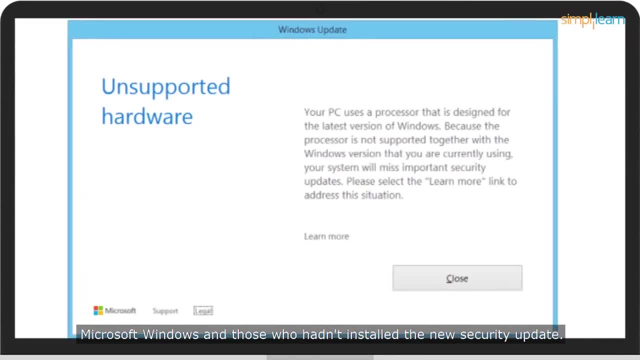 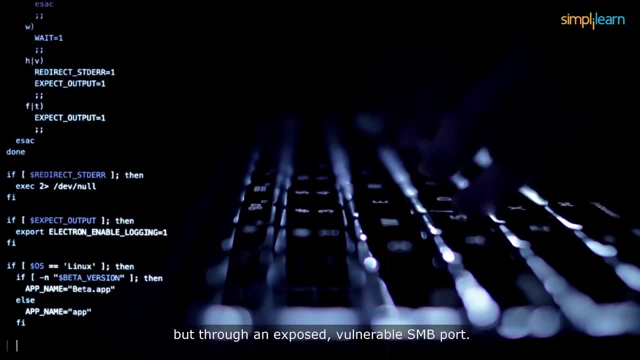 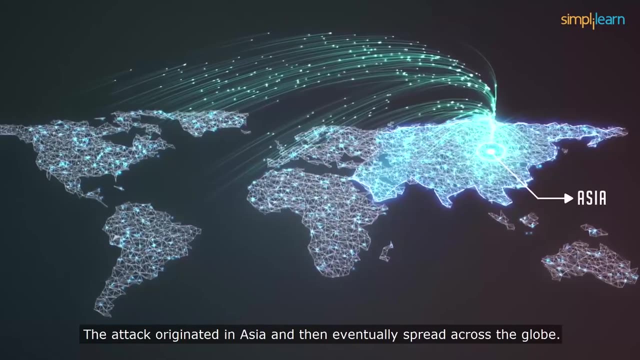 The victims were the users that used the unsupported version of Microsoft Windows and those who hadn't installed the new security update. This did not take place through phishing, like other attacks, but through an exposed, vulnerable SMB port. The attack originated in Asia and then eventually spread across the globe. 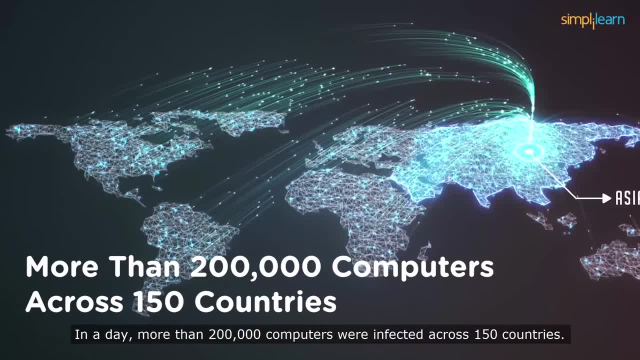 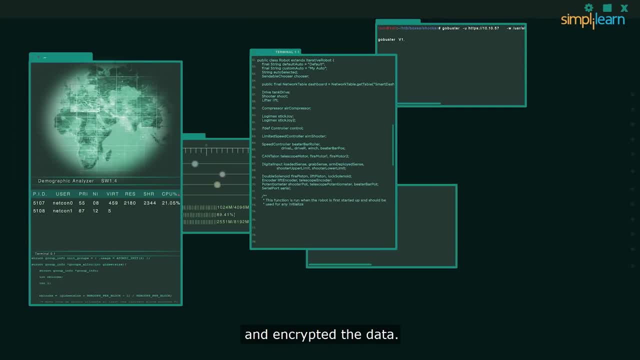 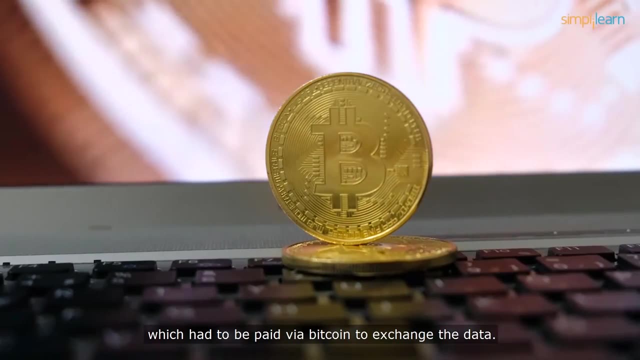 In a day, more than 200,000 computers were infected across 150 countries. The WannaCry cryptoworm locked the users out of the targeted systems and encrypted their data. The users were asked for a ransom of $300 to $600, which had to be paid via Bitcoin. in 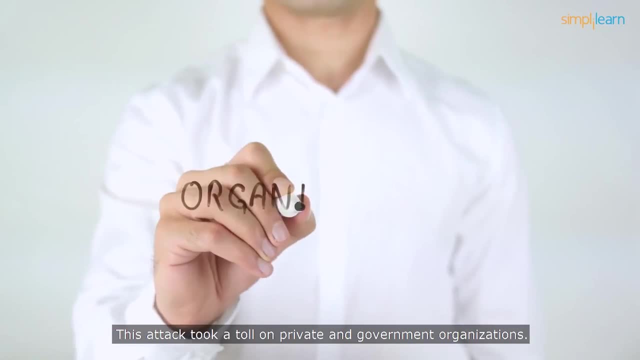 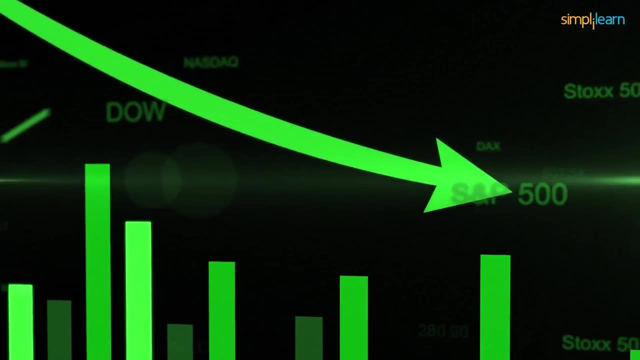 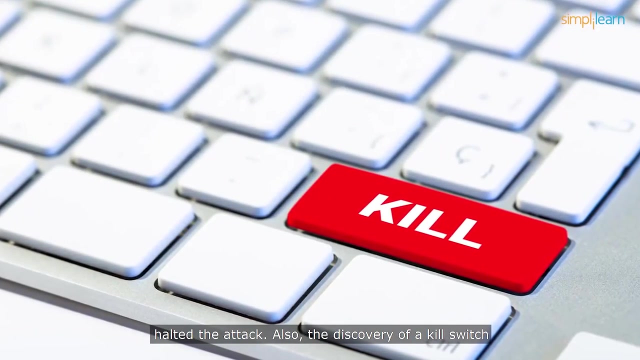 exchange for their data. This attack took a toll on both private and government organizations. It resulted in damages from hundreds of millions to billions of dollars In a matter of few days. the emergency patches released by Microsoft halted the attack. Also, the discovery of a kill switch by Microsoft. Microsoft, Microsoft, Microsoft, Microsoft. 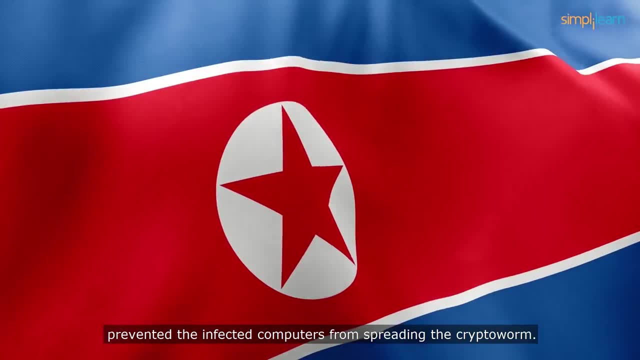 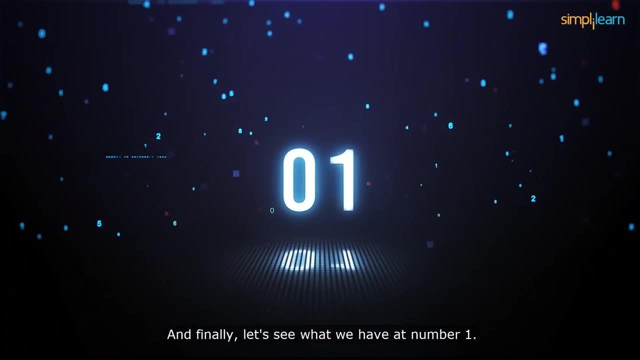 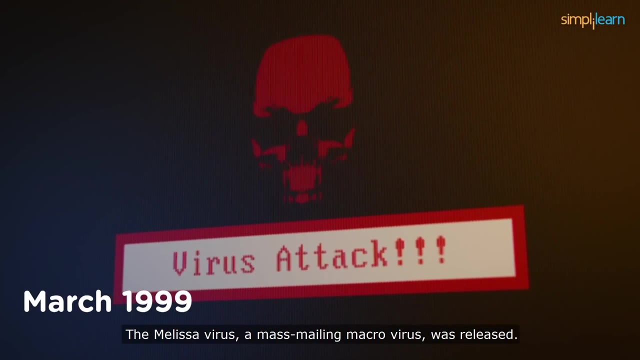 prevented the infected computers from spreading the cryptoworm. Security experts in a few countries believed that North Korea was behind this attack. And finally, let's see what we have at number 1.. More than two decades ago, in March 1999, the Melissa virus, a mass-mailing macrovirus. 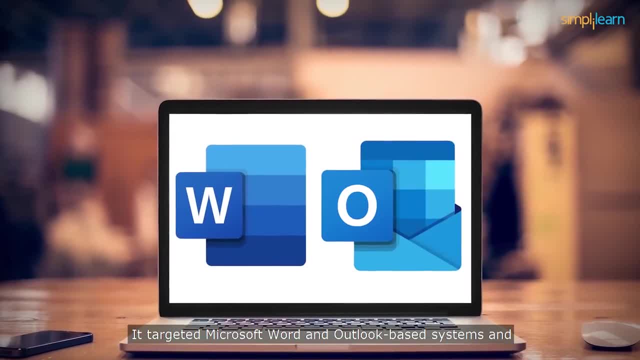 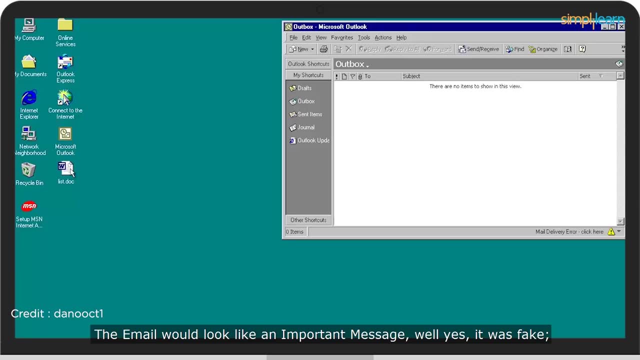 was released. It targeted Microsoft Word and Outlook-based systems and created considerable network traffic. Melissa virus infected computers via emails. The email would look like an important message, but it was not. The email would look like an important message, but it was not. 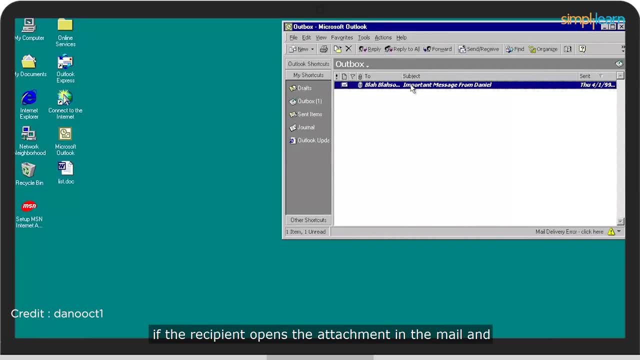 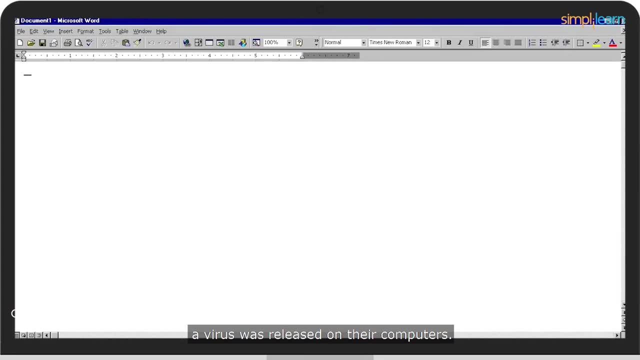 The email would look like an important message, but it was not. And a message? Well, yes, it was fake. If the recipient opens the attachments in the mail and downloads the document, then opens it with Microsoft Word. a virus was released on their computers. 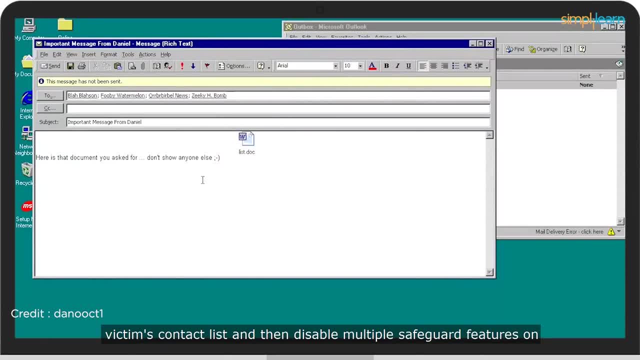 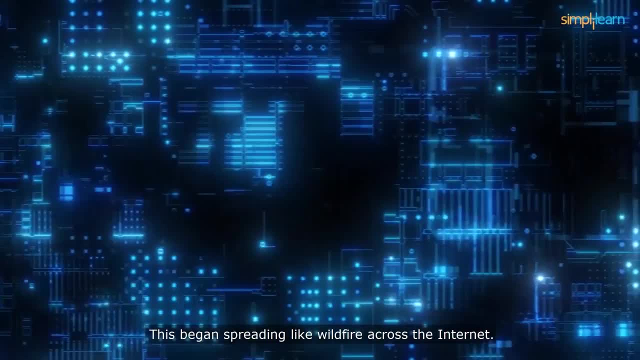 This would then mass-mail itself to the first 50 people on the victims' contact list and then disable multiple safeguard features on Microsoft Word and Microsoft Outlook. This began spreading like a wildfire across the Internet. David L Smith released the virus. The virus caused nearly 80 million deaths. 30 million- Yes, 20 million- damages. It did not steal data or money, However, it caused a havoc. Almost 1 million email accounts were disrupted, worldwide agencies were overloaded and some had to be shut down entirely, and internet traffic in some locations was slowed down. 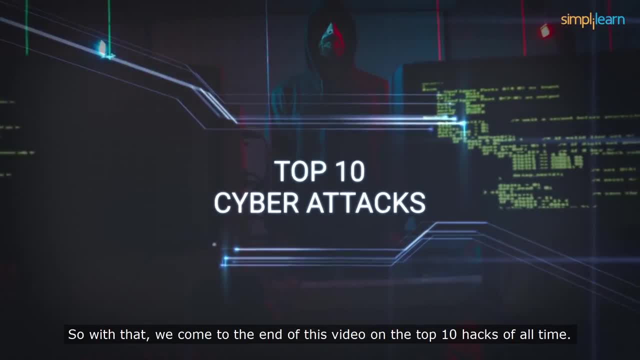 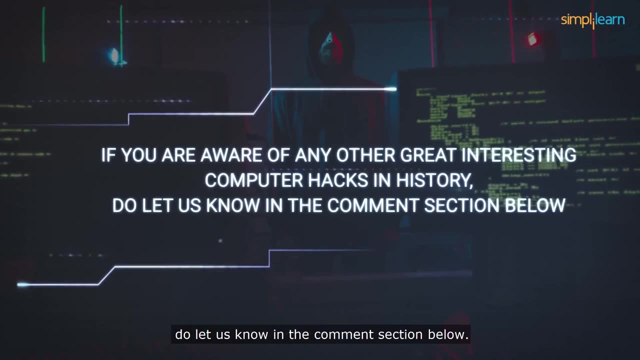 So with that we come to the end of this video on the top 10 computer hacks of all time. Do you agree with our list? If you are aware of any other great, interesting computer hacks in history, do let us know in the comment section below. 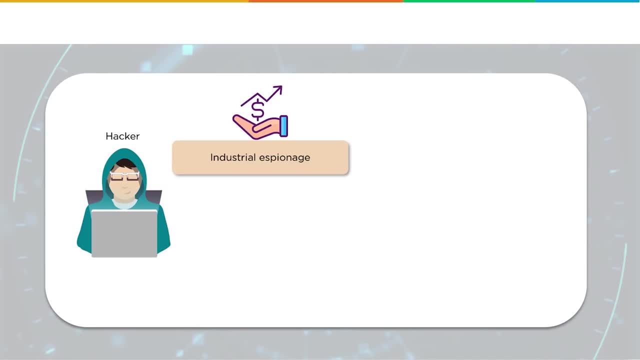 Let us know in the comment section below if you have any questions regarding this video. If you have any questions regarding this video, do let us know in the comment section below. If you have any questions regarding this video, do let us know in the comment section below. 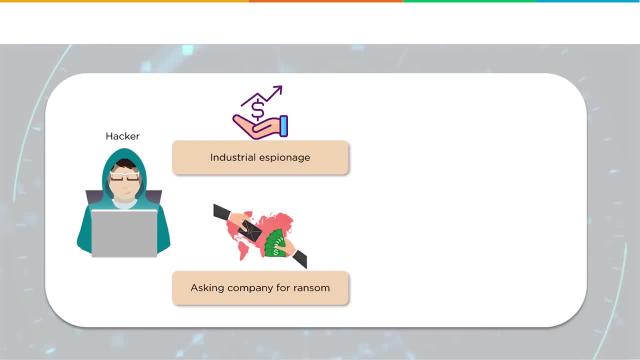 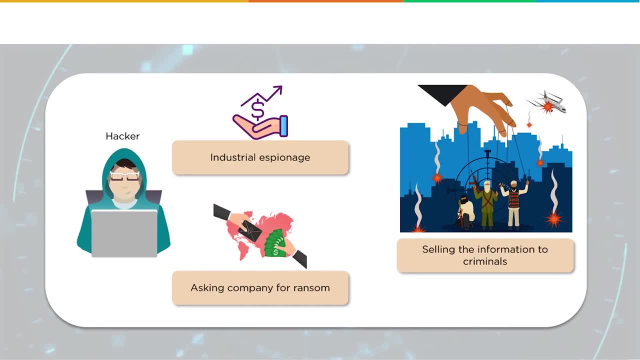 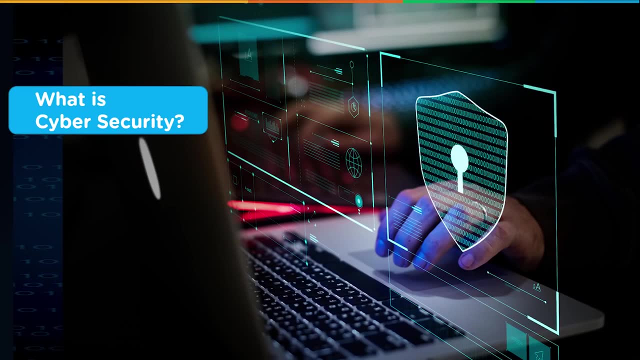 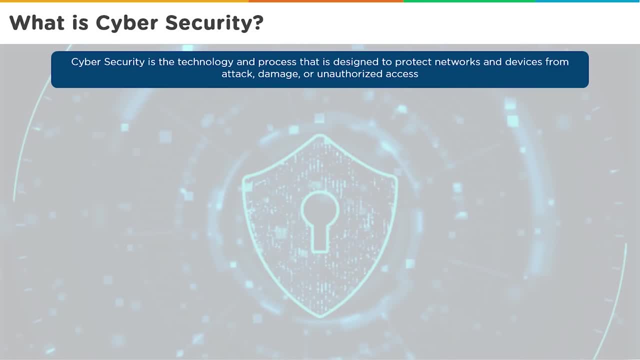 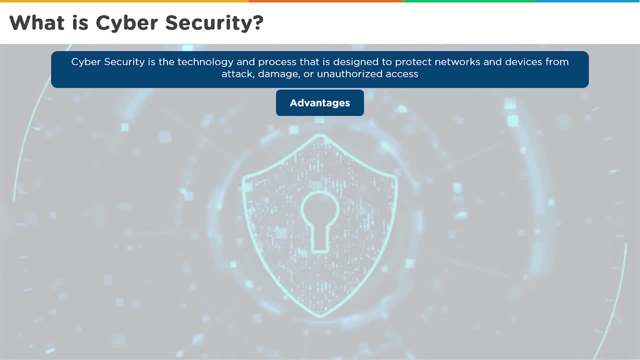 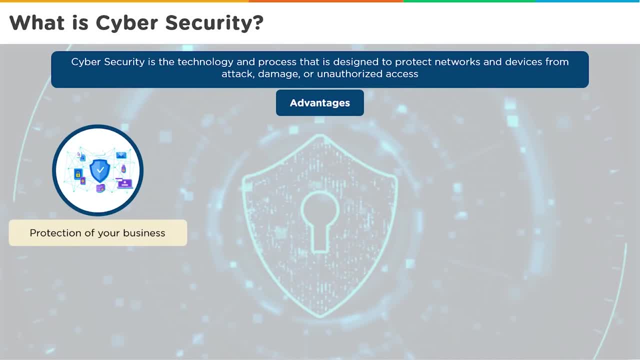 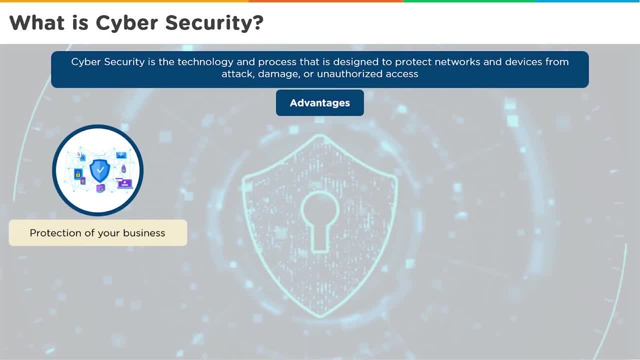 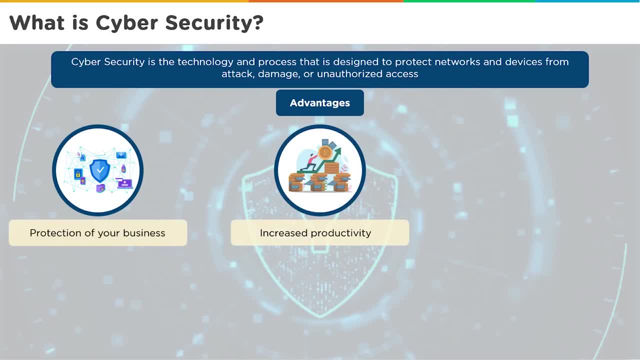 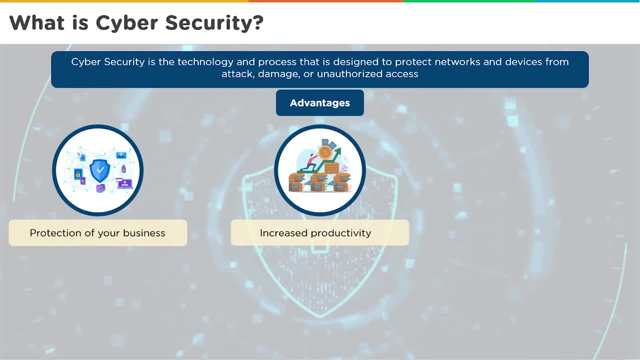 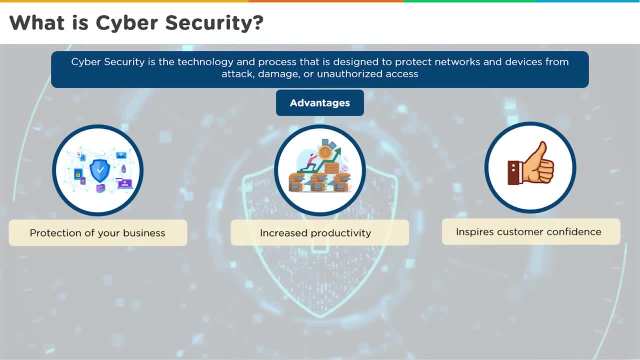 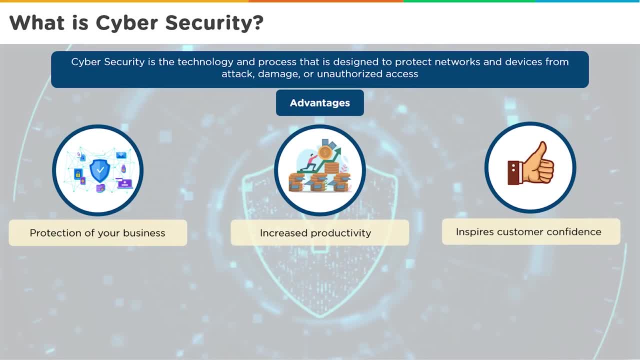 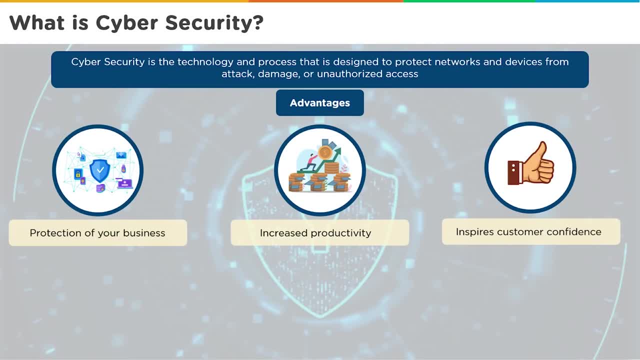 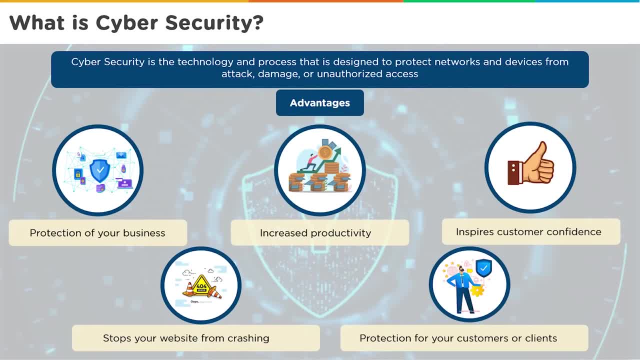 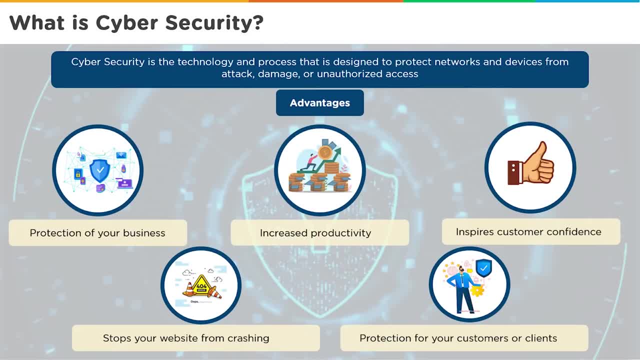 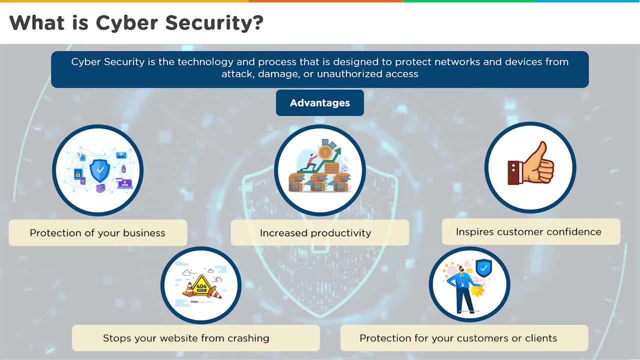 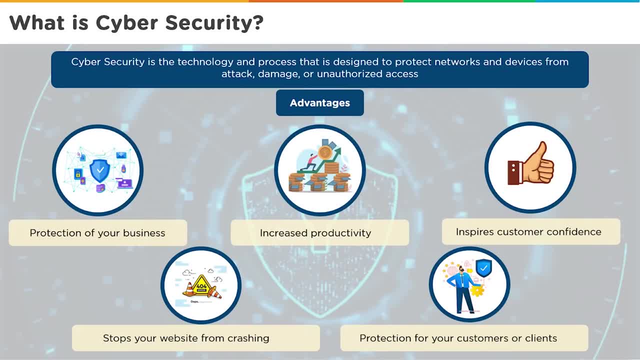 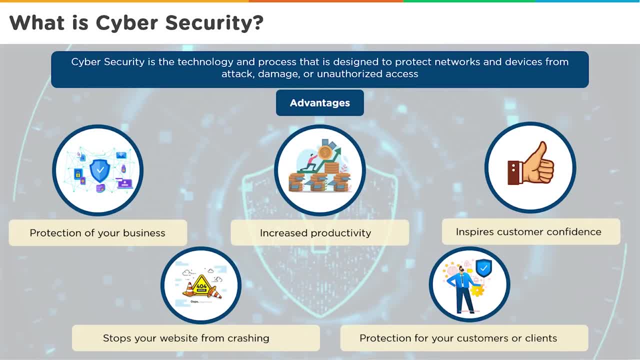 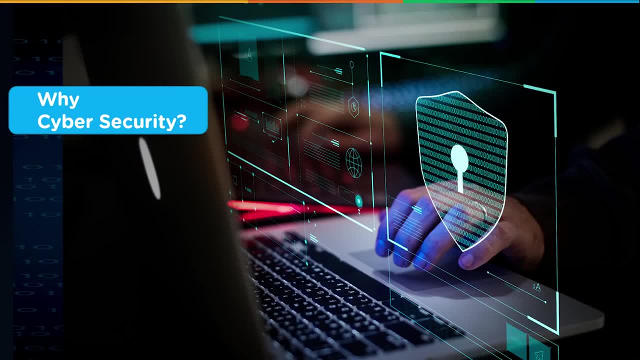 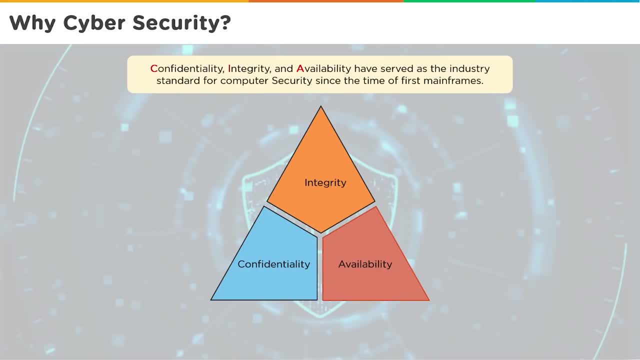 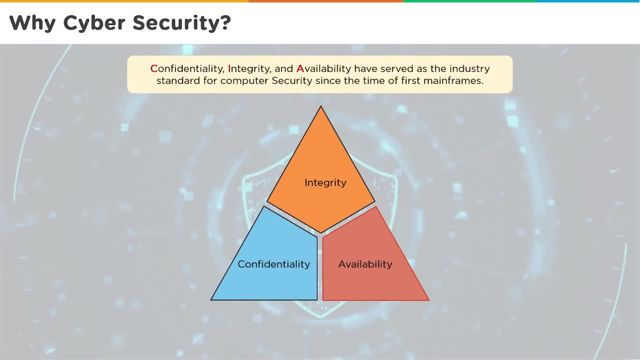 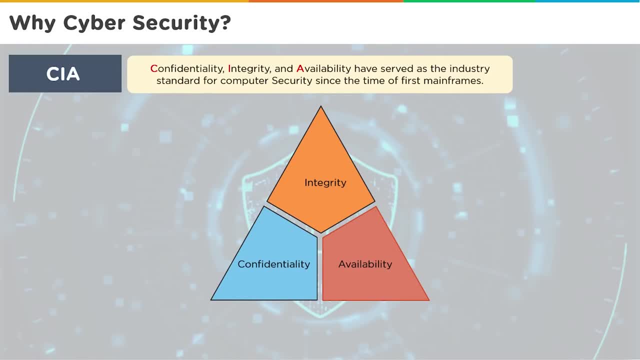 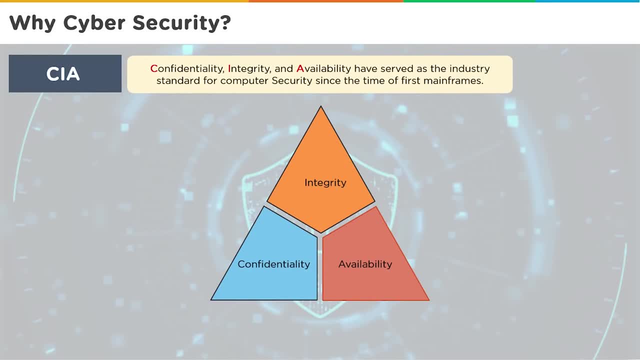 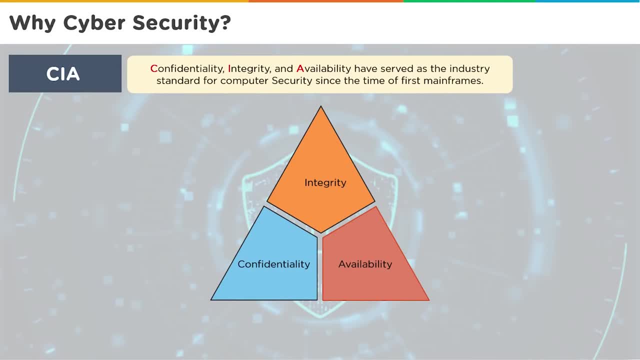 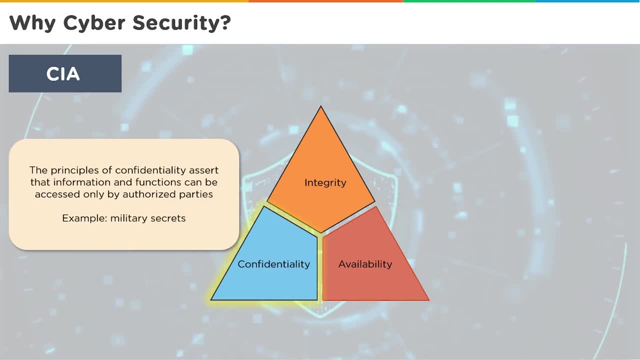 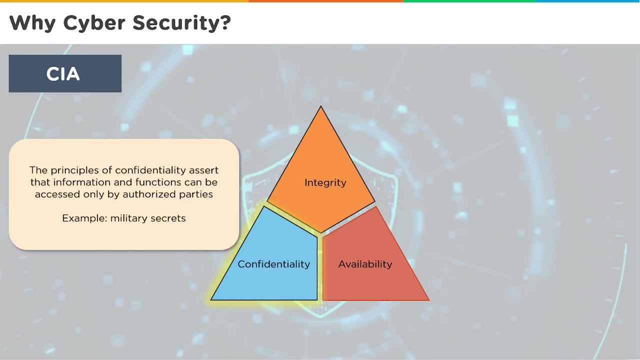 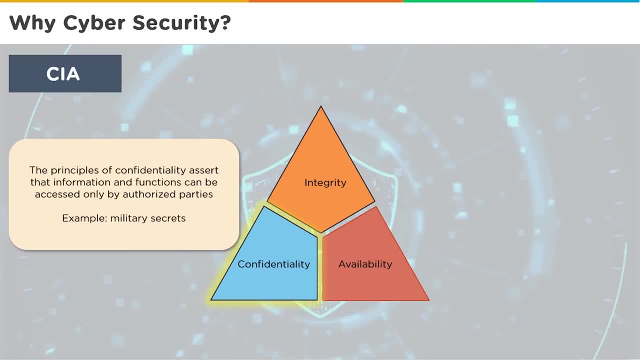 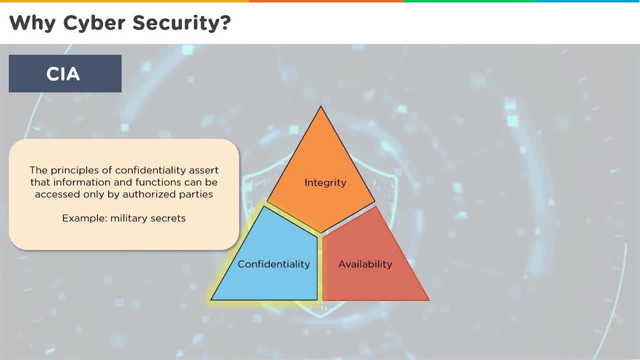 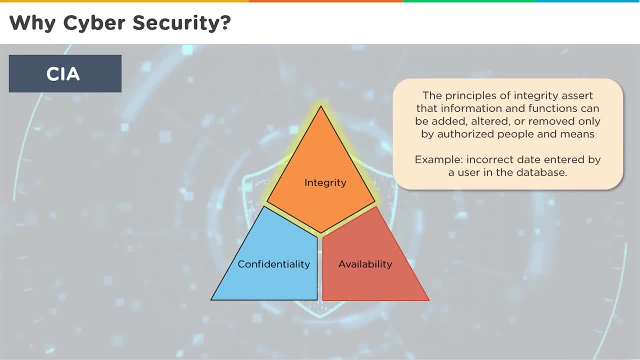 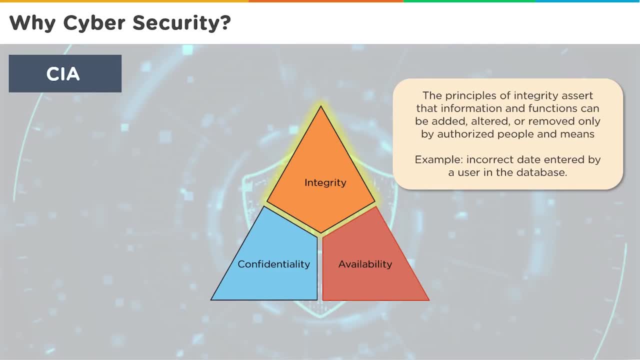 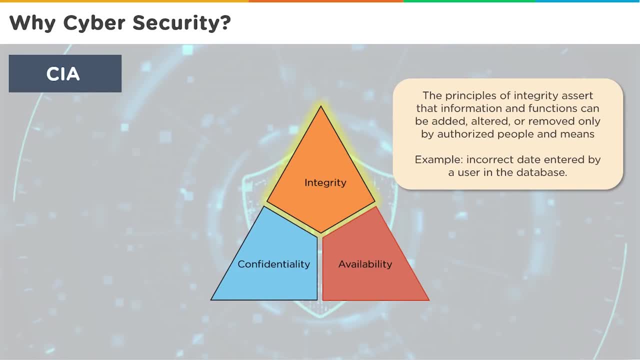 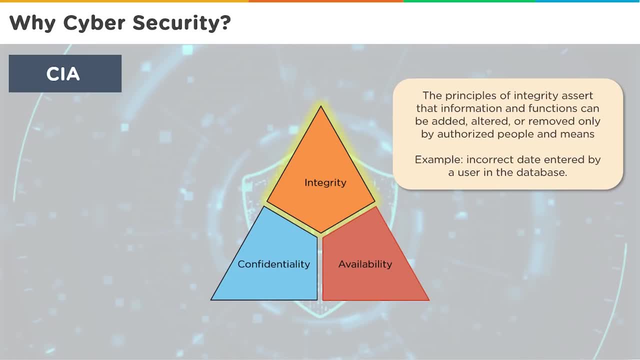 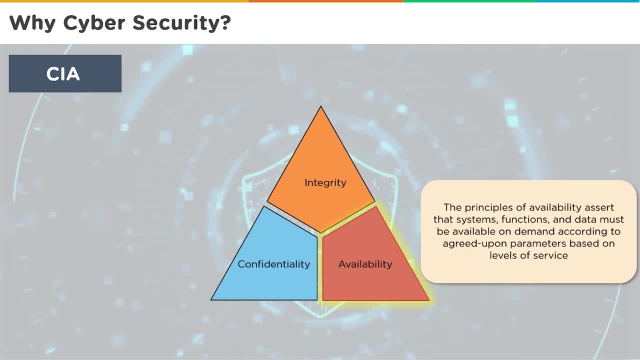 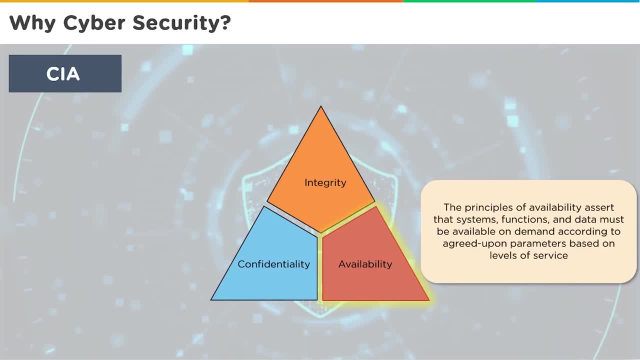 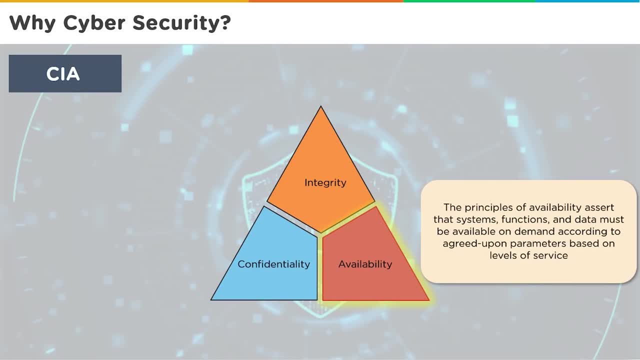 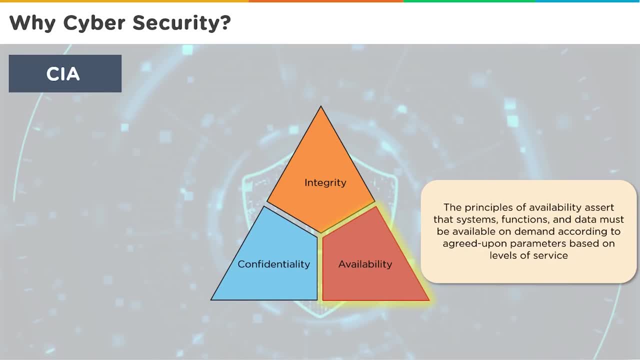 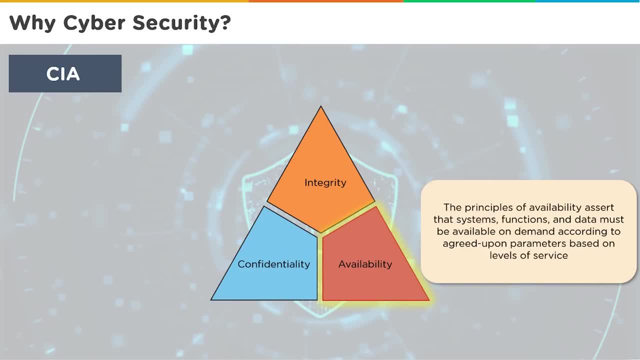 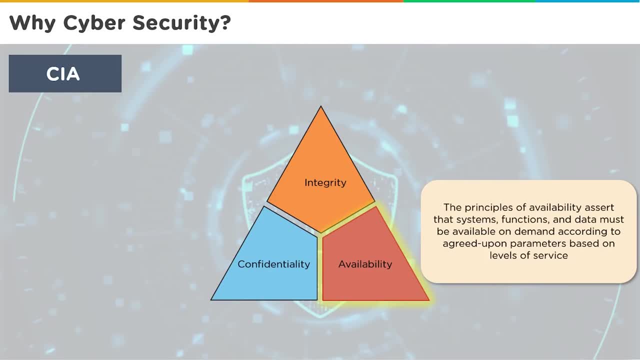 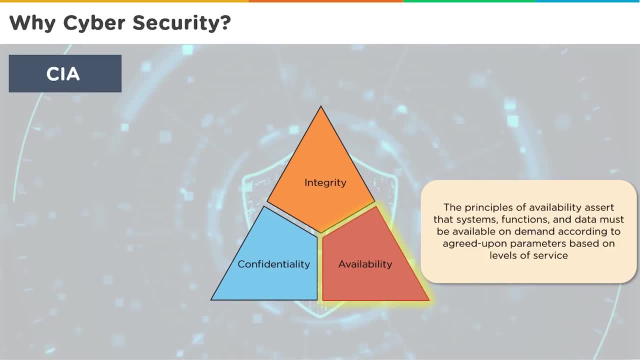 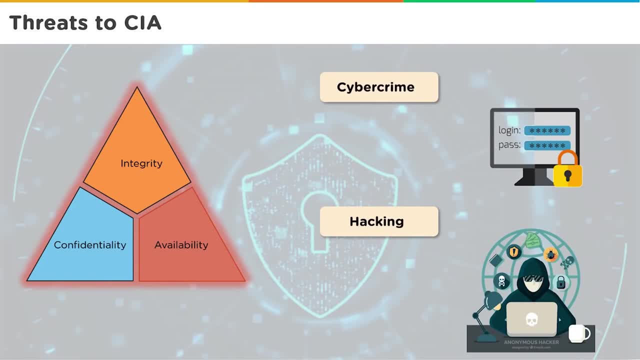 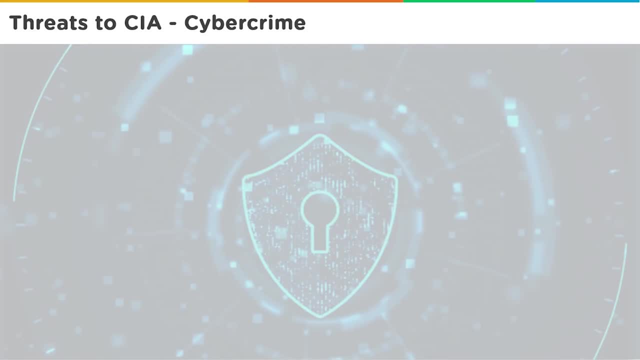 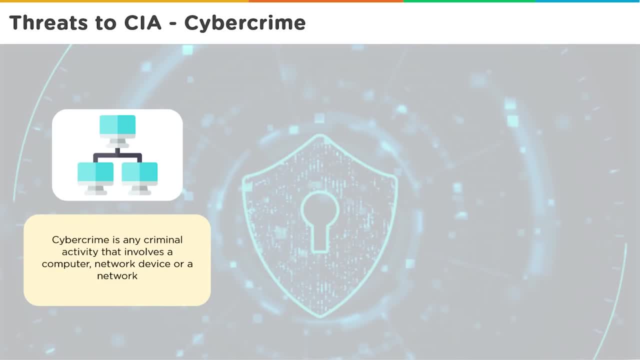 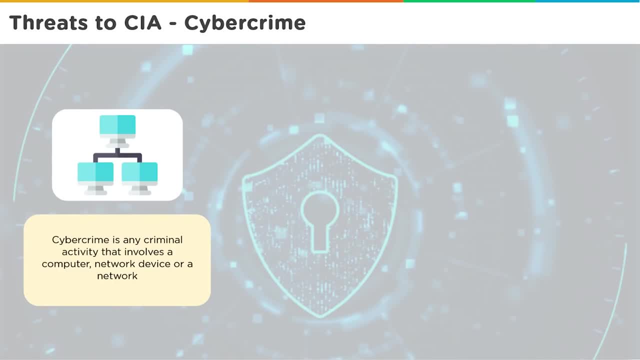 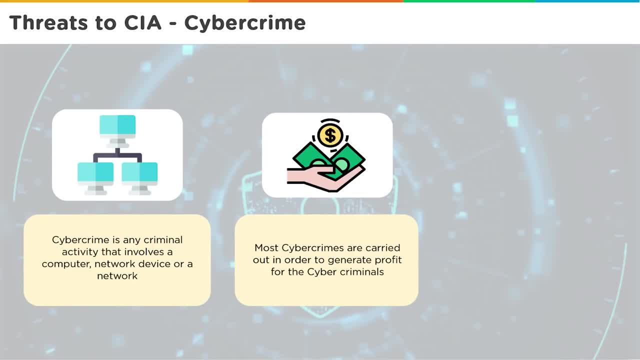 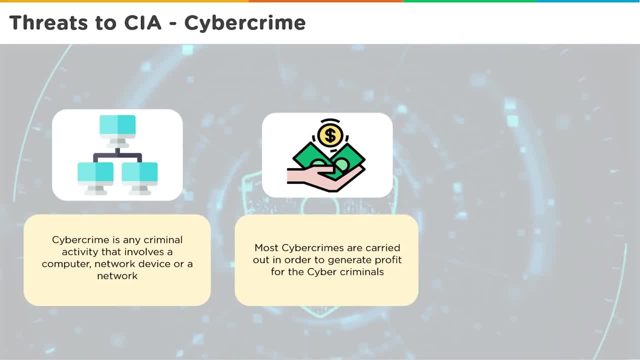 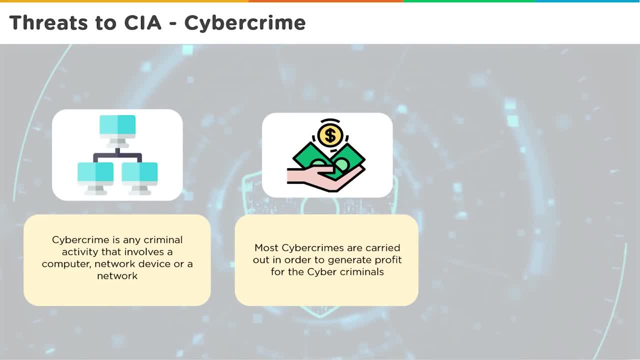 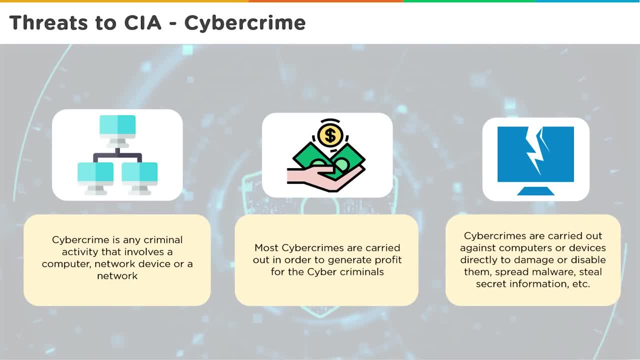 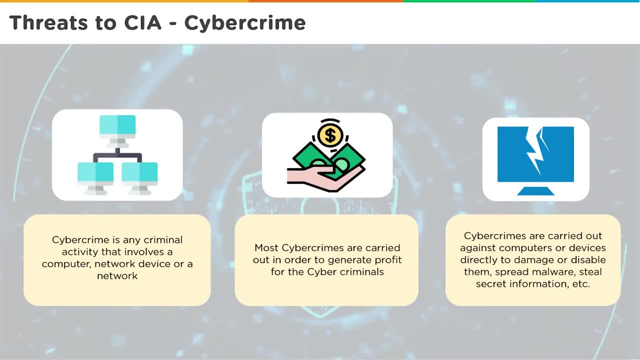 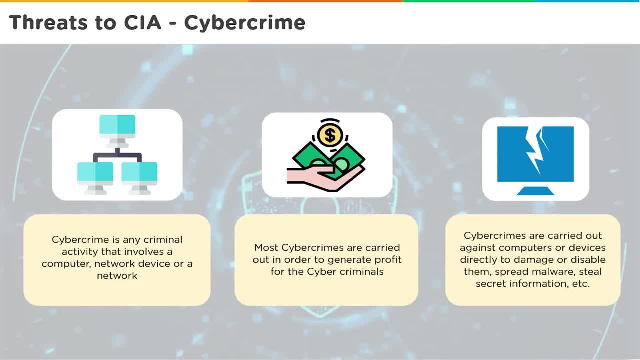 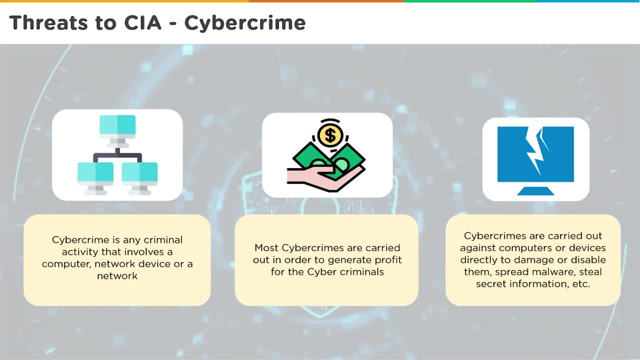 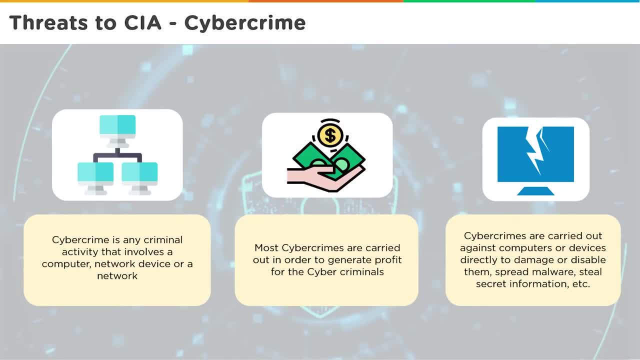 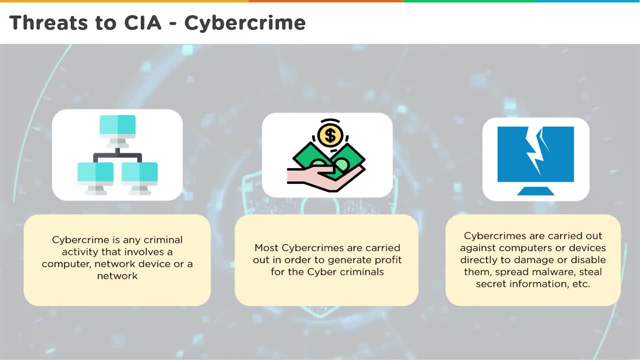 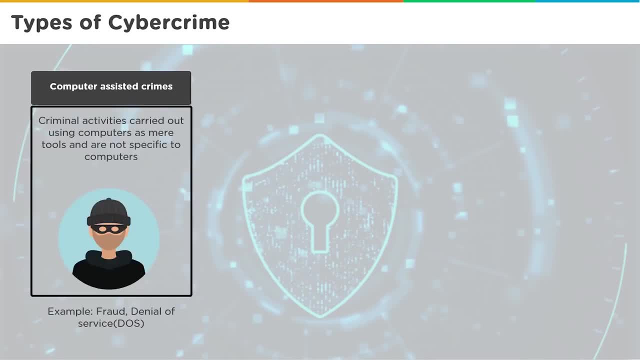 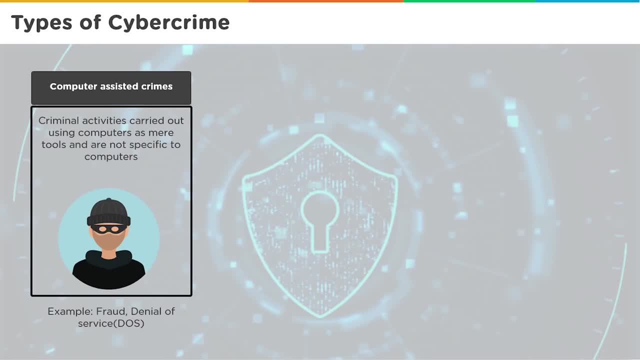 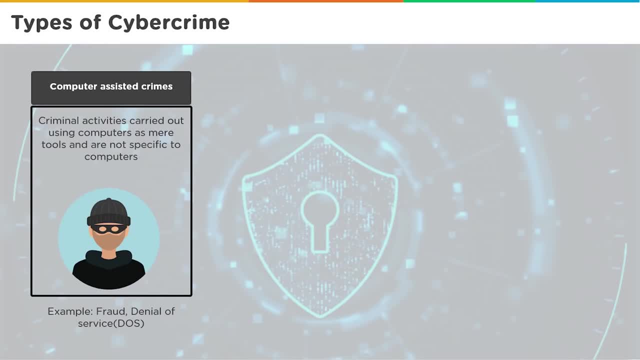 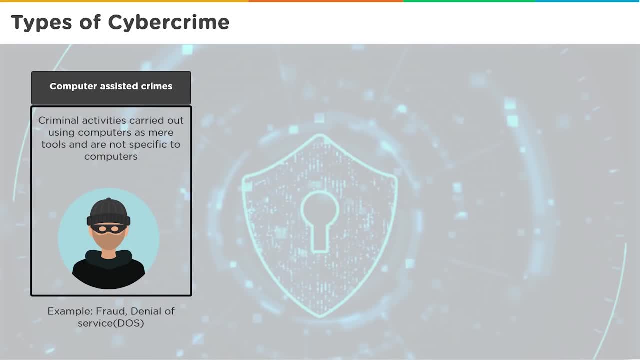 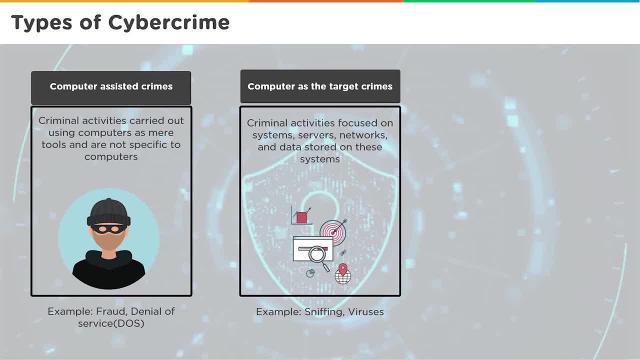 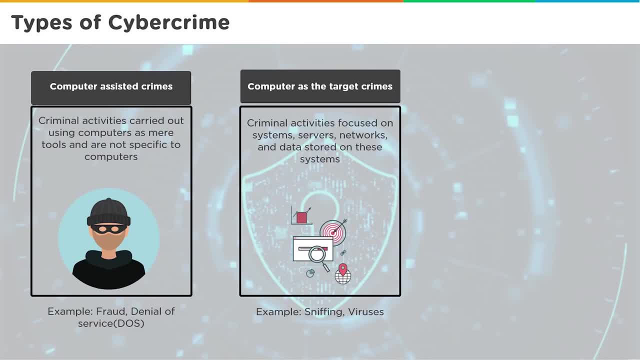 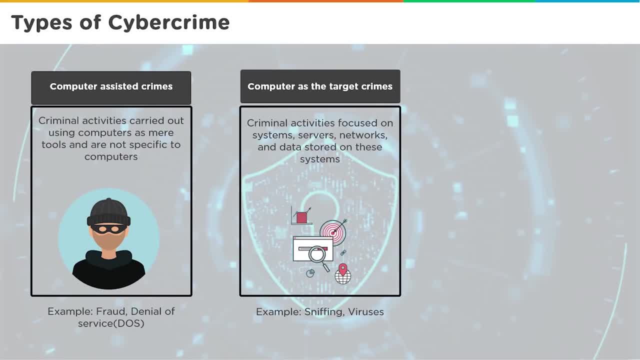 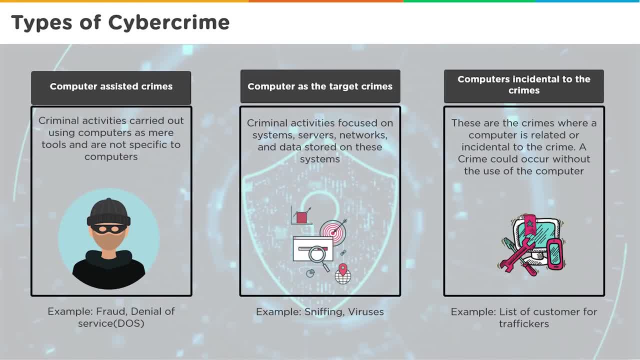 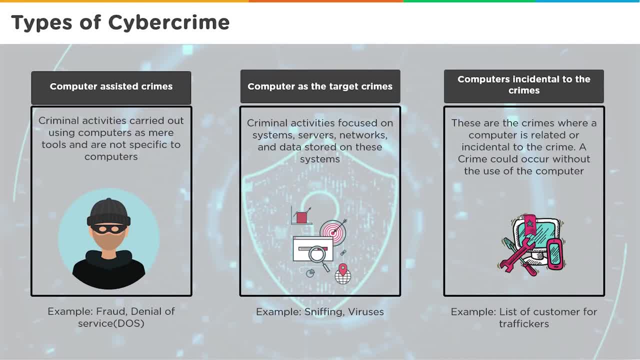 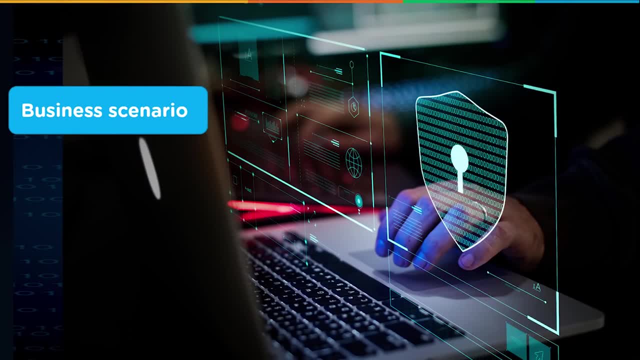 some data, such as child pornography or some other, some other data which made the computer incidental to the crime. all right, let's look at a business scenario for cyber security. there is a quiz at the end, so please listen up and pay attention. there's this company called stark industries. 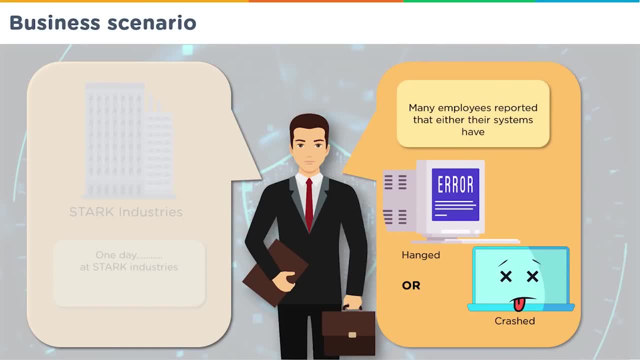 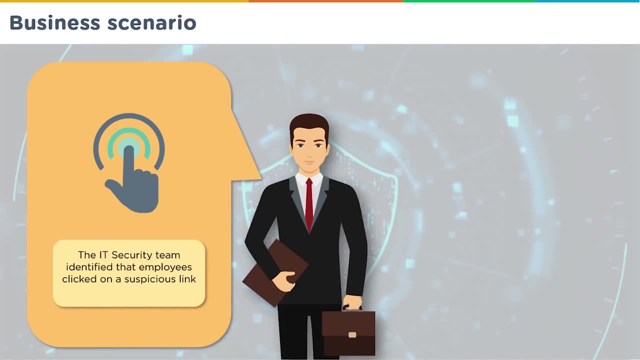 and one day most of the employees have started reporting that their systems have either crashed or have started hanging. so the id security team comes in, does the investigation, tries to find out what. what exactly went wrong, and they have identified that an employee has clicked on a suspicious link. now these links could either be received as an email or via an email through. 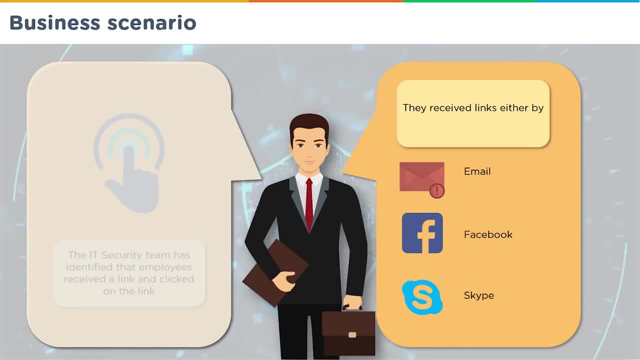 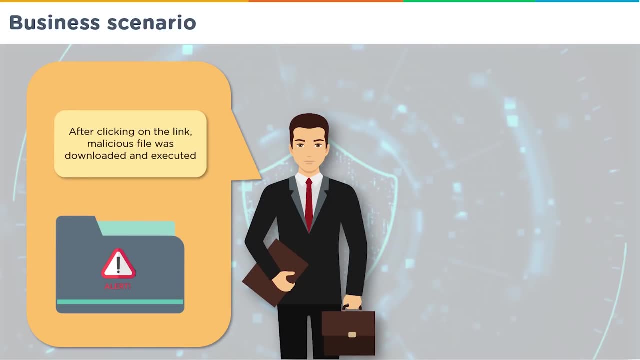 social media like Facebook, or somebody sending out a skype chat and attachments within skype. now, once a user clicks on these links, these links are designed to redirect the connection that the computer is going to make to a malicious server hosted by the hacker and it supposedly downloads a malicious file or some type of application by Apple in the background. then, 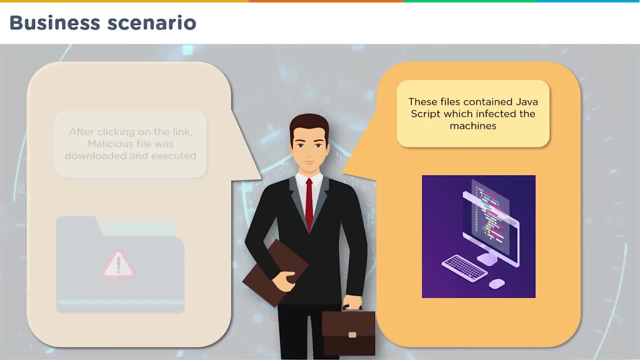 separates the data to any harmful intelligence or services that is available for them. so this scripts and executes them on the victim's machine. Once executed these scripts or the content within these files- maybe the content could be a virus or a trojan- these will start executing themselves and start infecting machines and 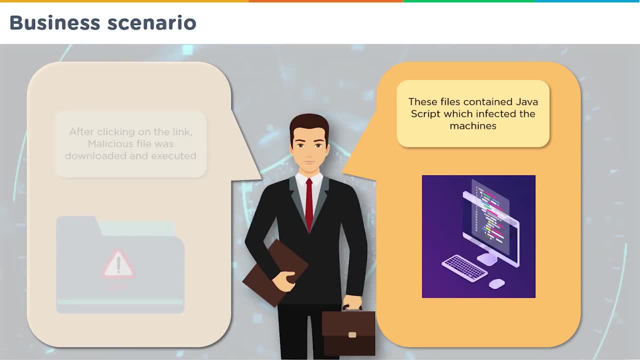 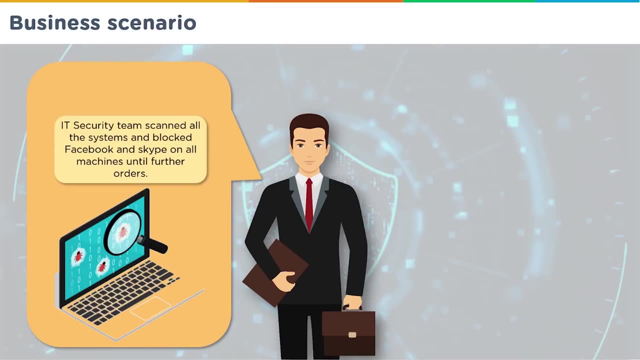 start basically behaving the way they have been programmed to behave In this scenario. a lot of users started reporting that their machines started crashing or their systems hanged. Now the security team scanned all the systems and blocked Facebook and Skype on all machines until further orders. 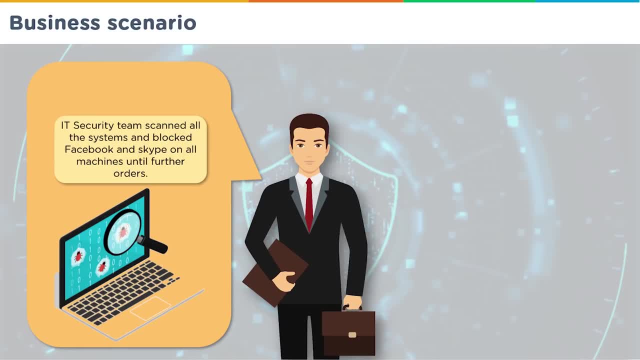 Now this is a preventive mechanism where you're going to prevent possible attacks or future attacks from coming in. So the reaction of the security team here is to block those sites from where the attack may have happened. The question to you at this point in time is: what type of computer crime is being referred? 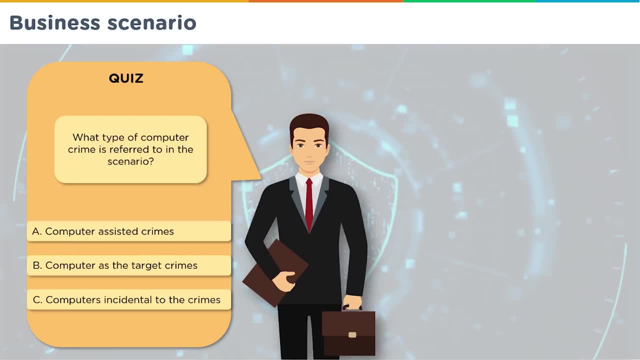 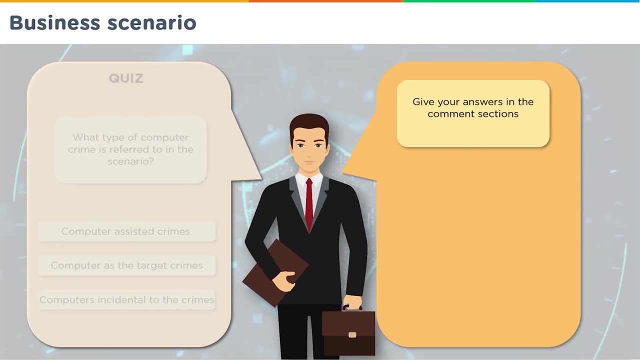 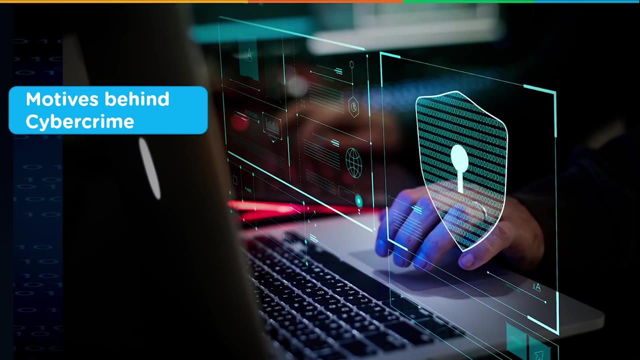 to in this scenario? Is it a computer assisted crime, computer as the target crime or computer incidental to the crimes? So please post your answers in the comment sections below and we'll respond back to you about your answers, Thank you. Now let's go a little bit further and see what would motivate people for committing. 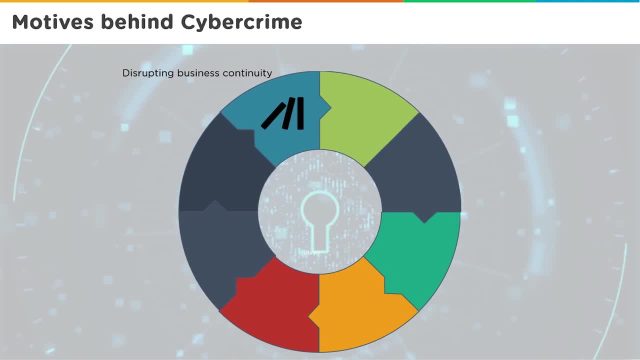 such cyber crimes right. The first and foremost motive is disrupting business continuity. Others would be looking at data theft or information theft and manipulating that data to gain from that data. So if I'm able to access your computer and steal some data that has some value to you, 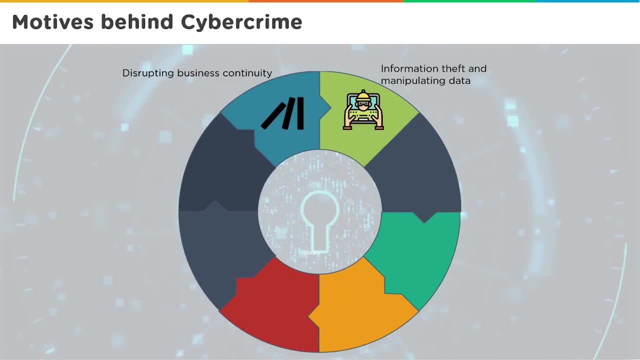 and sell it or make it public. you would be at a financial loss because that data no longer has any value, Creating fear and chaos by disrupting critical infrastructure. For example, a company's infrastructure crashes, the services are no longer being offered by that organization and people start panicking or start fearing an attack by cyber criminals. 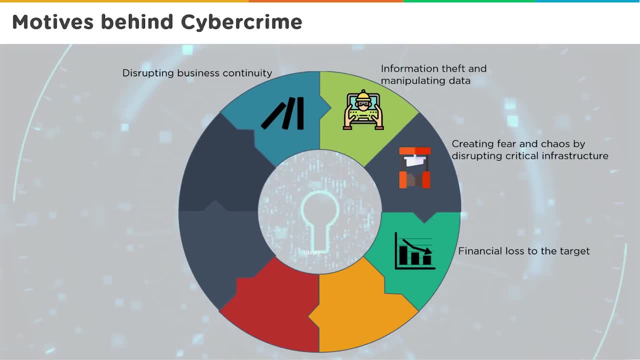 and it leads to chaos, Financial loss to the target, which is very obvious. If I do a denial of service attack, or if I make a service unavailable from an organization, what is going to happen is, since that service is not functioning, the company is not going. 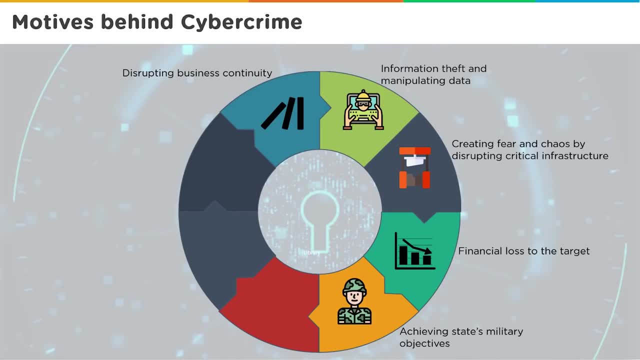 to make any money out of it and thus going to suffer a financial loss. Giving states military objectives, one country spying on another country, trying to gather information about their military intelligence, military activities or any other activities that can harm the original country. Demanding ransom: hackers can encrypt your data and then demand a ransom from you in. 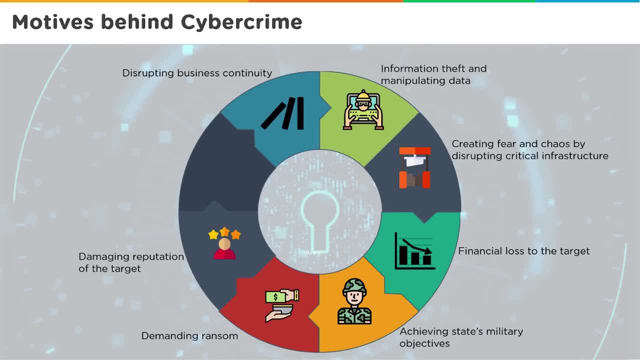 lieu of decrypting the data, again Damaging reputation of a target. impersonating a user on the social media platforms, making false statements, thus damaging the reputation of that person, and propagating religious or political beliefs, Religious fanatics, promoting whatever cultures that they want to promote, trying to gain. 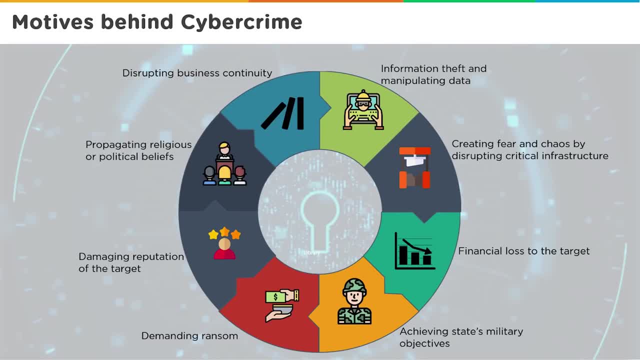 more followers, thus bringing more unrest to the world. Any of these could become motives for cyber crime. In fact, it could be just a script kiddy, where people are trying to learn about hacking and they just start hacking for fun. They might not even have a motive for making a profit out of it. 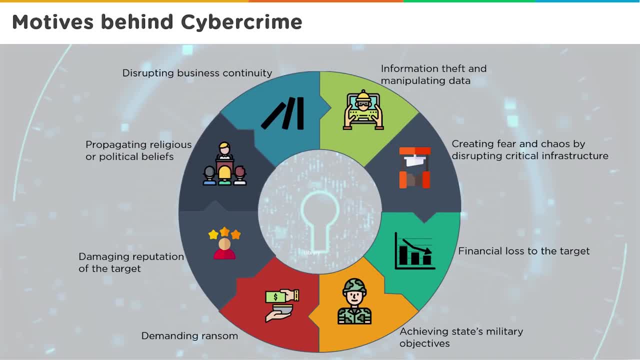 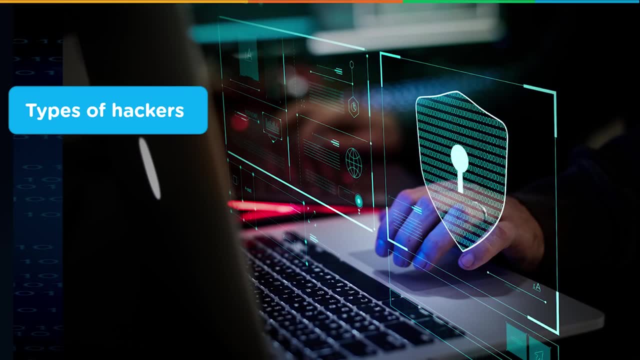 Maybe it just thrills them so that they are able to showcase their skills, and that's why they do a cyber crime, Thank you. So, which brings us to the next topic, where we talk about types of hackers. This will allow us to identify what kind of attacks are also possible on a particular 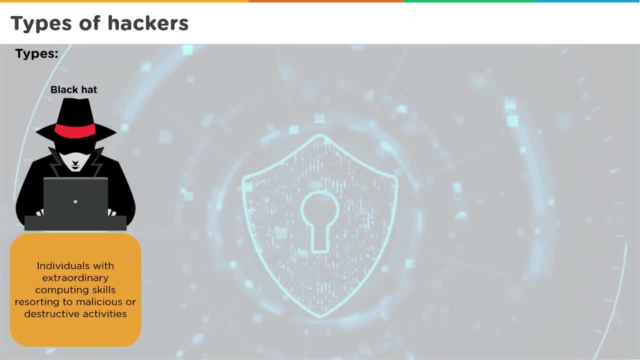 organization as far as motives are concerned. So the basic types. let's start off with the black hat hacker: individuals with extraordinary computing skills resorting to malicious or destructive activities. These are your criminal hackers who try to profit from their crimes, and they will have. 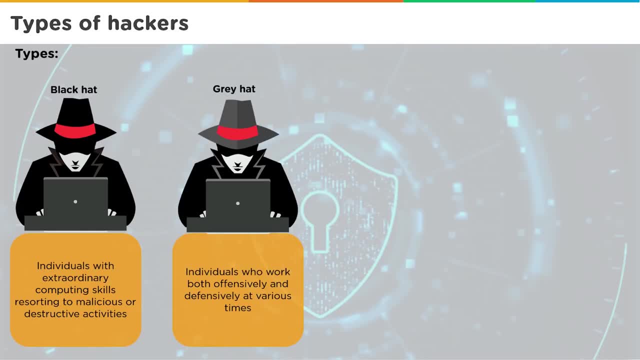 a malicious intent in trying to hack a victim organization. The grey hats: These are individuals who work both offensively and defensively. What does that mean? They could work as black hat hackers with malicious intent and try to harm some organization, while on the other hand, they would also try to work as a security analyst and try 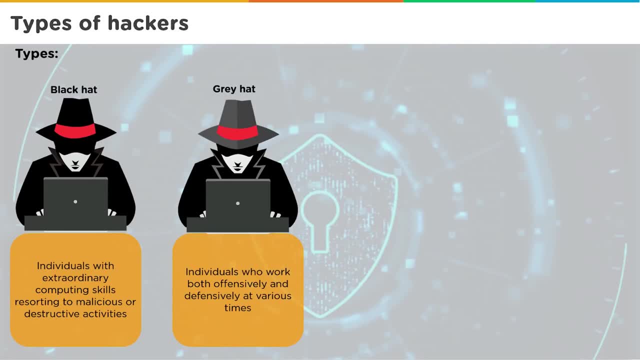 to enhance the security posture of an organization for a remuneration. Third one, which is white hat, which is what we want to be, or what we want to achieve ourselves as An individual who professes the same skills as a black hat hacker probably uses the same. 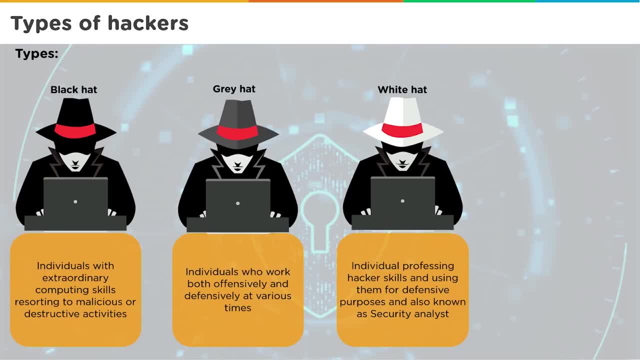 tools has the same kind of knowledge, but the intent is different. They're going to use them for defensive purposes. There's no malicious intent. They act with authorization from the organization and they will try to detect any flaws and try to plug out those flaws so that black hat hackers would not be able to misuse those. 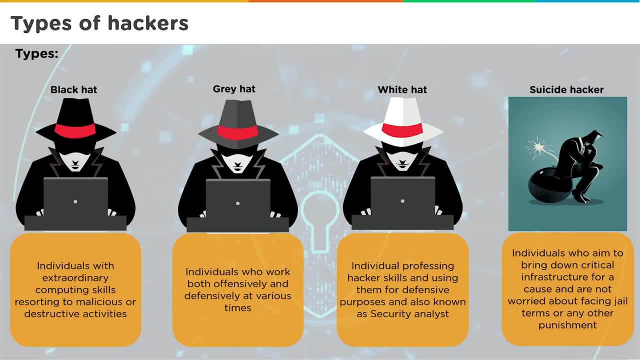 flaws to gain access. Suicide hackers, Now individuals who aim to bring down critical infrastructure for a cause and are not worried about facing jail terms or any other punishment, So any people or any organization or a group of people, for example, anonymous, or these. 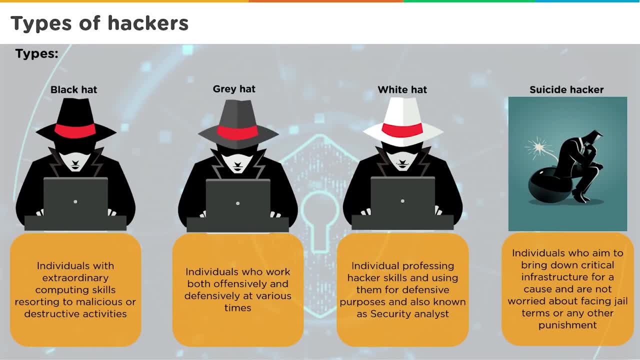 kind of organized hackers. they have a political cause or a social cause that they want to promote, and they do this by hacking critical infrastructure of organizations, bringing it down, defacing their website. Now, why would these not be classified as black hat hackers? 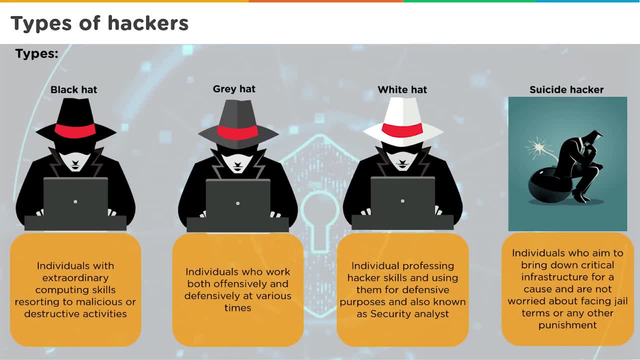 The main difference between black hat hackers and suicide hackers is that black hat hackers will try to hide their identity. They will always have a fake identity that they will utilize And try to hide behind it, whereas suicide hackers will claim responsibility for the attacks that they have done and will boast about it. 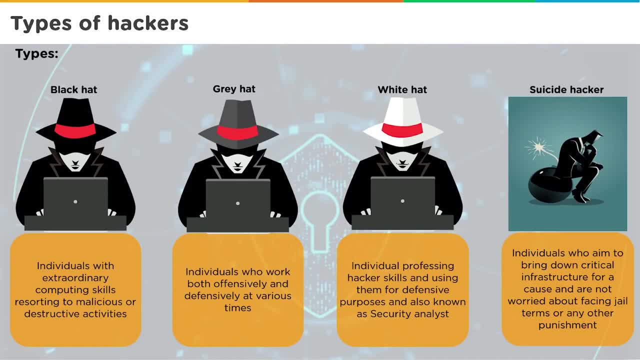 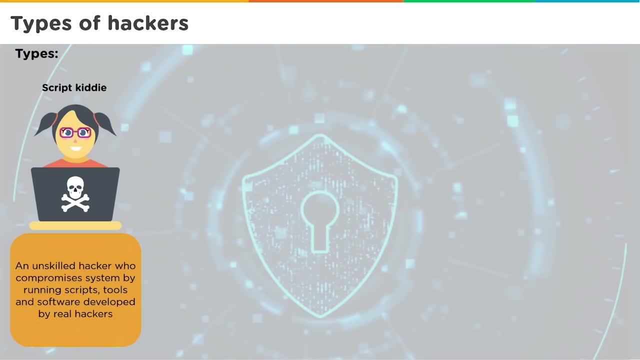 They will not be worried about facing repercussions for the attacks that they have done. The script kiddie- A script kiddie is an unskilled hacker who compromises systems by running scripts, tools and softwares already developed and already made available by real hackers. 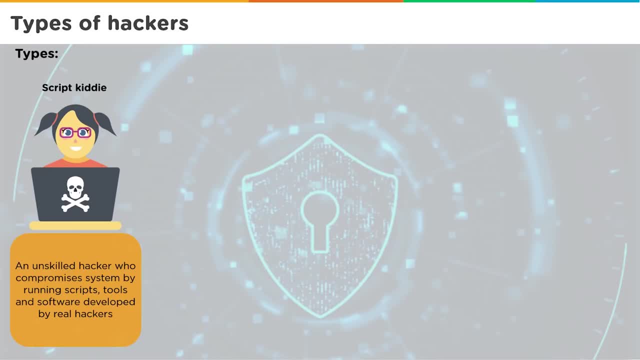 So these guys have very minimal technical knowledge. They have no idea how that attack works. They're just going to use an automated tool, click on a few buttons and hope that the attack succeeds. Individuals with wide range of skills, motivated by religious or political beliefs to create. 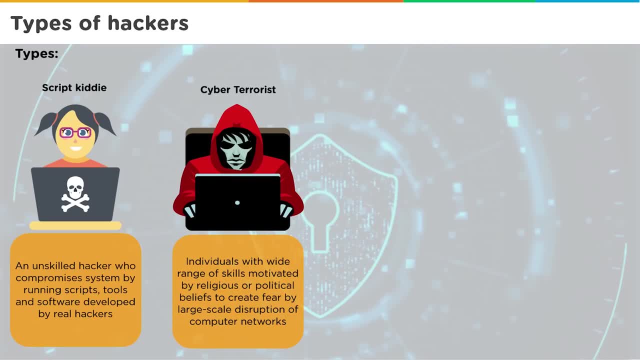 fear by large scale disruption of computer networks. We could talk about organizations like ISIS, who have a lot of digital propaganda that they use and target weak minded people to join their causes, or people who spread ransomware, who terrorize organizations and hold them to ransom and demand money from them by encrypting. 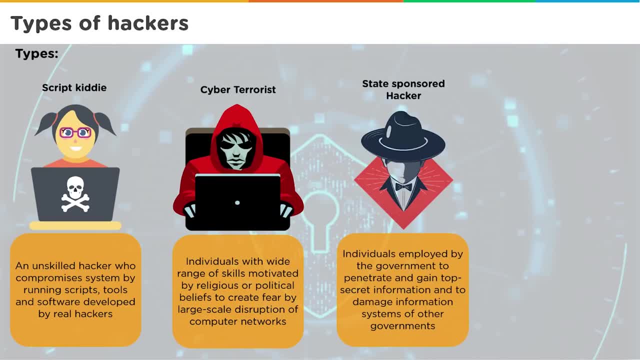 their data. State sponsored hackers, individuals employed by the government to penetrate and gain top secret information And to damage information systems to other governments. The best example would be the cyber wars that are going on these days. Most of the organizations, most of the countries nowadays would have a secret cyber cell consisting 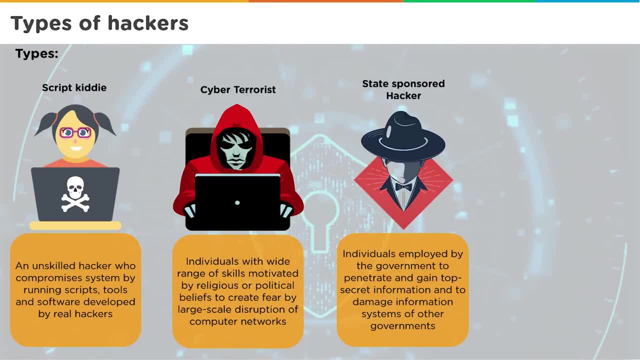 of highly skilled hackers who are interested with the task of spying on the enemies and trying to gather information by hacking into their infrastructure. Now, it is not going to be a legit job. It will always be masked by a legit organization. but this is. this does happen. 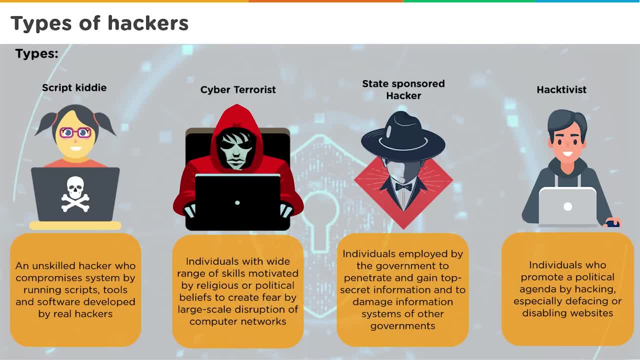 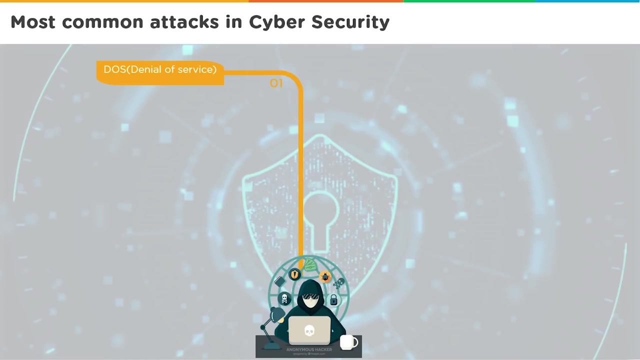 Hacktivism: Individuals who promote a political agenda. They are going to deface websites and they are going to promote their agenda by defacing such websites. All right, So let's talk about some common attacks in cybersecurity. The most common attack ever seen in today's world is a denial of service attack. 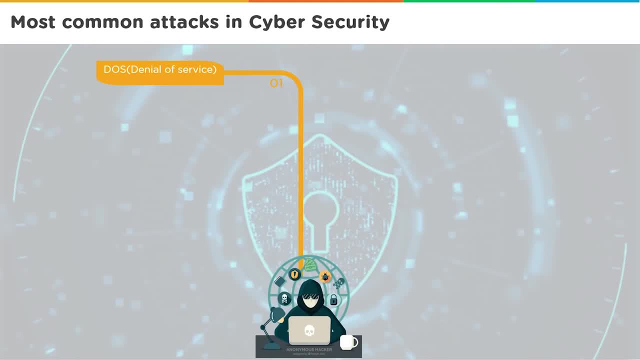 So this is where the hacker tries to consume the resources of the victim server in such a way that There are no resources available for legitimate users to connect to the server and conduct their business. Other attacks that you face would be malware attacks, where there would be a malicious software. 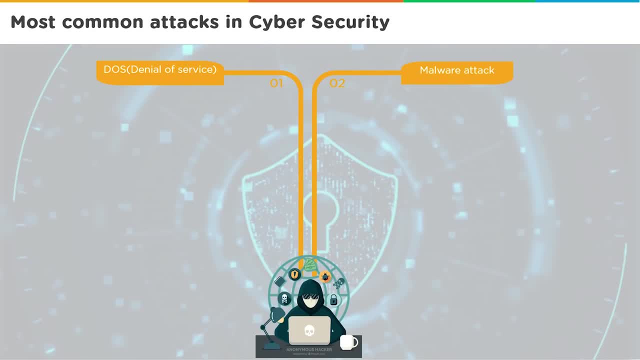 that would deliver a Trojan virus or a worm to the victim Does, infecting the victim's machine and rendering it useless. A man in the middle attack, where the hacker would put himself in between your machine and the router and start sniffing data packets that you're sending. 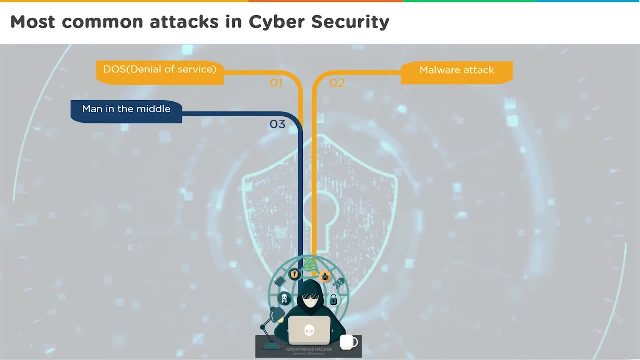 Does Compromise information contained within those packets. So the phishing attack is where a hacker will send a seemingly legitimate looking message to you and email that say asking you to perform certain actions where the hacker would be impersonating another organization, and you fall prey to that and end up giving your confidential 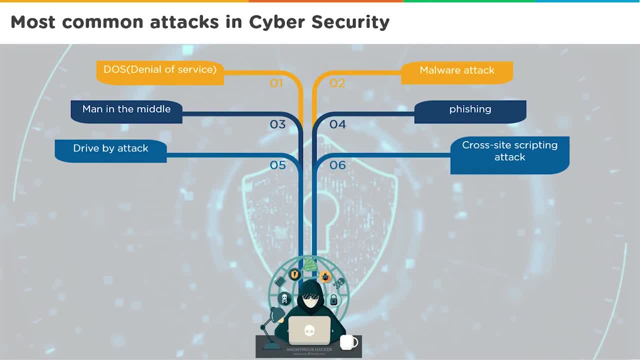 information A drive by attack. cross-site scripting attacks, where web applications get compromised and scripts are embedded within those applications Or Within commands that are sent out by the users. Password attacks, where hackers try to compromise the passwords of users by cracking them, based either on brute force, dictionary based attacks or password guessing. 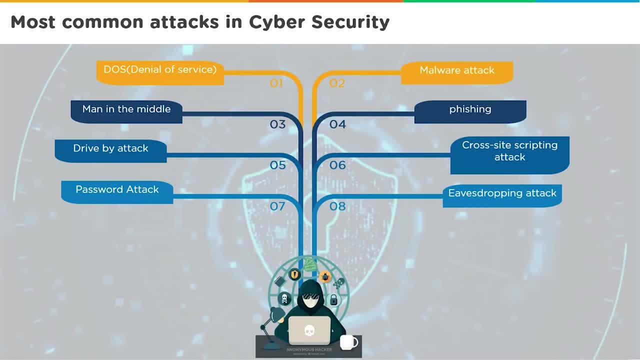 Eavesdropping attacks. This could be physical in nature, where somebody overhears what you're saying or tries to capture data packets that contain your VoIP transmissions. where, let's say, you're assuming you're making a Skype or a link based call. SQL injection attacks, where again, attackers will target your database. try to send in. 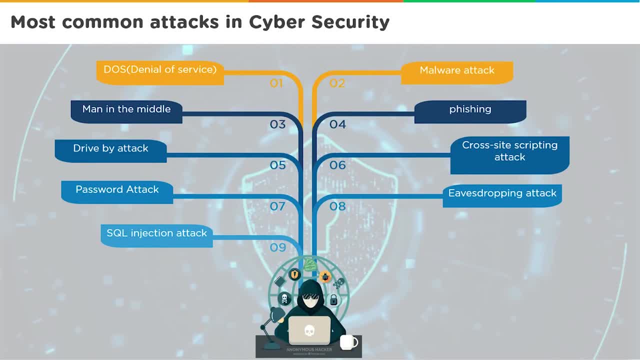 malicious queries which will compromise your database and the data within, But the attacks. it is based on cryptography, where you're looking at permutations and combinations of how algorithm functions and then you're looking at the permutations on how many times the processing needs to be done for the algorithm to be reversed. 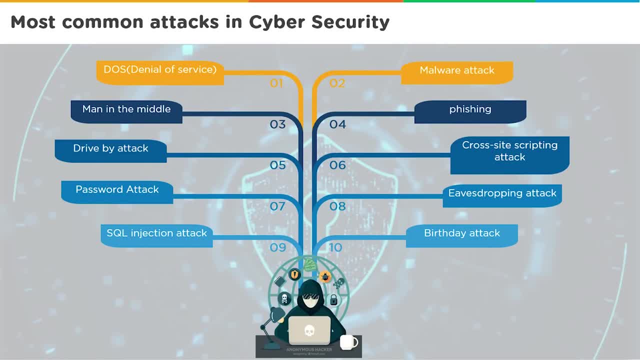 So these are some of the most common attacks in cybersecurity. Now, These, more than attacks, would be threats that you're going to face. there would be various different methods that these attacks can be launched, and that's where the cyber security expert comes in with their knowledge of identifying what exactly is a threat to the organization. 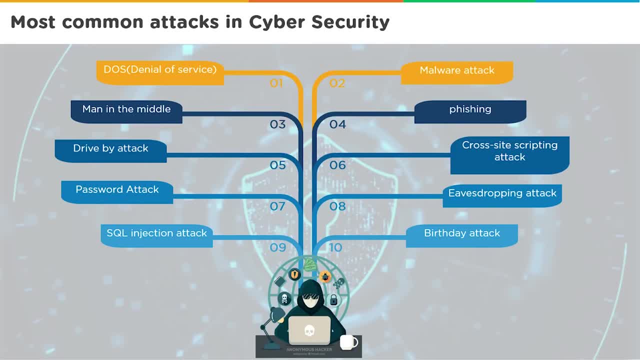 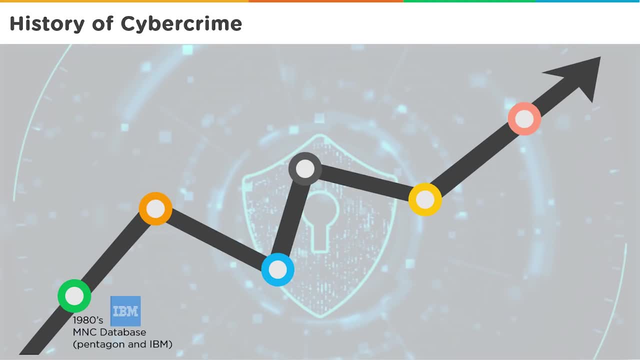 and how they are going to prevent that from happening. But more on that a little bit later. Let's look at the history of cybercrime. So, as you can see, this graph shows us how cybercrime has progressed over the years. in 1990s, 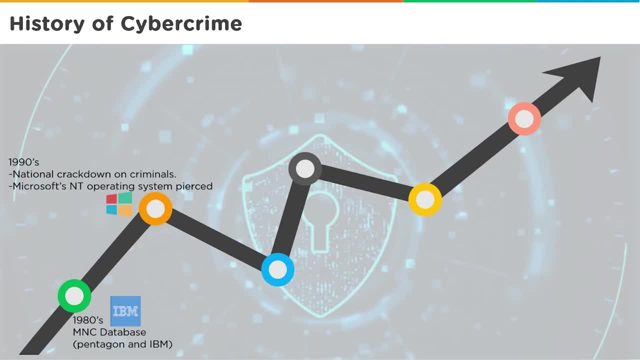 MNC database, Pentagon and IBM. In my, again in 1990s, National Crackdown on Criminals, Microsoft NT operating system pierced. So this is where hacking started becoming more mainstream. right before this, hacking was very much limited to organizations who use computers. But in the late 80s, internet happened and then we had e-commerce coming in, which basically 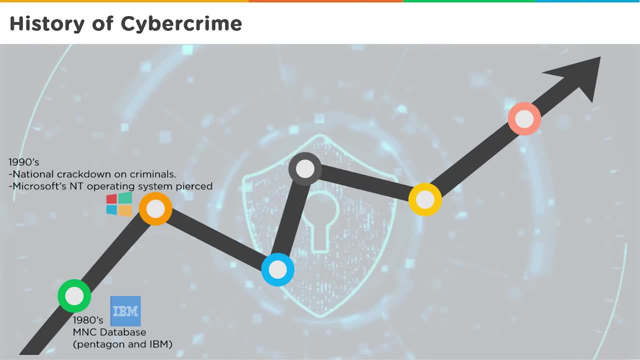 led to our online retail stores, online banking and online data stores as well, which then led to criminals hijacking this data, or hijacking your money, and trying to steal it on the internet itself. In 2001, cybercriminals launched attacks against eBay, Yahoo, CNN, Amazon and other organizations. 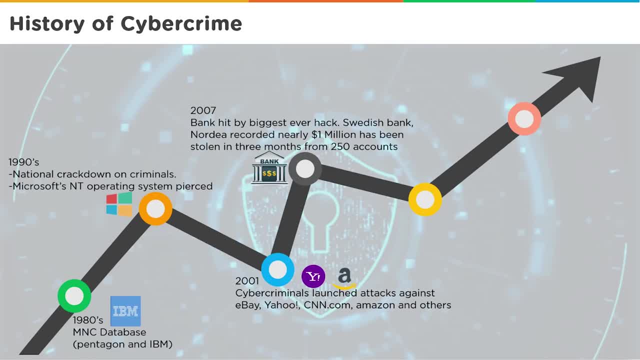 2007.. This was where one of the biggest bank hacks had happened: Swedish bank, Nordea. They recorded at least a million dollars being stolen in three months from 250 accounts. 2013, Adobe had 2.9 million accounts, Compromising. 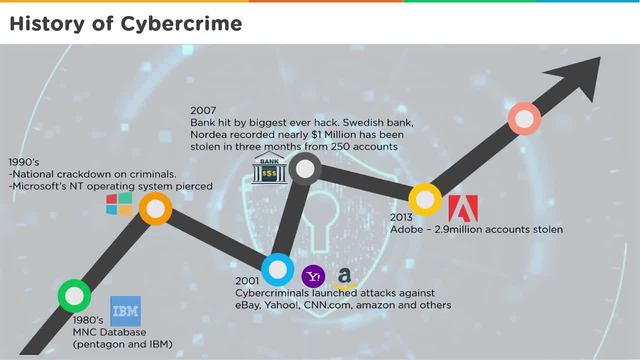 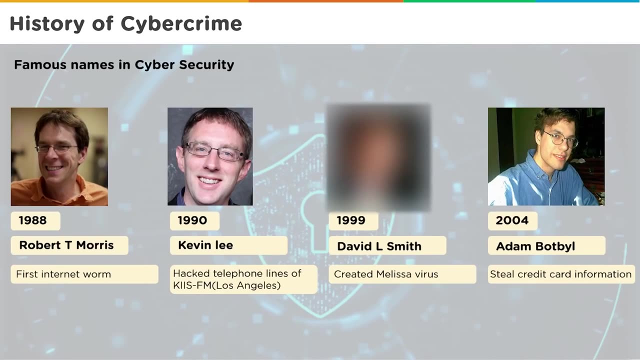 And then usernames and passwords released on the open internet. in 2016, Kaspersky, one of the leading antivirus providers to the world, reported around 758 million malicious attacks that occurred, which they identified themselves. These are some of the most famous faces in cyber security or earlier cybercrime in 1988. 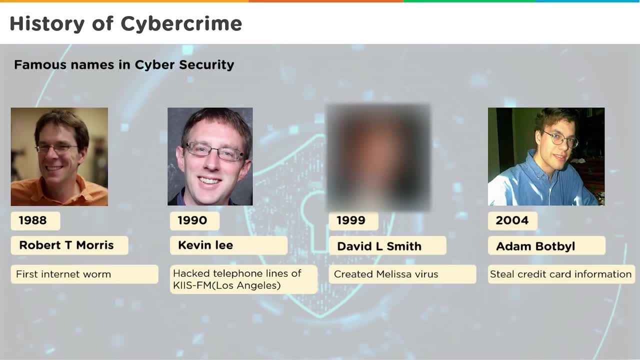 Robert Morris. He's an American computer scientist and entrepreneur. He's best known For creating what is called the Morris worm, and this was way back in 1988, and this is one of the first computer worm that has been identified on the internet. Kevin Lee or Kevin. 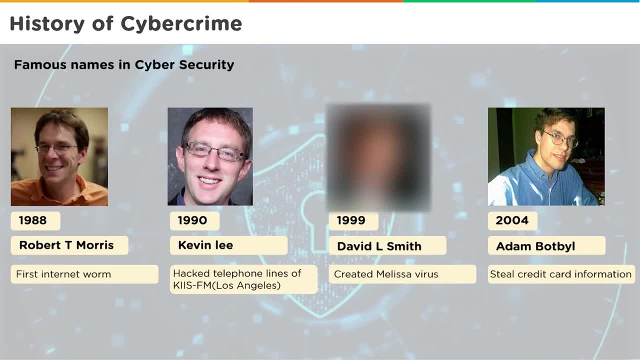 Lee Paulson. in 1990 he was accused of hacking into Los Angeles radio station called KIS hyphen FM, where there was a contest going on and if you're a particular number of caller and give a correct answer, You're supposed to be. 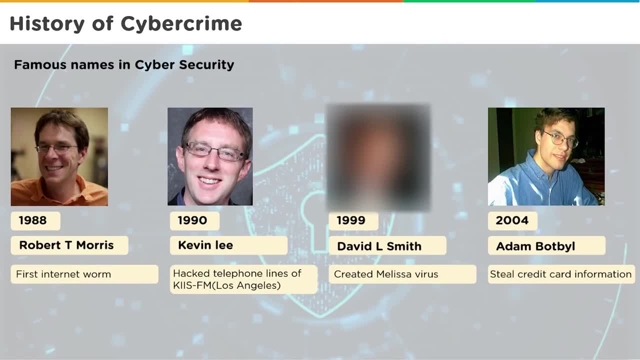 To win a Porsche 9, 4, 4, and he hacked the those telephone lines, ensuring that he became that particular person and answered the question correctly. It was later on revealed that this actually happened. He was jailed for it. Then comes David Smith. David Smith. 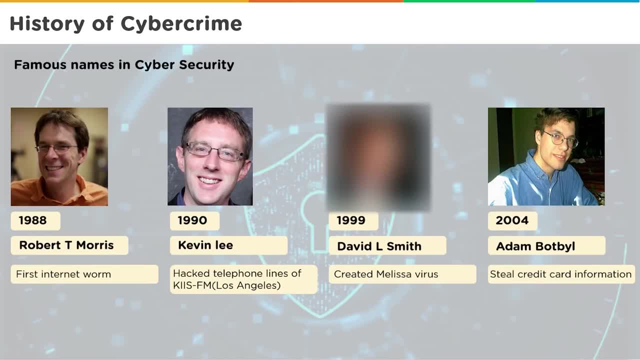 He created the Melissa virus, Now Melissa virus, one of the most dynamic viruses known, around March 1999.. That's when this happened. This virus was released. This was a macro based wireless which affected Microsoft Word and Outlook based files. Adam bought bill in 2004.. 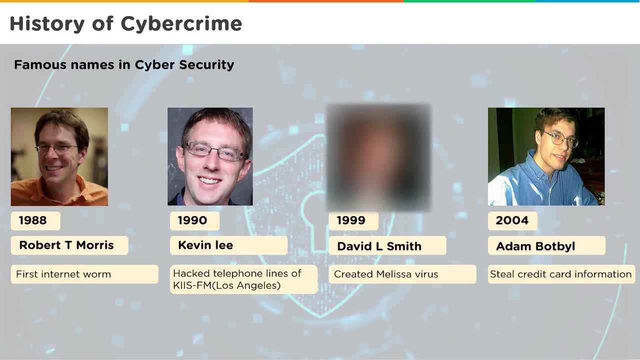 He's also an American computer hacker from Michigan. He gained unauthorized access to loves computer corporate computer network via an open, unsecured wireless access points. Now, these access points back then, when not that much secured the, these people were able to identify it. what they tried to attempt by doing that was gain access to the company's. 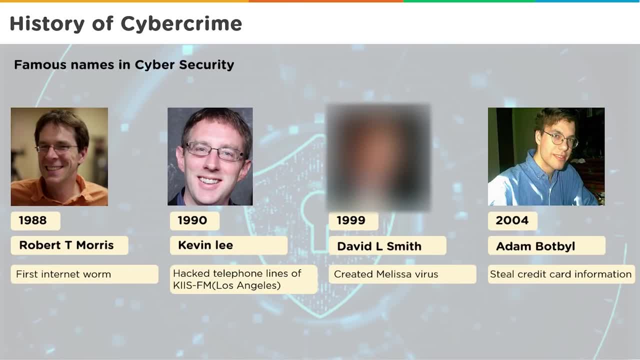 network and install the software which would then help them capture credit card information of their organization. right, and this was later on identified as well, and he was prosecuted for that crime. and what jail, just a matter of trivia, Kevin Lee Poulsen. He was one of the first people found guilty and was banned from using computers and the 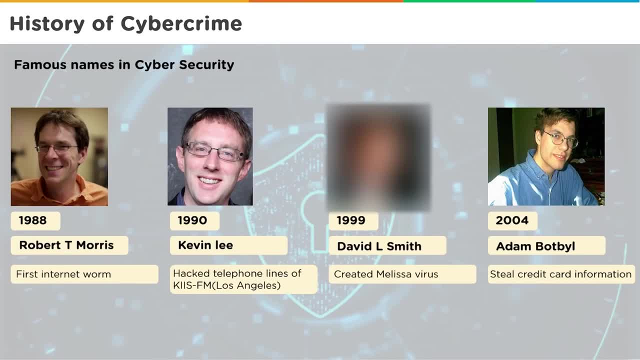 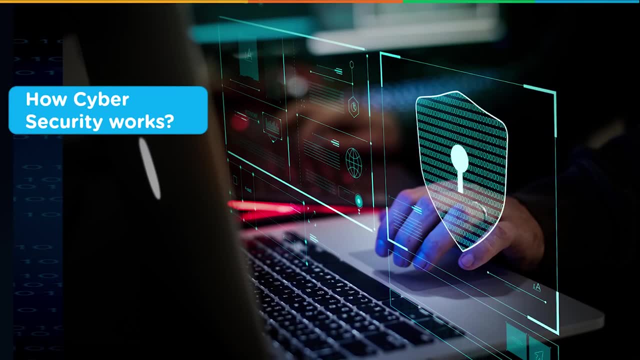 internet for three years after his release. in today's world, We cannot even imagine living without the internet. This guy lived for three years without it. Now let's see how cyber security works. It's all about securing a computer and there are various methodologies. there are various. 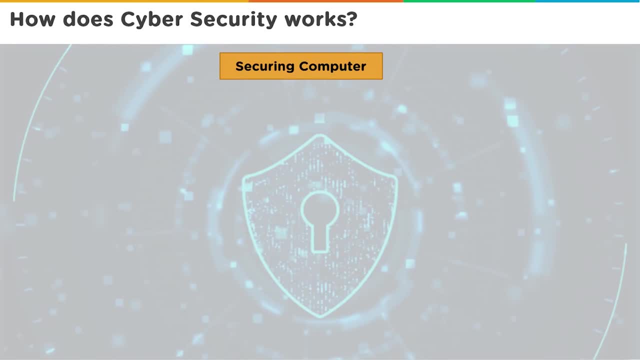 factors that come in on how you're going to secure of various aspects of the same computer. We start off by authentication mechanisms. What is authentication? authentication is the part where you're going to identify a person, authorize that person for some access controls and authenticate that person to ensure. 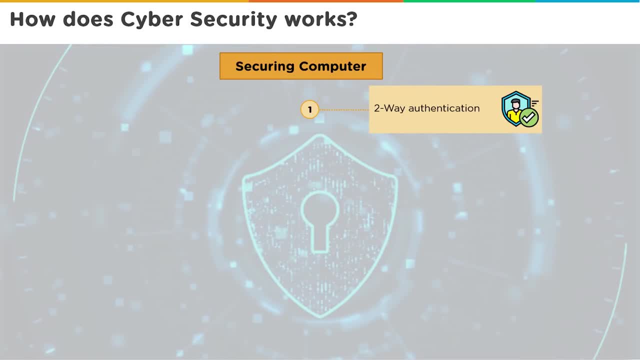 that the person is the same person who they claim to be. So You start off with a username and you associate a password with it. The username is used to identify the account that the person wishes to access. The password is the authentication mechanism to prove that the person is who they are. 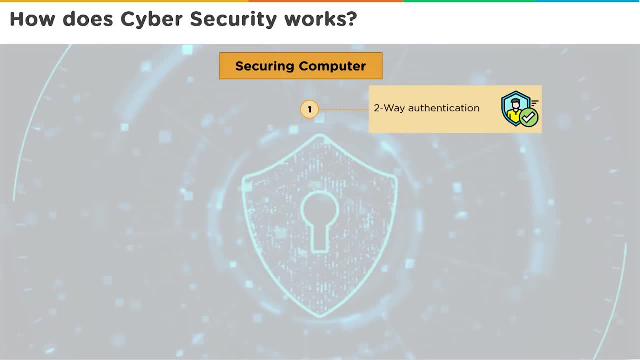 Now here. you may want to enhance the authentication mechanism by using a two way authentication mechanism. for example, with banks, when you type in the username and password, they send an OTP or a one time password, which is auto generated by a server and sent to a registered device that the person owns. 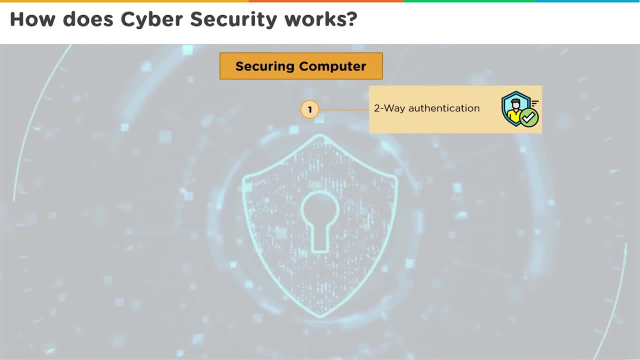 For example, a cell phone. So that's one added layer of security where you're not only relying on the password, which can be cracked, but you're relying on a third party device as well, which the person needs to have physical access to, where they're going to receive the OTP and then they're going. 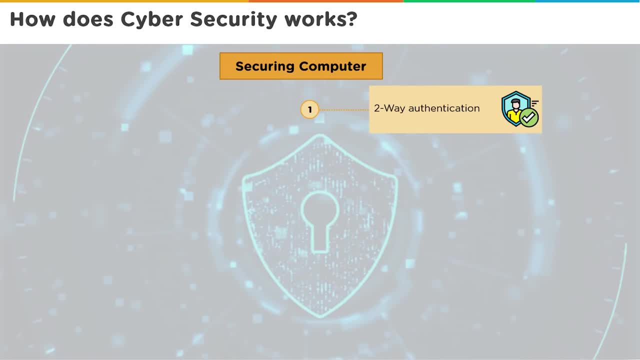 to input it. every time they try to log in, a new OTP will be generated. Securing your passwords. just having a password may not be sufficient. You have to ensure that the password meets some complexity standards to ensure that the security of those passwords or the complexity of the passwords is high enough where cracking. 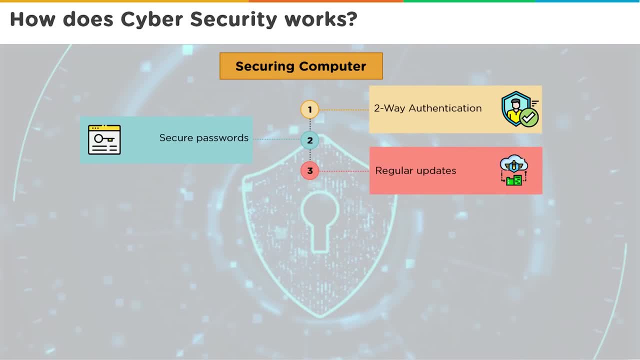 programs will not be able to easily crack the password. Regular updates on the operating systems or the applications that you use will be receiving. regular updates could be for functionality but more for security, So as new vulnerabilities in applications or operating systems are found out, the software 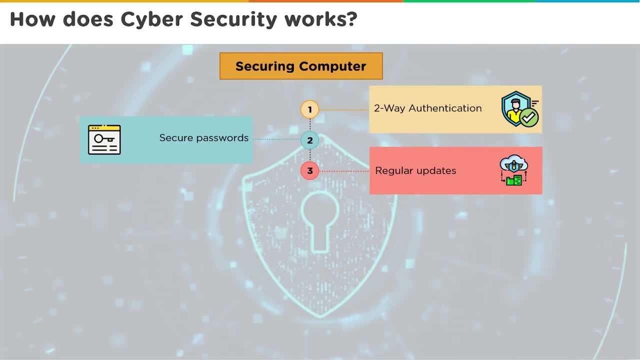 vendors or the developers of those softwares over a period of time, start sending out these updates, also called patches, to the end users. Okay, It is very important for the end users to identify these security patches and install them on their devices as soon as possible, else they remain open for those vulnerabilities. 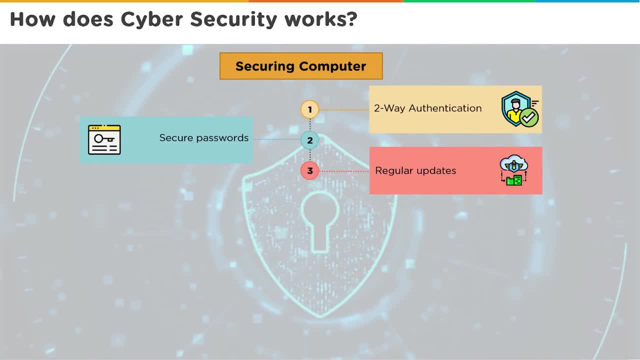 and unpatched systems thus can easily be hacked. Usage of an antivirus To protect yourself from viruses, worms, Trojans- essentially malwares. there needs to be a software that's installed on your computer that is going to watch out for them. 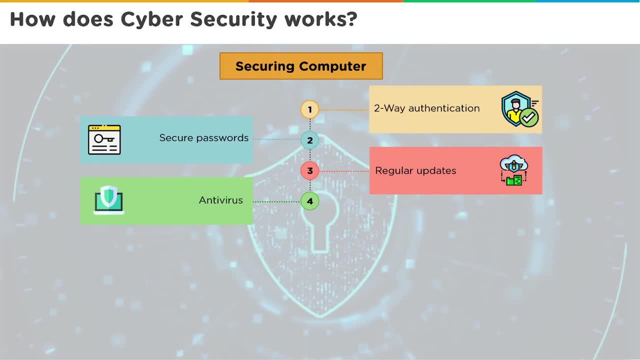 You cannot rely on the operating system itself to protect you, so there has to be an antivirus which will be scanning the connections that you are making, the websites that you will be visiting, the files that are getting executed in the background and ensure that everything that is happening is legit. 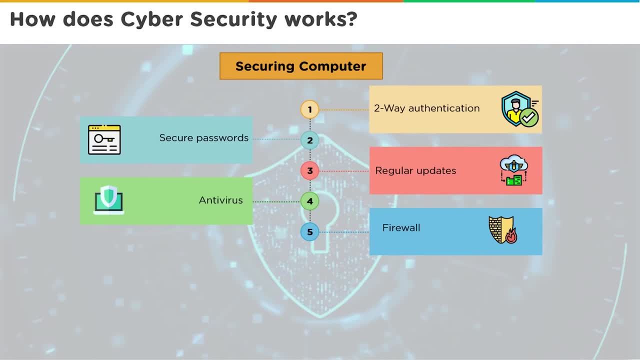 Installing a firewall on a system or a server. A firewall, essentially, is a software or a hardware that allows or disallows some functionality, for example a port to be opened or closed, or a service to function on a computer or not function on a computer. Thus what you are trying to do here by disabling unwanted services. 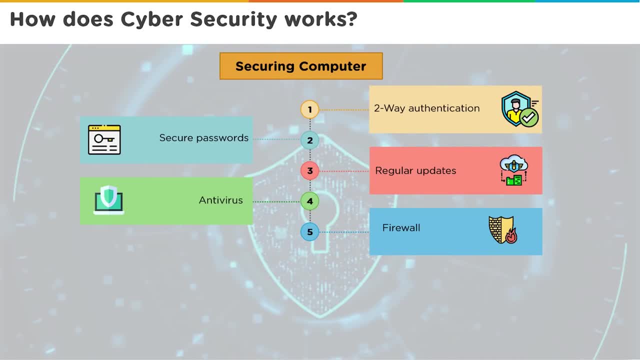 Is you are limiting the threat landscape that you are creating for your computer. If a service doesn't exist on your computer, it cannot be hacked. So the essence here is first identify which ports you will be using, which services you will be using, and then create a policy on the firewall to ensure that only required 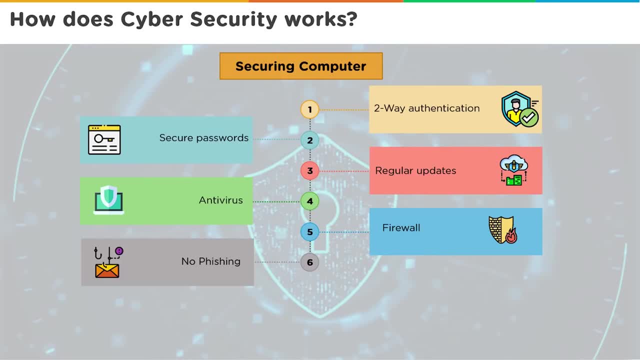 ports and services are running No phishing. So phishing, as we said, could be a malicious website that is being hosted by a hacker, The hacker sending you a fake mail looking like a genuine email, Asking you to connect to that particular server and fooling you into you giving that. 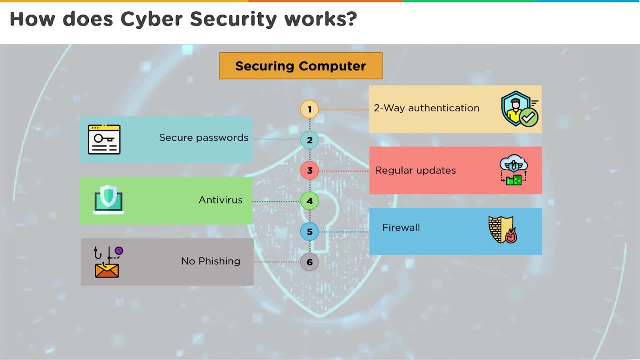 confidential information to the hacker. So you should either the antivirus or, in addition to that, would have an anti phishing toolbar which would identify the websites that you are visiting and give you the risk rating of that website, Giving you an idea whether this website was ever reported as a phishing website or not. 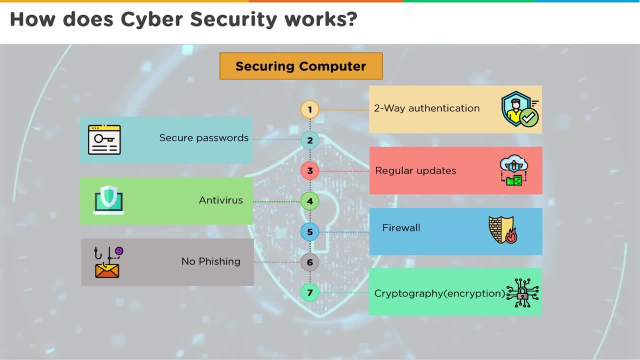 Cryptography encryption. The best way to keep everything secure is to encrypt it. However, How the encryptions are required, What should be encrypted, What should not be encrypted, How that encryption should function and how this encryption enhances the business value is what we need to ascertain. 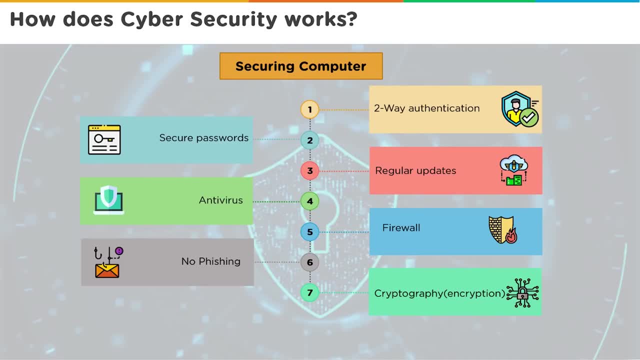 So the knowledge here that will be required is what protocols you want to encrypt. For that you first need to identify which protocols you are going to consume, What data is going to be transmitted over that protocol, How valuable that data is to your organization, and then you're going to add encryption or 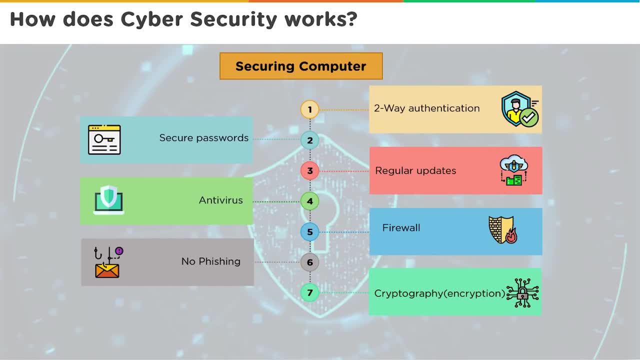 cryptography on top of it to prevent any attacks from hackers and then securing DNS servers. DNS is a domain name server, which is basically an index that maps your domain names to your IP addresses. So the domain name system is an index that maps your domain names to your IP addresses. 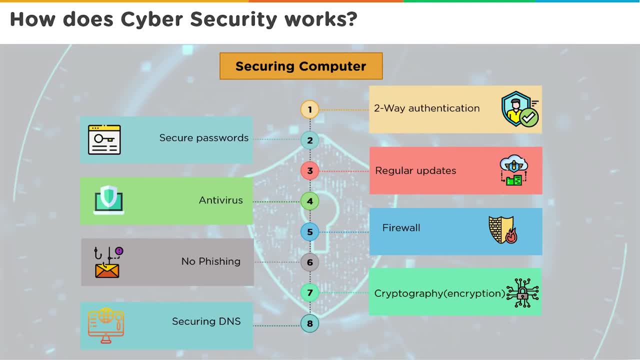 Now on the Internet. computers do not know domain names. They only they can only identify IP addresses and MAC addresses. So when we type in, let's say, Googlecom on our browser, The computer doesn't know what Googlecom is. What it does is it sends the packet to the DNS server and in the DNS server it queries: 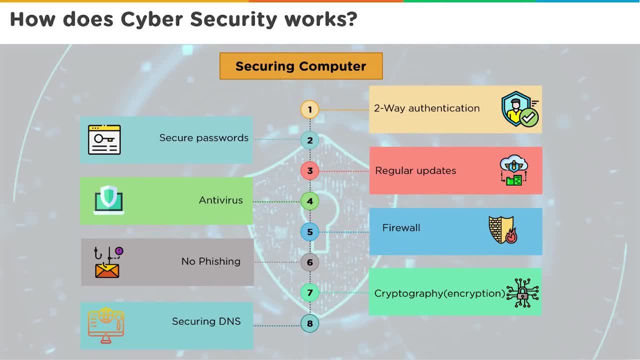 where Googlecom is located, It is given the corresponding IP address, because of which the packet then goes to the relevant server. There are attacks where a DNS can be compromised and the pointer pointing to your particular website can be changed to point to a malicious server that a hacker is hosting. 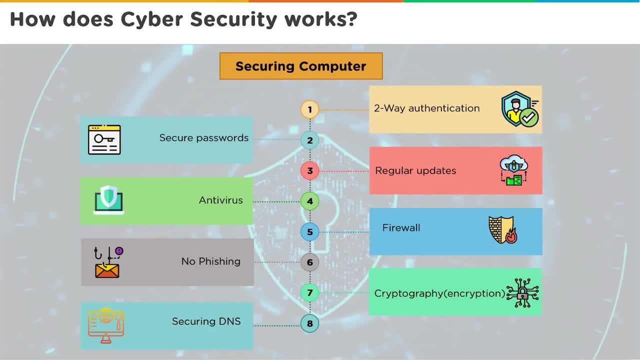 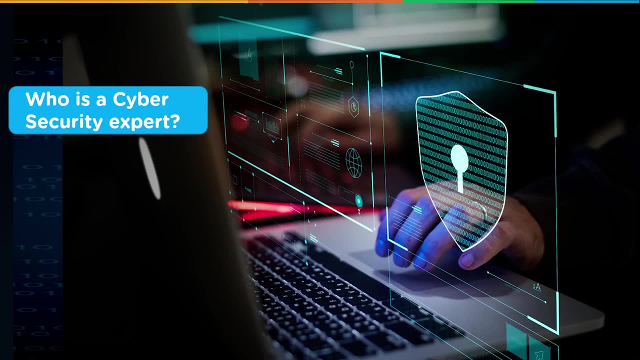 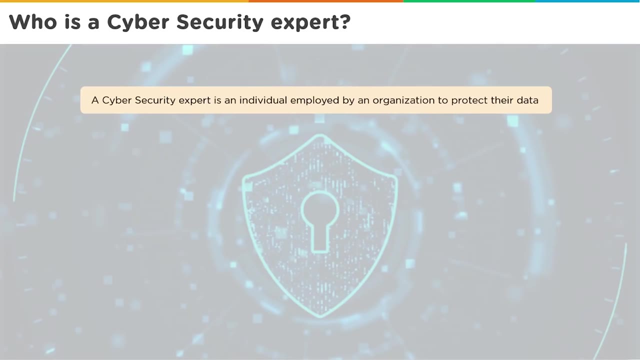 So to prevent that from happening, you need to secure your DNS servers. So, with these kind of attacks and the kind of defense mechanisms we have seen, let's see how do we become a cyber security expert. So, essentially, who is a cyber security expert? A cyber security expert is an individual employed by an organization to protect their infrastructure. 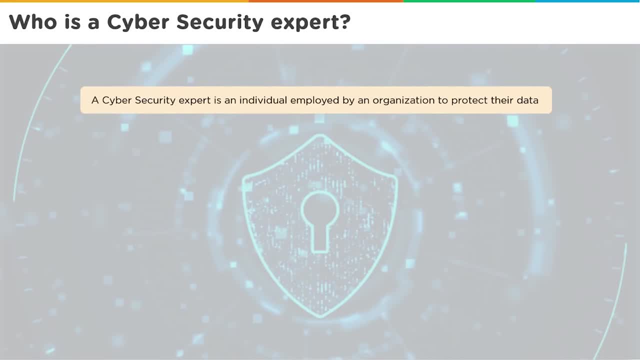 So this person is responsible to identify potential flaws, identify what threats the organization faces and then streamline Or create or design or architect methodology which is going to protect all the assets that the organization has. So this is going to happen through a variety of techniques, such as finding weaknesses. 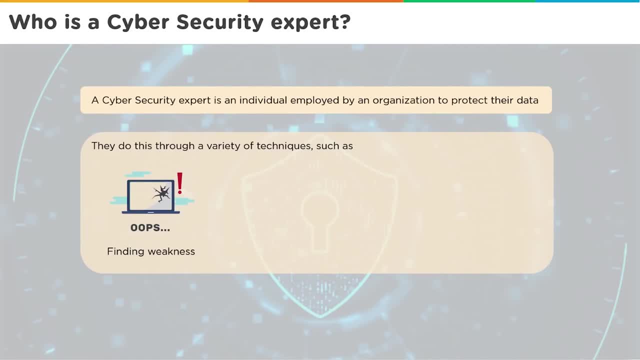 So vulnerability management, where you run vulnerability scanners, identify potential flaws in the organization's infrastructure- Could be applications, could be servers, could be desktops, could be operating systems, could be anything. could be network based flaws as well- And then you're going to monitor these systems. 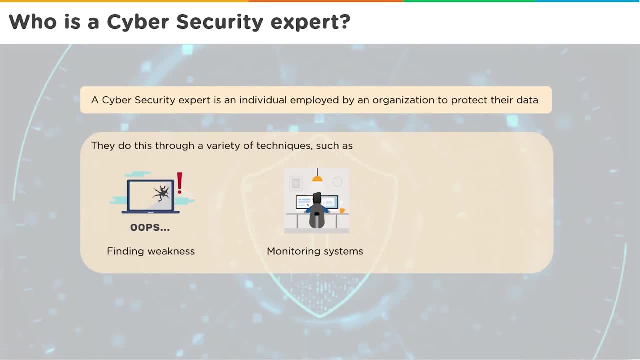 You're going to, You're going to look at the data flow that is going to the internet, through the network, to the intranet rather, And then you're going to check if there is anything malicious going on in that network. So, over these techniques, you basically going to monitor it on a day to day basis, on a regular. 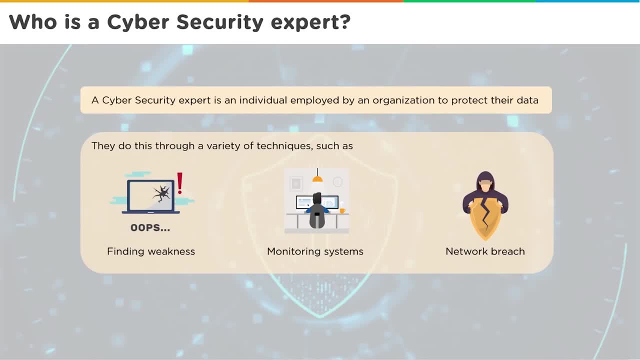 basis and you're going to try to identify if anything out of the ordinary is happening. right After you find the weakness, you're going to test those weaknesses to identify the complexity of those weakness, to validate those weakness actually exist, And then you're going to 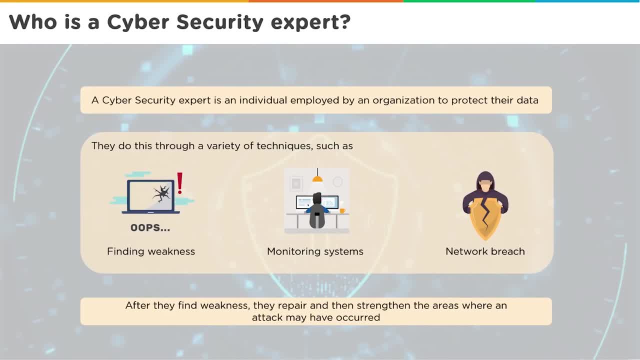 You're going to patch them, You're going to install updates or you're going to prevent. You're going to install mechanisms like firewalls or antiviruses to mitigate those weaknesses and even does, resulting in strengthening the areas where an attack may have occurred. 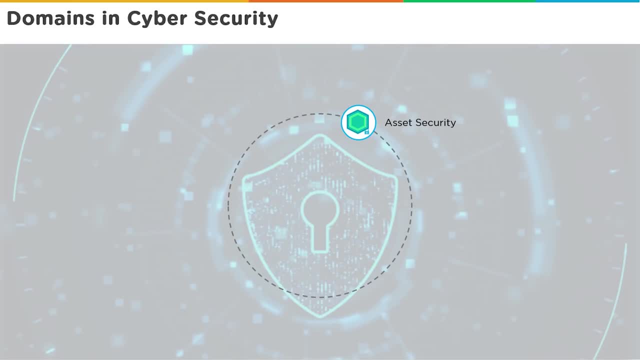 Let's see the domains in cybersecurity. Now, when you say domains in cybersecurity, in the previous slide we were discussing where these attacks may happen, like applications, infrastructure, network. So let's see these domains in detail. Assets security: now when we say assets, assets could be applications, could be networking. 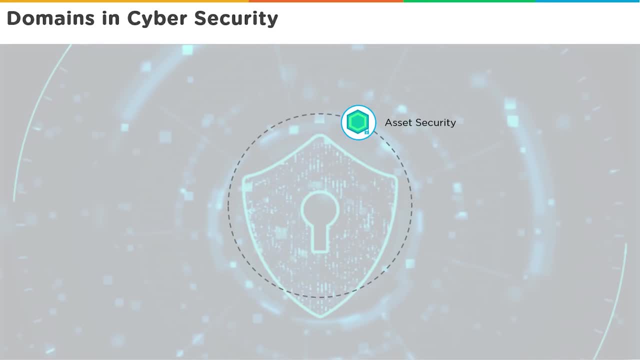 devices could be computers, could be routers, could be wireless access points, and these, all these devices have their own operating systems, they have their own functionality and it is important that we look at the security of each and every asset that the organization owns: Security, architecture and engineering. 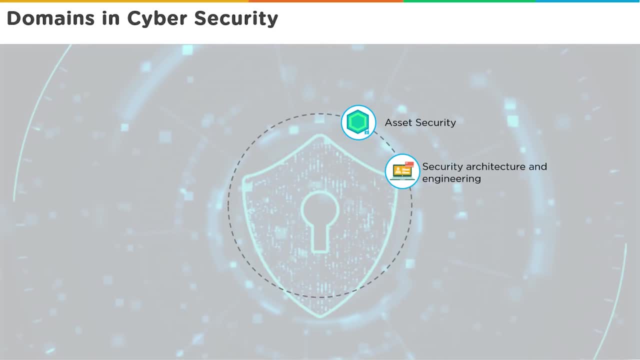 Now, not everyone can just walk in an organization and then say let's start implementing. is in Implementing security in a particular manner, We have to standardize the security in such a way where the security is constant for a long period of time and is consistent right. 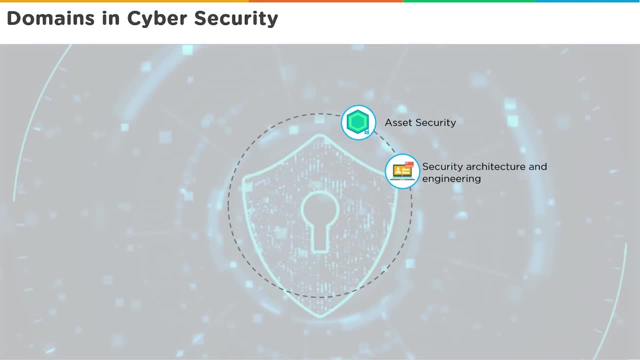 So for that to happen, there is an architecture, an engineering phase where we are going to create a plan of how the security needs to be implemented. For example, if I determine to install a particular antivirus, I have to ensure that the same antivirus is installed on all the systems in the organization. 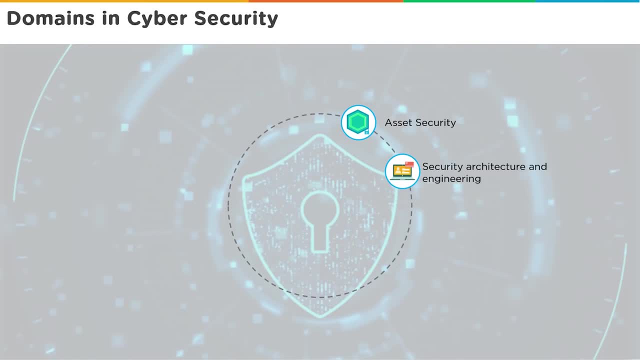 I cannot have different kind of antivirus is installed that do not talk to each other or do not report properly to the proper owner. So we have to create policies, procedures and we have to implement them in a standardized manner for our security to work properly. Communication and network security. 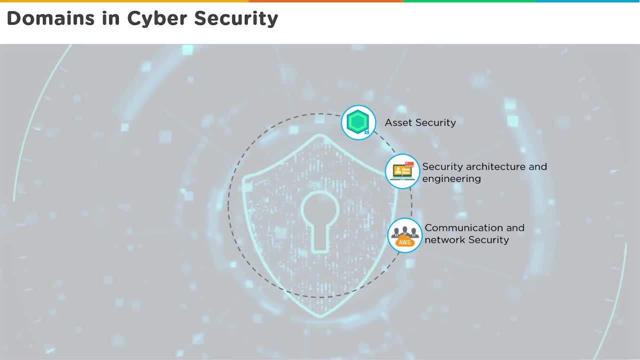 Now, with cloud computing coming in and hybrid clouds happening, where you've got a deployment of a physical infrastructure talking to something that is on the cloud- let's say AWS or Microsoft Azure, Right, And data flows are happening globally these days, You have to be very careful how these data are going to be transmitted across the network. 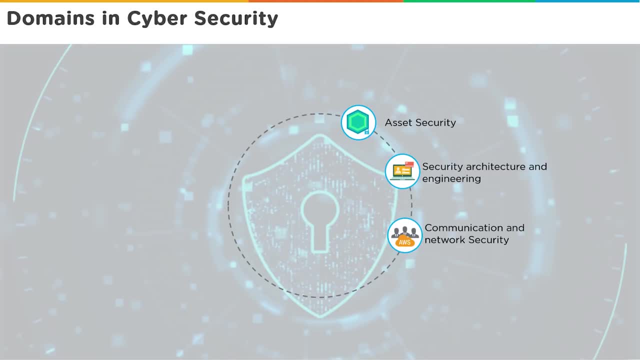 does you have to create those spots and ensure that those spots are monitored properly, are regulated properly and do not have any data leakages. Similarly, identity and access management. who is accessing my data? are they authorized to access my data and, if yes, how am I going to authenticate them? 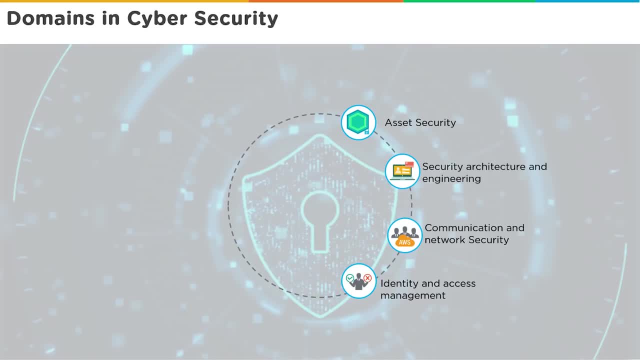 How am I going to track them home? How am I going to hold them accountable for whatever they have done? Even if a person is authorized to do something, we have to hold them accountable for that activity so that if something good, something happens later on, we can identify who made. 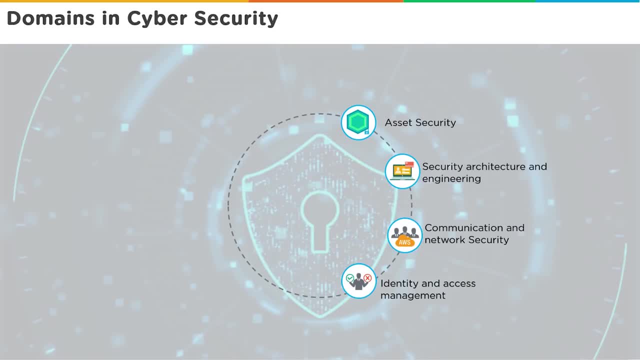 that change. So the identity and access management module will consist of us creating groups, policies, users, rules and interlinking them with the assets to ensure that only authorized people are able to access those devices. security operations on a day to day basis. we need to monitor the security of those devices. 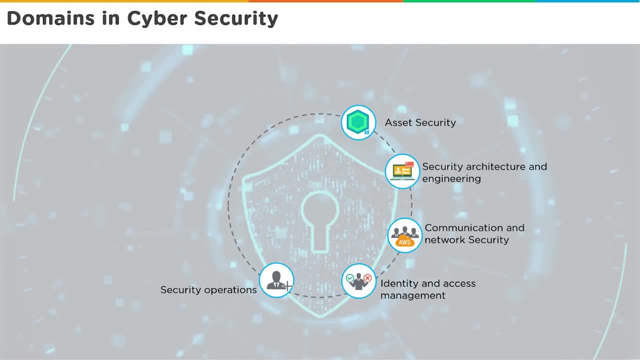 For example, if today I start facing a denial of service attack or somebody starts a password attack on my organization where they're trying to crack somebody's password, there should be some internal mechanisms that are in place which will try to identify these attacks one the appropriate administrator and that administrator will walk in and try to investigate that attack. 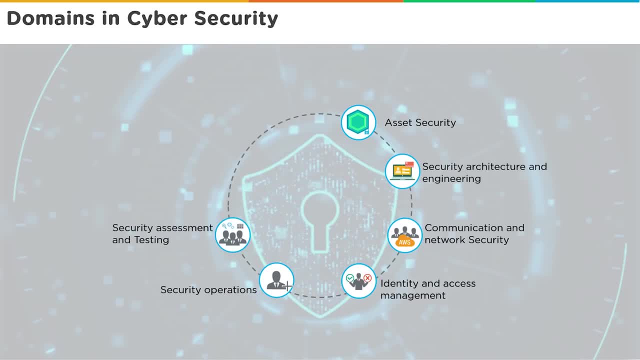 So day to day operations are a must: security assessment and testing. now that we all have these mechanisms in place, Are they going to remain constant for the rest of our lives? No, IT is ever evolving scenario, so we need to assess and test our security controls on. 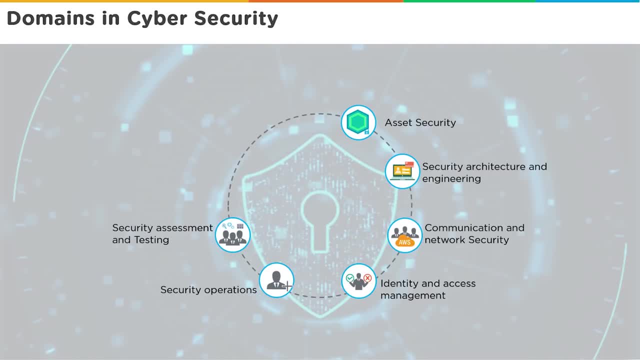 a regular basis to ensure that there are no gaps left. What I configure today may be irrelevant tomorrow, so I have to constantly keep on looking at the latest security trends, the latest vulnerabilities that are being identified, the patches that are being installed, and I have to compare my infrastructure to all of these to see that. 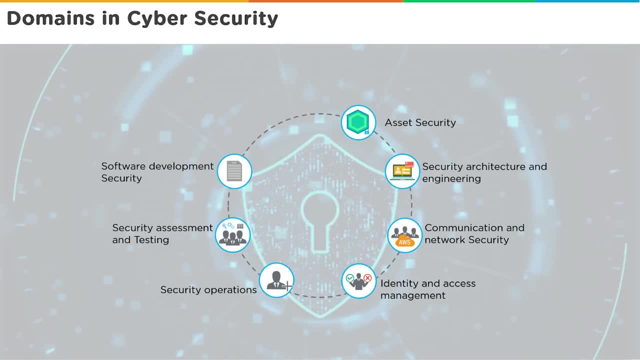 I am compliant The latest security standards, software development security. So if you're an organization who is developing software and who's going to sell that software to end users, security becomes a huge part because the end user or the buyer- if it is an organization- is going to ask what kind of security testing was done in the application. 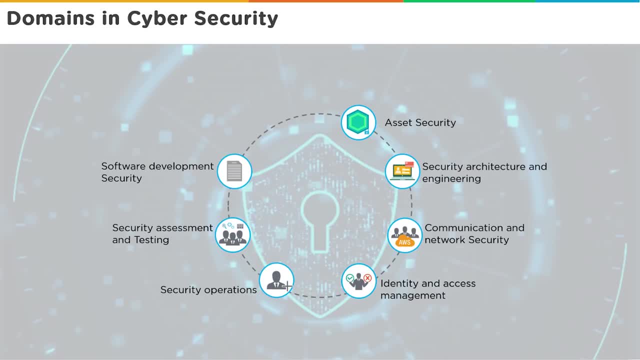 So that brings us to a software development lifecycle, which a lifecycle which talks about how you're going to create that code, how you're going to test that code, ensure that the code is secure enough. So you need to follow secure code. Okay, Coding practices are going to test the software over and over again till you're satisfied. 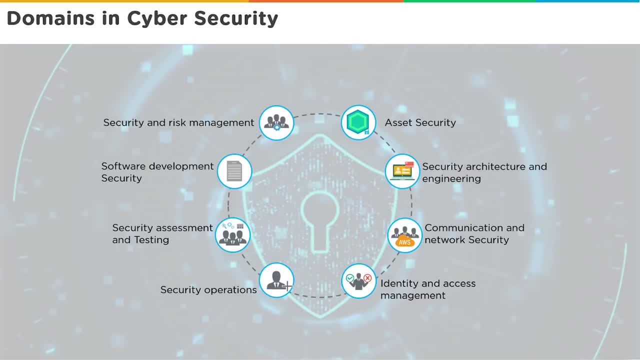 with the outcome, and then security and risk management. Now, when we come to risks, risks are basically events that may occur, compromising the security of an organization. So it is very important that we identify these risks, we map these risks, we verify how that risk is going to impact the business and then try to figure out security controls to mitigate. 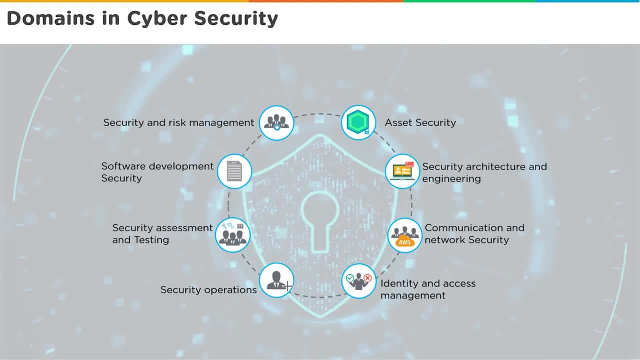 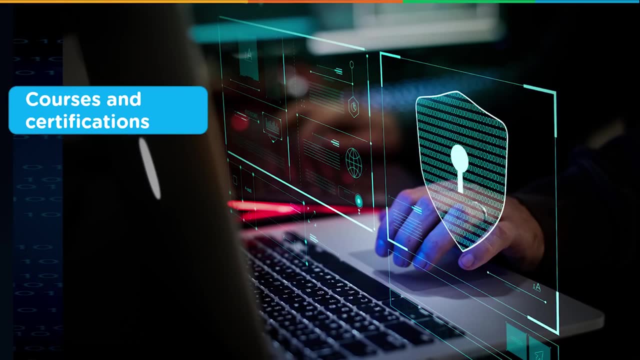 that risk or bring it down to manageable aspects. So that's a lot of talk, that's a lot of domains, that's a lot of attacks that we have discussed. Now let's see what kind of courses and certifications are available for us to enhance our careers. 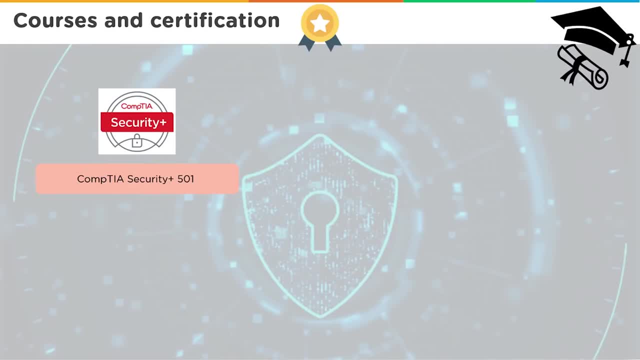 and address all of these domains, all of these attacks. So, starting off from a technical perspective, where we are going to look at ethical hacking, or security, where we are going to assess and do a vulnerability assessment and penetration test, there are certifications from Comchia, like security plus, or from EC Council, which 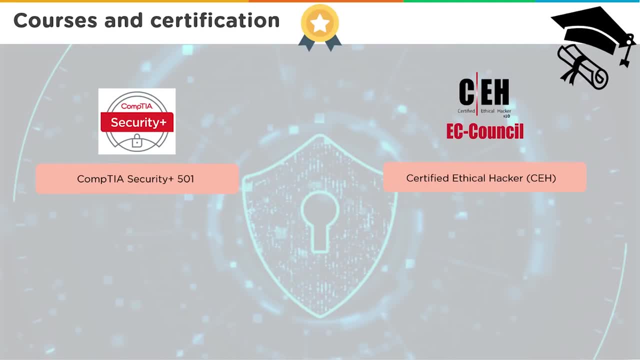 is the certified Ethical hacking training which basically allows us to become vulnerability assessment and penetration testing experts. So we'll be, technically, we testing each and every device and trying to hack those devices to see if that vulnerability is real and what can be attained out of that vulnerability. 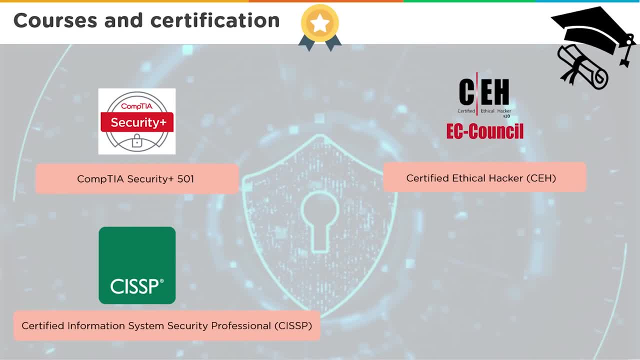 CISSP is very high level is a very high level certification that normally is considered as a management level certification right. So just to get certified yourself, you need at least five years of experience in the IT security field. This is where you get certified and you're basically a chief information security officer. 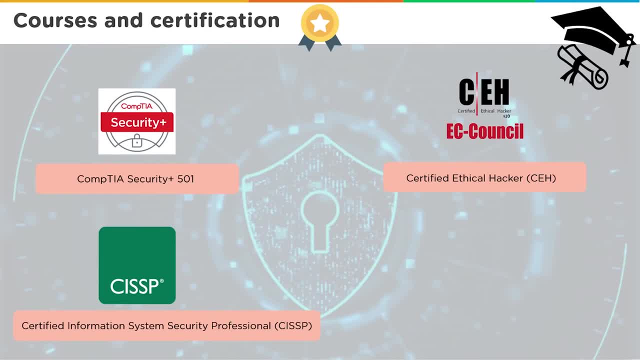 where you're going to develop policies, procedures and security control mechanisms and you're going to standardize the security policy of the entire organization. Then you've got the CISA, or also known as the CISA- certified information systems auditor. It is from an organization called Asaka. 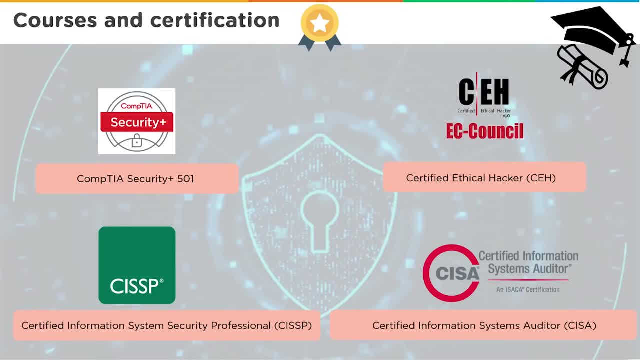 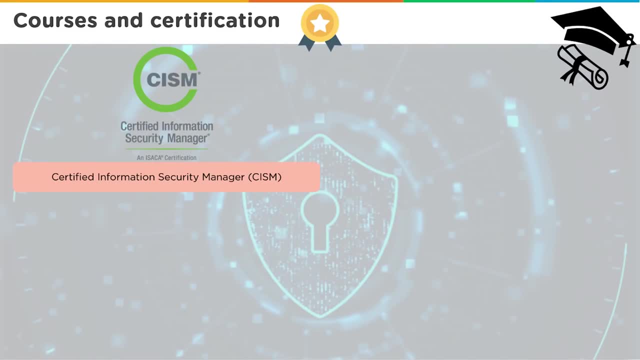 It's more on the system side, where you're going to audit systems and you're going to verify that they are adhering to the policy Policies that you have implemented. the CISM or system is a certified information security manager. This is again a project based oriented approach where you're going to manage the security. 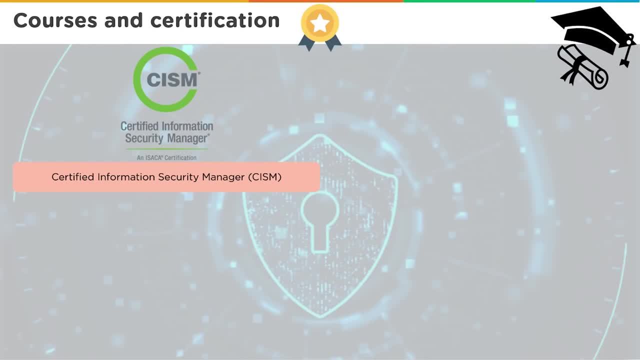 of an organization and you're going to look at all the daily operations of the security operations center and you're going to maintain and manage all of those functions overall. When we talked about risk assessment and risk strategy, for that we've got the CISC, which 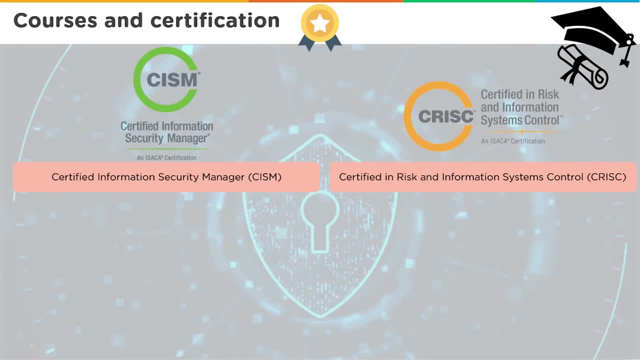 is a certified in risk and information systems Control. now for these certifications. this is more on the business side of everything, where you understand the business processes, you understand the business requirements and, based on those business requirements, you compare the technical implementations of compute of computing powers that you have implemented and then you're going to compare how those 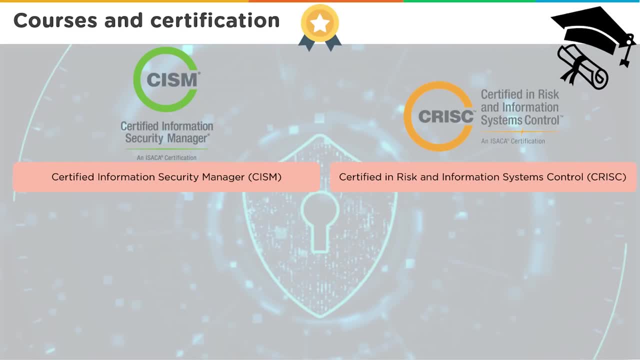 technical aspects can be converted into a risk. For example, a vulnerability assessment identifies a possible sequel injection attack. Now technically, it becomes Technically A big risk. however, which system is being affected if that system gets compromised? what kind of losses is the organization looking at? how much are they going to be? what kind of losses? 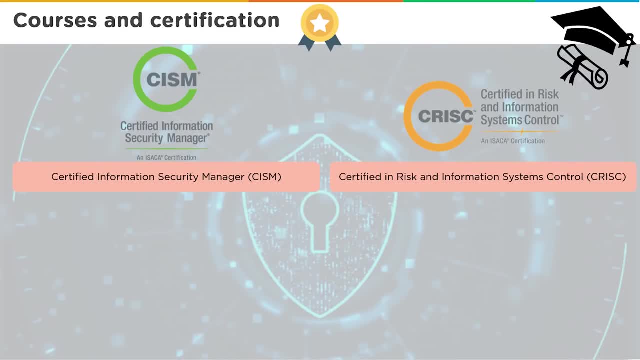 the organization is looking at? are they looking at lawsuits from the customers? are they looking at penalties from regulatory authorities? So that risk that implied, risk that this, if this vulnerability is hacked. that is the aspect that you want to look at when you're looking at risk information and controls. 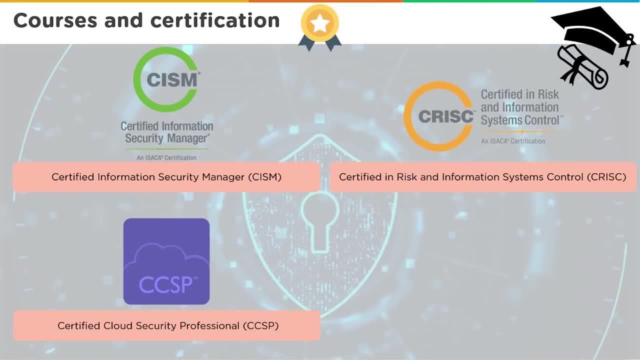 Similarly, you have CCSP. this is a certified cloud security professional certification. So this is especially for people who want to deal with the cloud, Let it be a public cloud, a private cloud or a hybrid cloud. this certification gives you an architectural overview over different aspects of cloud and how you want to implement security. 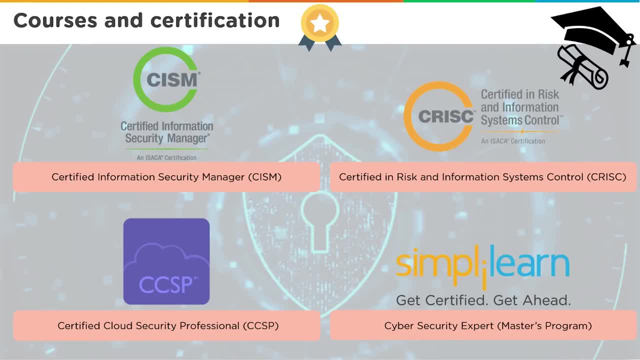 in a cloud based scenario. So simply learn offers all of these certifications with trainings from certified professionals. So there's a master's program from simply learn. We have a master's program Which talks about becoming a cyber security expert, which includes all of these trainings. 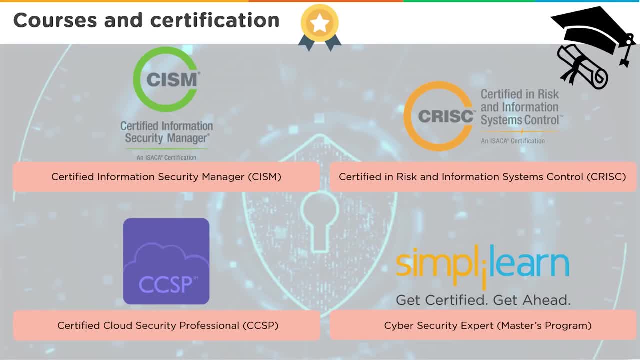 once you have these kind of trainings and you get those certifications on your profile, That's where you're basically a cyber solutions or cyber security expert and you'll be designing and developing security policies, structures, architectures for various organizations and helping them enhance the security of their infrastructure. 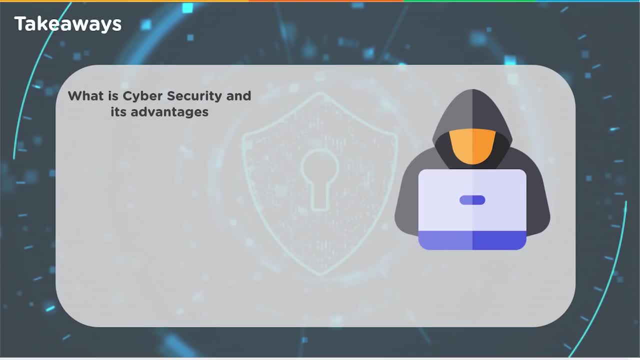 So let's see what we have talked about during this entire video. First, what is cyber security and its advantages? we have talked about the confidentiality, integrity and availability triad and we have talked about the threats that pose for the CIA triad. motives behind cyber crimes. we have seen what motivates people to attack other computer. 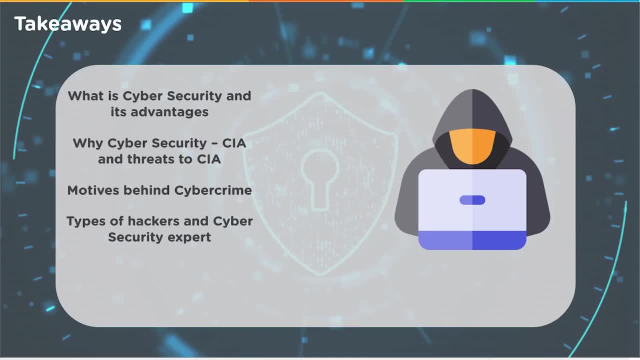 systems and steal data from it. we have talked about types of hackers and cyber security experts. we have talked about white hat, black hat and grey hat hackers. there are other types that we have talked about as well. we have looked at the domains that are available in cyber security and the courses and certifications that can be mapped with these domains. 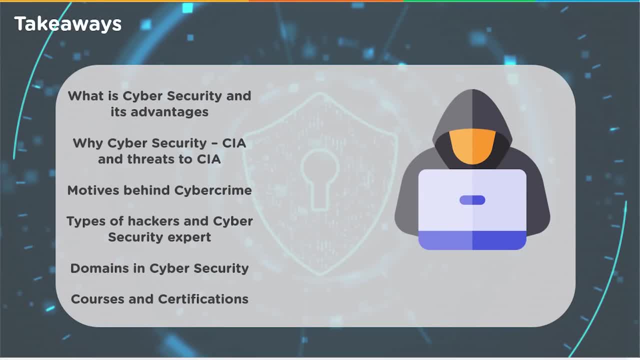 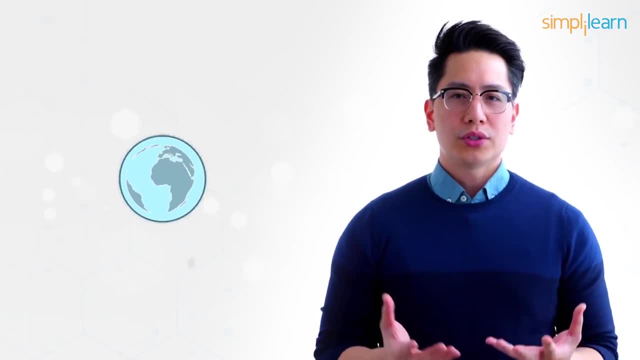 So this is what what we have discussed within this session. If you have any further queries, please go ahead and post them in the comment section and we'll try to address them as soon as possible. With the world turning, virtual cyber attacks are constantly flooding new headlines. 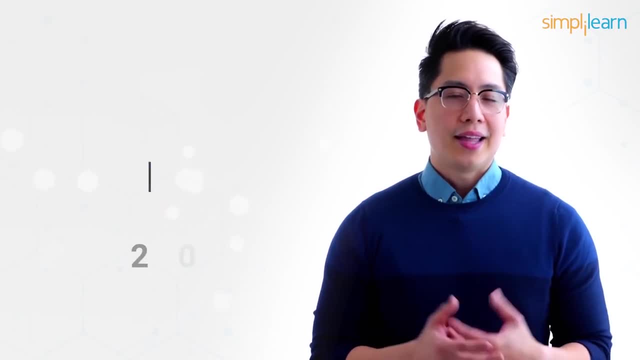 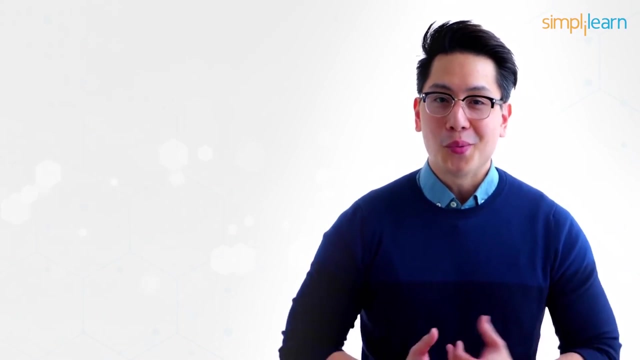 COVID-19 accelerated the current digital transformation, and the year 2020 witnessed several data breaches. Since technology has become more intertwined with our daily lives, It is no surprise that the need for skilled cyber security professionals is increasing. On that note, everyone welcome yet to another exciting video by simply learn which will. 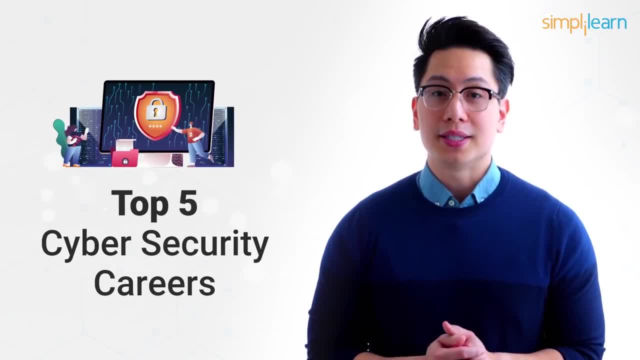 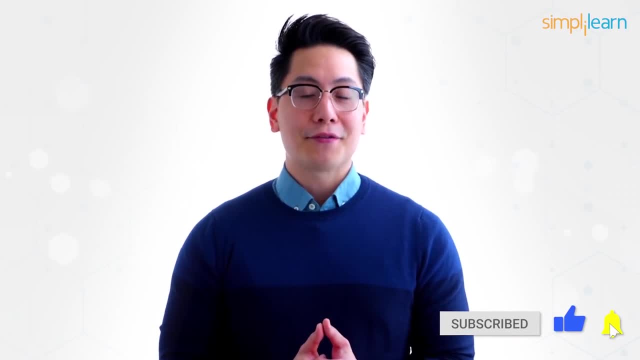 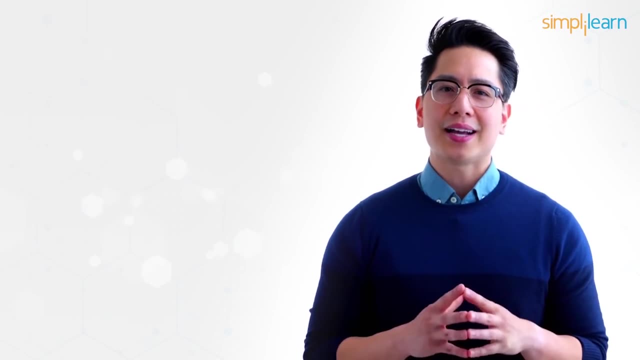 take you through the top cyber security career options available today. But before we begin, if you're new here and haven't subscribed already, make sure to hit the subscribe button and that bell icon for interesting tech videos every day. There is a significant lack of skilled cyber security professionals who can tackle the 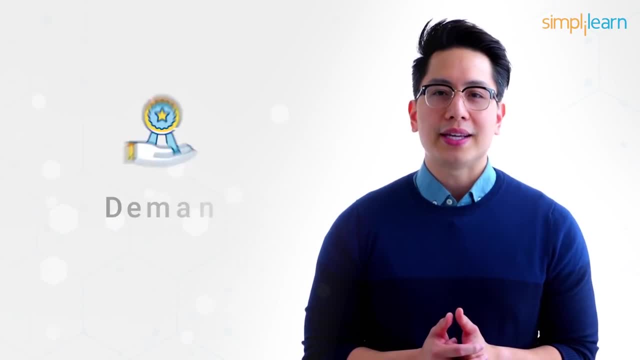 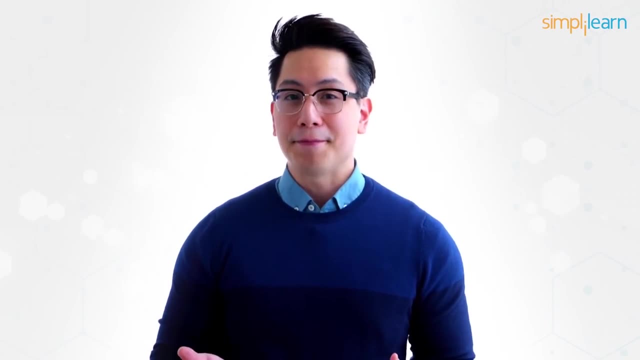 challenges faced daily. Hence a career in cyber security is demanding and equally rewarding. Finding the right career path in the cyber security industry isn't always easy. Here we are here to help you with that. There are a few prerequisites for a career in cyber security. 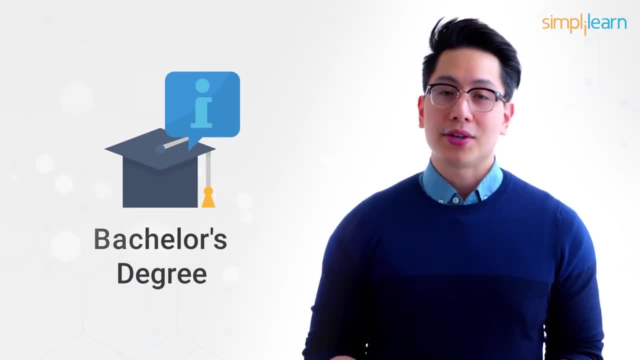 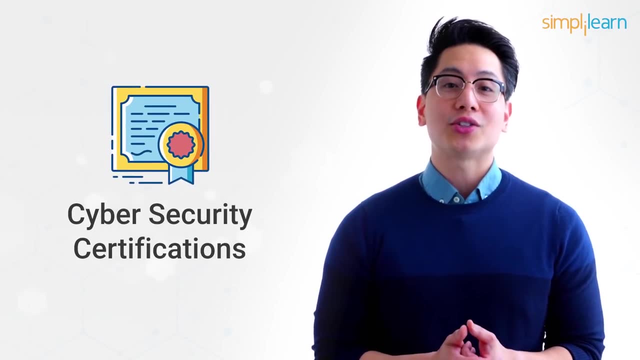 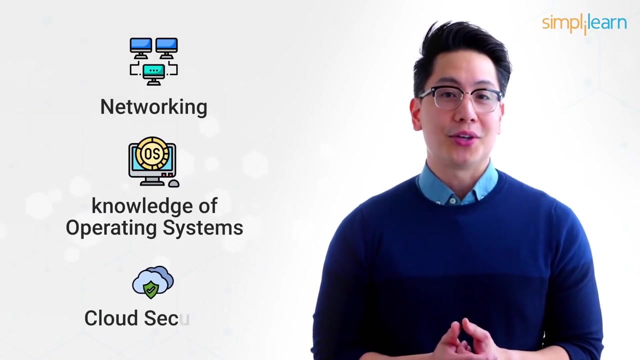 The basic one being a bachelor's degree in a subject relating to cyber security. However, if you don't have a relevant degree, you can always take up relevant cyber security certifications and kickstart your cyber security journey. A few other skills like networking, knowledge of operating systems and cloud security are. 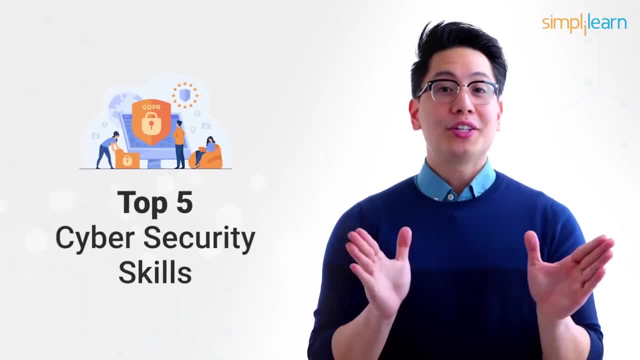 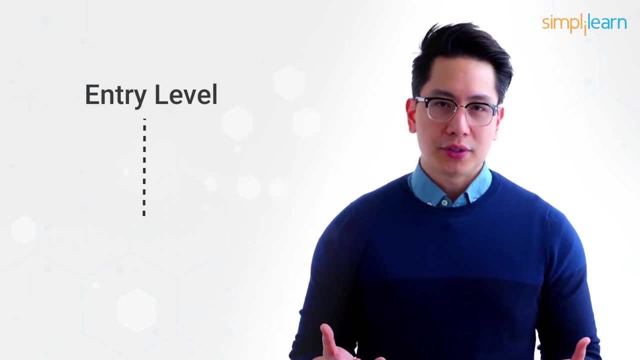 required to start and grow your cyber security career. You can check out our video on the top five cyber security skills to know more. Cyber security jobs vary from entry level to executive management and everything in between. There are several cyber security paths available today. 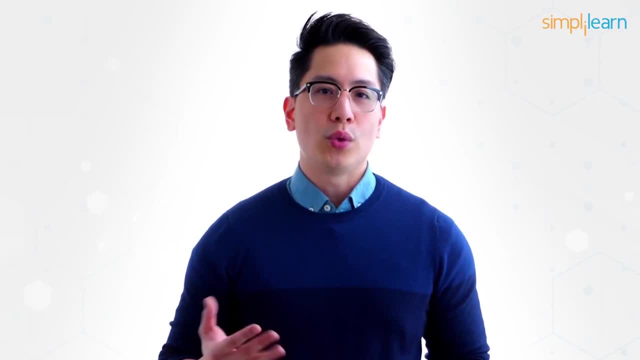 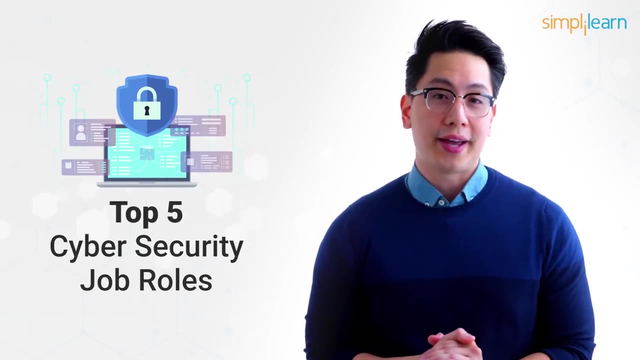 It is best if you start with entry level and then move on to the next level with the help of certifications and relevant experience. Here Let us have a look at the top five cyber security job roles today. The first job role is that of a network engineer. 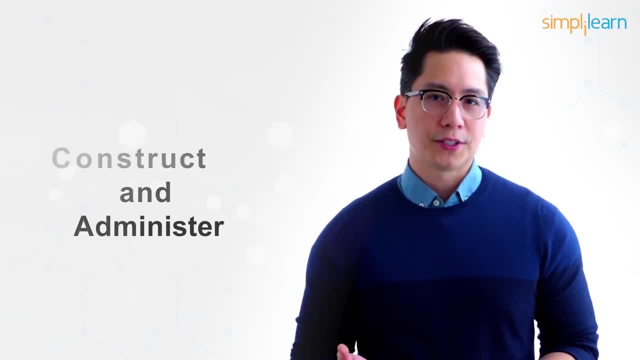 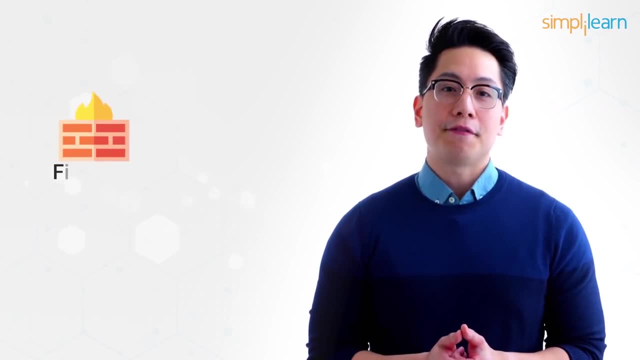 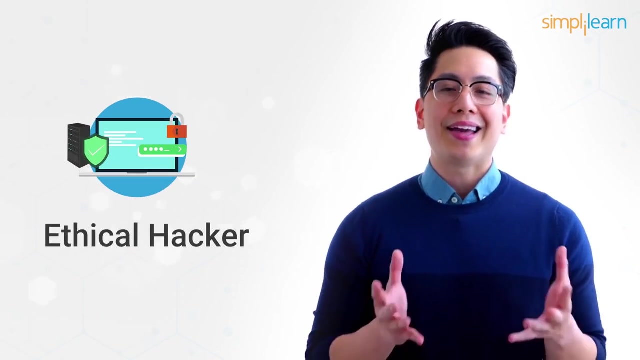 Network engineers construct and administer a company's computer networks. They are responsible for installing, configuring and supporting network equipment. They also configure and maintain firewalls, switches and routers. This entry level cyber security job can help you start your journey to become an ethical hacker. The annual average salary of a network engineer in the US is $8,000.. The average salary of a network engineer in the US is $8,000.. The annual average salary of a network engineer in the US is $48,000. 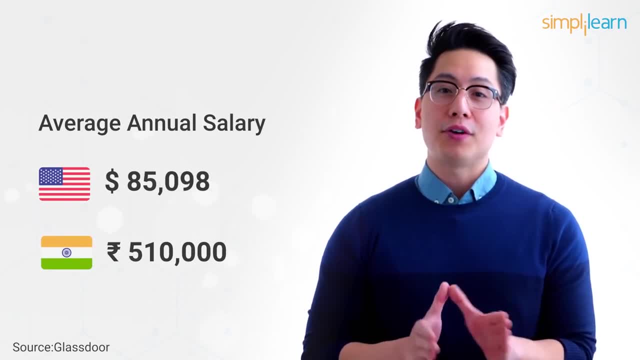 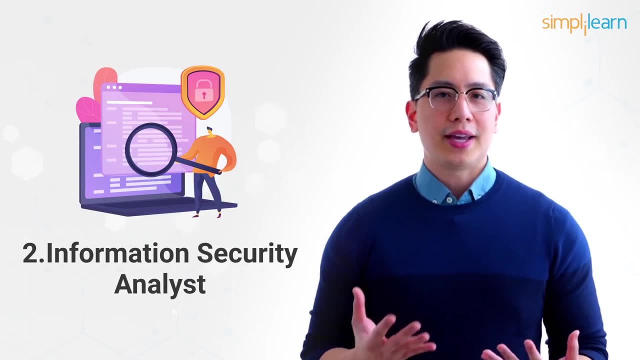 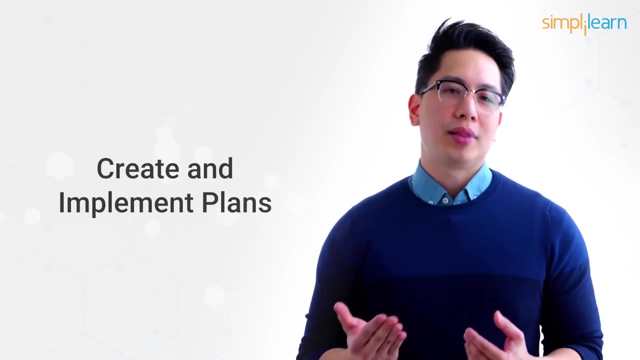 And in India it is around 510,000 rupees. Second on our list is Information Security Analyst. As an information security analyst, your primary duty is to protect sensitive information. Information security analysts create and implement plans for preventing cyber attacks. They monitor data access and ensure compliance with policies. Depending on the cyber threat, they decide if it has to be resolved or escalated further. In the US, an information security analyst earns $89,140 annually, And in India they earn 6,42,756 rupees. Third on our list is Ethical Hacker. 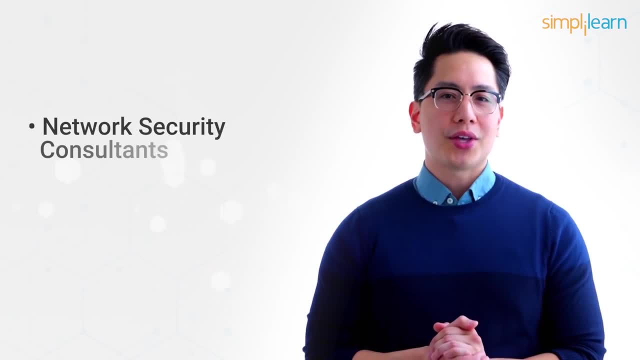 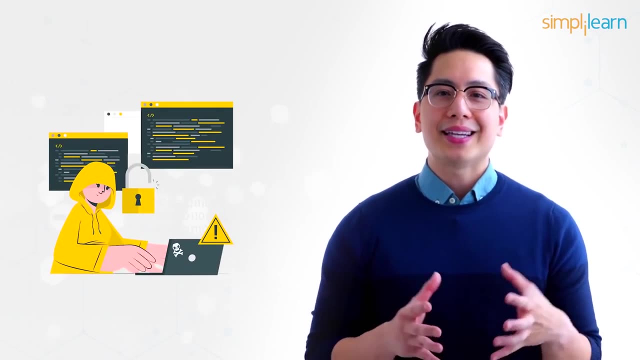 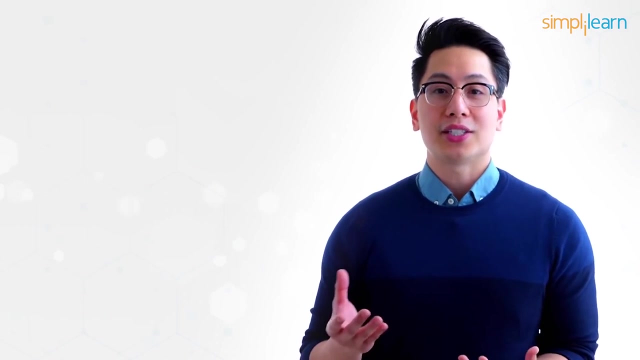 They're also known as penetration testers. They are network security consultants who identify and exploit system vulnerabilities just like how a hacker would do. They probe and test the network using various penetration tools and software. They also design new penetration tools and document the test results. 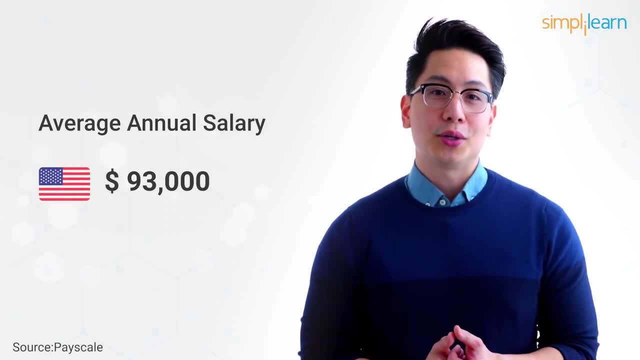 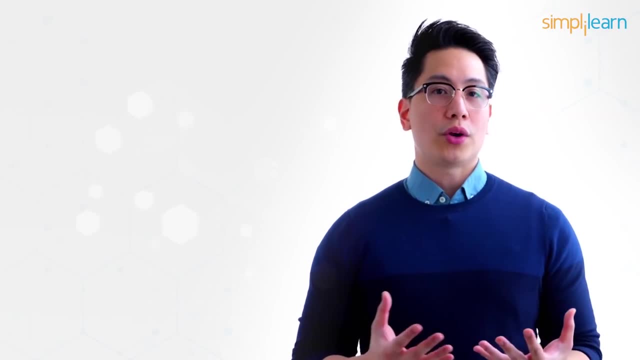 In the US, a certified ethical hacker earns around $93,000 on an annual average basis, And in India they make around five lakh rupees. The fourth job role that we are going to talk about is Security Architect. Security Architects, research and plan the security elements. 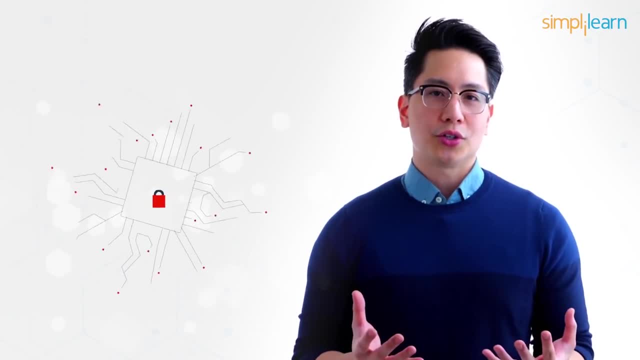 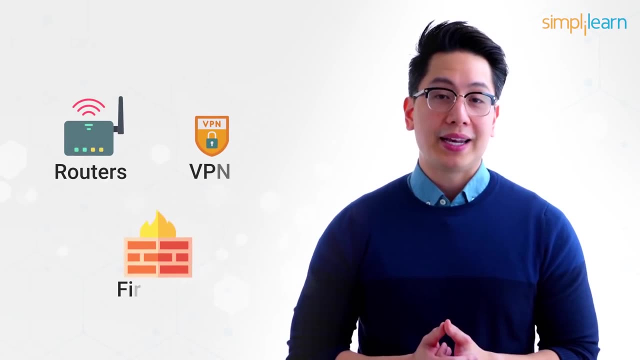 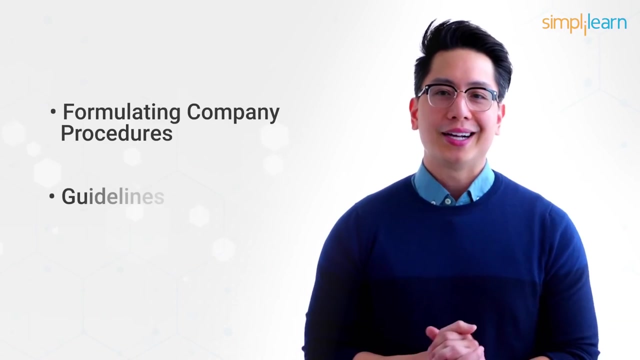 for their organizations. They design robust security structures that are capable of preventing malware attacks. A Security Architect approves the installation of routers, VPN and firewalls. Their duties go beyond just architecture building and including formulating company procedures, guidelines and user guides. 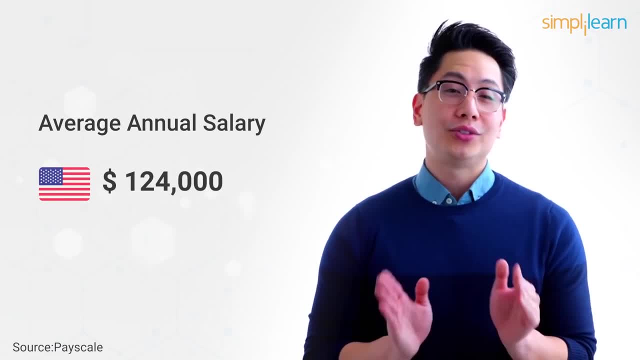 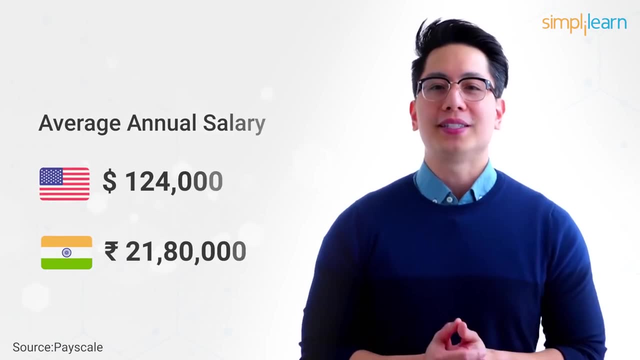 Security Architects in the US make a handsome sum of $124,000 a year on an average, And in India they make nearly 21,80,000 rupees. And finally, fifth on our list is Chief Information Security Officer CISO. 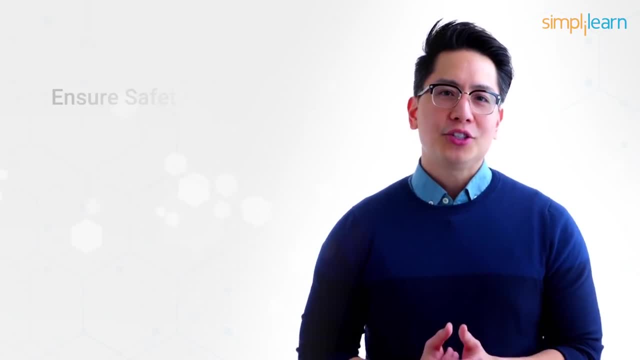 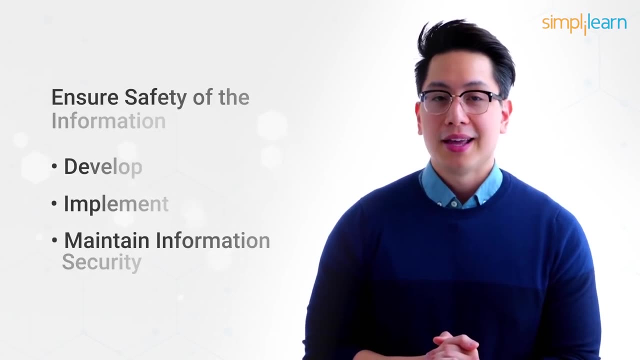 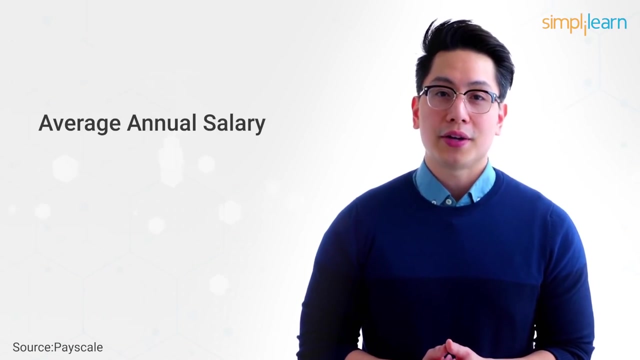 They are senior level officers in an organization. They ensure the safety of the information. they develop, implement and maintain information security and risk management programs. They also interact with stakeholders and regularly brief them with information security concerns. The average annual salary of a Chief Information Security Officer in the States. 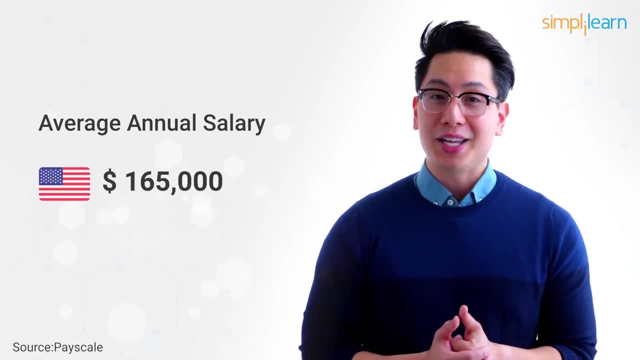 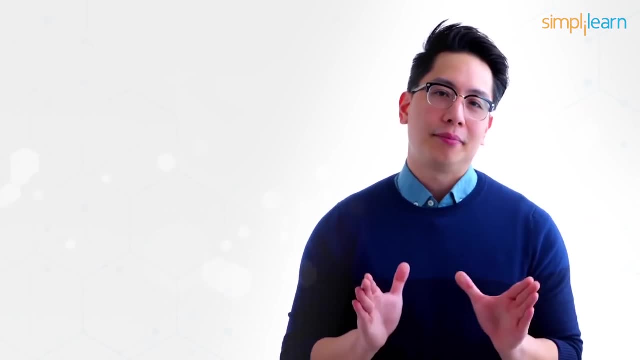 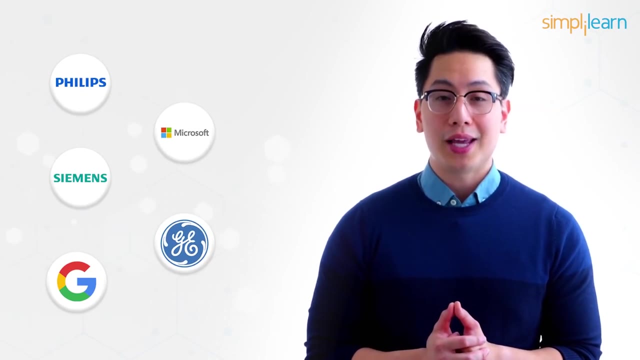 is a whopping $165,000 annually, And in India it is 22,22,845 rupees. Several companies are looking for skilled cybersecurity professionals: Philips, Siemens, Google, Microsoft and GE, to name a few. With passion, the right amount of experience. 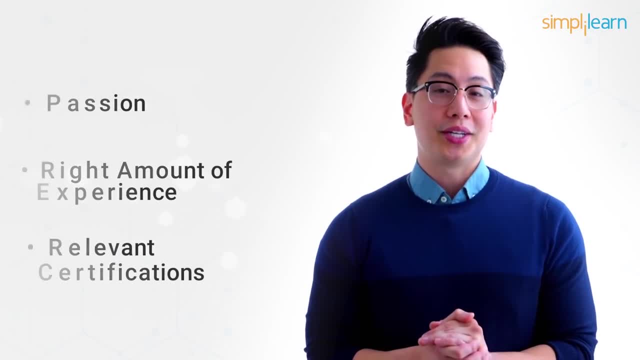 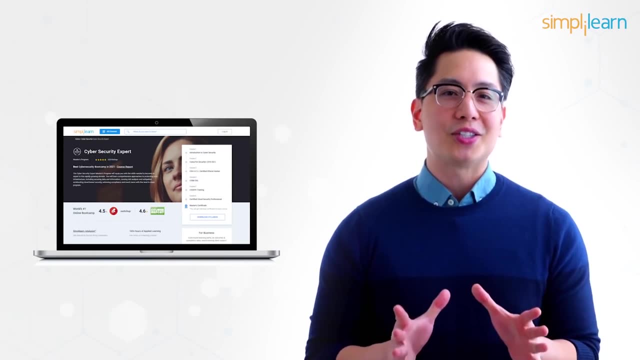 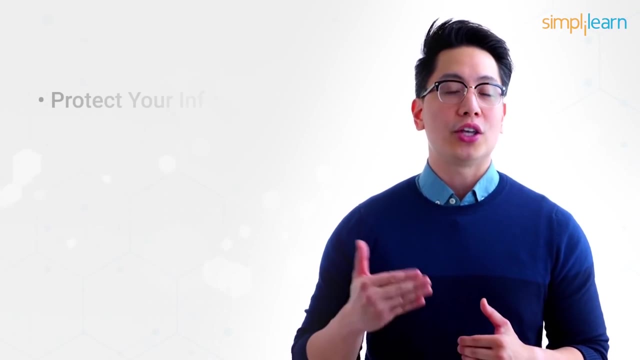 and relevant certifications, you can grow your cybersecurity career. You can check out Simply Learn Cybersecurity Expert Master's Program to equip you with the necessary skills needed to become an expert in this rapidly growing domain. This course will help you learn various methods as to how you can protect your infrastructure. 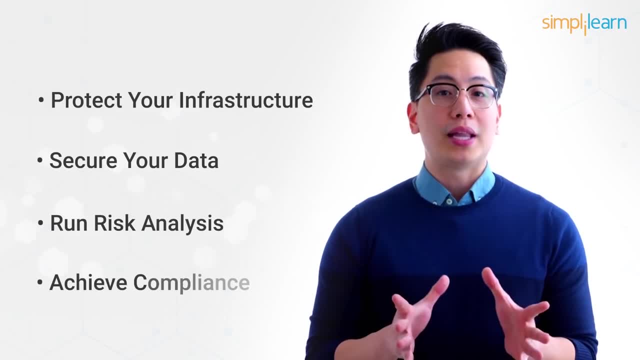 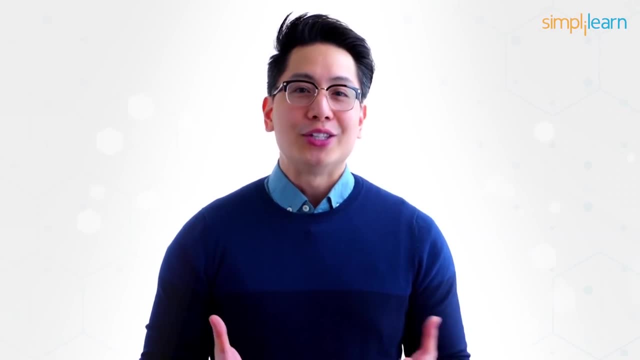 secure your data risk analysis, achieve compliance and much more So. with that, we come to the end of this video on the cybersecurity career. Think we missed anything important? Do let us know in the comments section below. Let's start off with networking questions. 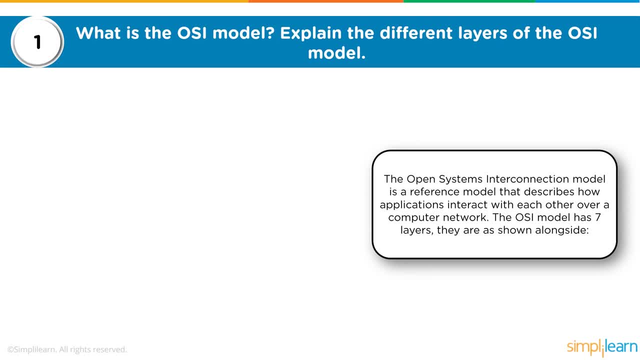 Let's start off with question one: What is the OSI model? Explain the different layers of the OSI model. OSI, largely, is a theoretical model utilized to understand networking and how data packets are created and how they are being processed by a computer. This is normally used by the TCP IP. 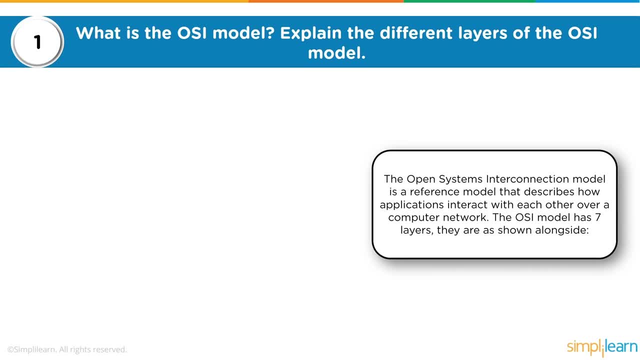 the transmission control protocol over internet protocol software suite. So OSI is known as the open systems interconnection model. It is a reference model that describes how applications are going to interact via the computer network. There are seven different layers that we need to understand. 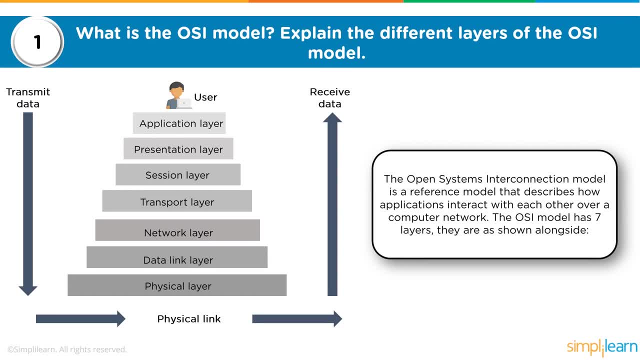 They are as follows. So in this diagram there are these seven different layers. We start off from the bottom. First is the physical layer, the data link layer, network layer, transport layer, Session layer, presentation and application- When such a question is asked in an interview. 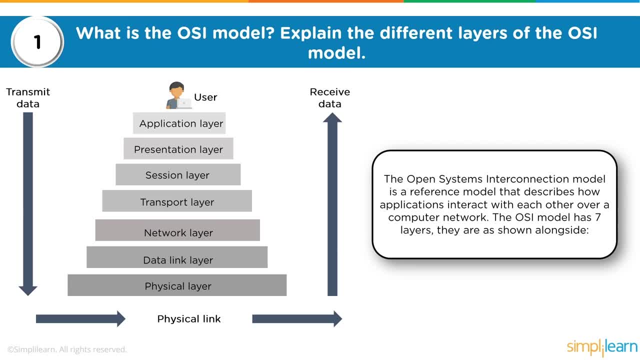 it is not only that we identify these seven layers, explaining what the OSI model is in the first place. We then try to identify these seven layers and we give a brief description about each and every layer. If there are any additional questions, they will come after this basic question. 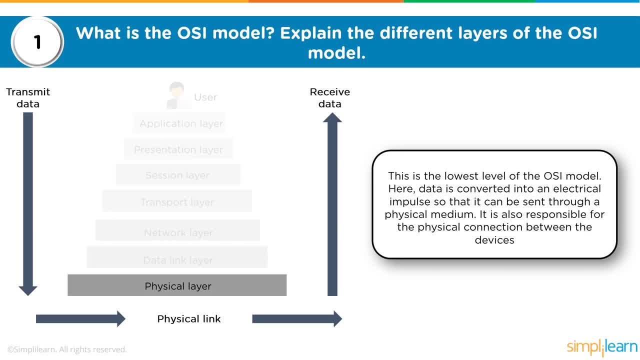 So let's start off with the physical layer. This is the lowest layer of the OSI model. Now, this is where any and every physicality of your computer comes into the picture. So it could be a network interface card, It could be an RJ45 or a CAT5 cable. 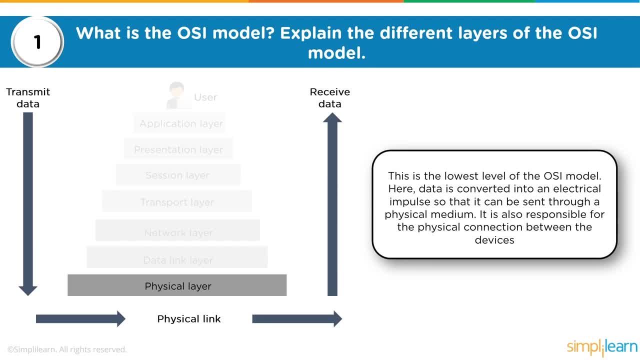 Anything that allows data to be transmitted physically from your machine to another machine. Next comes the data link layer. So, on the data link layer. as far as networking is concerned, we just need to understand that data packet is encoded, decoded into bits, at this layer. 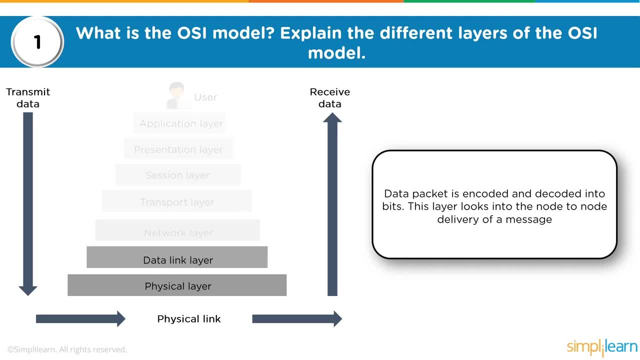 This is also the layer that deals with MAC addressing, So the physical address of every network interface card, which is the MAC address which is utilized to route data packets over the network. This is where the MAC address resides on the data link layer. 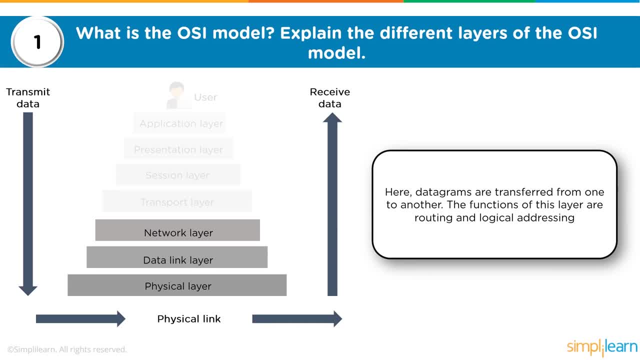 The next layer is the network layer. Here data grounds are transferred from one to another. The function of this layer are routing and logical addressing. The moment we talk about routing and logical addressing, IP addresses come into the picture. IP version four. IP version six. 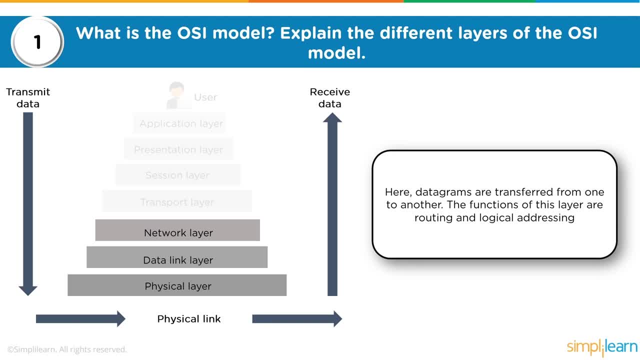 So network layer will deal with IP addresses and the routing of those packets. Then comes the transport layer. This is the layer responsible for end-to-end connections. That automatically signifies that this is where TCP and UDP will be working. TCP stands for transmission control protocol. 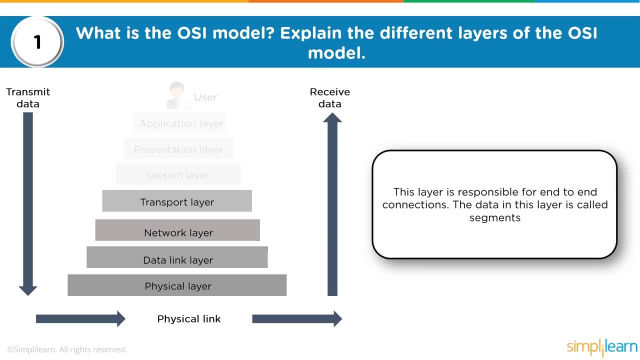 UDP for user datagram protocol. TCP is a connection-oriented protocol, whereas UDP is a connection-less protocol. These two protocols are utilized to establish connectivity between the two layers of the network. TCP is a more reliable method of connectivity because there are a lot of packets that are sent across. 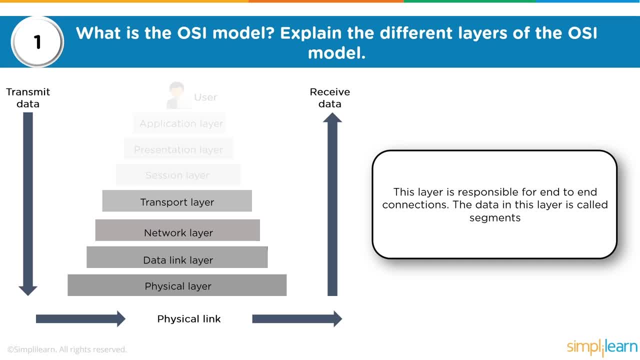 to verify that the data has been sent, data has been received, and so on and so forth, Whereas UDP is a connection-less protocol where data is just dumped without verifying whether the receiver actually receives that data or not. So, in a nutshell, on the transport layer. 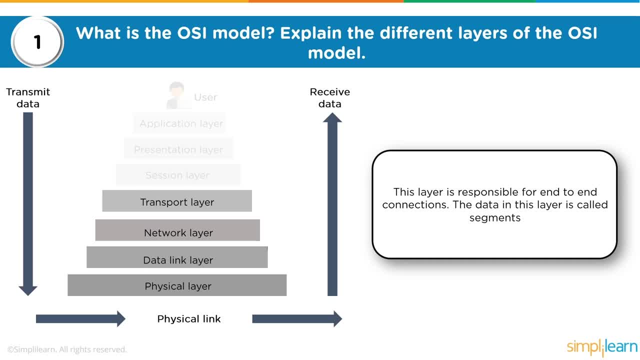 TCP and UDP make their appearance, and this is where that functionality lies. Then comes the session layer. This controls signals between the computer. it establishes, maintains and terminates connections between processes. So in the transport layer we talked about TCP and UDP. 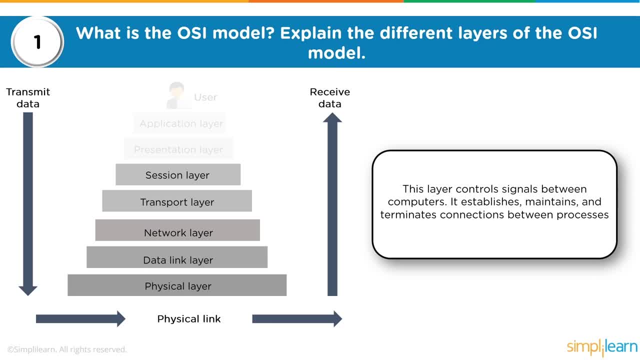 UDP being a connection-less protocol where data is just transmitted without verifying whether the receiver received that data or not, Whereas TCP we studied is more of a reliable protocol. Thus there are different packets signals that will be sent across to verify that data has been transmitted. 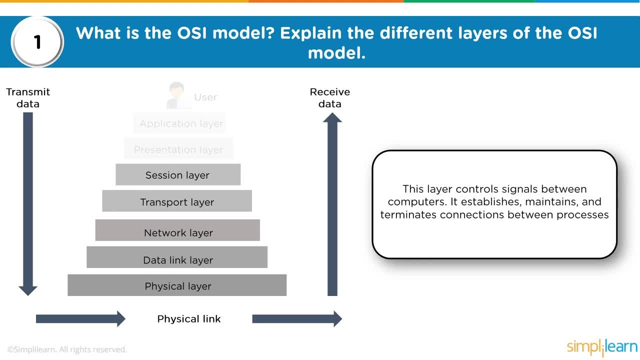 it has been received properly and then the next segment of that data is being sent. So those control signals are established using the session layer. So the three-way handshake of TCP, the acknowledgement packets and those kind of packets will be taken care of on the session layer of the OSI model. 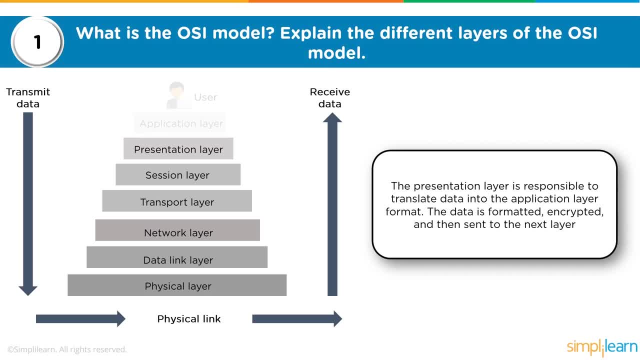 Then comes the presentation layer. The presentation layer is responsible to translate data into the application layer format. So the formatting right, MIME or encoding that is being utilized, The UTF-8 character set that we utilize for presentation, Encryption mechanisms, All of these work on the presentation layer. 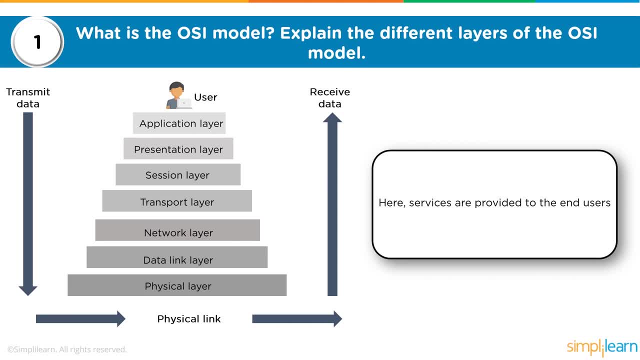 And finally comes the application layer, where the application itself uses a particular protocol, so that the other machine on the receiving end, the application on that machine, will be able to understand what the communication was about, Right? So in a nutshell, if I start from up top, 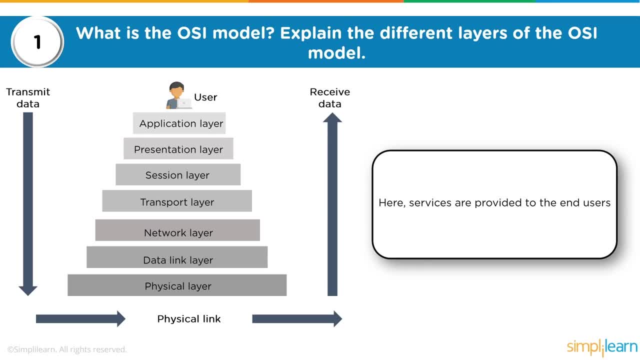 the application layer will deal with any of the data that the application is generating. So maybe an user input. You're logging in, you're typing the username password. All that data will be constructed, let's say, into an HTTP or an HTTPS format. 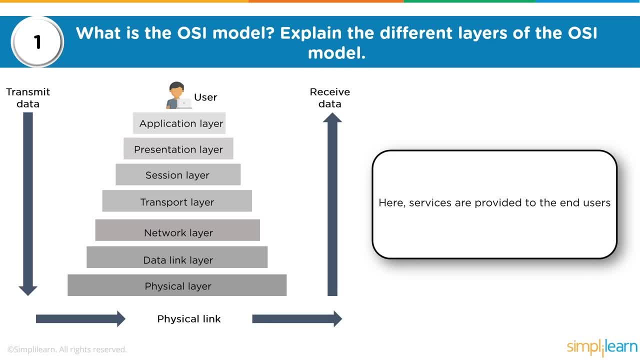 That's where the application layer comes into the picture. Then the formatting of which into UTF-8 and the encryption of which would be done at the presentation layer. Then the transport layer and the session layer would kick in to establish a TCP session. do the three-way handshake establish that connectivity? 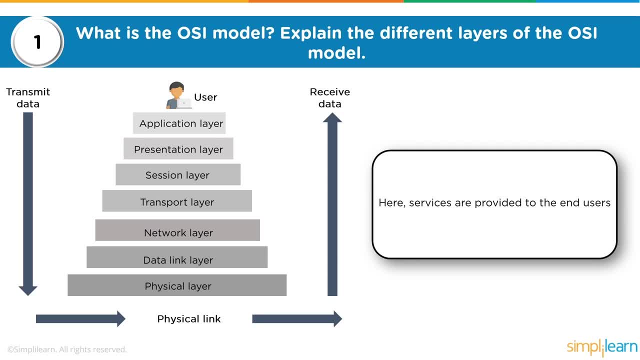 IP addressing would be done on the network layer, MAC addressing would be done on the data link layer, And when everything is ready on the physical layer, the packet will be sent out At the receiving end. the packet will be received on the physical layer. 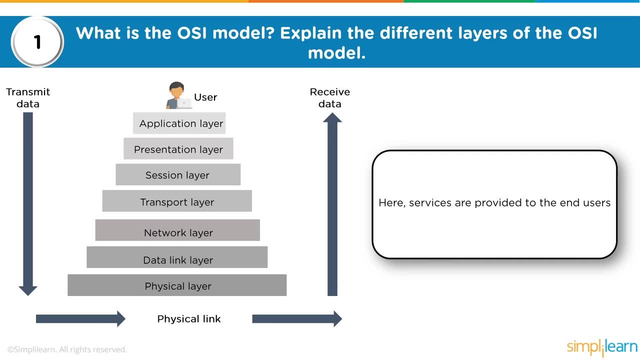 and then all these layers will be reversed And finally, at the application layer, the data will be presented to the application, who would then execute it and showcase it on the screen of the recipient. So this is the way you want to explain this question. 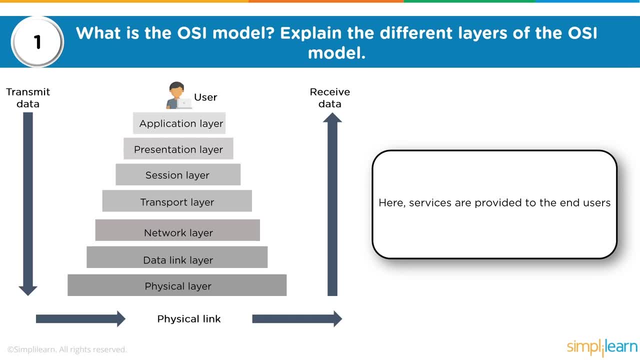 You want to be very concise, precise about what you are explaining. You don't want to go into two hypothetical scenarios. You don't want to delete a layer with the layers. You just want to give the basic functionality. You want to demonstrate that you understand. 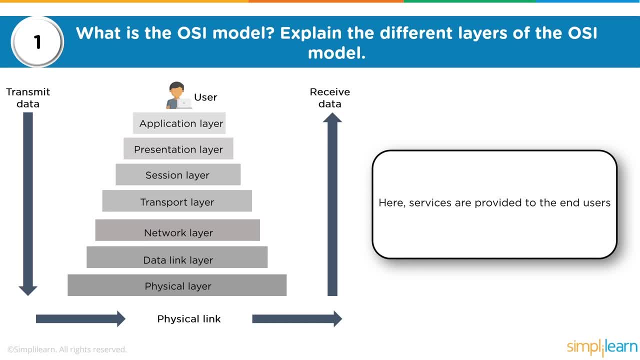 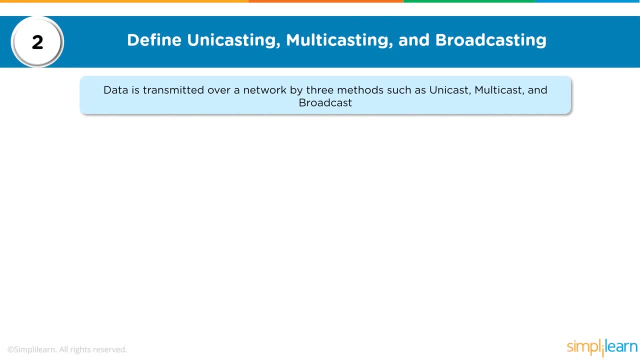 what the OSI layer is, how the computer functions, and you want to move on from there. If the interviewer has any further follow-up questions, they will ask those specific questions. So that's question one. Moving on to the question two, Question two is: define unicasting. 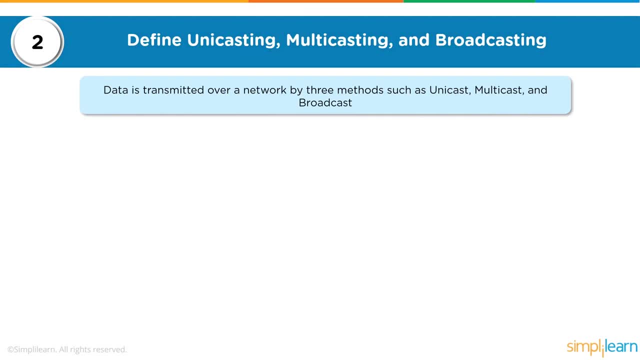 multicasting and broadcasting. Now, this is a question which can be very lengthy, But, again, most of your interview questions are designed that way. It's basically to understand how much, conceptually, you are aware about these technologies. So you have to be very concise. 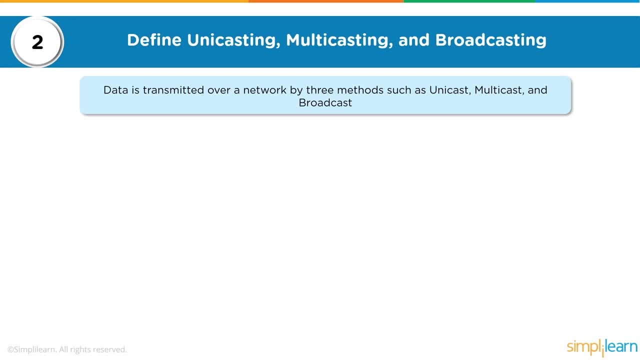 Don't go rattling about technology too much, But in a concise manner, just try to explain what these things is. So when data is being distributed, it's being transmitted over a network. It can be transmitted either in one of these particular manners. 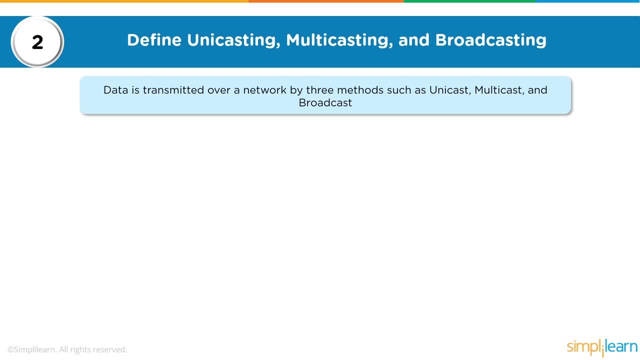 It can either be a unicast multicast or a broadcast. So what is unicast? Unicast is when a message is sent from a single user to a single receiver, So one-to-one right. So one machine talking to another machine and nobody else. 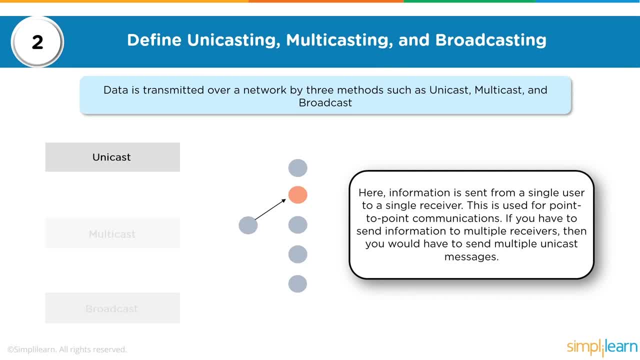 So also known as point-to-point communications, One point to one point. If you have to send information to multiple receivers, then you will have to send it using multicast, Right? So this is where your multicast networking comes into picture. So in our case, let's assume it's a network- 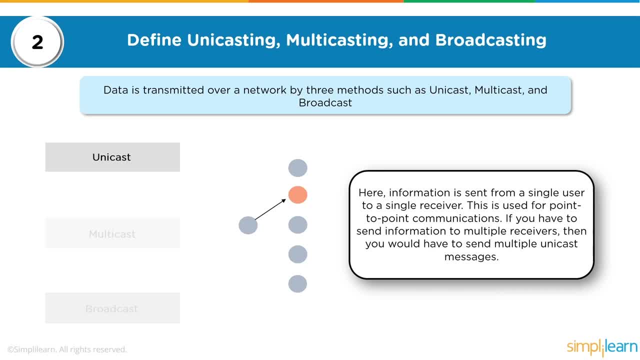 where there's a class C network, approximately 255 odd machines, And within these there are two machines that want to talk to each other. If they want to talk between each other, it would be a point-to-point communication where they will utilize unicast. 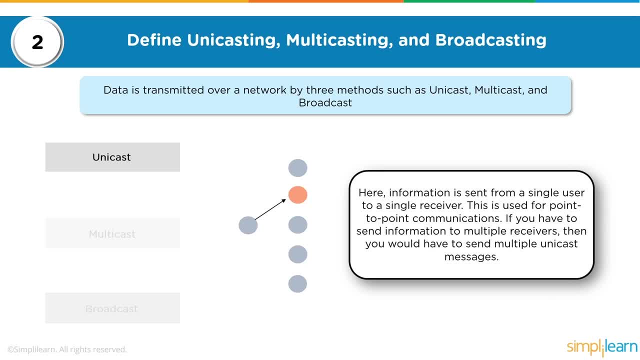 where only these two machines will have visibility of that conversation and the other machines will not even realize that this conversation is taking place. If one machine wants to talk to multiple machines, then the multicast comes into the picture, As the name suggests. in this mode of communication, 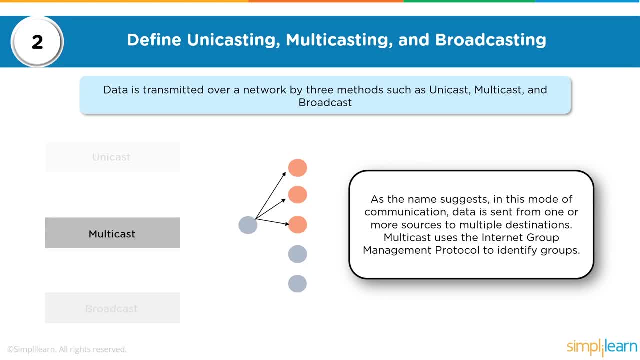 data is sent from one or more sources to multiple destinations. Multicast uses the Internet Group Management Protocol, also known as the IGMP protocol, to identify groups. So under this IGMP protocol, various groups are created, where machines are subscribed to those particular groups. 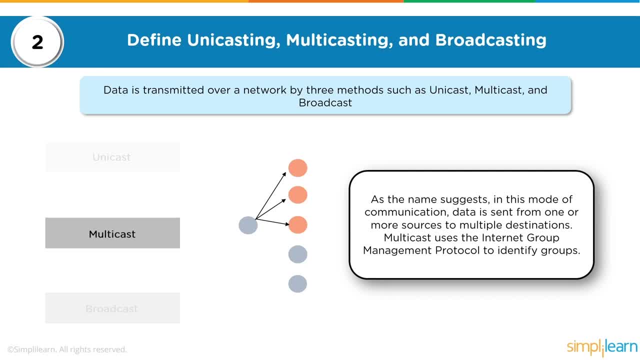 And whenever a message needs to be sent through those groups, it will be identified by the IGMP protocol and then that particular message will be sent to those multiple machines that are members of those particular groups. And then comes the broadcast. The third method is known as the broadcast. 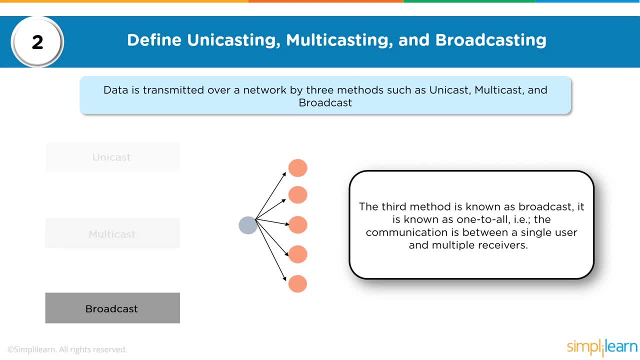 As it says, it is going to broadcast to all. So this is one-to-all. that is, communication between a single user and it is going to be sent to all the machines in that particular network. So the three ways, unicast is one-to-one. 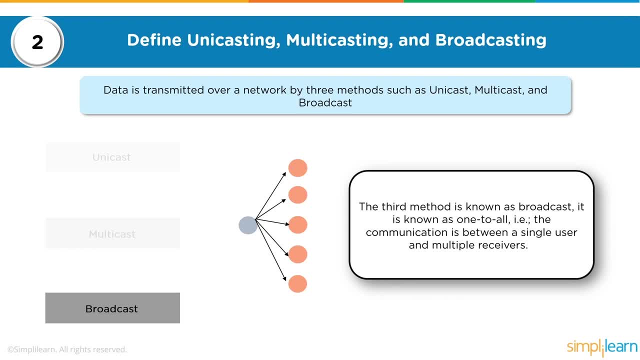 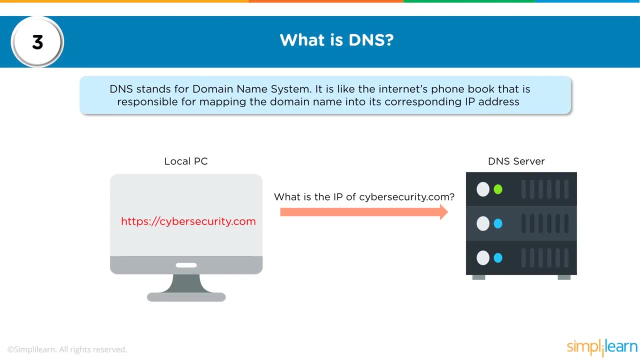 multicast is one-to-many and broadcast is one-to-all. Then question number three: What is DNS? DNS stands for Domain Name System. It is like the Internet's phone book that is responsible for mapping the domain name into its corresponding IP address. 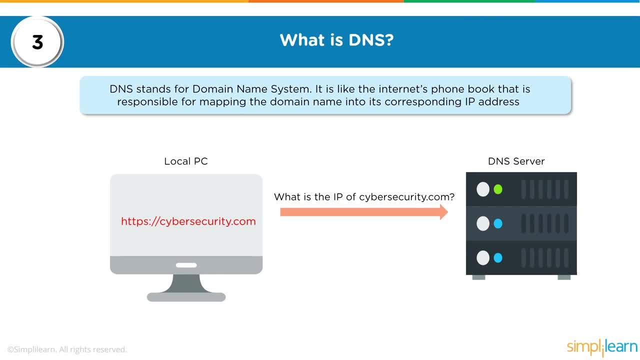 And let me give you an example over here. Whenever we go and open up, let's say, a browser, a Google Chrome browser, we type in wwwgooglecom and then we press enter and magically Google comes in front of us. 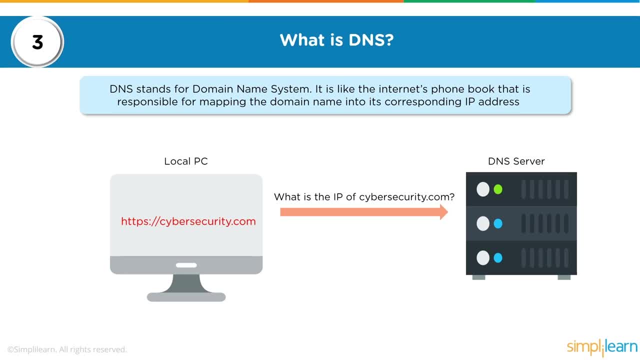 the website. rather. Now, how does the computer know who Google is? Because, as far as we are concerned, humans understand Google and words like that. Computers don't. Computers deal with binary zeros and ones right. And as far as Internet is concerned, 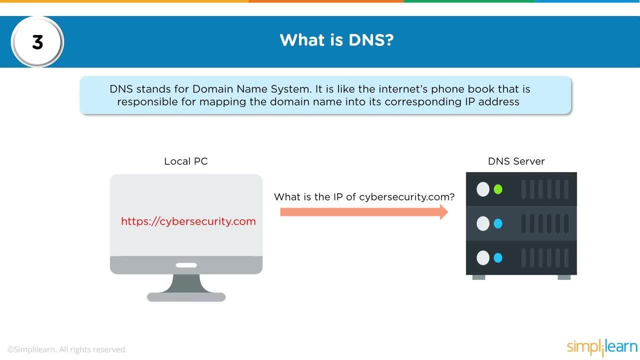 they will only deal with IP addresses and MAC addresses. So how does a computer know how to find Googlecom and where is it located? So the moment we type in in the browser window in the address bar googlecom and press enter, 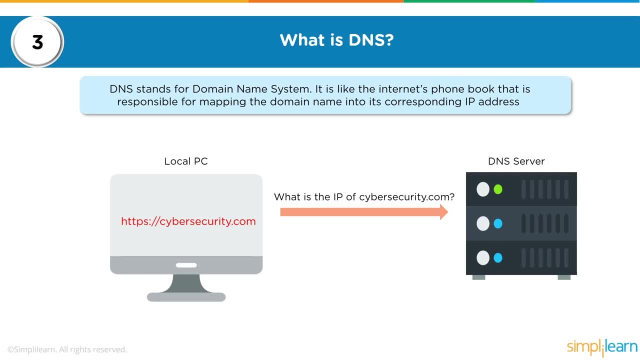 a DNS query is generated automatically by the browser where a packet is sent to our DNS servers asking what the IP address is. So, in short, DNS results domain names to their corresponding IP addresses. There is a DNS server which will have this index, A database of all the domains associated with their IP addresses. 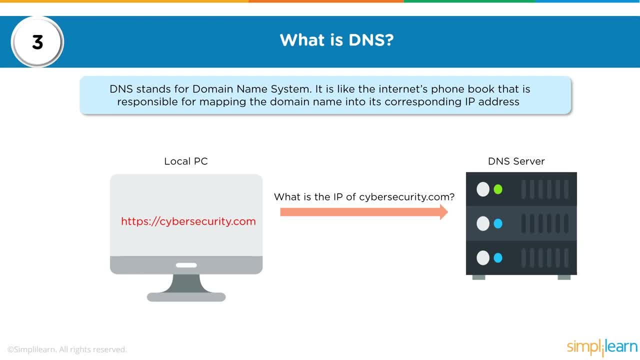 If one particular DNS server does not have that information that you are looking for, it may query another DNS server who may have that particular response. So the first thing is when you type in domain name, it gets resolved with the DNS. It identifies the IP address corresponding to that particular domain name. 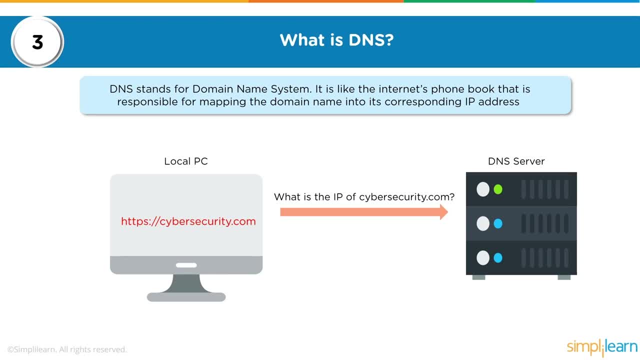 and thus allows the computer to route that packet to the particular server where that domain name resides. So in this scenario, if you look at the screen on the local PC you have typed in cybersecuritycom, There is a DNS resolution, a query that goes to the DNS server. 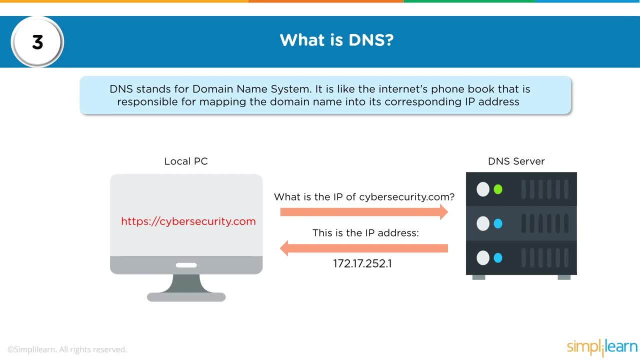 What is the IP of cybersecuritycom? The DNS server looks it up in its particular database. If it has the corresponding IP address, it will then respond back. The IP address is 172.17.252.1, after which the packet is sent off to cybersecuritycom. 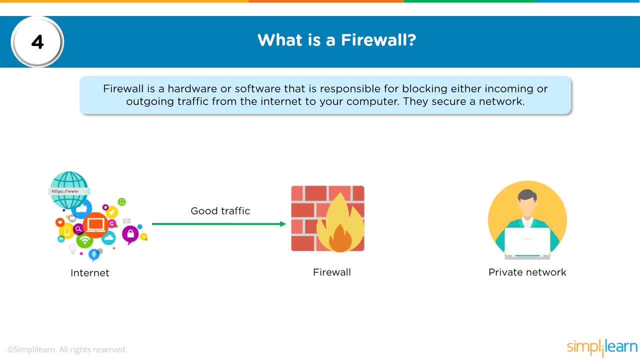 Moving on to the question number four, what is a firewall? Now, this is a very good question and normally a very basic answer that I've ever heard is that a firewall is a hardware and a software firewall, But that's the functionality of a firewall. 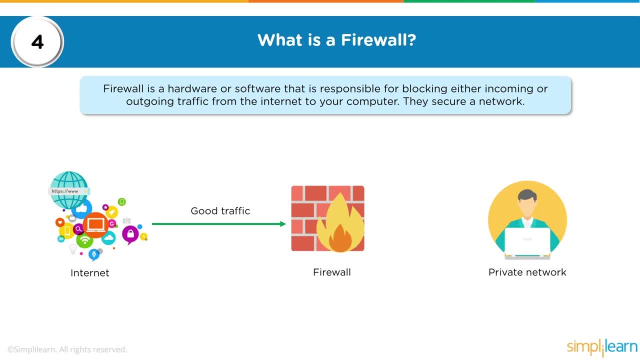 That is how we can install a firewall, But there are different types of firewalls and there is a specific functionality that a firewall is created for. So a firewall is either a hardware or software, but its responsibility is for blocking either incoming or outgoing traffic from the internet to your computer. 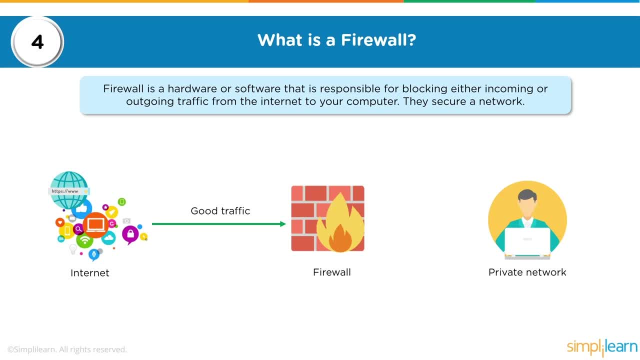 They secure a network. So, essentially, the firewall will allow a connection to happen or disallow a connection to happen. It won't go beyond that. That's the basic functionality of a firewall. So, based on the configurations that you have done, based on the rules that you have created on the firewall, 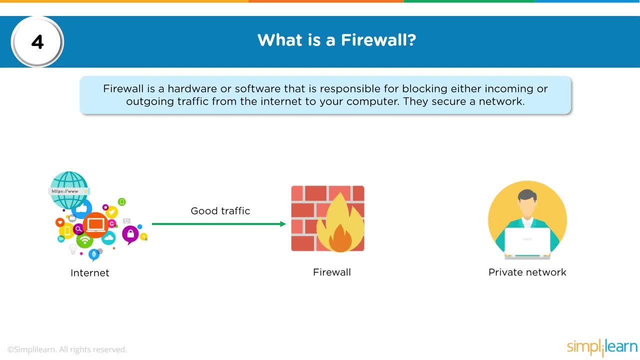 it will then, based on those rules, identify whether some traffic is allowed in that network or some traffic is to be blocked. So, as the screen shows, the firewall rules will analyze whether the traffic is good. If yes, it will allow. If the traffic is bad, it will block the traffic. 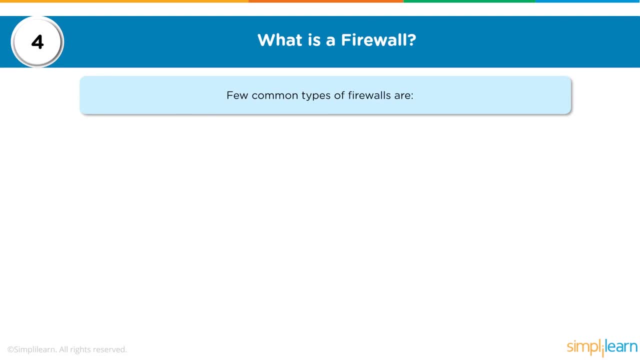 and not allow that connection from happening in the first place. Now there are a few common types of firewalls that also need to be included in the answer to this question, And the first one is a packet filtering firewall. These are the most common types that you will come across. 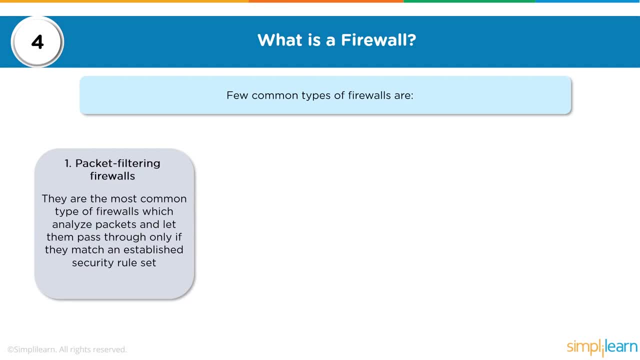 which analyze packets and lets them pass through only if they match an established security rule. Now here people do get confused. when we say that we analyze packets, People think that these firewalls will analyze the contents of that packet, which is not correct. 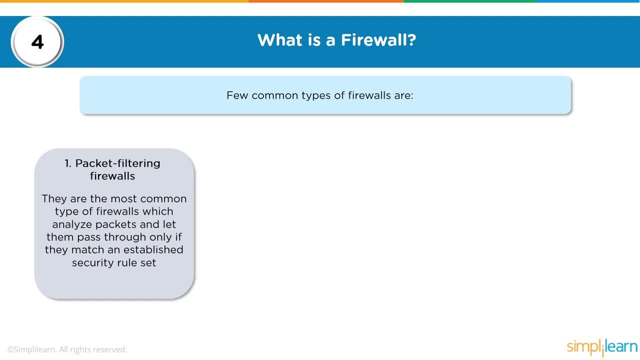 When a definition for a packet filtering firewall says that these firewalls analyze packets, it means that they are only analyzing the source and destination, IP addresses, port numbers and the protocols that are mentioned in those packets. These firewalls do not have the capability. 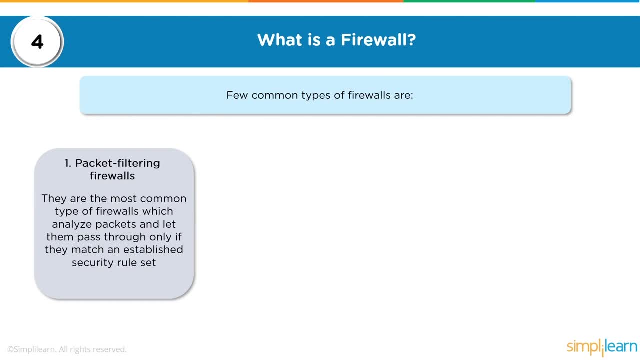 of deep packet inspection, or DPI as it is known. If that capability comes into the picture, you are basically looking at an intrusion detection system, or intrusion prevention system, in today's world called as a next-gen firewall. So a packet filtering firewall essentially will only analyze data packets for its source. 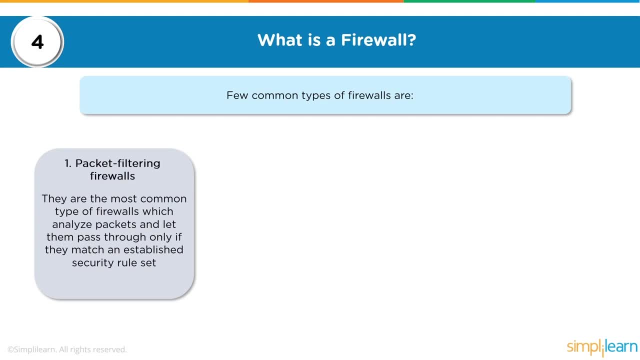 and destination, IP addresses, port numbers and the protocol that is being utilized. It will then map that information to the rules that are there on the firewall And, based on those rules, it will either allow that connection to happen or disallow that connection. 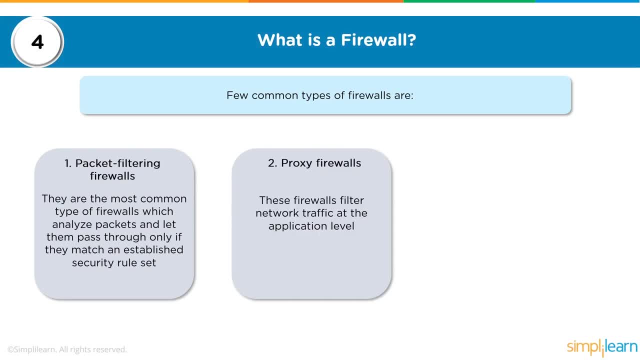 from happening. The second type is a proxy firewall. These firewalls filter network traffic at the application level. So when you say application level, they work at the layer 7 of the OSI model Packet filtering firewalls. since we have mentioned, 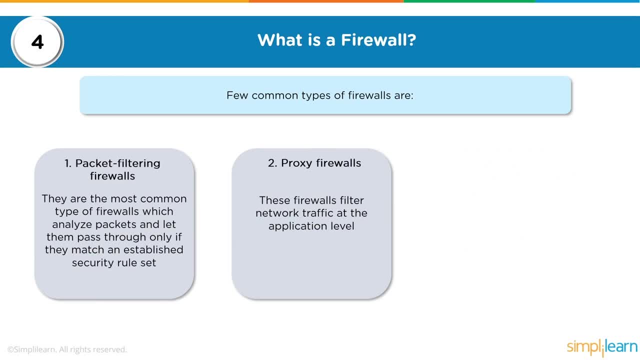 that they work on IP addressing and port numbers will work on the network layer of the OSI model, also on the transport layer, because you also look at protocols. Proxy firewalls will work at layer 7, which is the application layer of the OSI model. 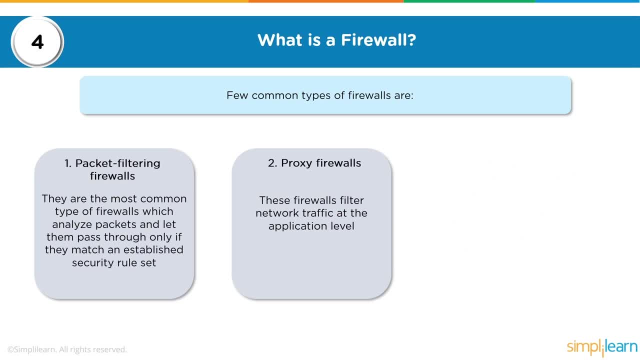 and will deal with application level protocols such as HTTP, HTTPS, FTP, SMTP and so on and so forth. And the third one is a stateful multilayer inspection firewall. These filter packets are the network, transport and application layers. 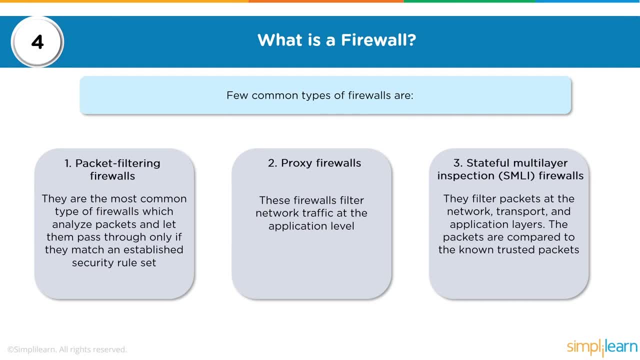 So they basically do the job of the first and the second type of firewalls. The packets are compared to known trusted packets. but now the first question is: if there is a stateful multilayer inspection firewall, why do we have type 1 and type 2 firewalls? 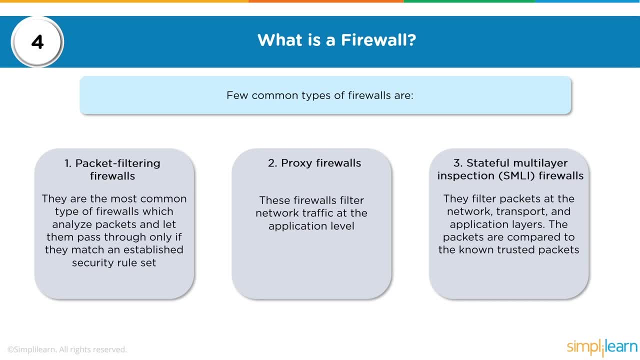 like packet filtering and proxy firewalls. That is because that is how the firewalls have evolved. We started off with the packet filtering, then we added functionality to it, and so on and so forth. So if a question comes, what is a firewall? 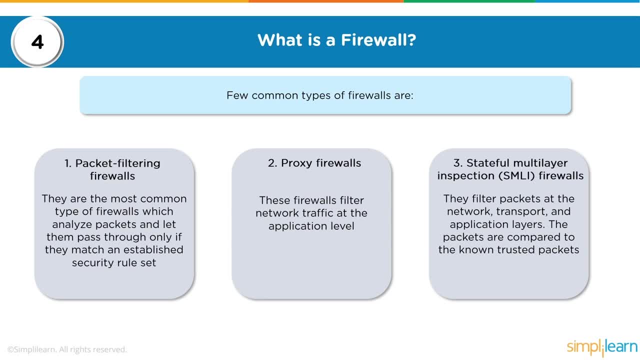 You start off with the option saying it is a hardware or software. This is the responsibility. the functionality of a firewall is to allow good traffic and disallow bad traffic, based on the rules that have been configured on the firewall, And then you've got basically three types of firewalls. 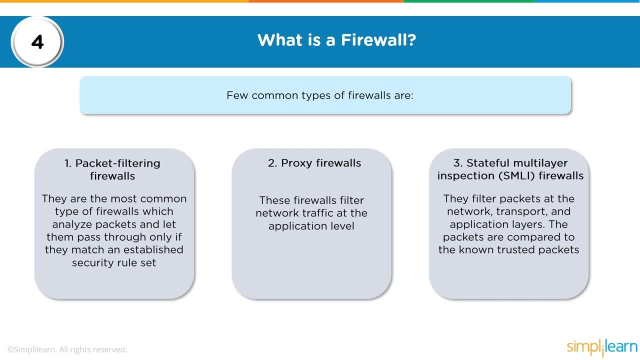 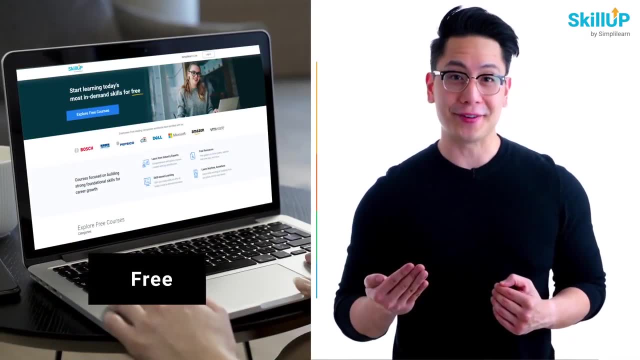 packet filtering, proxy and stateful multilayer, and just include a brief description of each of these firewalls. If getting your learning started is half the battle, what if you could do that for free? Visit SkillUp by SimplyLearn. 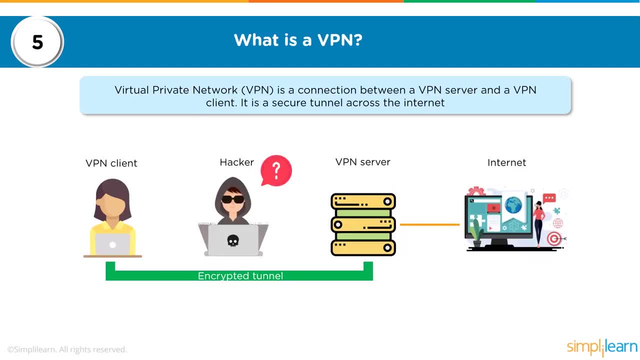 Click on the link in the description to know more. Then, moving on to question number five, what is a VPN? VPN is also called a virtual private network. It is a connection between a VPN server and a VPN client, So it basically creates an encrypted tunnel. 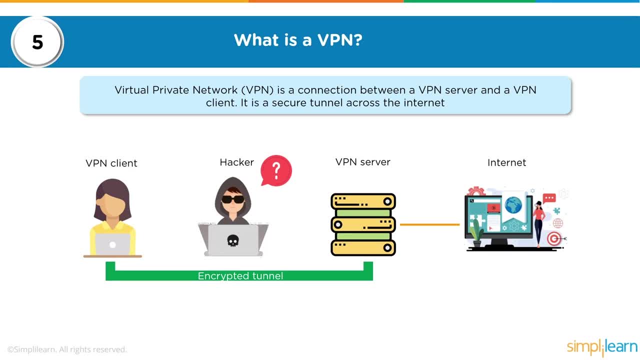 between the client and the VPN server, which is then utilized to secure the connections that you're making with the internet. So, as you can see in the diagram, the user has a VPN client installed on their machine. The VPN client then creates an encrypted tunnel. 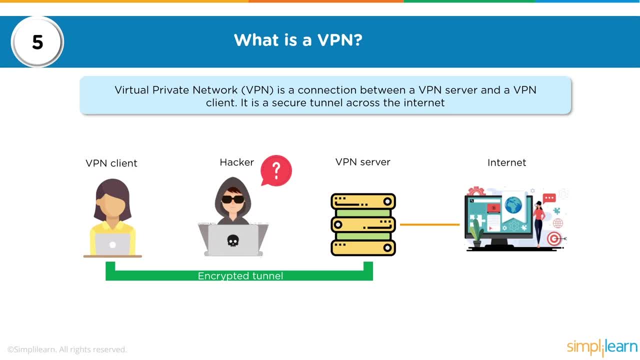 to the VPN server and through this tunnel, encrypted data is transmitted which can then be processed by the VPN server. sent to the internet, Information can be received back by the VPN server. The VPN server will encrypt that data back and send it back to the user. 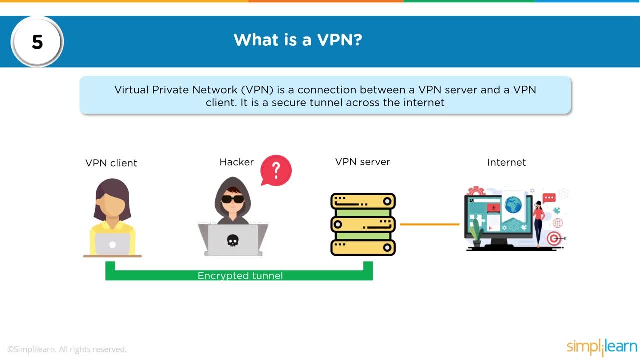 So if there's a man-in-the-middle attack that is happening or a hacker trying to eavesdrop on the communication mechanism, they will not be able to do so because of the encrypted tunnel. It is very difficult to decrypt this or hack through this encrypted tunnel. 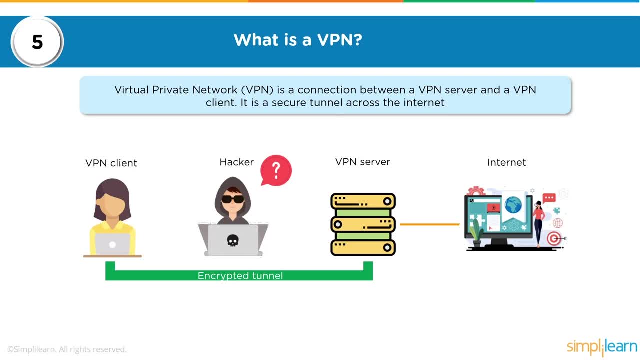 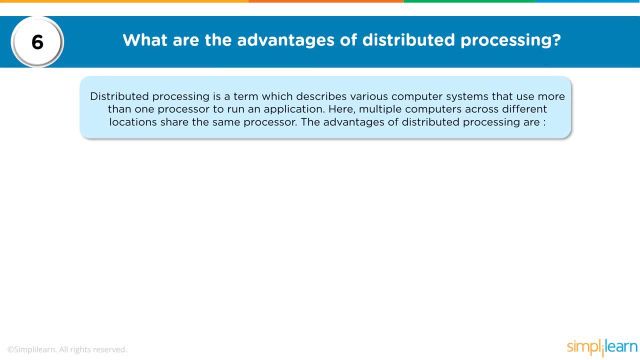 It is possible, but it is very difficult to achieve that. Moving on to question number six: what are the advantages of distributed processes? Now, before we go into advantages of distributed processing, we first have to understand what is distributed processing. So it is a term which describes various computer systems. 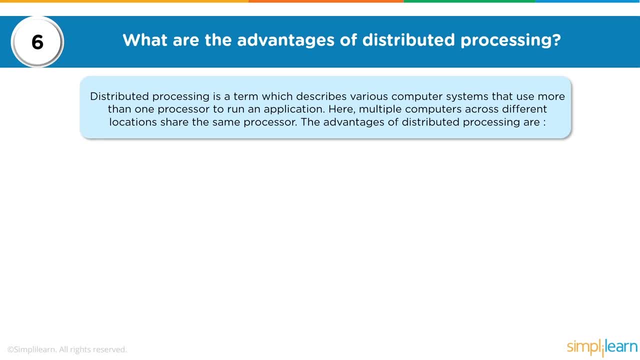 that use more than one processor to run an application. Here multiple computers across different locations share the same processor. The advantages of distributing processes are as follows. But before we go into the advantages, distributed computing is basically where multiple machines will pool their resources together. 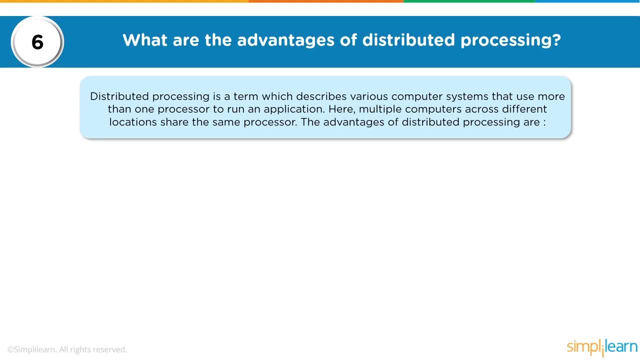 to run an application, To run a singular application, So an application that has multiple resources and can scale up and scale down as and when required. The advantages are that it can be very useful in data recovery, For example RAID, where you are striping data on various hard disks. 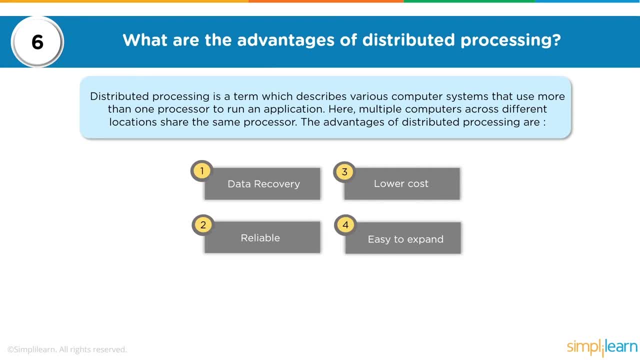 It is reliable, It is cheaper, Lower cost can be achieved And it is easy to expand because of the scalability factor that we just talked about. If there is loss of data in one computer, it can then be recovered by another interconnected computer. 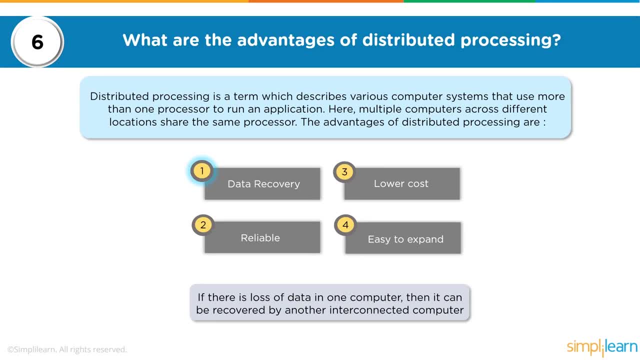 And one of the examples would be blockchain. in today's world, What is blockchain? That this data is created live and stored on a connection of computers, So if one of the computers goes offline, the other computers in that network will still have that data. 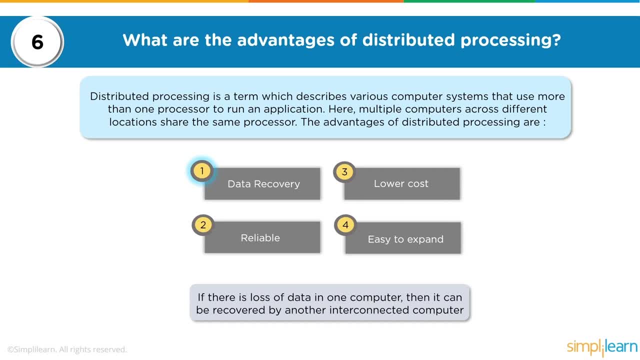 and the blockchain will still function without any issues. The second point: a glitch in one machine does not affect the processing, as there will be multiple other machines. like we discussed in the blockchain, Several cost-effective mini computers are used instead of costly or mainframe machines. 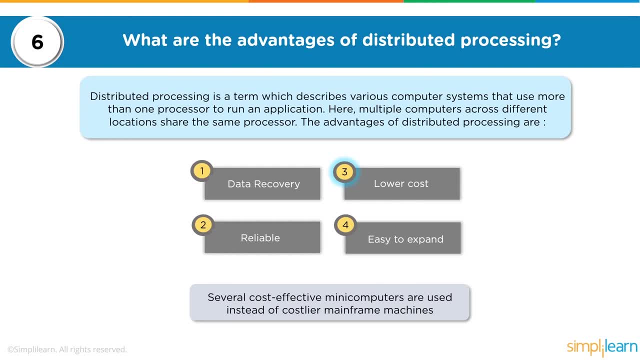 So, instead of having a server bank, I can have multiple machines interconnected together and they can function in that particular blockchain or for that particular distributed processing mechanism. Depending on the amount of data processing, more computers can be attached to the network. Thus you can increase the number of computers. 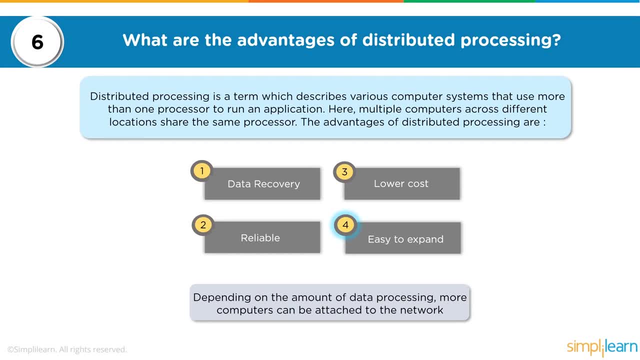 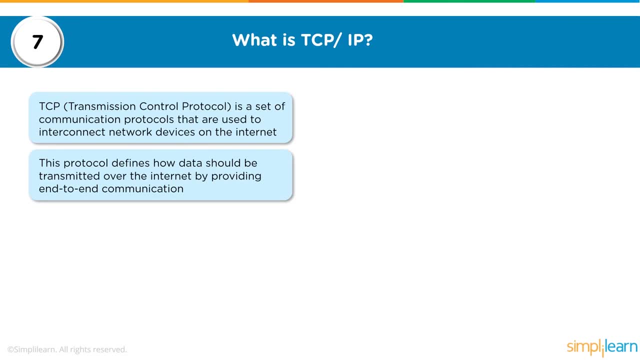 that can be a part of that blockchain, or you can reduce them as and when necessary. Moving on to question number seven, What is blockchain? TCP, IP? TCP, IP, or transmission control protocol over internet protocol, is a set of communication protocols that are used to interconnect networking devices. 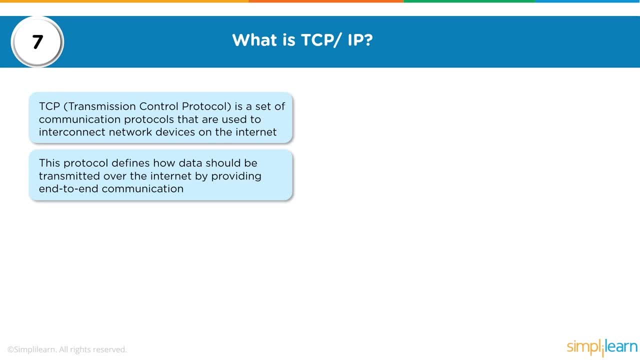 on the internet. This protocol defines how data should be transmitted over the internet by providing end-to-end communications. So, essentially, if you want networking to be established on your machine, you will need TCP IP. Without TCP IP, there will be no work groups. 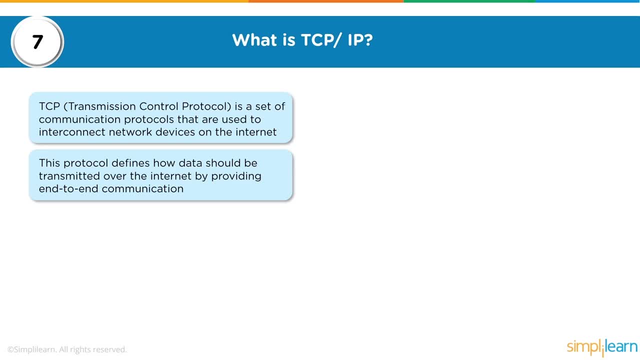 there will be no domains. Basically, your interconnectivity will go for a toss. TCP IP is a software that, once installed on your machine, will then interact with the hardware, which is your network interface cards, and then your switches, wires, cables and all those. 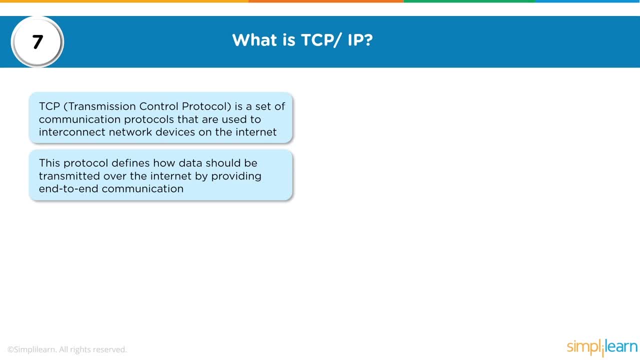 through protocols that have been already pre-configured in it. So, within the TCP IP suite of softwares, you will have all the protocols, all the functionality of the OSI layer, and each and every protocol that works on each and every layer will be predefined and pre-configured. 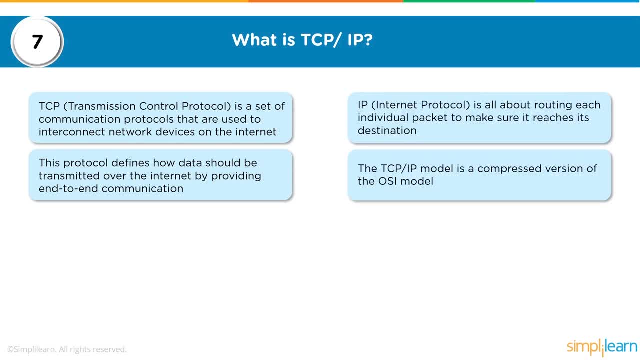 to work in a particular manner. The internet protocol is all about routing each individual packet to make sure it reaches its destination. So with the TCP, you are talking about the protocols that will allow you to format the data and generate it so that you can communicate it over the network. 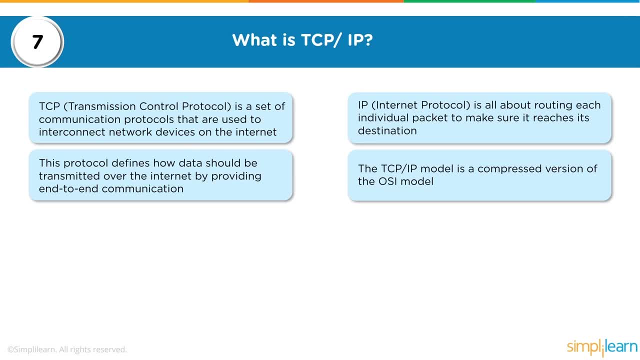 The IP will then deal with the routing of those packets, so that the packet can be routed to the correct computer and be received by the recipient. So the TCP IP model is the compressed version of the OSI model. The seven layers will get converted into four layers. 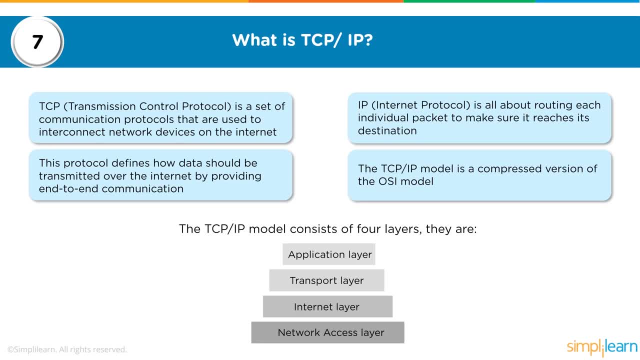 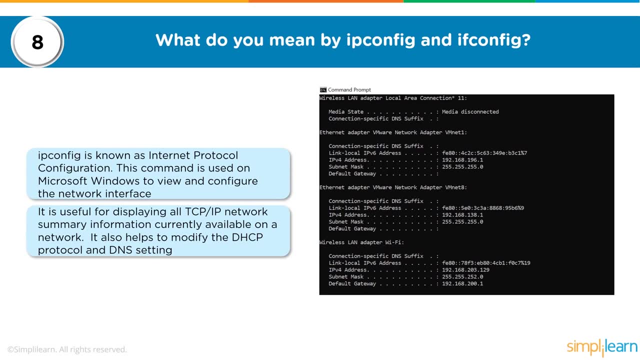 The network access layer, internet layer, transport layer and application layer. Moving on to question eight, What do you mean by IP config and IF config? Both of these are commands, The first one on a Windows machine, the second one on a Linux machine. 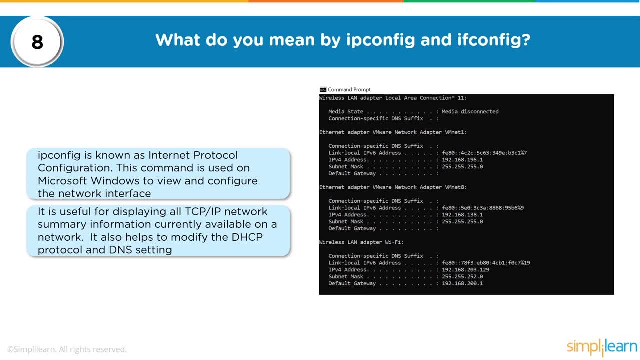 So IP config is known as the internet protocol configuration. This is a command that is used on the command line interface of Microsoft Windows to view all the adapters and the configuration of each and every adapters for their network interfaces. So, as you can see on the right hand side in the command prompt screen, 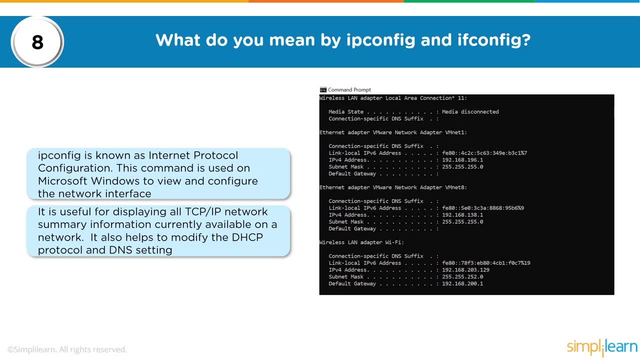 if once you type in the IP config command on the C prompt and press enter, it will give you a list of all the adapters that are there, So you can see wireless LAN adapter- local area connection. the media is disconnected. it doesn't exist. 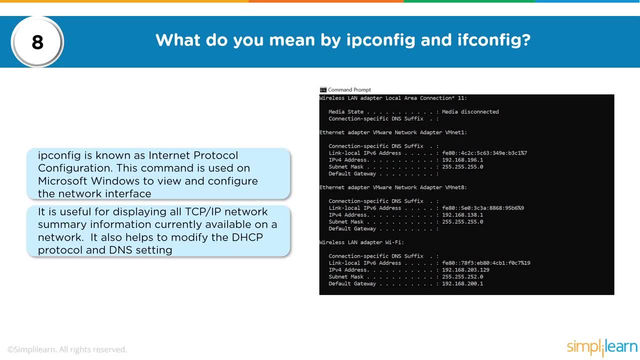 At the bottom you will see the Wi-Fi connection wireless LAN adapter and it can give you the IP version 6 IP address, IP version 4 address, the subnet mask and the default gateway. So this is the configuration that allows the machine. 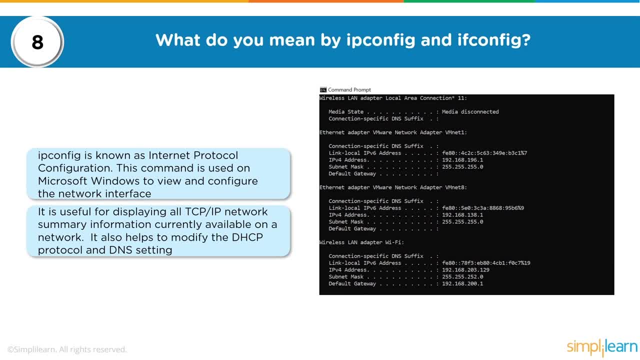 to know on what network it is on, what is the default gateway for communicating to the internet, what is the subnet mask, so how many computers may exist in that particular network, and what is the IP address of that specific computer, so that it can communicate across the network as well. 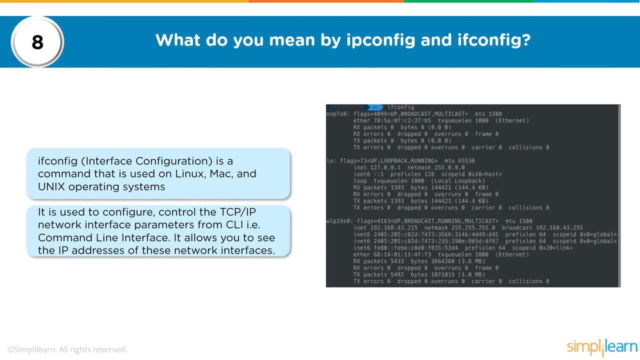 IFConfig is the same thing on the Linux, Mac or Unix operating system, So the command will also give you the list of interfaces and the configuration of each and every interface. It is used to configure, control the TCP IP network interface. 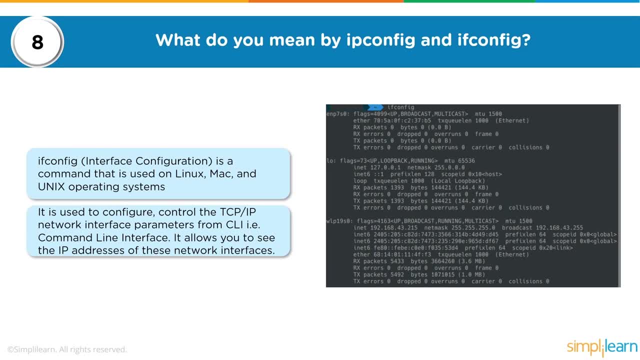 interface parameters from the command line interface. It allows you to see the IP address of these network interfaces. So here you can see the WLP 19 S, the IP address being 192.168.43.215,, subnet mask being 255.255.255.0,. 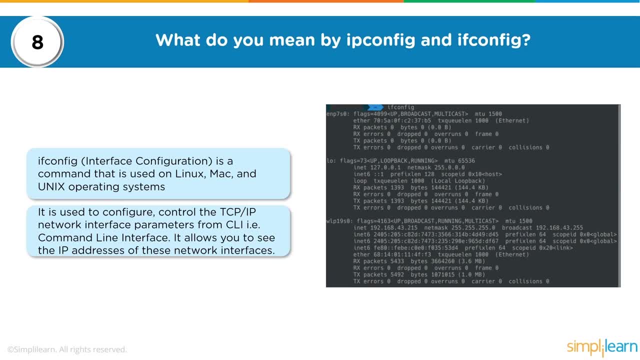 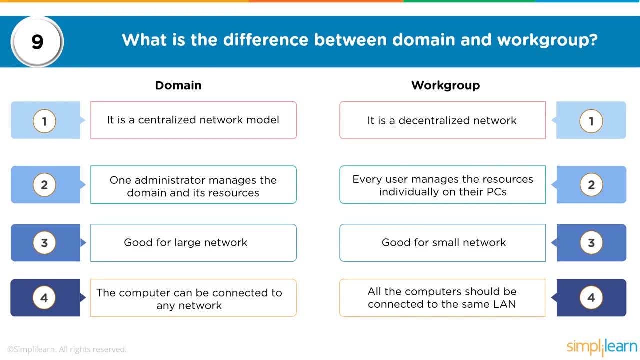 with the broadcast being 192.168.43.255.. Question 9.. What is the difference between a domain and a workgroup? This can be a very interesting question And can be a very lengthy question at the same time. A workgroup is nothing but a decentralized network. 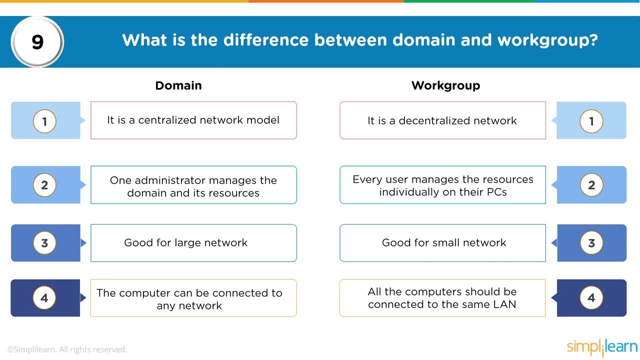 where you have interconnected multiple machines together and each machine acts in its own individual capacity, thinks of itself as a server right. So a decentralized network. every user manages the resources individually on their PC. So local users on their own PCs. 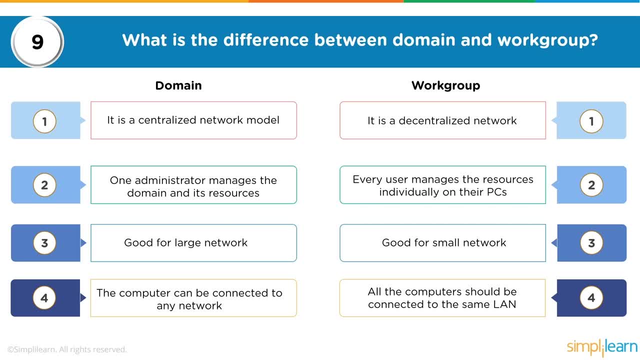 managing the network shares what can be shared from that particular machine, what data should be shared, should not be shared, to whom it can be shared with, and so on, so forth. It is good if you've got a small network. 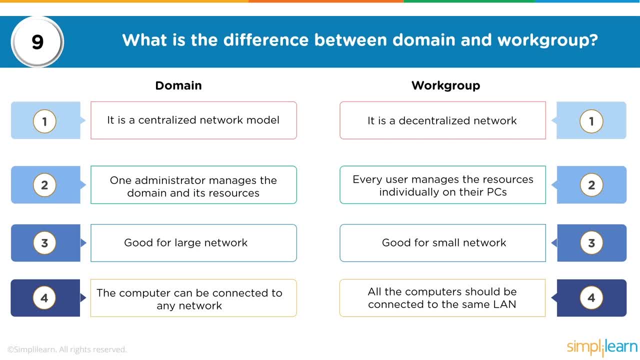 a few machines altogether and you want them to interact with minimal management effort, right? So each computer, each user will decide what they want to allow other users to see on that particular network, And all of them would be connected over a LAN. 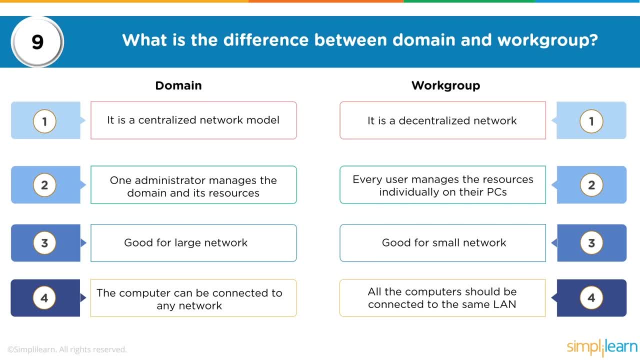 a local area network, either a wireless or a wired one. So if you look at your home Wi-Fi right now, that is one of the best examples of having a workgroup. The domain, on the other hand, is a centralized network model. 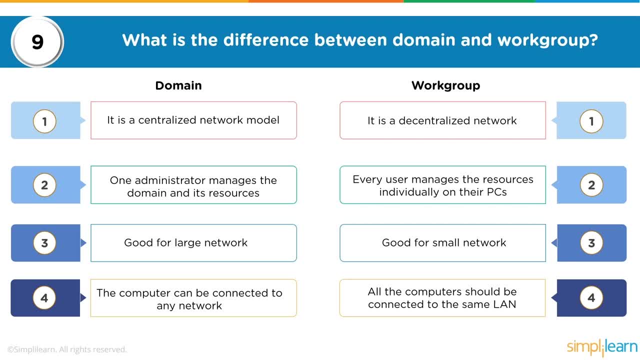 So, in a corporate environment, whenever you go there and you've got a domain-based username and password which, when entered onto a particular machine, gives you access to the entire network or whatever applications and whatever resources have been allocated to you, that is where the domain comes in. 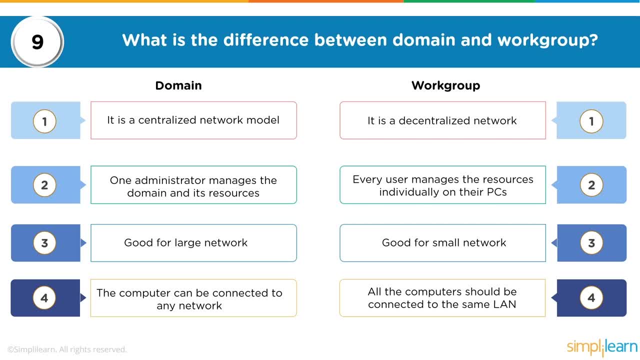 So it also uses a single sign-on mechanism for all the resources that are to be made available to you, Whereas in a workgroup your local user is only meant for that particular computer right. So, coming back to the domain, it is an administrator who's going to manage the entire domain. 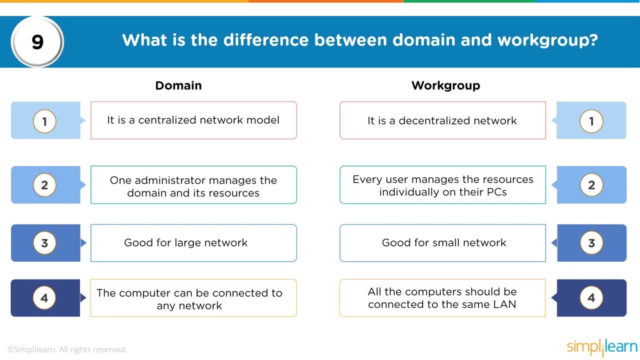 and all of the resources connected to the domain. The resources could be switches, routers, servers, data stores, applications, web servers, mail exchange servers and so on so forth. So all of these are administered by an administrator through the domain. 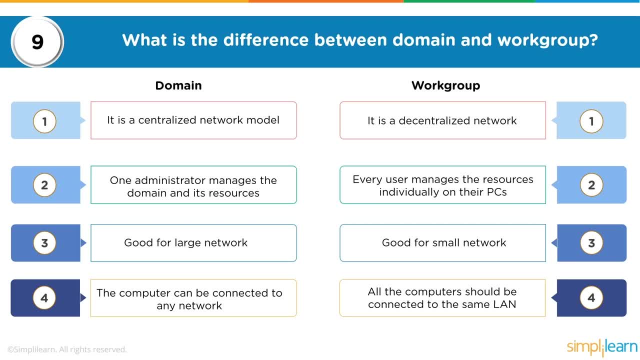 It is the most reliable and optimum solution for a large network where multiple users are going to be able to interconnect and share that data amongst each other. right, The computer can be connected to any network. that means you can be on the internet and through the internet using a VPN. 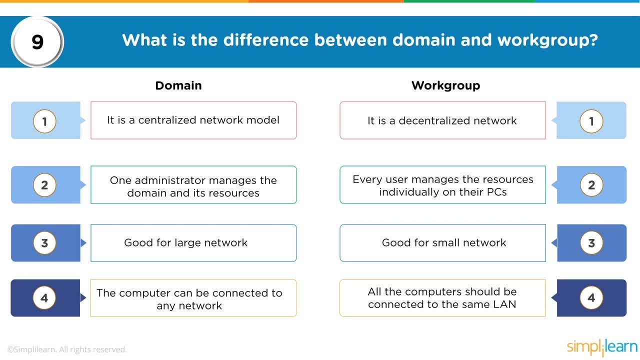 you can connect to your corporate network, authenticate in and get access to whatever resources you are allowed to access, Whereas in a workgroup you have to be a part of that network to access that particular network. If you change your location, you go and connect to another Wi-Fi. 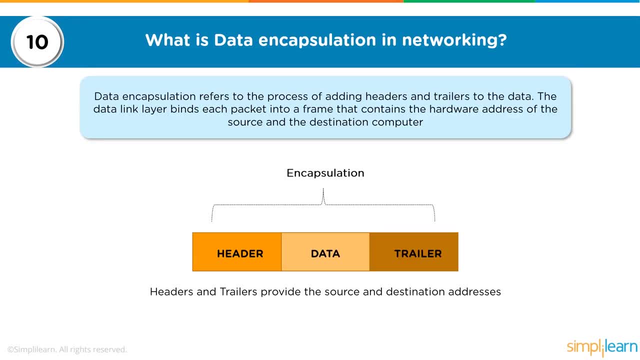 you will lose access to your previous Wi-Fi. Then the last question for the networking section is: what is data encapsulation? in networking, Data encapsulation refers to the process of adding headers and trailers to the data. The data link layer binds each packet into a frame. 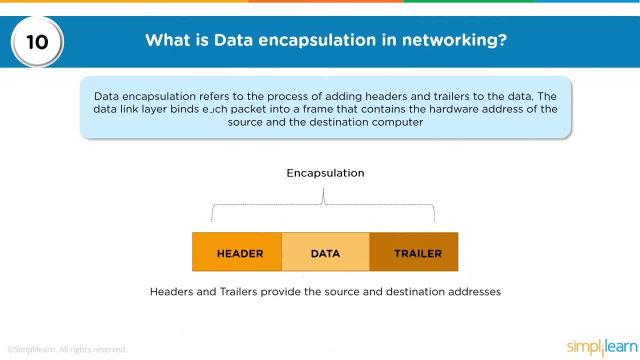 that contains the hardware address of the source and the destination computer. So in this example, when you are talking about data encapsulation, we have talked about how data that has been created by the application layer would have a header and a trailer that will give the various information. 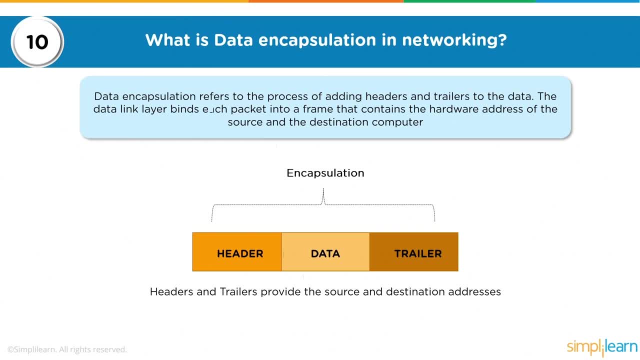 of where that data needs to be sent. So the hardware address, which is the MAC address, comes into the picture and gets added to the header, And the IP addresses, port numbers and all of those things would then be added to this trailer as well. 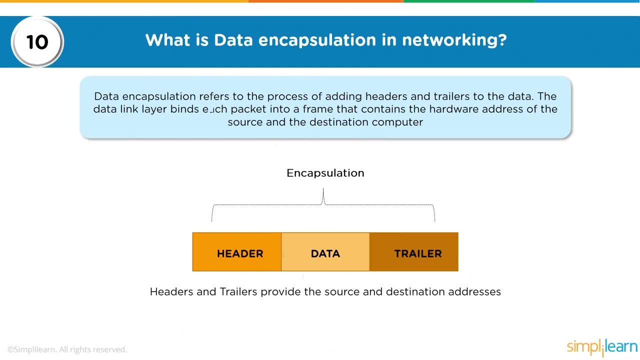 so that the data can be then routed to the intended recipient of that particular communication. With this we end the first 10 questions in networking, And in this video we are going to look at software and programming. So we are going to look at the first 10 questions. 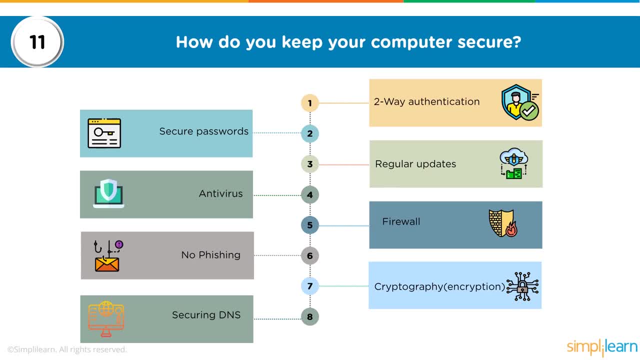 First question being: how do you keep a computer secure? Now, this is going to be a very generic question, So you want to put your best foot forward and you want to identify the most common methodologies on how you can keep a computer secure. 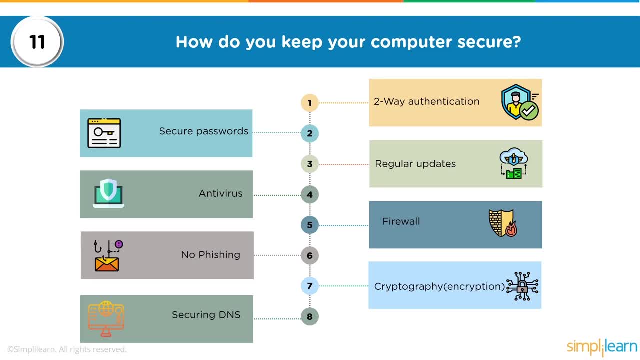 So, when you talk about computers, the first thing that you want to talk about is authentication mechanisms, where you want multi-factor authentication or two-way authentication to ensure that your accounts are kept secure. Now, if you look at using passwords- depending on how passwords are being used- 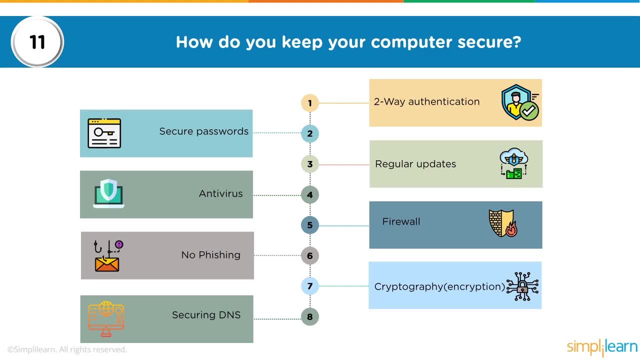 how they are being stored by the application. password attacks can be possible: either a brute force attack or a dictionary-based attack, or even password guessing attacks are possible. To mitigate those kind of attacks, we need multi-factor authentication to ensure that accounts are kept secure. 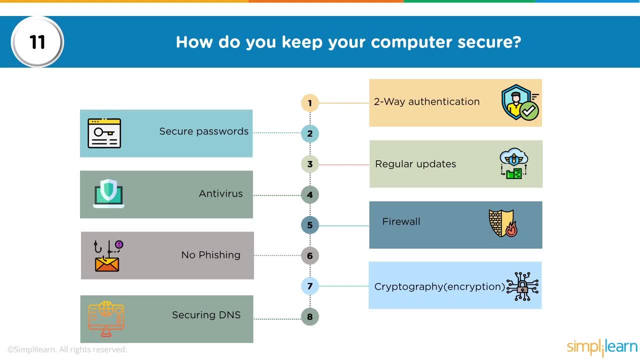 Now, even if we are using multi-factor authentication, we also want to look at secure passwords, which means that the password is complex enough to understand most of the common attacks and a brute force attack or a dictionary attack is just not possible. So we want to randomize our passwords. 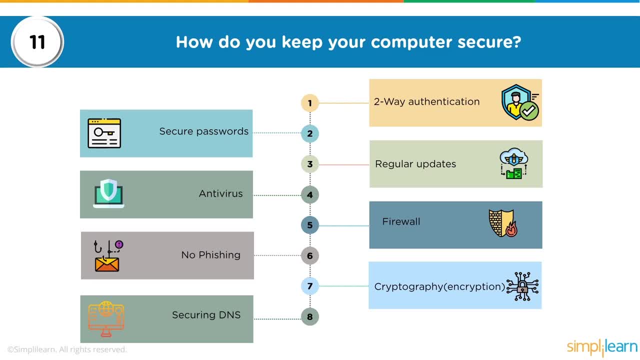 We want to create a complexity where a password meets standards such as has at least one lowercase, one uppercase character, has numerics and special characters and is randomized, is not based on a dictionary word, doesn't contain usernames, email addresses, phone numbers. 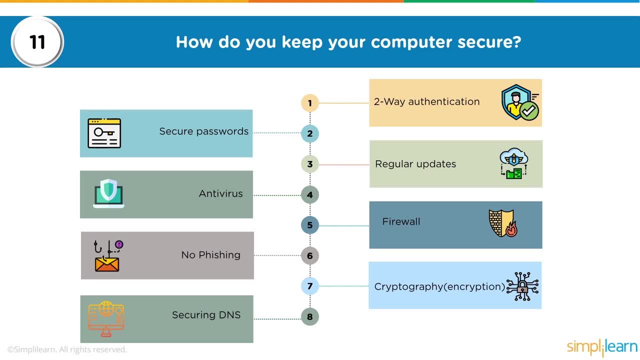 or anything that is personal to that particular user. Third, keep regular updates, which means that there will be patches that will be released for the application, for the software that you are utilizing. Download the patches, install them on a regular basis to ensure that you are secured. 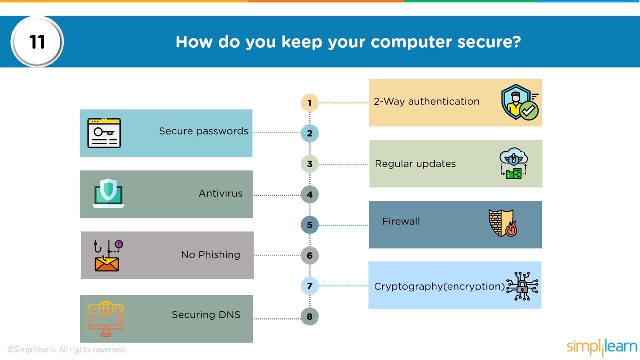 against the most recent attacks that have been identified. Install a good antivirus could be an internet security suite, which will have an antivirus, an intrusion detection system, a firewall, and will help you protect yourself against ransomwares, malwares and any script-based attacks. 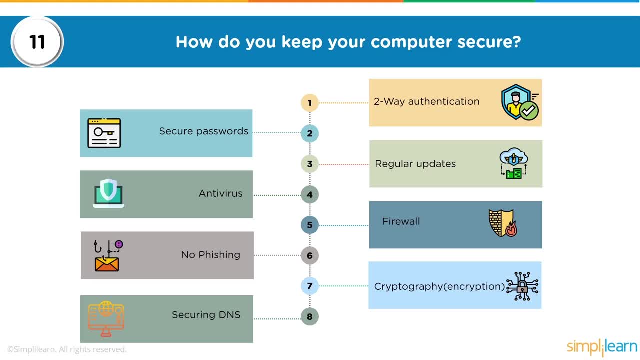 Also have a specialized firewall on your system- could be a host-based firewall or a network-based firewall- to ensure that attacks are kept at a minimum and you have your network definitions in place to allow or disallow connections from happening to your devices. Have anti-phishing software. 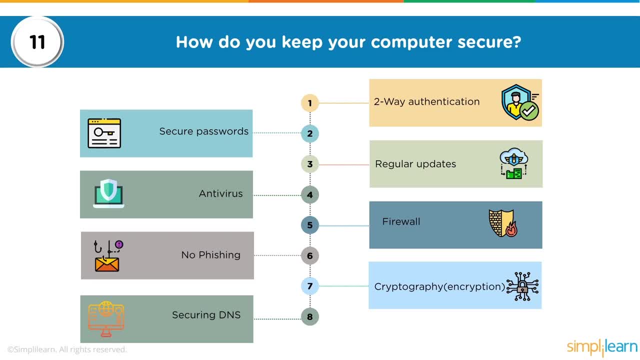 installed as well to ensure that you are not getting any spam mails. Even if you do, you are able to identify that And not fall prey or victim to those spam mails. Phishing attacks are generic where they are directed towards individuals and they prey on the gullibility. 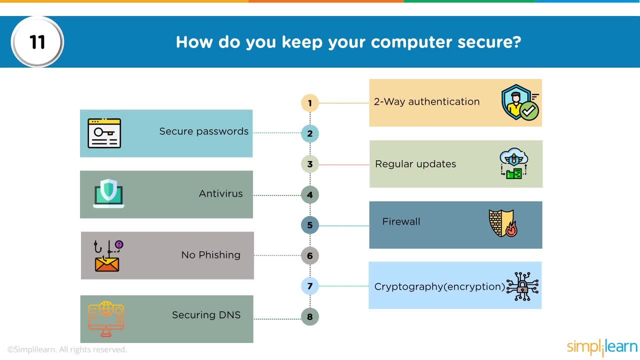 of that particular individual. So our Nigerian frauds, or the lotteries that we win on a regular basis of hundreds of million dollars, those messages, the emails that we receive, they are all phishing emails where they're basically prone to victimize the user. 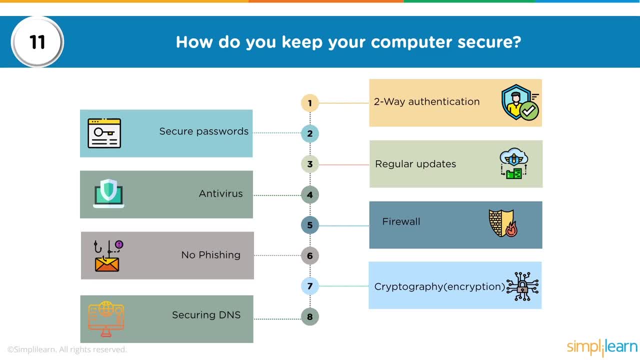 and then rob them of money or install some malware or do some other malicious activity. If you want to enhance encryption about data that you have stored on your devices or that is accessed by your software or being transmitted by your software, use encryption. Encrypt your data. 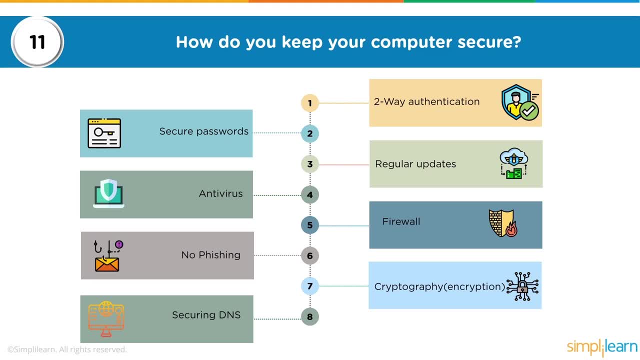 whether it is at rest, whether it is in motion or whether it is at use, thus reducing data leakage and data loss possibilities. And, finally and the foremost, secure your DNS. DNS is the domain name server, which is utilized by computers to resolve domain names to IP addresses. 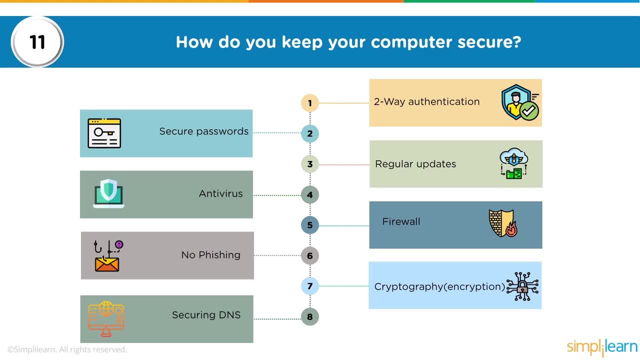 If a DNS poisoning attack is possible, where your DNS settings have been modified by an attacker and you're redirected to a malicious DNS server, that server is going to redirect you to another malicious application which may have a malware or a malicious software as a payload. 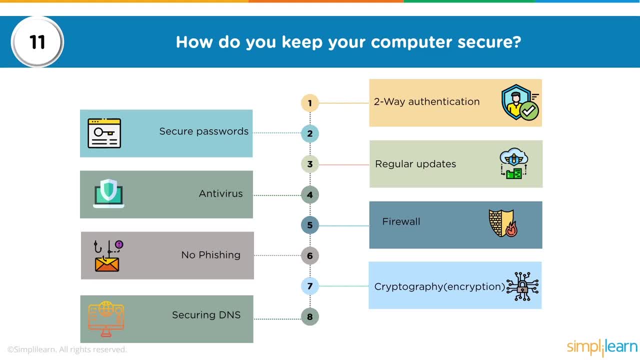 Also, you don't want people to know your DNS server because of the queries that you're making, So you want to use secure DNS or DNS over HTTPS to encrypt your DNS queries as well. So, in a nutshell, if you follow these eight steps, 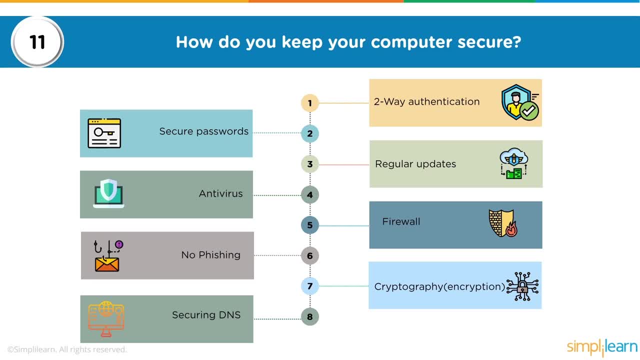 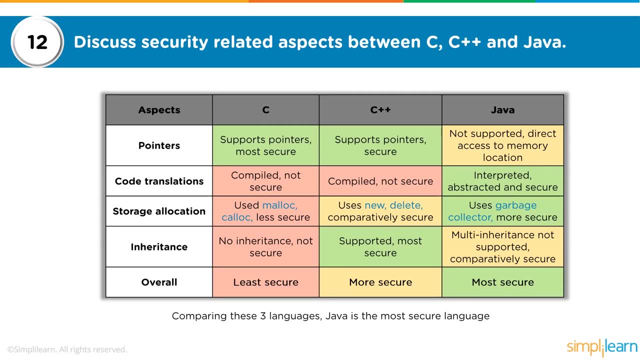 your devices, your computers, your applications are going to be as secure as possible. The next question discuss security related aspects between C, C++ and Java. Now, this is an open-ended question. It depends on which level you're giving an interview on. 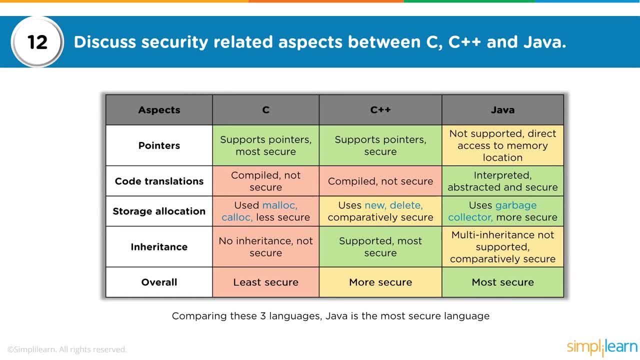 but you're looking at it from a freshers perspective or a less experienced perspective, And thus these are some of the aspects that we want to look at and the comparisons between C, C++ and Java, So the five aspects that we are looking at. 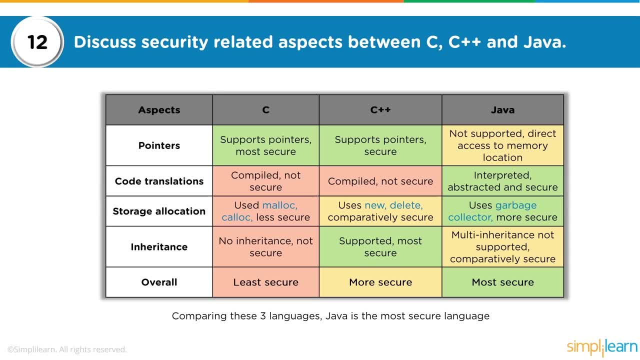 are pointers, code translations, storage, allocation, inheritance and overall security based on C, C++ and Java. So when we say pointers, we are looking at how we are going to. we are using pointers and stacks and keeps to point to functions. 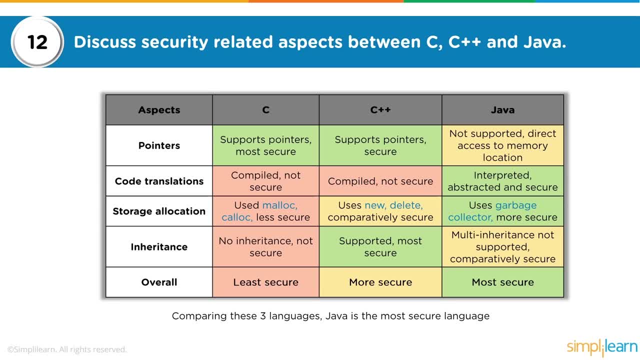 and how we exit those functions and how those functions are then recalled into the next function. So C supports pointers. it is most secure. C++ also supports pointers, but it is a little bit less secure than C Java. it is not supported. 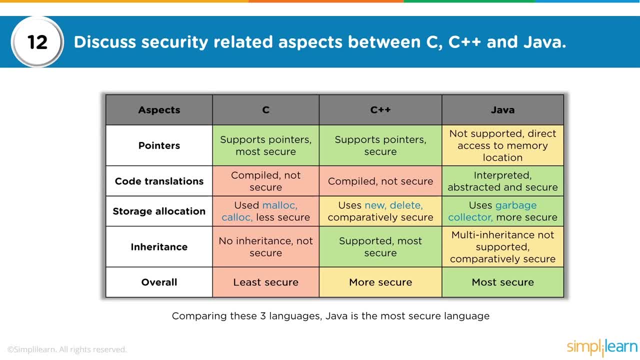 Tarot, access is given to memory allocation and thus it is the least secure. as far as pointers are concerned, When we look at code translations, C is able to compile, but it is not secure. Same with C, C++, but in Java. 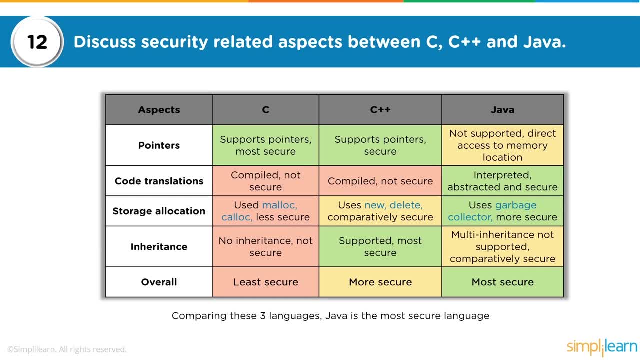 it is an interpreted language and it is abstracted and secured. In storage allocation in C we use malloc and calloc memory allocation, which is less secure because it does not have internal checks on verifying what memory is allocated and the user input that is being compiled. 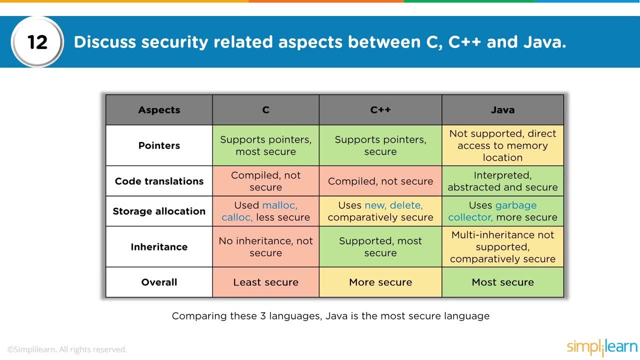 or that is being input to that memory right. Thus this can allow buffer overflow errors to creep in because of the non-verification of the input data. So it is the least secure. In C C++ it uses new and delete options. 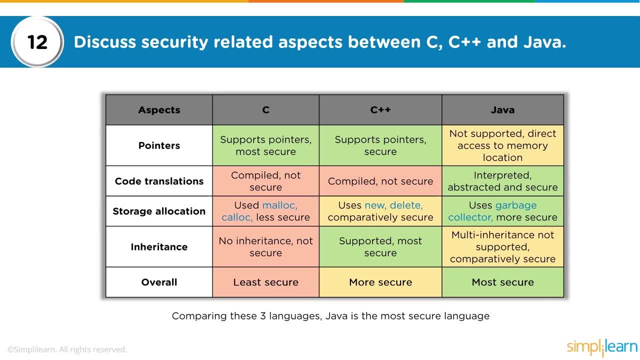 and is comparatively secure, but Java uses a garbage collector and thus is the most secure. as far as storage allocation is concerned, When we talk about inheritance, the most secure is C, C++. C has no inheritance, so it's not secure In C++. 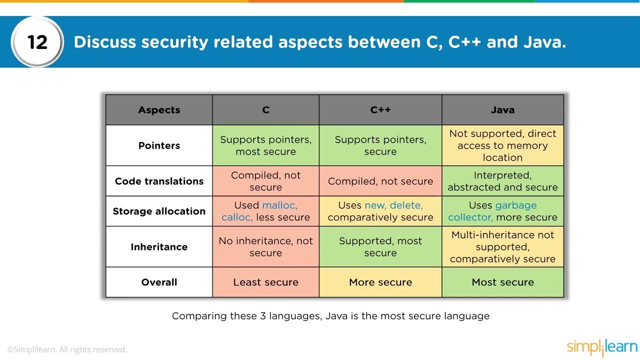 it is supported. Thus it is the most secure, Whereas in Java there is multi-inheritance that is not supported and thus is comparatively secure. Overall, the most secure out of all these, based on these five aspects, is Java. The least secure is C. 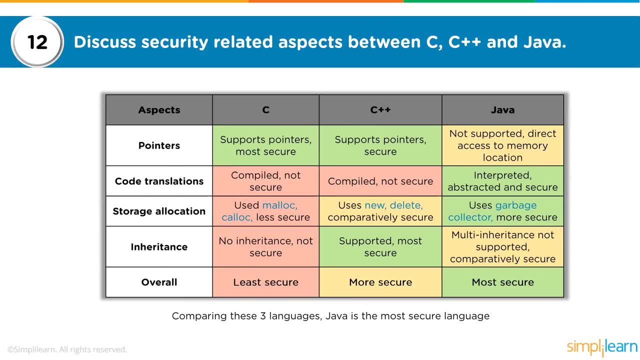 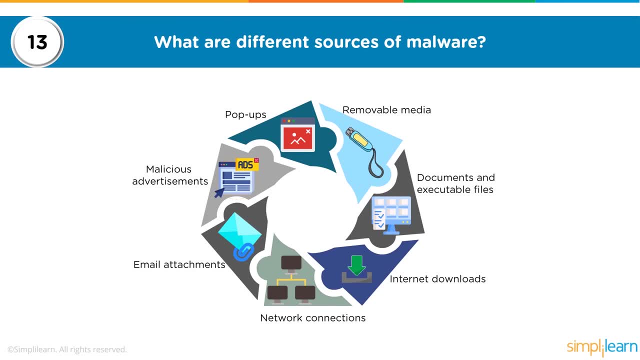 and the mid-level is C++. Moving on to question 13,, what are the different sources of malware? Now, malware stands for malicious software. Malware is basically a software that poses as a legitimate software but has a payload of a Trojan virus. 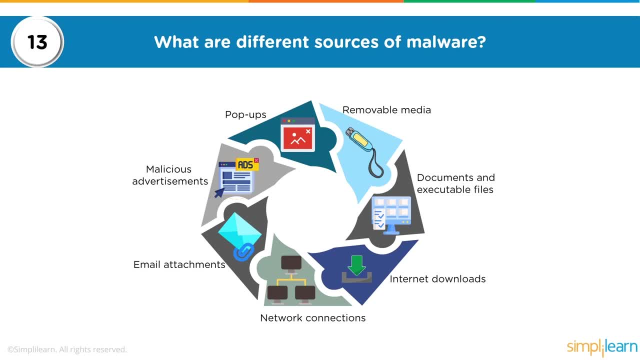 PiWare Keylogger or some malicious software that is going to have a negative impact on security of your particular device. So the question here is: what are the different sources of malware? We want to identify the most common sources through which malwares infect. 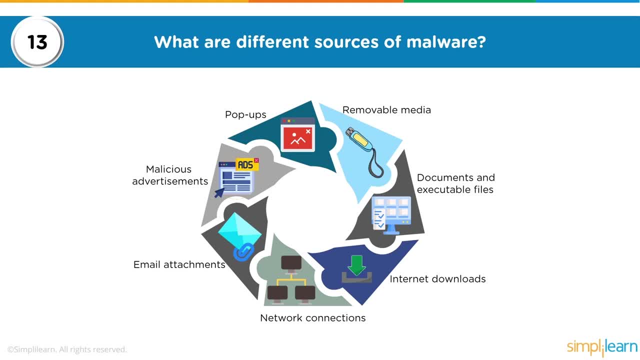 end-user devices in today's world And we can start with pop-up ads. So most of the websites, if you look at the website, if you're visiting untrusted sites, if you're being redirected to sites that you don't know about, 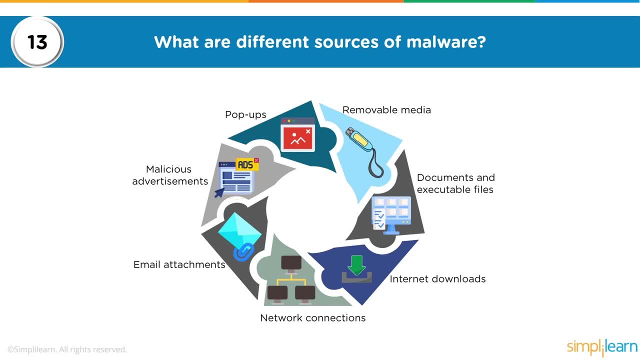 there will be a lot of pop-ups coming your way. when it says you're the one millionth visitor to this site, please click here to download your gift. Or it will say congratulations on winning a particular product for visiting this page, and so on and so forth. 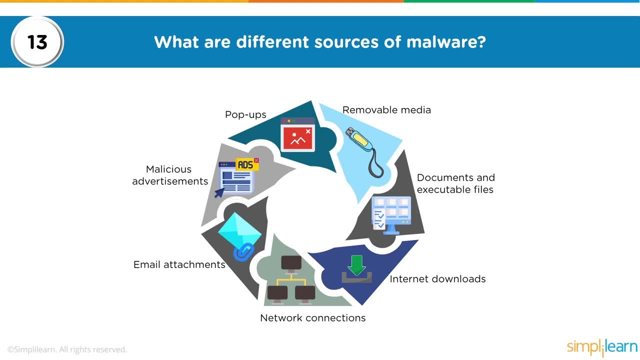 There are some instances where you can see a banner which is flashing at you on top of the page and says that there are eight infections that have been identified by the computer. click here to download an antivirus to clean the infections. So all of these pop-ups. 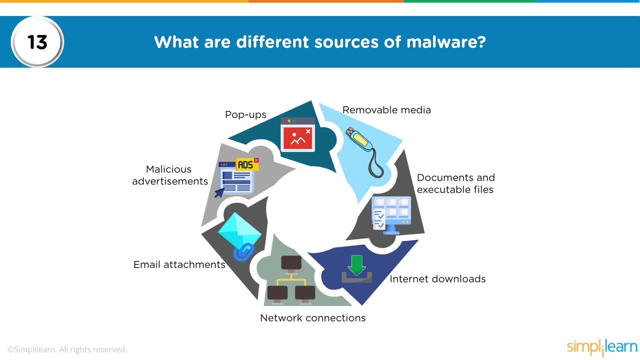 are there as a social engineering attack, as a phishing attack, to make gullible people click on those links and download those malwares. Now, the software that is posing as a security software itself can be a malicious software, which is going to install a Trojan or a virus. 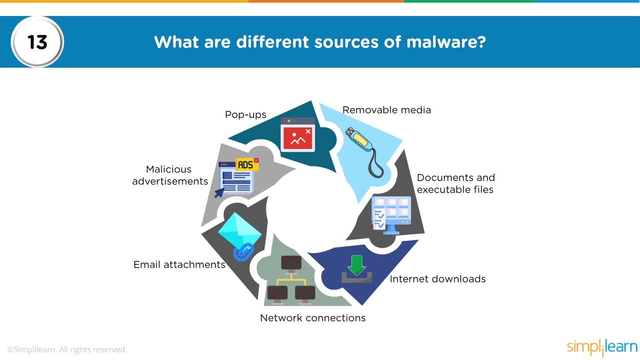 or a bot on your machine, compromising the security of that machine. The second is removable media: USBs, And humans have a fascination with USBs. So if you find a USB lying around, it's a free USB. you get excited about it. 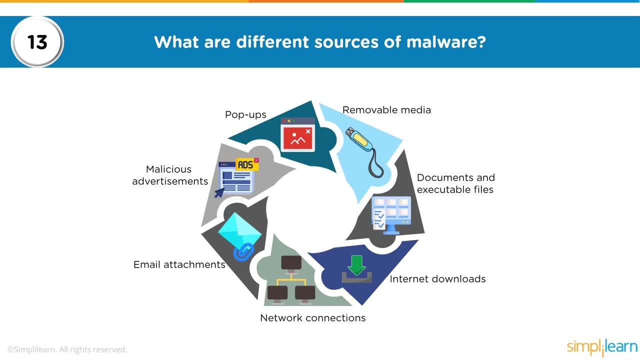 and you want to take it home. you want to plug it into a machine and see what's on the USB. Worst case scenario: you format it and you've got a free USB to utilize. The higher the capacity, the better, But that is one of the most. 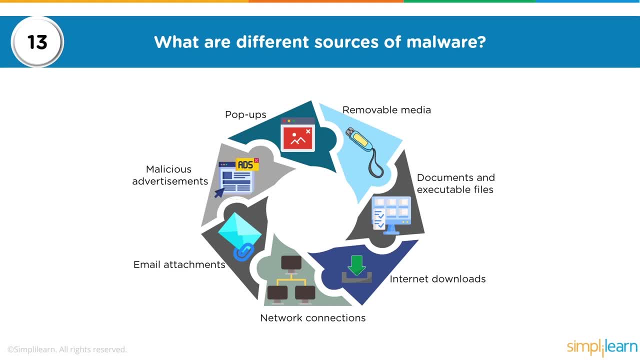 easiest way people use malwares to be deployed on unsuspecting users. If there is a USB lying around, why would somebody want to forget a USB? It's most likely planted over there as a social engineering attack so that a gullible person is going to pick it up. 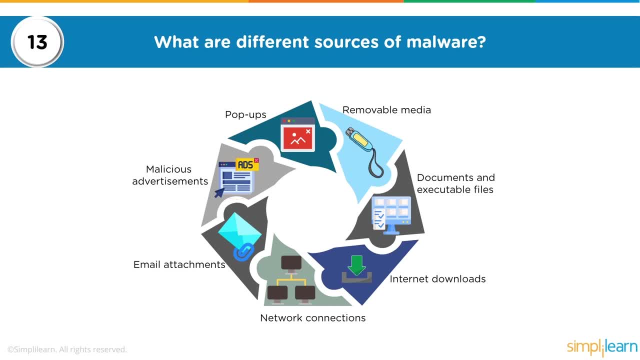 plug it into their device. If the device is not secured enough, it is going to install the malware. Then documents and executable files. This is where your viruses and all those creeps in. So let's say you're surfing on the internet. 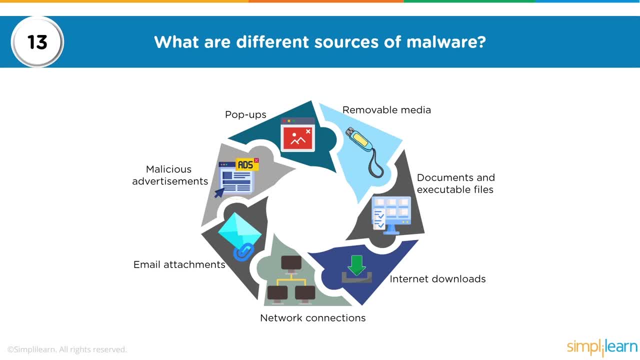 you're looking for a software and you find the software on a particular website. you do not verify the trustworthiness of that site and you just download and install that software. Now, that software could be a malware as well. Thus, if you're surfing, 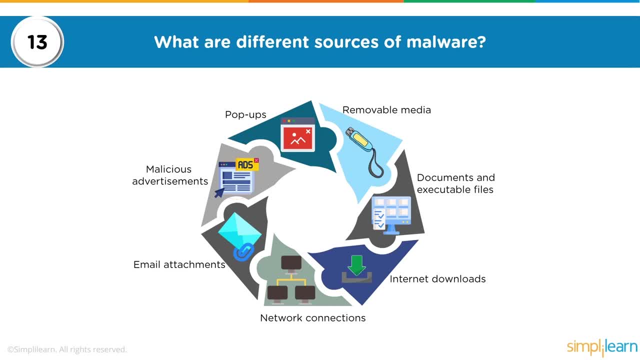 on the internet, you're downloading files from different locations. you have to research the website, you have to research the source to ensure that it is trustworthy, and only then are you going to download and execute those files. Thus, internet downloads as well. 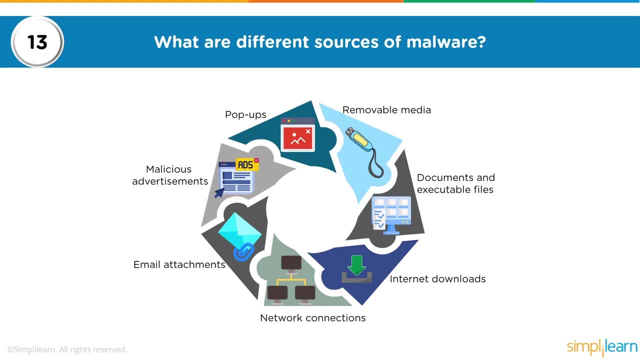 And when we say internet download, it's not just untrustworthy sites. We go to torrents, we go to the dark web or the deep web and we're searching for other softwares, especially those who are researching security right. We're always on the lookout. 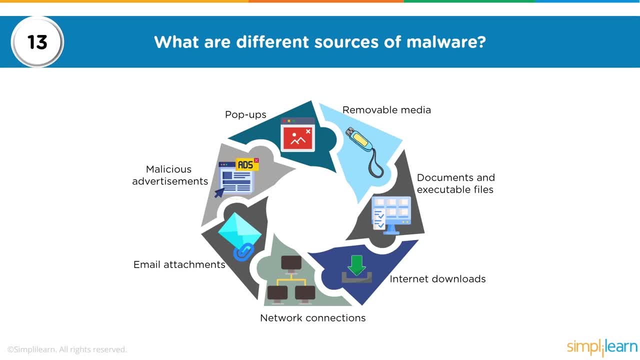 of new softwares, and we're always on those forums which may not be so much trustworthy, and we just download those files and start installing them. That is a very bad scenario, right? So you have to be very careful what you're downloading from the internet. 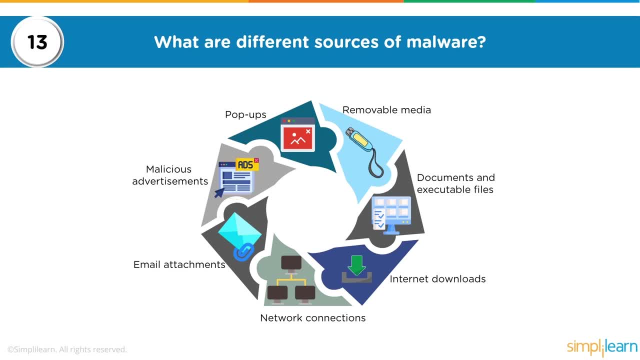 your antiviruses, your anti-phishing mechanisms, your threat intelligence mechanisms. have those mechanisms installed and you want to verify where your downloads are coming from? Then your network connections. If it is a P2P connection, it is a local area network connection. 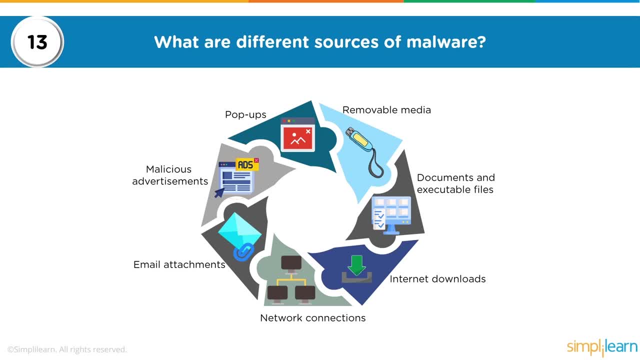 or a metropolitan area network. you have to verify which devices are connected to your machines and you have to validate those connections before you want to trust those devices and before you connect to them. If you're on a public Wi-Fi, you probably don't want to connect. 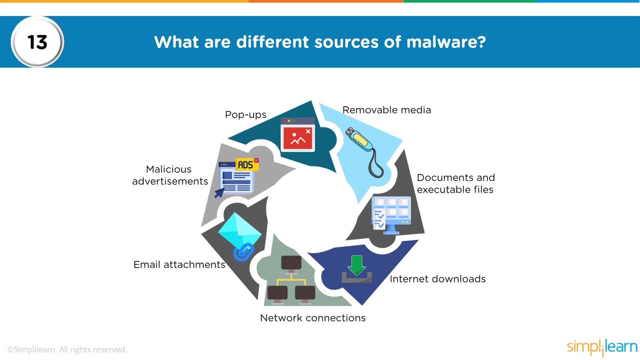 to a public Wi-Fi in the first place. Then comes email attachments. There are so many attachments that come across in today's world, most of them in a zip format or a RAR format. Some of them come as document files, where there are macros hidden within them. 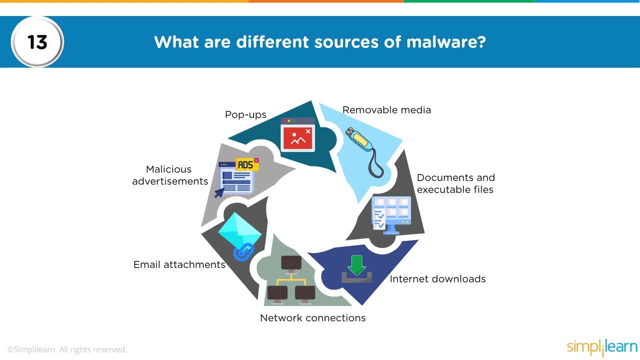 Macros are scripts that are recognized by Microsoft Office files, right. And then, finally, there are these malicious advertisements that we find online, right, Let it be Facebook, let it be WhatsApp, let it be any social media platform that you go. 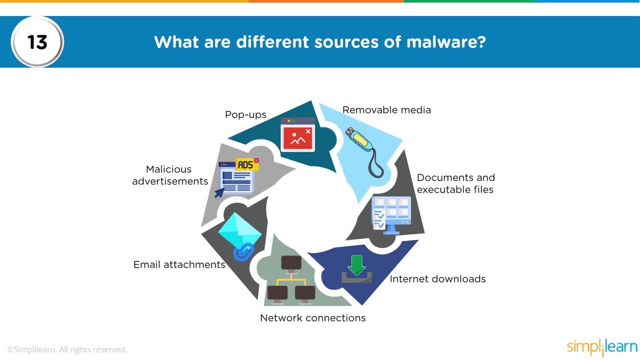 or even your search engines. Their job is to display ads. Their job is not to verify whether the ad is legit or not. It is for us, as consumers, to be careful and validate that ad and verify whether it is a genuine ad or not. 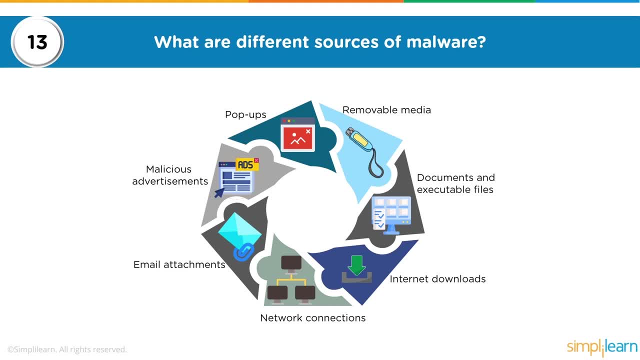 So just don't start clicking on any of the ad, trusting the platform that you're on, Be sure that you are investigating that ad. So these are the most common sources of malware And the end user will always get infected by one of these mechanisms. 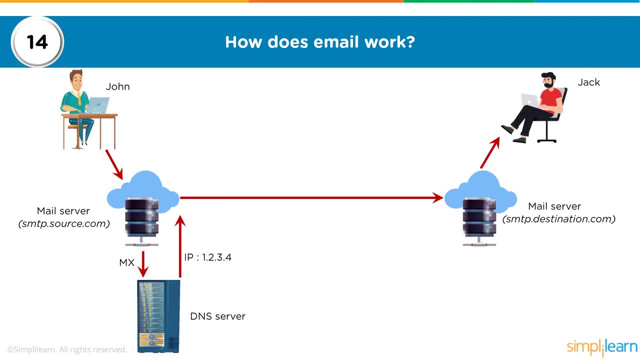 Moving on to question 14, how does email work? Now, this is a very can be a complex question, but we have to keep it as simple as possible And we have to identify that there are two servers, both of them either using SMTP. 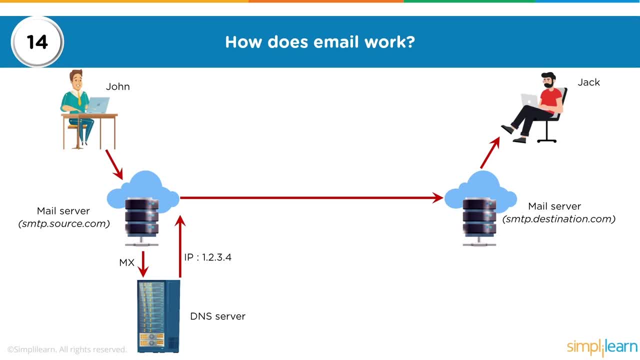 which is a simple message transfer protocol where, in this scenario, John wants to send an email. Thus, they've got an email client installed on their machine which is connected to the mail exchange server, which has a DNS server which maps the routing. 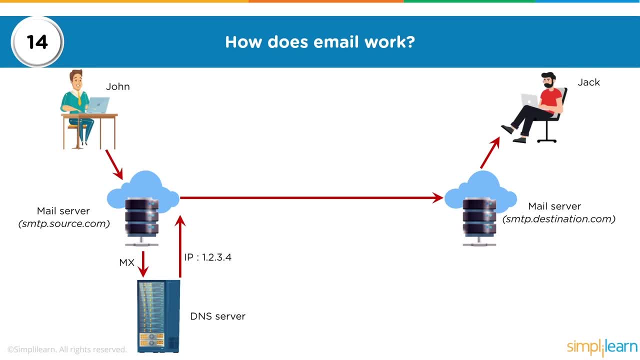 and which maps the exchange server and inboxes. So when John composes that message and clicks on send, John should be connected to a mail exchange server where the email is sent through that particular person's inbox. This inbox will then be validated and that 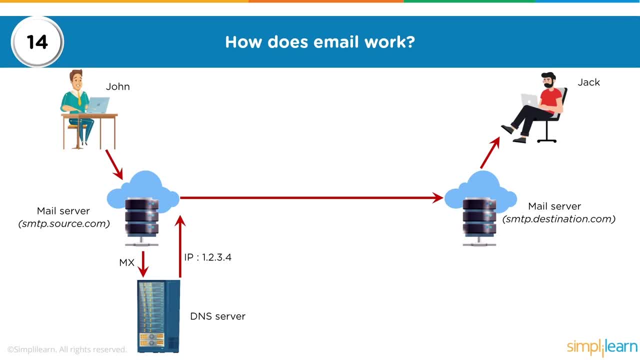 email will then be sent through the DNS server, through the internet, and will be received by the recipient mail server. So at this point in time, John also requires the recipient's email address. So in this case, this is Jack, So jack at something dot com. 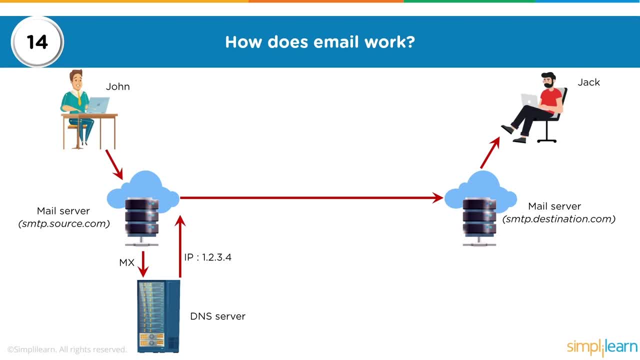 would be the email address. So while John is composing the to field will have Jack's email address, the from field will have John's email address. the subject field will have whatever they want to convey as a message. the message body will have the message itself. 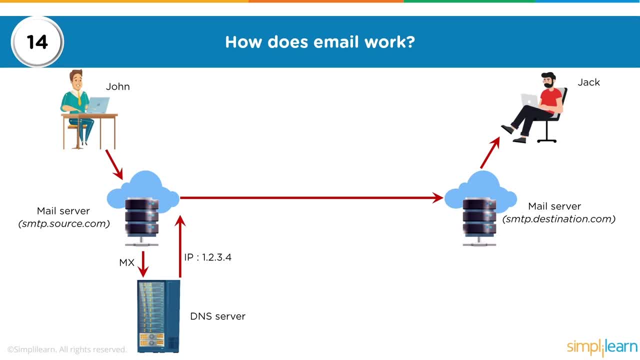 and then, when John clicks on send, it will go to their exchange server. The exchange server will then validate the inbox and identify where that inbox is located for Jack, and then, through the internet, it will be sent to the mail server of Jack. The mail server will then identify the proper. 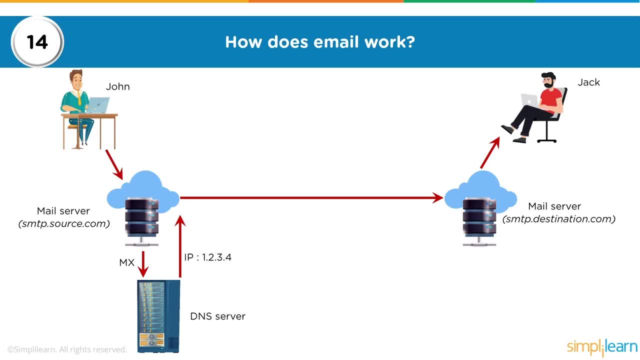 inbox that that email is to be sent to and it will store that email in that particular inbox. When Jack opens their computer and accesses their inbox, this email from John will be already waiting for them and they can respond to it the same way John had sent that email. 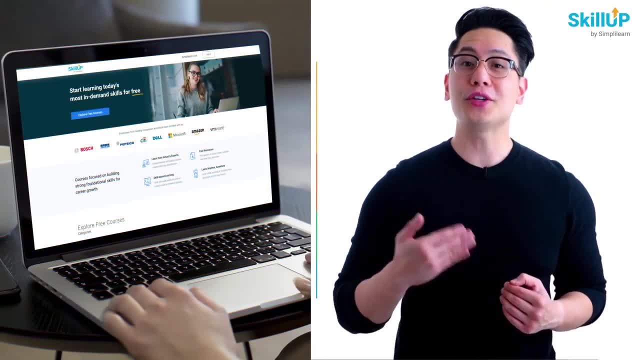 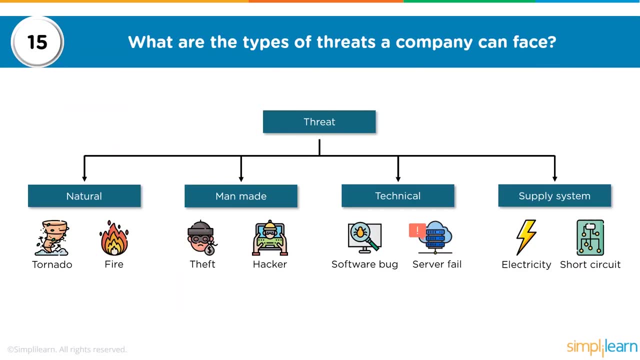 If getting your learning started is half the battle, what if you could do that for free? Visit ScaleUp by SimplyLearn. Click on the link in the description to know more. Moving on to question 15.. What are the types of threats a company can face? 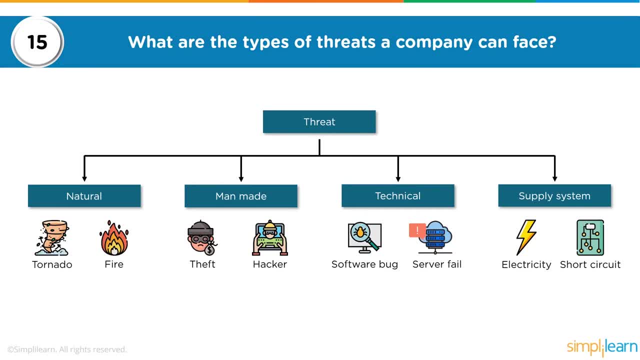 And this is where your threat modeling comes into the picture. So you're looking at softwares, you're looking at operating systems, and the company comes and asks you: what are the threats that are most likely that a company will face? So on a. 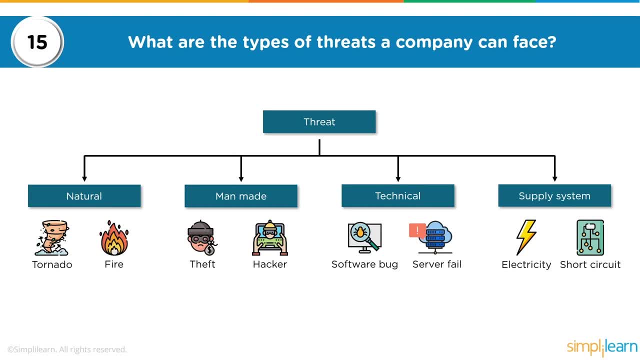 broader scale, the threats that a company will always face would be classified as natural threats, man-made threats, technical threats and a supply system threat. So a natural threat would be an act of God which is outside the control of human beings. Could be storms. 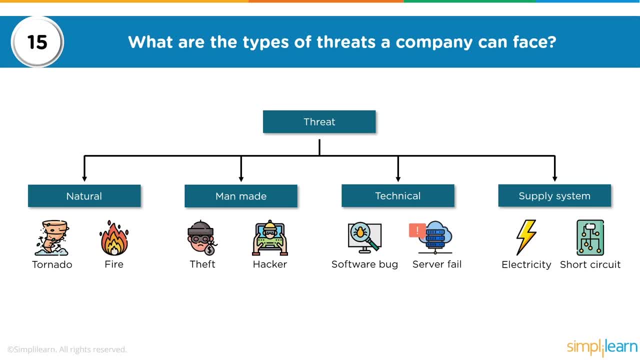 or any natural occurrences like volcanoes, thunderstorms, flooding, earthquakes, fire and so on and so forth, So anything that is natural. So it depends on the geographic location that you're in and what kind of climate that area faces, And you need to. 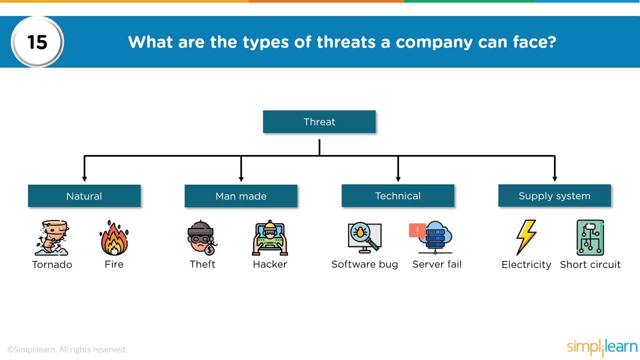 identify the immediate threats and prepare for them. So if it is flooding that you're looking at and you want to look at an office and the possibility of the office getting flooded is real, you probably want to take office at a higher floor so that the threat 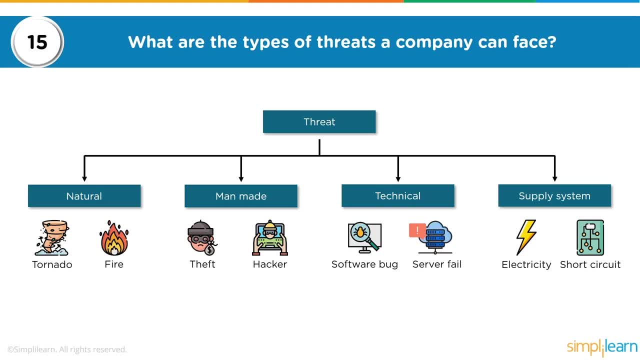 of flooding is minimized. For fire, we always have a fire drill where we practice our fire mechanism so that we can evacuate all humans as soon as possible and then worry about the technicalities of it. Under any circumstances, under any threats, humans will always have the first priority. 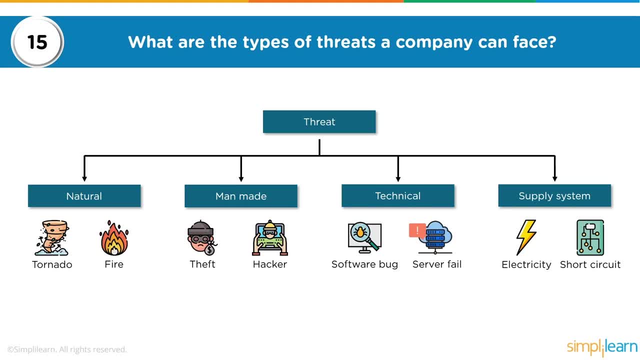 and then everything else comes in. Man-made threats are where man themselves are a problem. So strikes, lockouts, hackers, threats, theft, war, rioting, all of those are man-made threats which we ourselves cannot be in control of. but we need to plan. 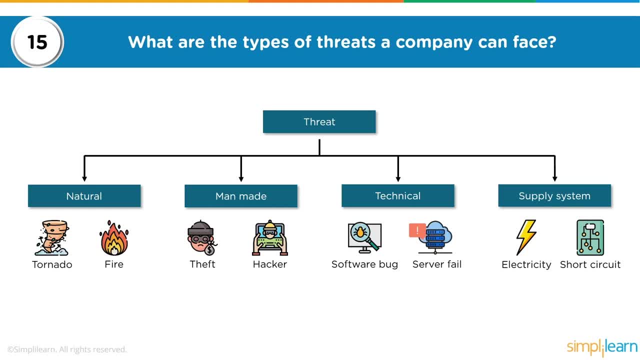 for them and we need to have a business continuity plan or a disaster recovery plan for any of these threats that have been identified. Then come the technical threats. Technical could be software bugs, operating system bugs, application bugs that come with the applications that we have, or a hardware. 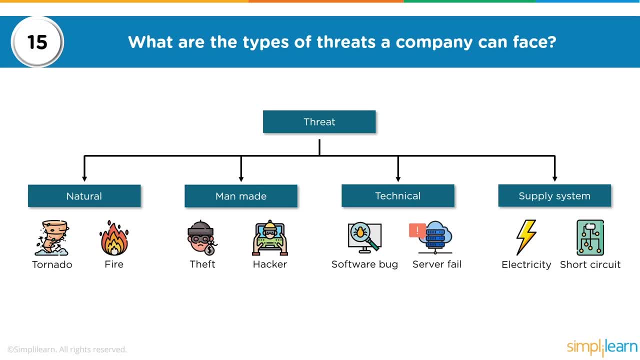 failure where a server crashes, a hard disk crashes, maybe the processor stops working, the motherboard stops working, RAM gets corrupted, any of the technical aspects stop functioning. thus creating a break in the business can come under technical, So anything to do with computers. 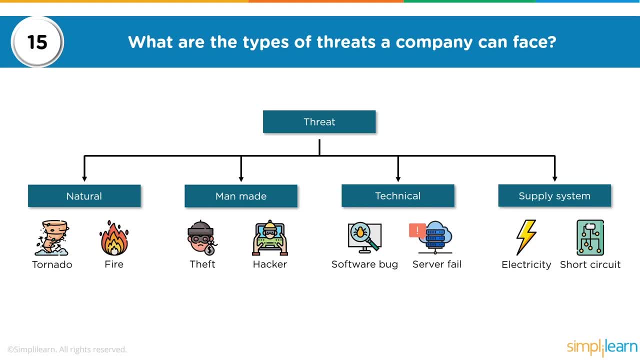 let's say a server failing or a patch that is not installed on a particular software. those would come under technical threats. And then the supply system. The supply system are your environmental threats, which depend on your supply chain failures. What is the supply chain For the office to function? 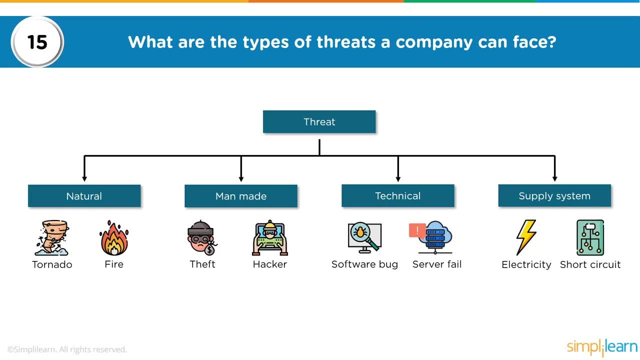 there are a lot of dependencies that office goes through. There are a lot of other vendors that support and provide critical infrastructure, non-critical infrastructure for the office to function, First and foremost, electricity. Without electricity, nothing is going to be powered on and your 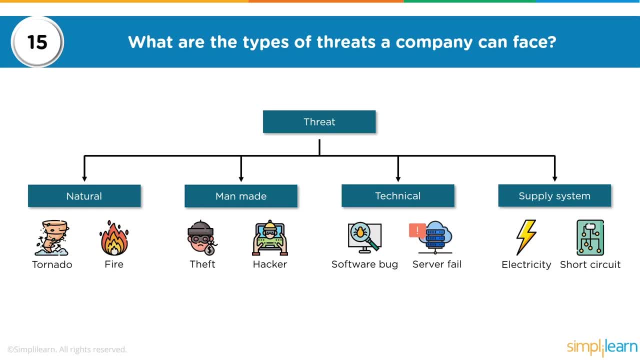 not going to be able to function. So if there is an electricity service provider and if there is an electric outage that comes under supply system, So that is a supply chain failure, where the vendor that provides electricity to you has failed in providing that particular service. 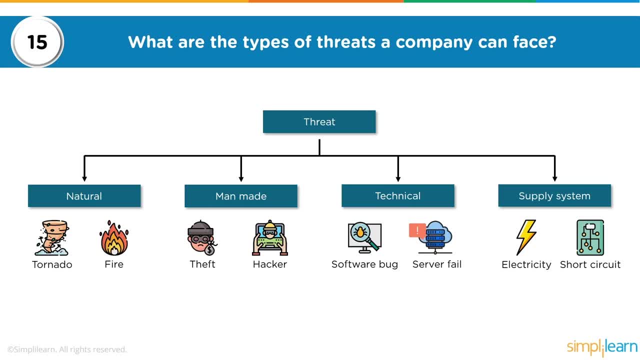 and now you need a business continuity or a disaster recovery plan. So you probably have an inverter or you already have a power generator plant that is going to generate your own power and supply it to your system. There could be short circuits because of fluctuation in electricity. 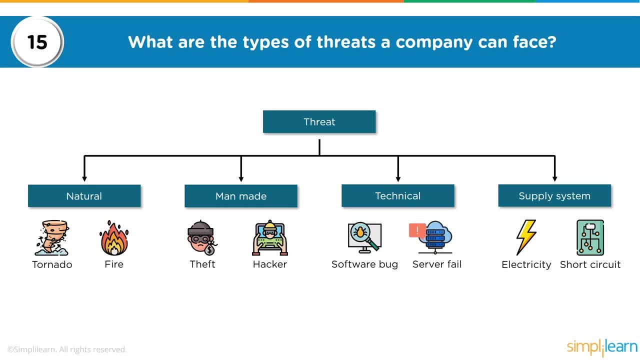 Maybe the internet service provider fails and your internet caches so you have a backup line for the internet from a different vendor, Right, And so on, so forth. Maybe your hardware vendors, who are supplying you servers, desktops, laptops and what not, They fail because 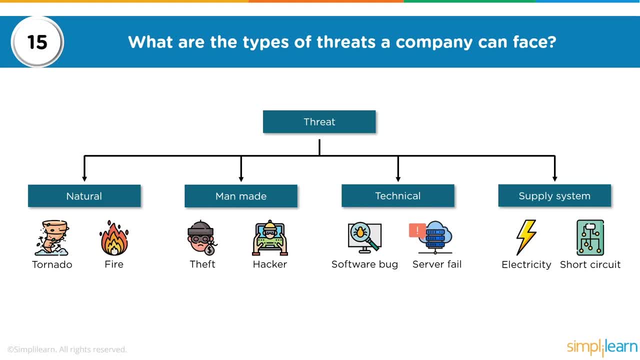 they are facing a strike or they go bankrupt and suddenly you can no longer purchase hardware from your vendor because they no longer are in business. So that is a supply chain failure. So any of these systems failing would also come under threats, So under a broad category. 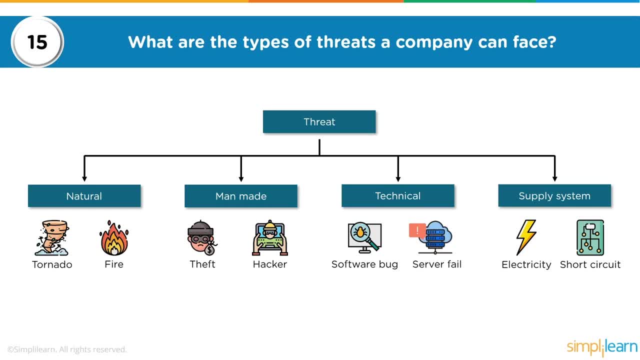 these are the first four threats that you need to identify and then you can elaborate by providing more scenarios based on the experiences that you have had towards each and every of these threats. So, a natural threat where you may have had experience where there would have been, let's say, a flooding. 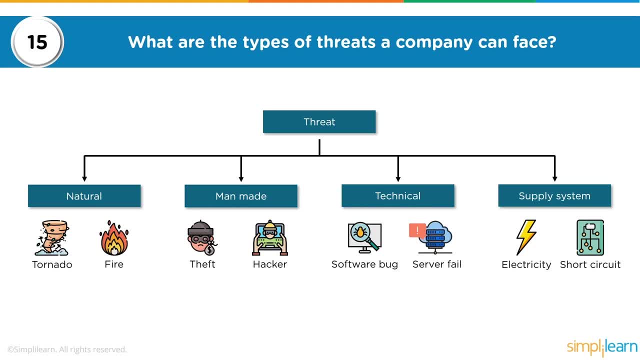 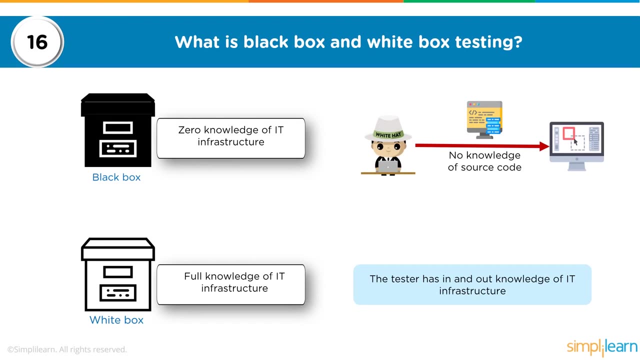 or any natural disaster which caused a problem for the continuity of your particular business. So identify each and every example for each of these threats and provide that as an example in the interview. What is black box and white box testing? So when you are testing a software, 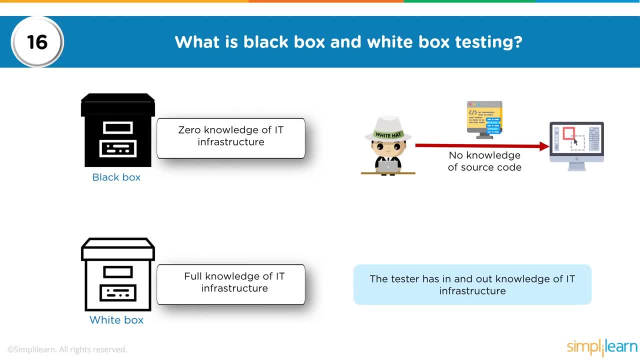 or you are testing your infrastructure. there are two different tests that you can conduct. The first one is a black box. The second one is a white box. In a black box test, there is no knowledge that is shared with the tester. So let's say: 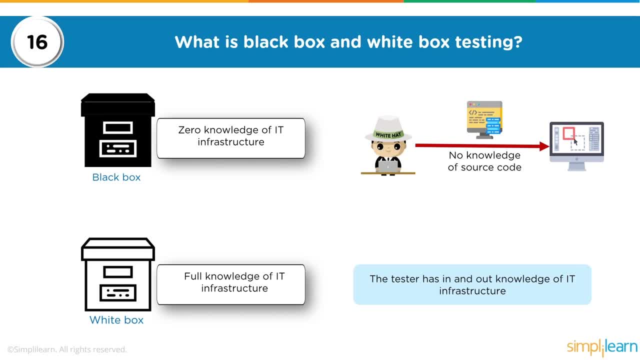 you are an ethical hacker and you have been awarded a contract by an organization to test their current application that they have developed. Now they are not going to give you any information. They are not going to tell you what the application is, They just probably give you an IP. 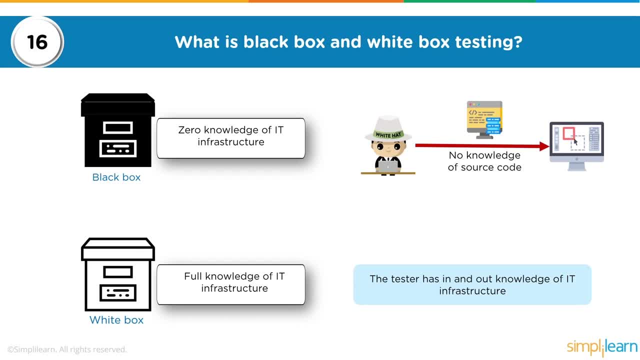 address and a port number where the application is hosted. and now you have to fire in your own queries and try to figure out what the application is, try to gather information, see what information can be gathered in the first place and based on that you are going to. 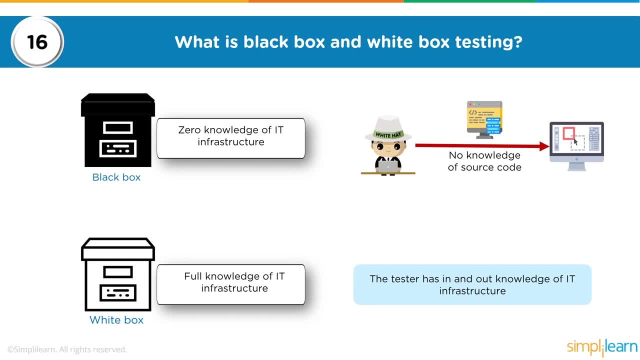 figure out your way, identify vulnerabilities and see if any of those vulnerabilities can lead to an security incident. So, without any knowledge, zero knowledge of the IT infrastructure or the source code, that's a black box attack or a black box test. A white box test, on the other hand, is where 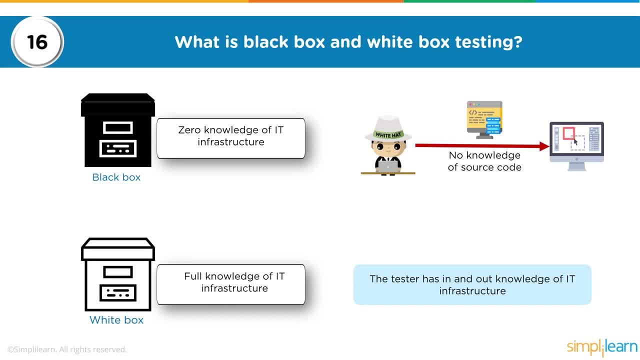 full knowledge of the IT infrastructure or the source code is shared. So the ethical hacker has complete knowledge and, based on the knowledge, they are then going to test out the system to see if there are any flaws that they can identify. So why would these two audits be? 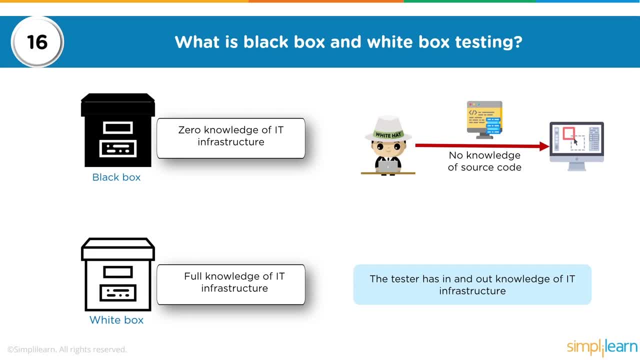 important Because the first one, a black box audit, emulates the attack of an outsider, an external hacker sitting outside the organization trying to figure their way in, Whereas a white box attack can emulate the attack of an insider, So a disgruntled employee, within that organization. 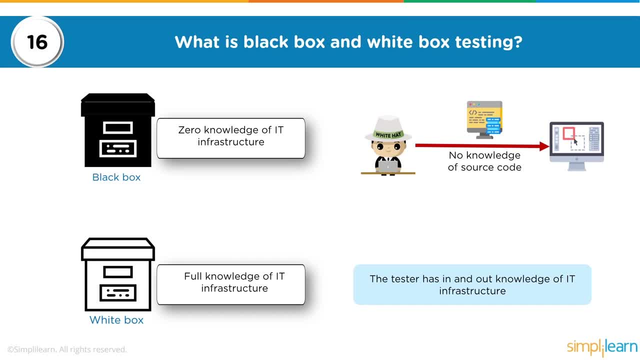 misusing their access controls or their access rights to make unvalidated profits. Right, So somebody is corrupt, who has been bribed, who wants to sell out company secrets. so they are going to try to find out vulnerabilities, try to steal data and try to sell it on the 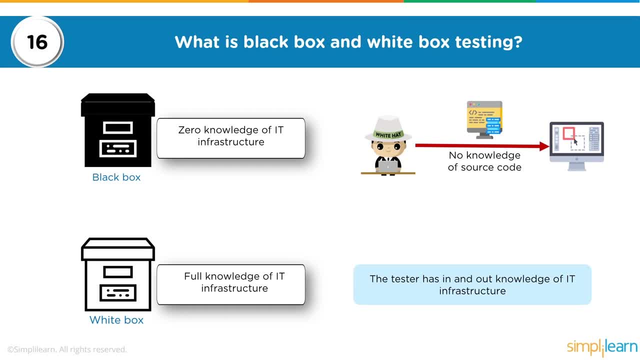 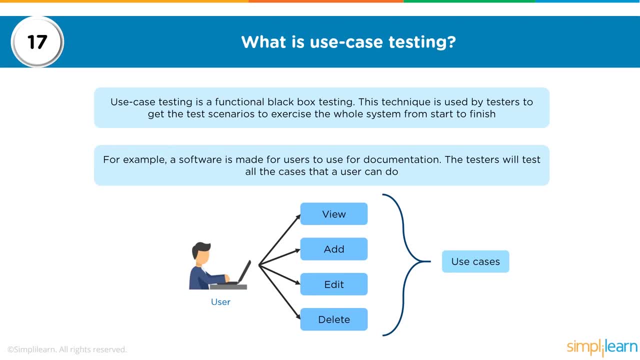 grey market Right. So a white box would emulate an internal attack, a black box would emulate an external attack. Moving on to question 17,. what is use case testing? Now, use case testing is a functional test and it is also a black box. 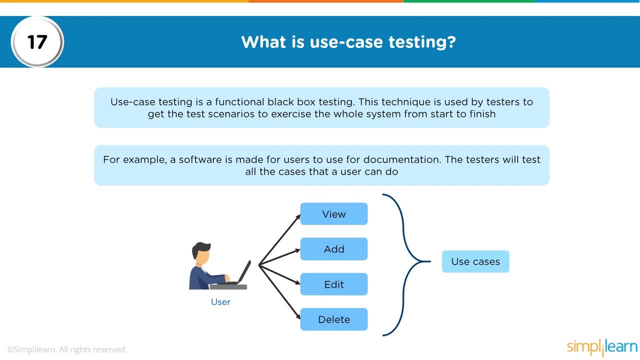 test Right. What is a functional test? It tests the functionality of a particular software once it has been created. Why is it a black box test? Because the user doesn't know what the functionality is. they just want to find out each and every scenario. 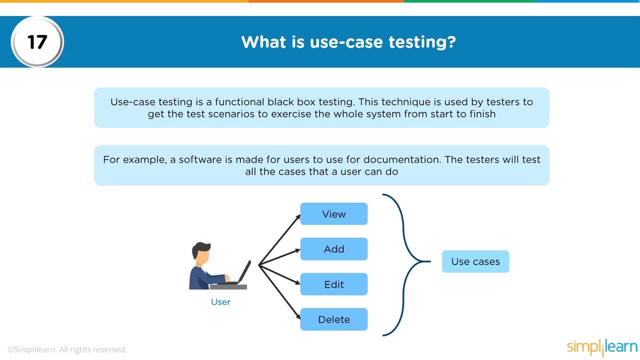 and try to see what that scenario generates as a response. They are not sure whether that is the appropriate response that should be generated or not. They are just trying to find out the response that is going to be generated after they fire off a query. 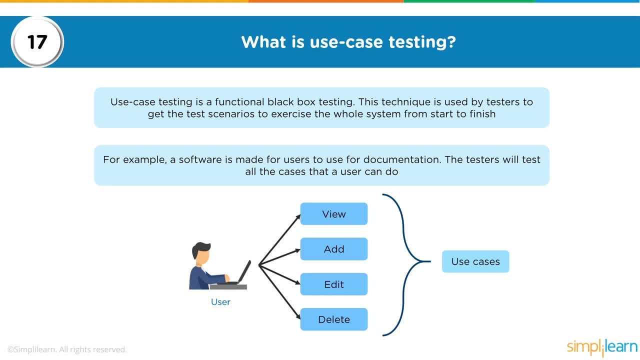 So this technique is used by testers to get the test scenarios to exercise the whole system from start to finish. So let's say it's a login mechanism for an application. Right Now a user, at this point in time the tester, since it's a black box test. 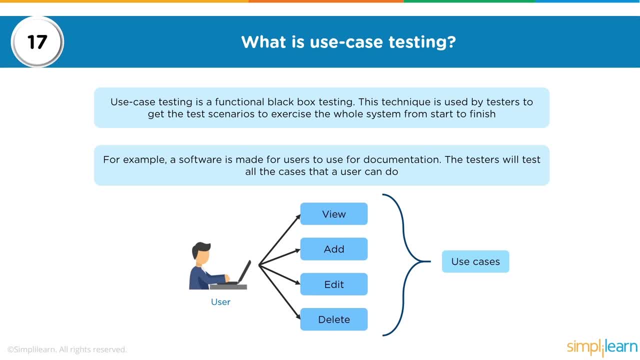 testing will know that it is a login mechanism. They will not know the details of what logging mechanisms are being utilized. So they wouldn't know whether input validation is done. They wouldn't know whether output encoding is done. They wouldn't know how the CGI calls are being made. 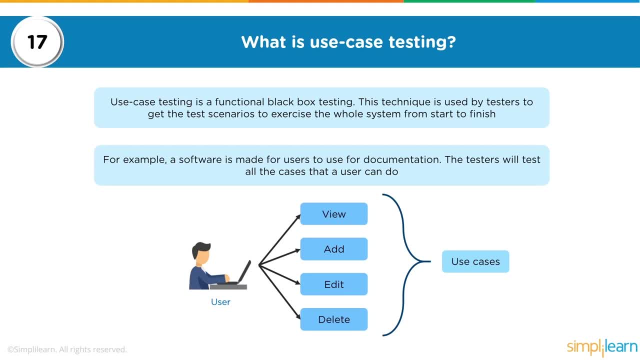 They will not know how the queries are handled at the server side and how the database is going to treat that particular query. So they have no idea whether SQL injection attacks are possible, and so on, so forth. So for them, with whatever input they are going to try to insert, 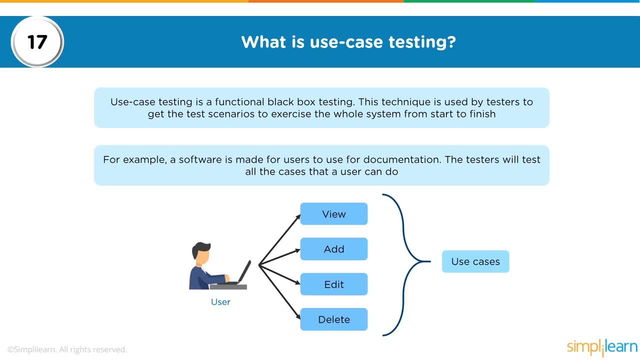 for that login mechanism. that's a functional black box test, The functionality being whether the login mechanism works and, based on the type of inputs that they are going to put in, whether it creates an unwarranted output, Whether they can bypass the mechanism or. 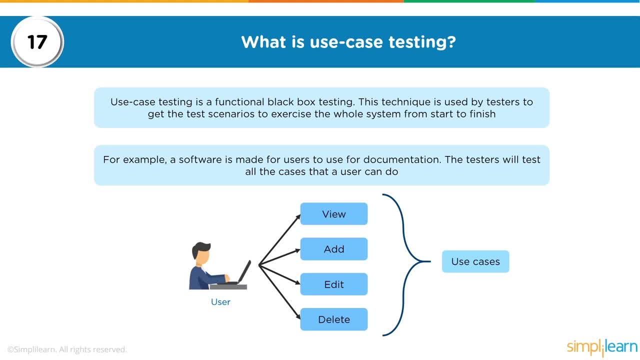 they can hack into the system because of some of the flaws that were left behind Right Another example here is a software made for users to use for documentation. The testers will test all the cases that the user can do So. can the user view? 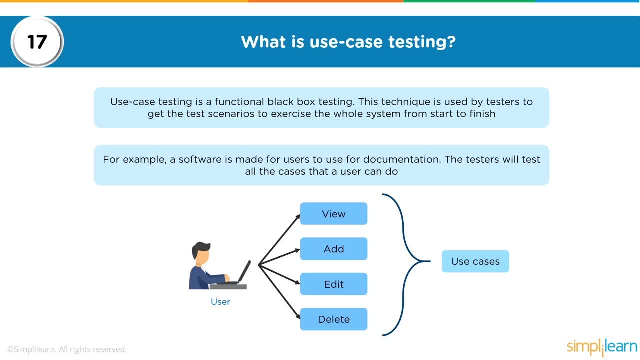 a document, Can they add new documents, Can they edit documents and can they delete documents. So this functionality will depend upon the access controls that have been granted to a particular user. So for this particular user, the tester, at this point in time they would not know whether 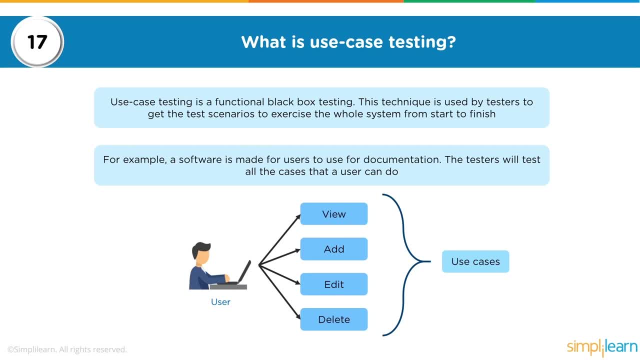 they are an administrative user or they are a regular user. They will just try to do all of these and then write the responses saying I was able to view, I was able to add, I was able to edit and I was able to delete. Now the 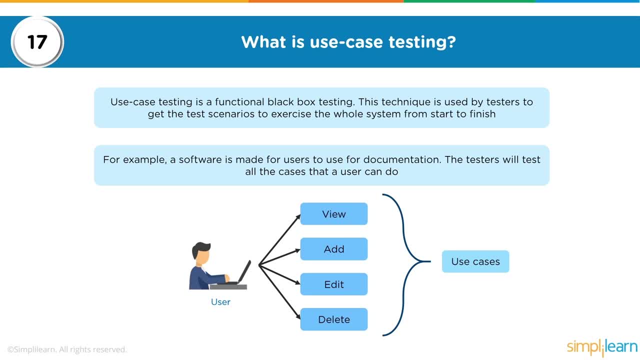 result will be then sent to a manager, that the manager will look at the results and then, based on the actual access controls that were supposed to be there for this particular user, then we will try to identify whether this is an acceptable case or whether there were any flaws within. 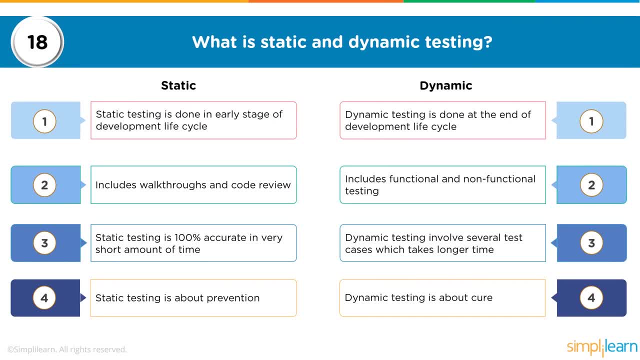 this case. Moving on to question 18.. What is static and dynamic testing? Now, this is again in application testing. Static testing is done in an early stage of development life cycle. Now, software development life cycles, there are multiple of those. What are? 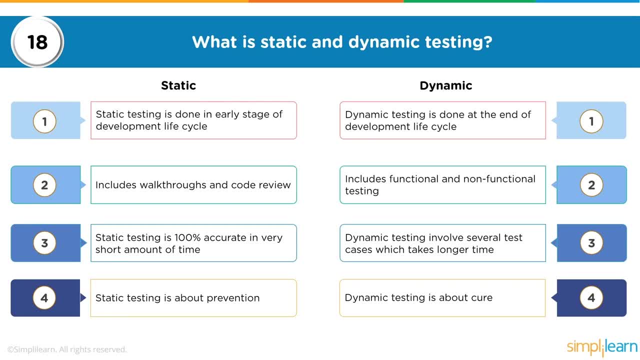 these life cycles. There are different stages in which an application is created and provided to the customer. So your first stage would be determining the scope of the application, determining the hardware requirements for that application, then creating a flow chart for that application, a functional chart for that. 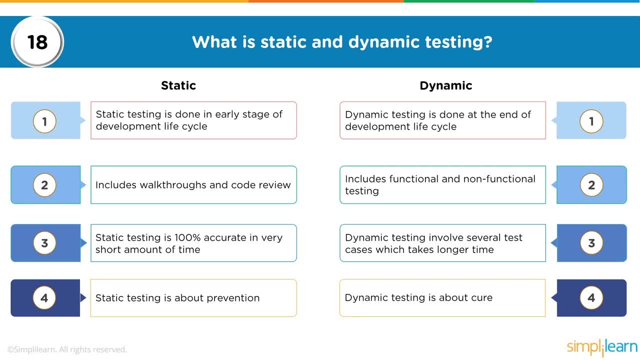 application and then maybe start coding. then an architect comes in, tests the code, verifies the code, then the testing phase comes in, then the security testing phase comes in and then the user acceptance testing comes in. But in every stage, at the very earliest of all stages. 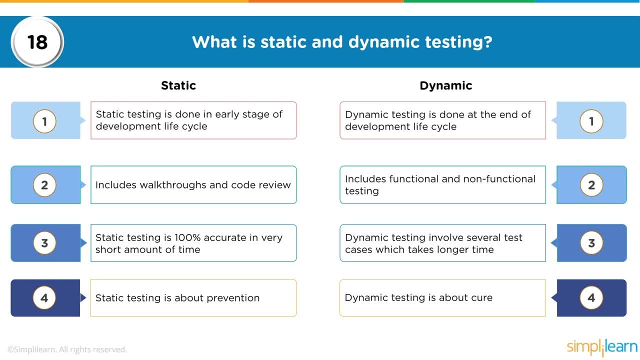 a static test will always be started to see whatever code has been developed, whatever scope has been developed, whether that scope is going to be correct or not. This will include walkthroughs and code review. What is a walkthrough? A walkthrough is going through documents that have been generated. 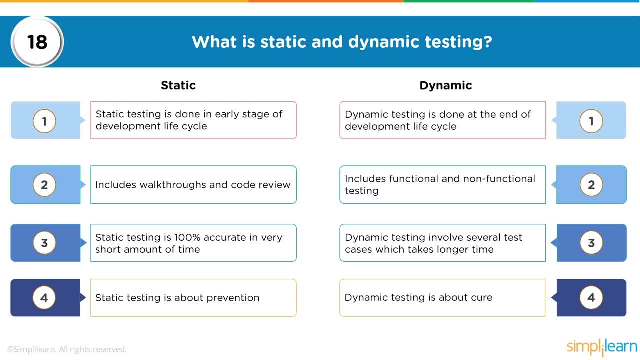 and trying to find faults in the documented journey that has been created so far. So let's say somebody has created a workflow or a flow chart for a program, how the functions are going to be called and how they are going to be executed. So a walkthrough would be where 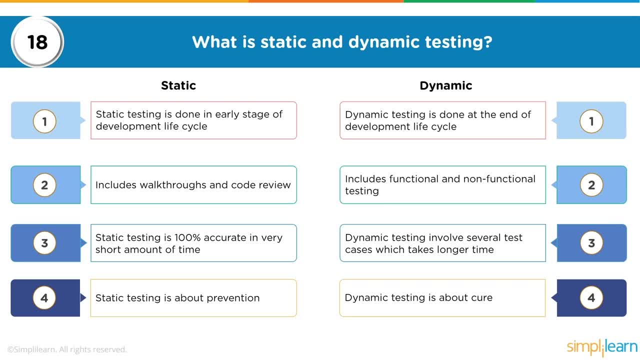 all these responsible people will walk through that particular flow chart and find out any flaws within that and then rectify them. If there is any code that has already been written, this code will be reviewed manually and any flaws within that code would then be identified. 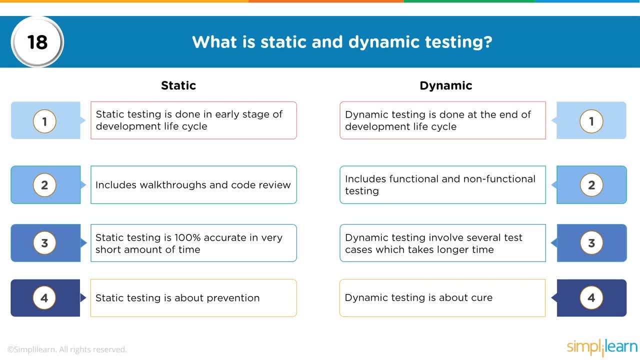 Static testing will always be 100% accurate in a very short amount of time because it is immediate. You have created it and then the robot is going to test it to see whether everything is fine or not. It is all about prevention mechanism, Since you are doing it at the inception itself. 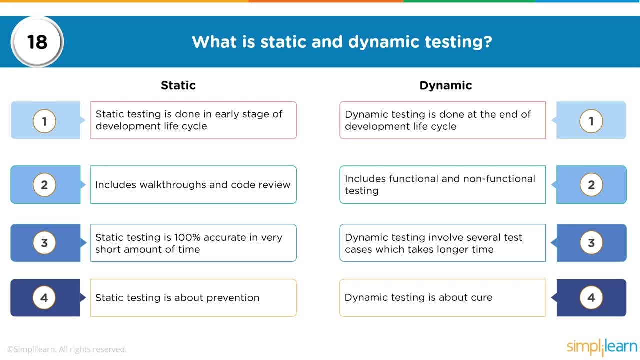 if you find any flaw, it gets immediately repaired. So this is about preventing vulnerabilities from creeping into that application at a later point in time, Whereas dynamic on the other side is done at the end of the development lifecycle. So you have generated the application, everything is ready. now you want to do. 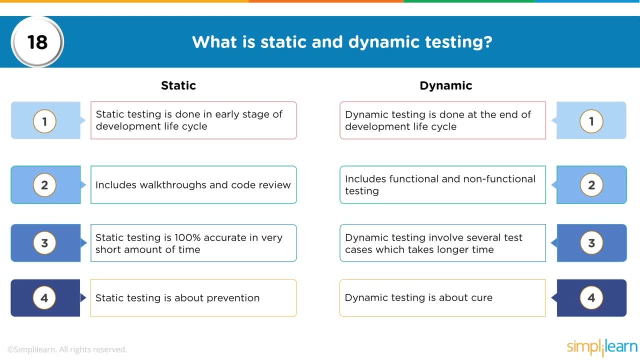 dynamic testing. It includes functional and non-functional testing. Functional testing is where the application itself is being tested, the functions, to see that all the parameters that are given to the application are functioning properly. Non-functional testing would be where security parameters, administrative parameters, all of them. 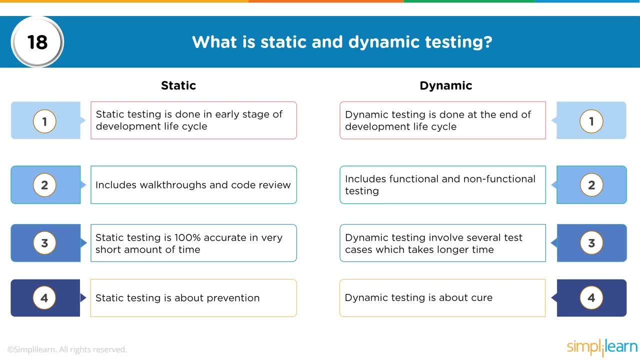 are being verified. This is where your test case scenarios come in, and you are going to test each and every scenario by generating inputs and analyzing the output that the application is going to give you. Dynamic testing is all about cure. You are going to identify vulnerabilities. 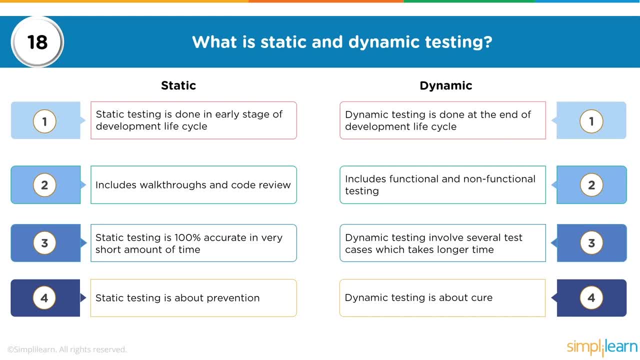 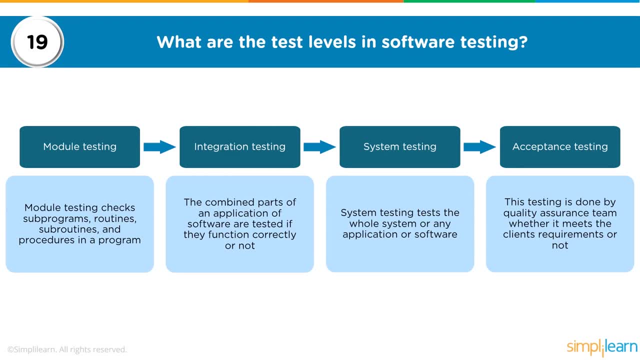 report them to the management, and the management is then going to figure out a way of patching those vulnerabilities so that they can be mitigated. Moving on to the next question, what are the test levels in software testing? So, as far as software testing is concerned, 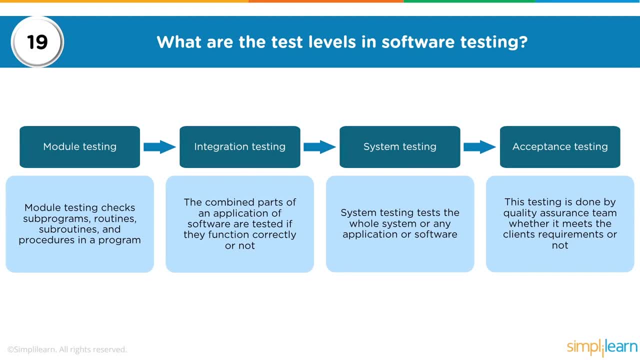 there are four test levels: Module testing, integration testing, system testing and the final one is acceptance testing. So, in the testing phase of your development lifecycle, the first thing is a module test. You are going to check your routines, your subroutines, your subprograms. 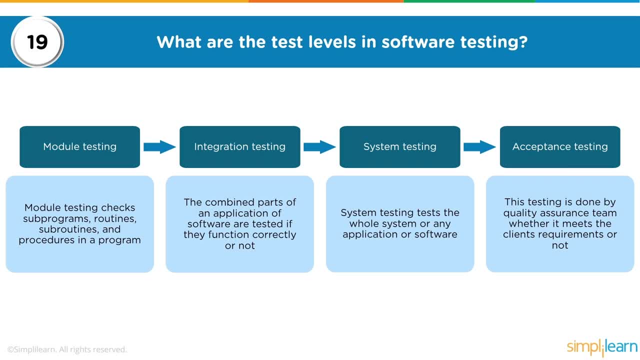 procedures that have been written in a program. So all your functions, all your mechanisms for that application are going to be tested When you go into integration testing. the software may have been integrated with multiple softwares. there may be different API calls coming in, maybe a third party software. 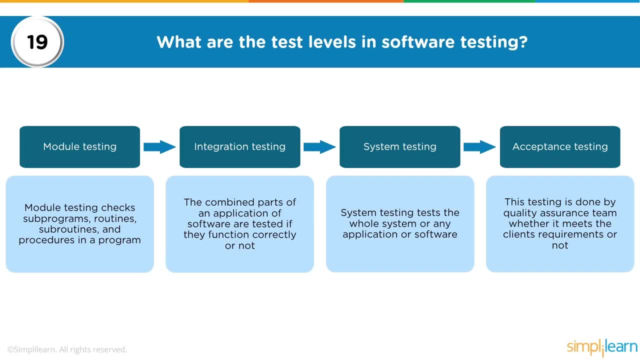 on which you are depending upon to supply for information. So all of these integration of various softwares, various APIs, are tested to ensure that they are functioning properly and there are no flaws, errors or mistakes left behind in the integration of all of these softwares. 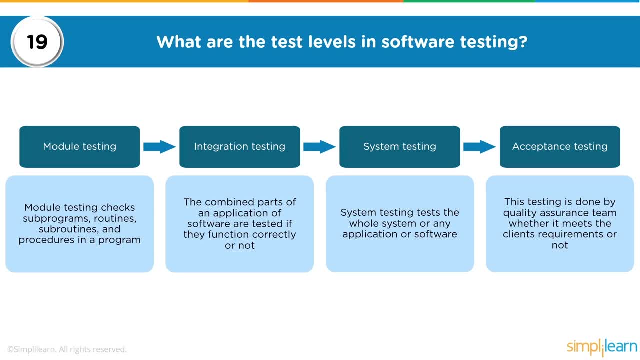 Then the system testing is where the entire system- so including the hardware, including the software- right it starts from the installation. So now the software is complete, we know which hardware we are going to support for it. we start by installing the software and see whether the installation is going to be. 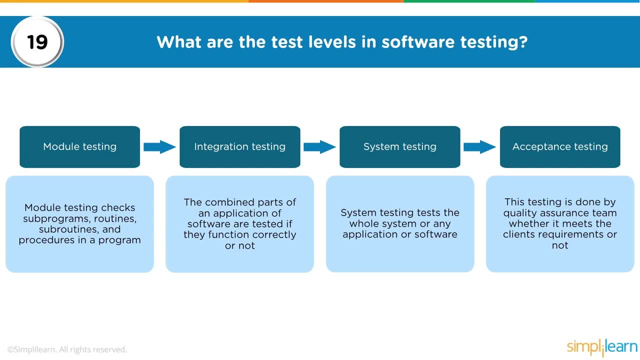 completed properly. if there are any errors in the installation process itself, Then once it is installed, the performance of that particular application, the write speeds, the read speeds on the hard disk, the transaction speeds that the application is capable of, the network dependencies that the application may have. 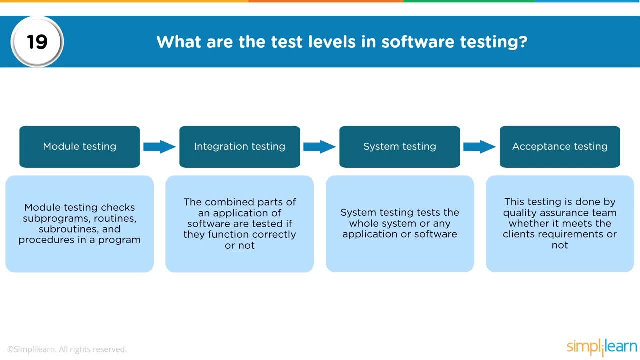 all of those would come under system testing And then the acceptance testing, which is basically a quality assurance exercise that the application meets the client's requirements. So the client in the first stage would have given the scope of what needs to be achieved In the acceptance testing you are 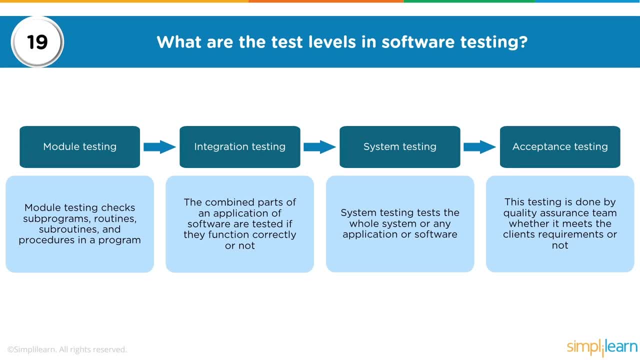 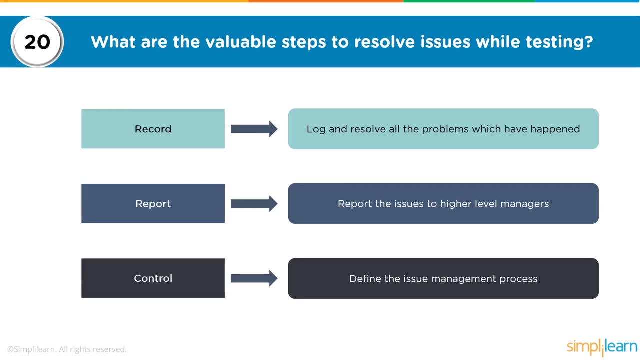 verifying that that scope has been met and the client requirements have been met and you can assure the client about the functionality and the performance of that particular application. Coming to the last question, in this software program, what are the valuable steps to resolve issues while testing? So, in the previous scenarios, when 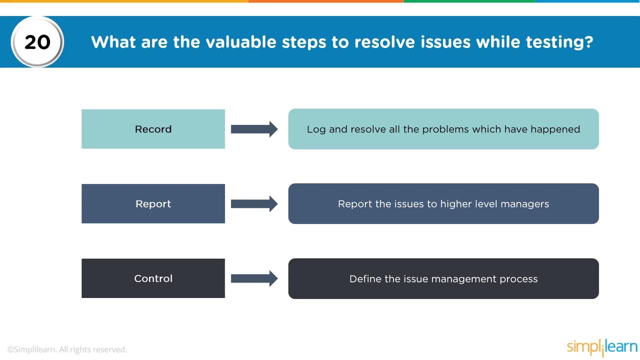 we have started testing now. if you find out, when you execute a particular use case and then you find out a flaw, what would be the steps that you would utilize to address those particular flaws in those tests? The first step will always be record. then you are going to report it. 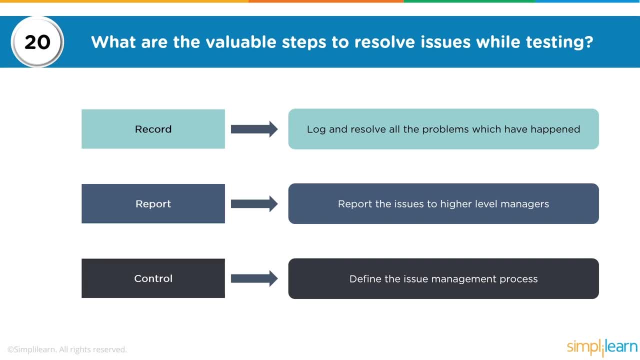 and then you are going to introduce a control process for it. So when you say record, you are going to create logs and you are going to try to resolve all the problems that have happened. Now, when you say resolve, you are not going to recode the application. 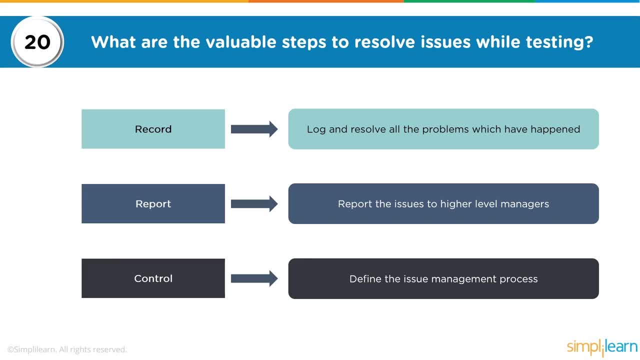 but you are going to test the system again and again to ensure that whatever is being recorded is accurate and all the logs, all the error mechanisms, all the dumps, all of those that have been generated due to this particular log or due to this particular error. 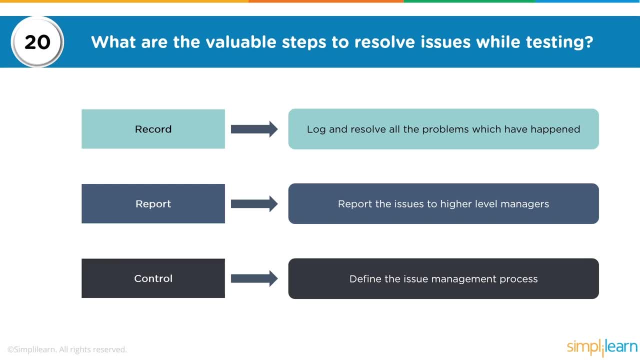 are being captured so that they can be reported to the higher level managers. So the next step is, once you have accumulated all these logs and records, you are going to report them to the higher level managers, who are then going to investigate it and go back to the developers trying to 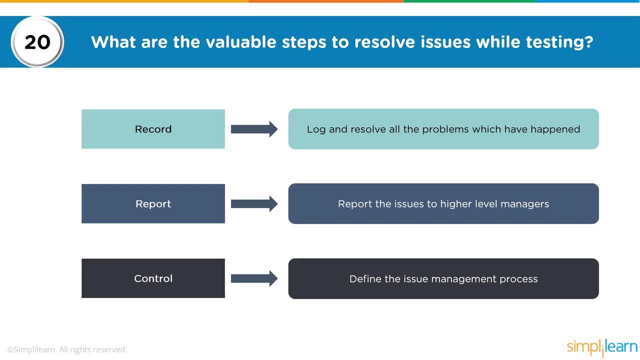 figure out the best way to mitigate those particular flaws. So the report writing also needs to be accurate. it needs to be to the point, it needs to detail what the problem was. it will document all the steps that you took, all the inputs that you put in, and it will also 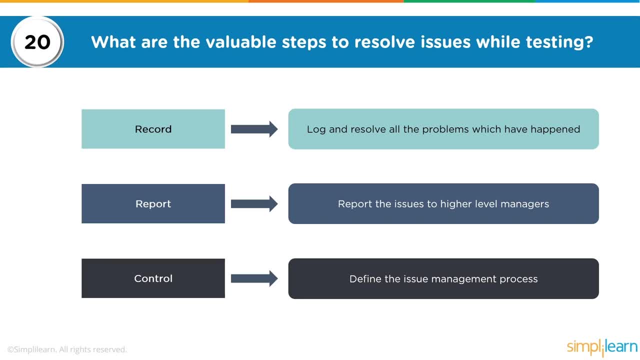 record all the errors and it will also record all the mechanisms that were utilized and errors that were generated, and that report will be given to the higher level managers, who can then forward it to the developers who, based on those reports, can start their troubleshooting. And then the control mechanism comes in. 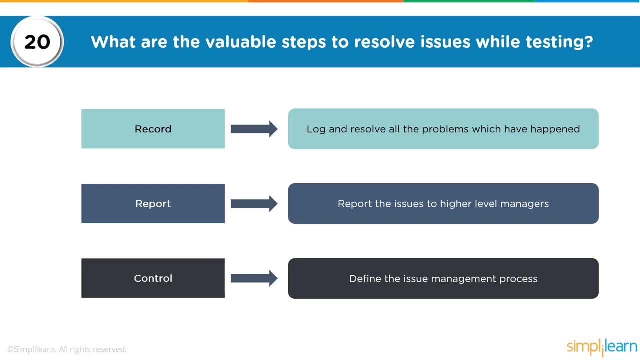 you're going to define the issue management process. So this process needs to work in a particular manner: where you're doing a test, you're recording whatever is happening, you're creating a report out of it, you're sending it to the management. the management will then take those. 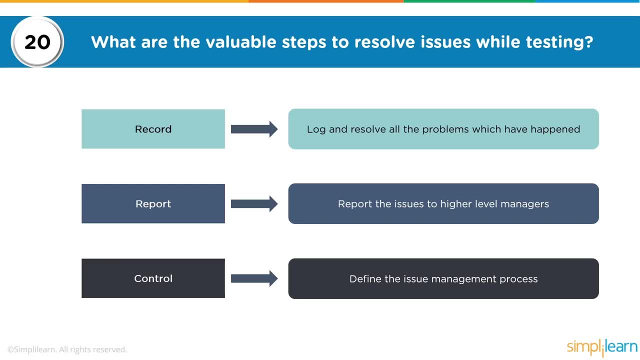 reports, study them, take it to the developers. the developers will test based on their criteria. they might interact with the testers at that point in time to identify particular flaws and then they might want to report that application on a developer patch which, once installed, will mitigate that particular flaw. 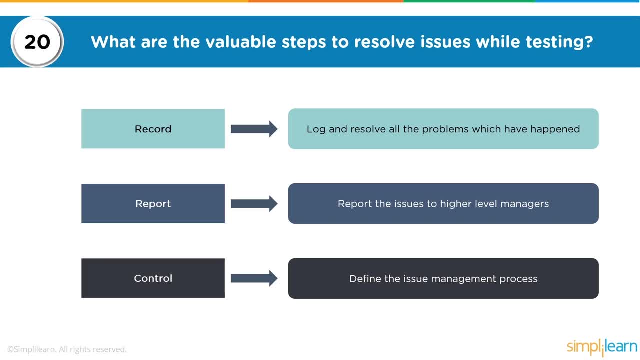 and then it can come back to the testing phase again, where you can repeat those tests and validate that the flaw is no longer existing. So these are the three steps that would be utilized for testing purposes, And that brings us to the first ten questions on the software. 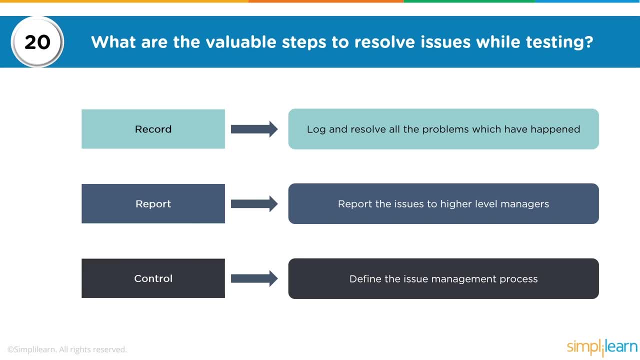 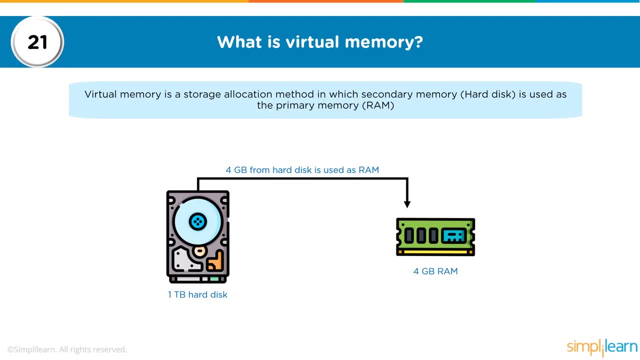 platform. In the next video we'll be looking at operating systems and applications. The first question is on virtual memory. What exactly is virtual memory For a computer? we have two types of memory. First is the primary memory, which is your random access memory, which is also known as a. 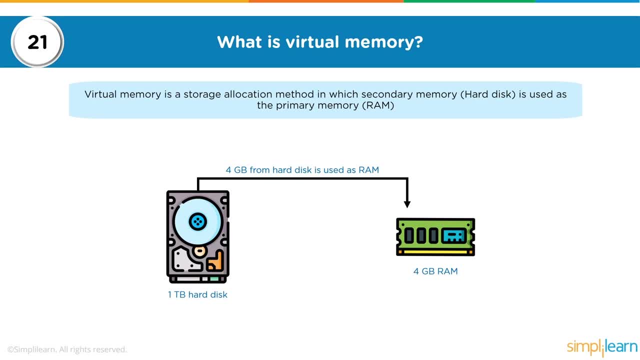 volatile memory, And the secondary memory is your hard disk, where your data is stored permanently. But for a computer, when it has, let's say, a 4 GB memory or a RAM, as in this scenario on your screen, it is going to replicate that and 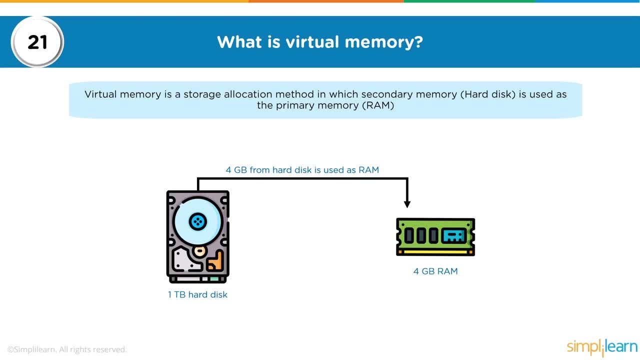 is going to create another 4 GB of virtual memory on the hard disk And it is going to use it in tandem along with the RAM. So if the RAM is insufficient, the processor is going to utilize the 4 GB of the virtual memory that is created on the hard disk. 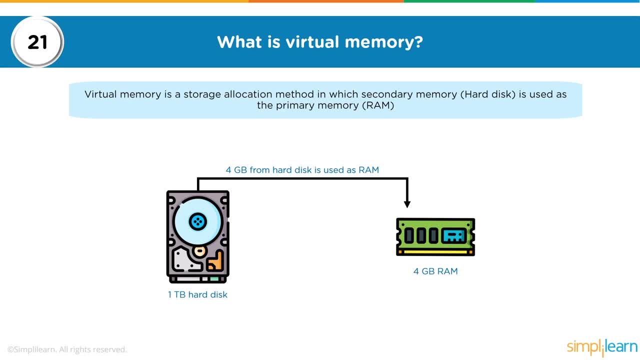 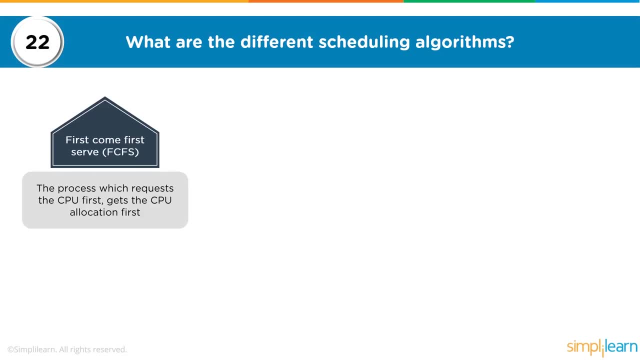 and it is going to swap data from the RAM to the hard disk. This can also be known as a page file or a swap file. The next question is: what are different scheduling algorithms? Now, the context for this question is: you are talking about a processor and you are 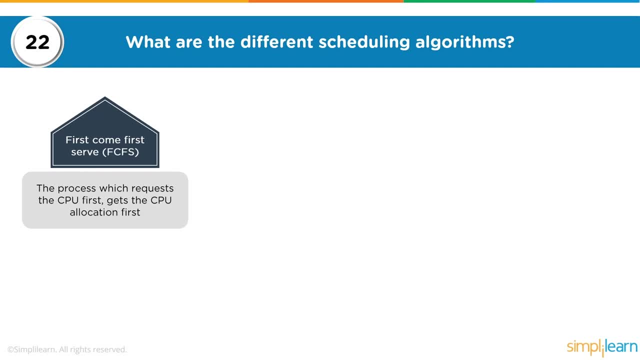 talking about how processors are going to be fed to the processor and how the processor is going to treat these processors. So the first is first come, first serve. So the process which requests the CPU first gets the CPU allocation first. Now, whenever there are processes that are being run by different, 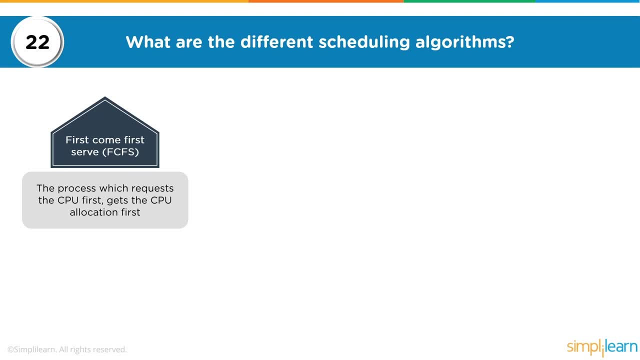 applications they make requests for some CPU time. Now, in first come, first serve, the first service or the first process that is going to request some processing time will get that much allocated to them. They will run through the process first and then the next, and the next, and so 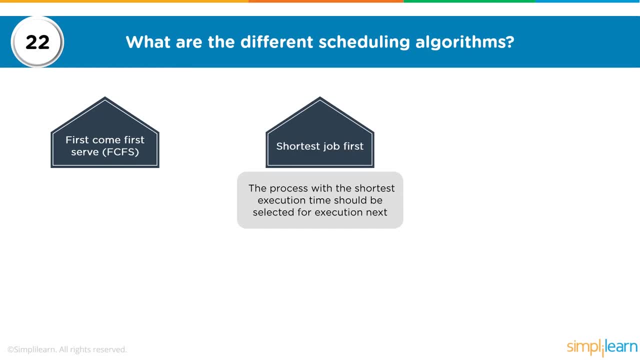 on so forth. The second one is the short disk job. first, This is the process where the short disk execution time for that process is calculated and that process is selected, first for the CPU, Then there is priority scheduling. This scheduler selects the task to work. 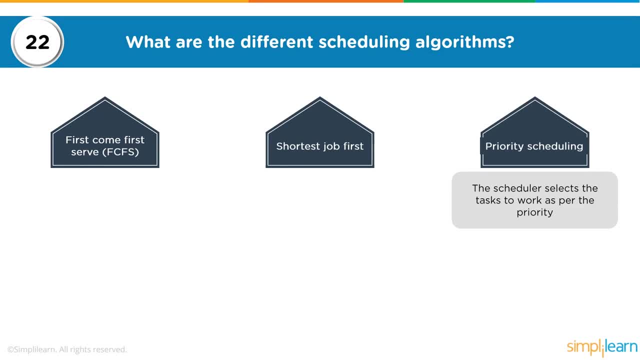 as per priority. So there would be some tasks that are marked with high priority, some would be normal and some would be low. So based on this high, normal or low priority, all the processes will be classified. High priority will be dealt with first, Then 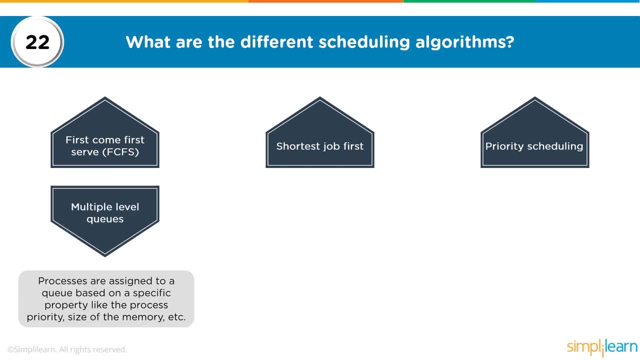 the normal and then the least priority. The fourth option is multiple level queues, where processes are assigned to a queue based on the specific property, like process priority, the size of memory, etc. So it will be classified based on the attributes given to that particular process. 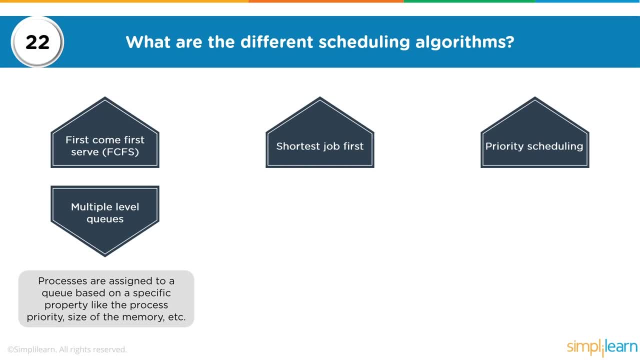 and multiple queues will be created and then, based on the attributes, the processes will be processed by the CPU. Then, shortest remaining time, The process will be allocated to the task which is closest to its completion. So look at it this way: The process that will 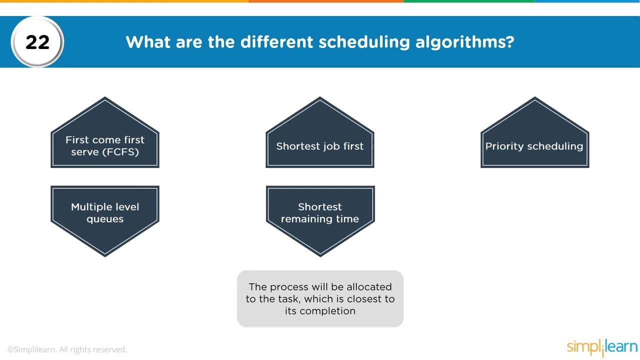 take the least time to complete its processing will be chosen first, And then the round robin method, where each process comes in turn gets an equal share of time. So, if there are 10 processes, each process will be allocated a certain amount of time, after which the next process. 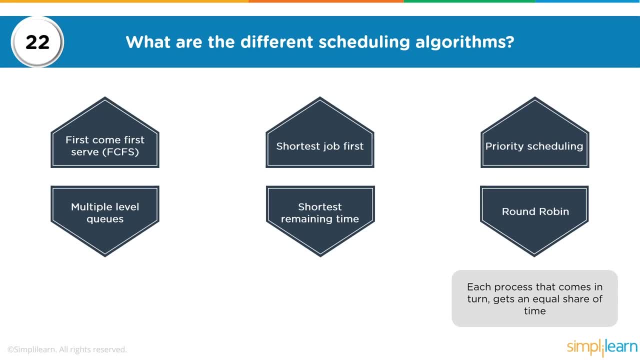 will be processed, and so on, so forth, and it will continue in a round robin fashion till all the processes get executed. So, in short, six different scheduling algorithms, depending on how the operating system deals with it. The next question is: what are the steps involved in hacking a server? 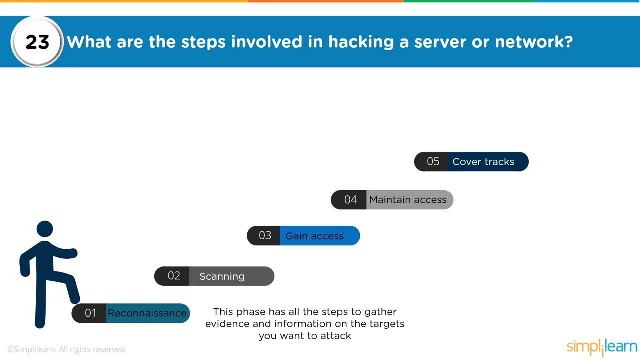 or a network. So this is more of an ethical hacking question. You are looking at devices and the interviewer asks you what kind of steps are involved. what are the activities that you would do in hacking a server or a network? Now there are no specific steps. 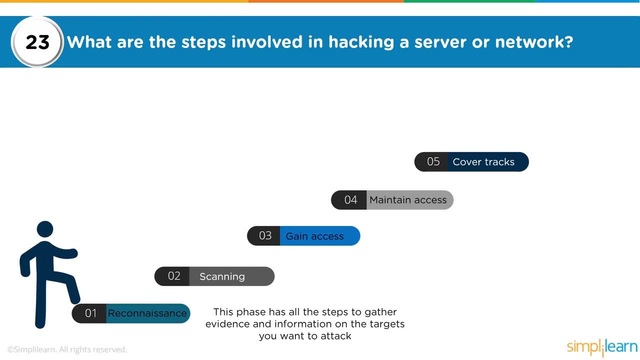 that you would define, because every hack is going to be unique, but a hack can be classified in five different steps, which are quite generic. So the first step will always be the recognizance step, also known as information gathering phase, also known as footprinting or fingerprinting. 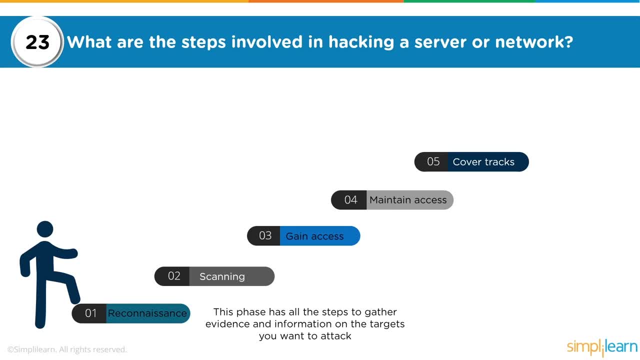 depending on what exactly you are doing. But in this phase the attacker gathers all the evidence, all the information that is possible about the targets that they want to attack. So here you are, trying to get to know the victim so you can launch specific attacks towards them. 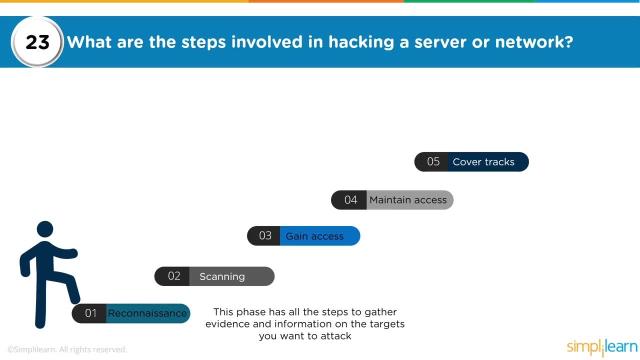 You want to identify what operating system they are utilizing, what IP addresses, MAC addresses, the versions of the operating systems and applications, the patch levels. find out vulnerabilities. find out whatever information is possible. find out the information about the person who is using those. 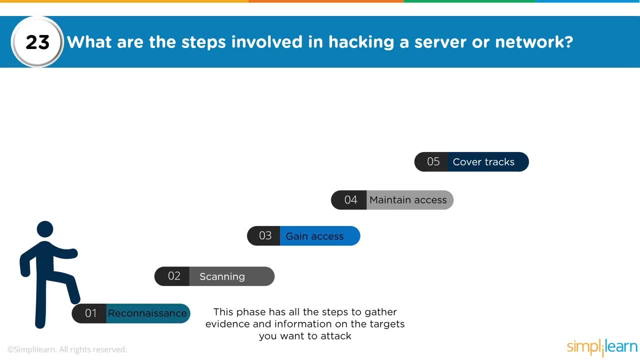 computers so you can launch social engineering attacks and so on, so forth. So the first step is all about gathering enough information based on which you can launch further attacks. Once you have that information comes the second phase, which is known as the scanning phase. This is more of a technical phase. 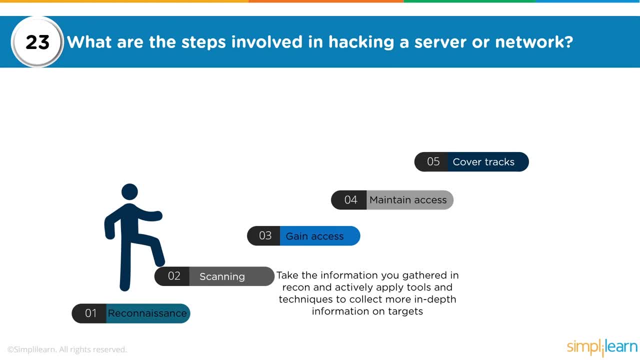 So in the first step, you have got your IP addresses, domain names, maybe even network maps, and you have identified which devices are available. Now, in the scanning phase, you are going to identify live devices and then you are going to scan them for open ports. 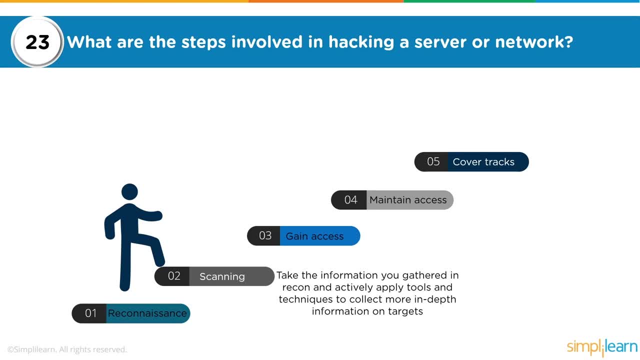 processes, protocols, services. You are going to identify vulnerabilities, you are going to enumerate them, to identify more information from them. Thus, at this point in time, you will have identified a certain set of vulnerabilities or a certain set of security loopholes that you can misuse. 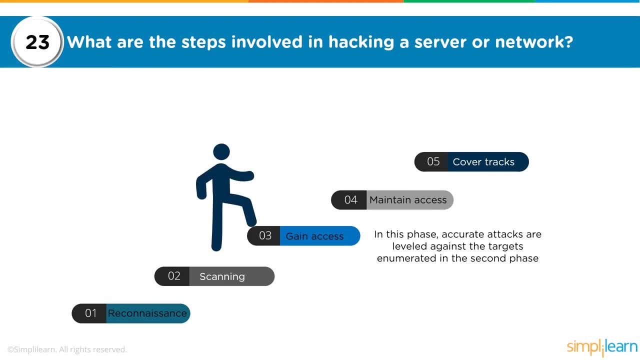 Once you have identified those, you are going to the next step, which is the gaining access step. In this, you are actually going to execute your attacks based on the vulnerabilities that you have identified, and you are either going to gain access to that particular system by installing a 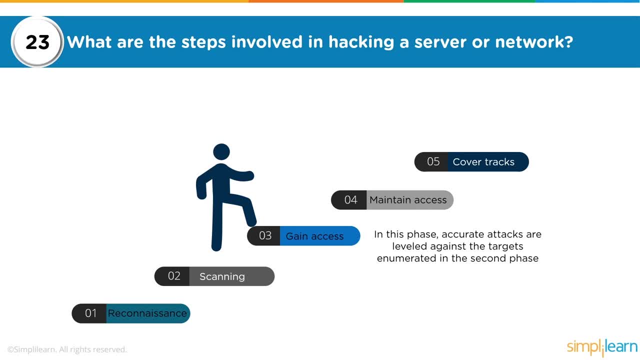 trojan or destroy the system by installing a virus, or install a spyware or a keylogger, whatever you wanted to achieve. So in the gaining access phase you would have based on the knowledge that you have gained in the first and the second phase you are going to launch. 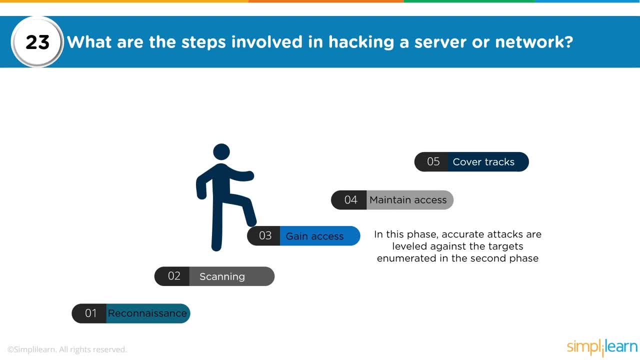 your attacks and you are going to try to gain access to that particular device, Then the next step is where you are going to maintain that access Now that you have hacked into that device. it is not necessary that you will always be able to get access to that device. 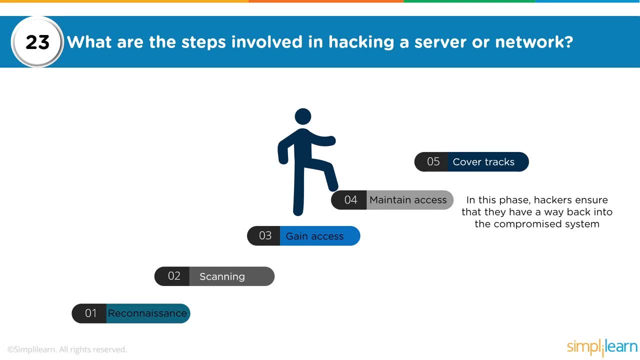 Suppose you have cracked the password of that particular user and the user changes that password after a few days. your attack is worthless. So what you are going to do here is you are going to maintain your access. So this is where it is assumed that you want. 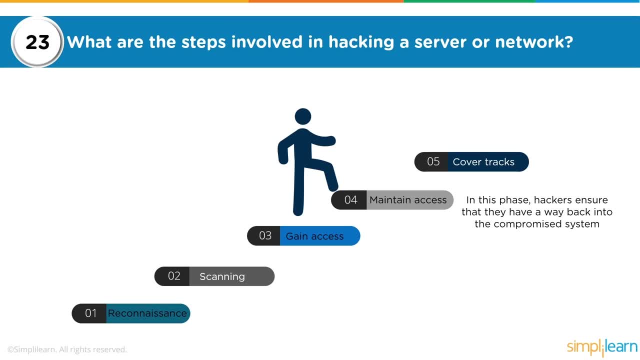 repeated access to that device, and thus you are going to install a keylogger or a trojan or some mechanism which will still allow you to get access to that device without the knowledge or the authorization of that particular user. And finally, the last step is where you are going to cover your tracks. 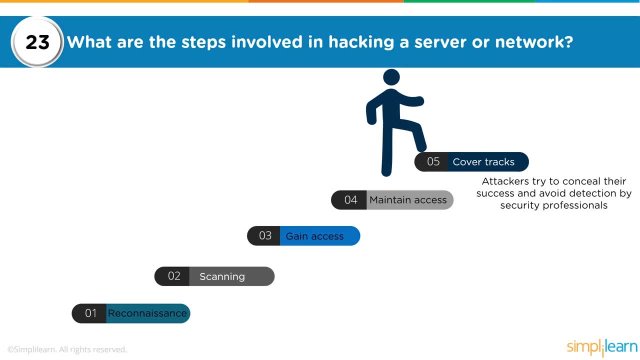 So whatever activity that you have done so far will have created logs and will have created information based on which the victim will come to know that they have been compromised and may be able to trace that activity back to you So to prevent the user or the victim from realizing that they. 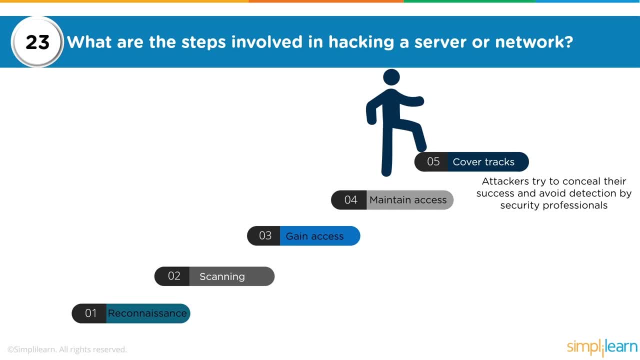 have been hacked and to prevent them to discover who has hacked them, you want to cover your tracks by deleting logs and any references that point to that particular activity. You are going to hide the files that you have created. So you have installed a trojan or a keylogger. 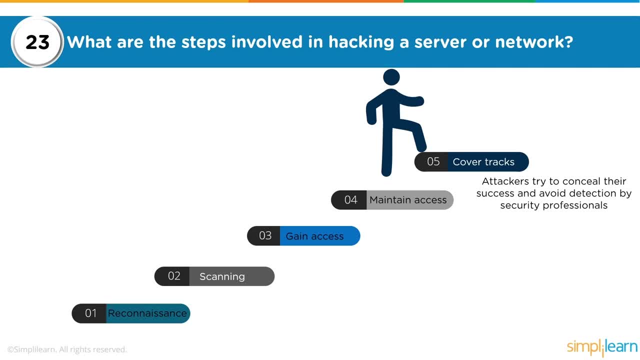 these will create files and directories. You are going to hide them so that they are not discovered. You are going to hide processes that have been created. You are going to try to hide all the activity that you have done so that to conceal the actual attack. 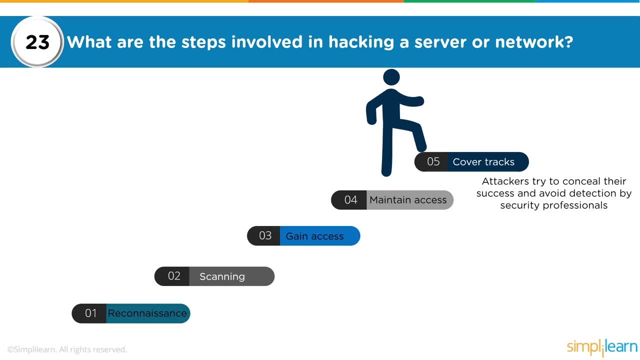 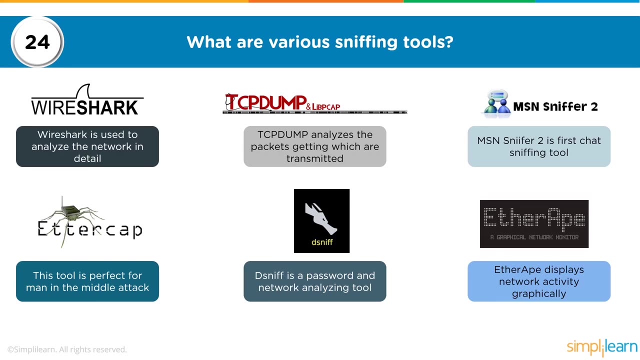 and preventing the user from realizing that they have been compromised. So these are the five steps that will be involved in hacking a server, network application or any computing device you will come across. The next question refers to what are the various sniffing tools. Now, this is a network based attack, where you are 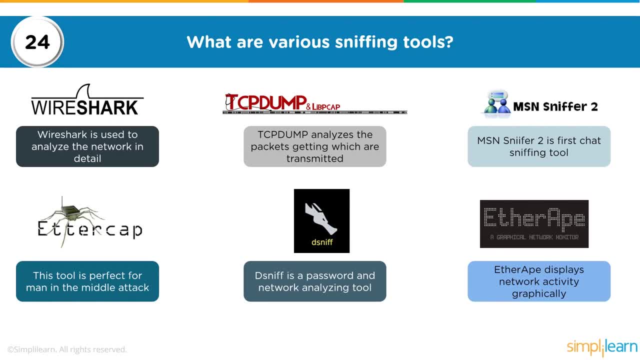 trying to capture data packets that have been transmitted over the network, and then you are going to analyze them to see if you can capture any sensitive information like usernames, passwords, bank details or anything of that sort. Now, these tools will also depend on which operating 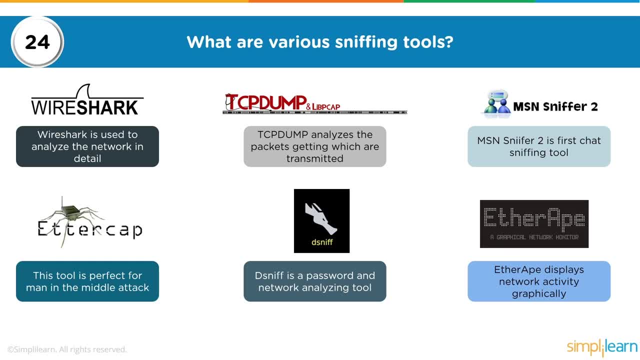 system you are utilizing. For example, MSN Sniffer would work on Microsoft operating systems, Etercap would be more based on Linux, and so on, so forth. So on the screen you will see six different sniffing tools that work on different operating systems. 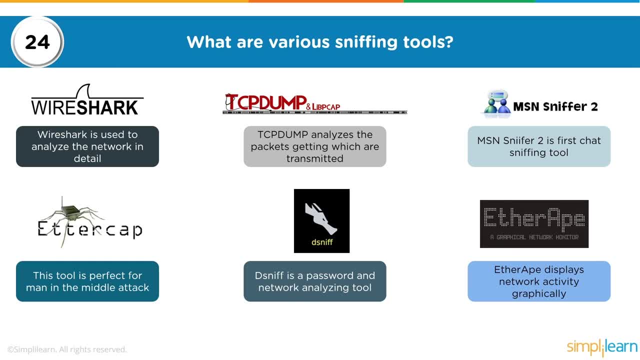 Wireshark is something that is common both on Windows and Linux. It is used to analyze network in detail. It is the de facto tool that you will come across in most of your ethical hacking trainings, in most of your organizations when they want to do data captures. 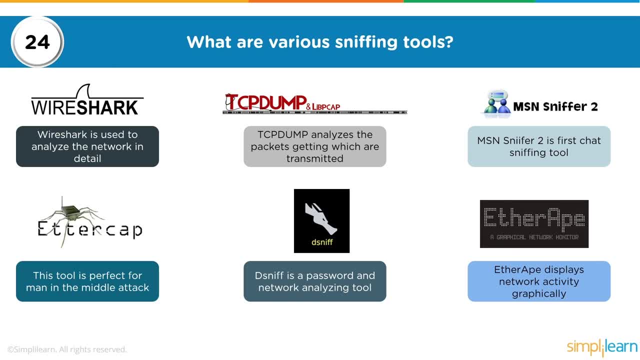 Now, data capturing, or packet capturing, is not only done by hackers to gather more information, but it is also a known troubleshooting technique used by administrators and network administrators to analyze any issues that may be going on in the network. So the first tool you see on the screen is Wireshark. Like we, 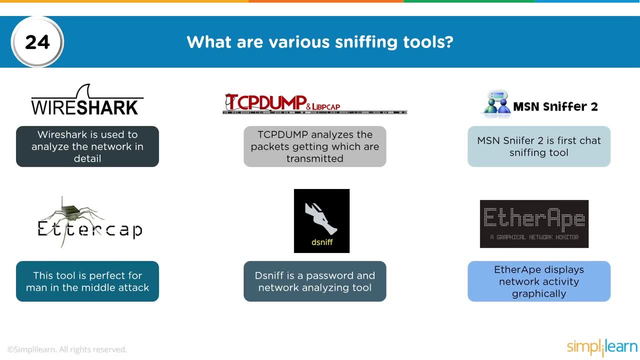 stated, it is available for Windows and Linux as well. Then there is TCP dump, which again has the same capability of Wireshark, but is a command line version. whereas Wireshark also has a GUI, a graphical user interface, TCP dump is available on Linux. 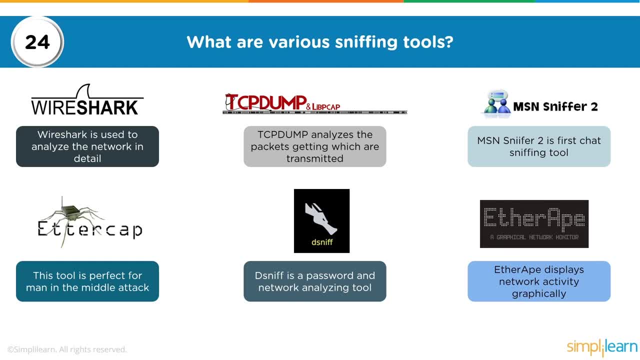 MSN Sniffer is a very old tool when we had MSN Messengers. MSN Messenger is no longer there, but Microsoft does, or did have a Microsoft Message Analyzer tool, which they have stopped development since 2015.. But that is another tool that is. 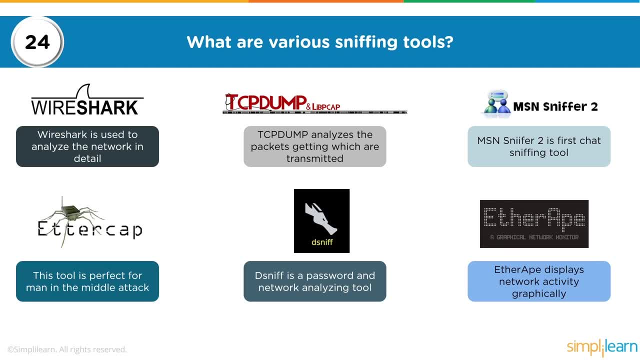 specific for Microsoft operating systems from Microsoft that can be installed to gather more information. Then you have got Ethercap, which is a tool to launch man in the middle, attack data capturing and is essentially a Linux command line based tool. Then Dsniff is another password and network. 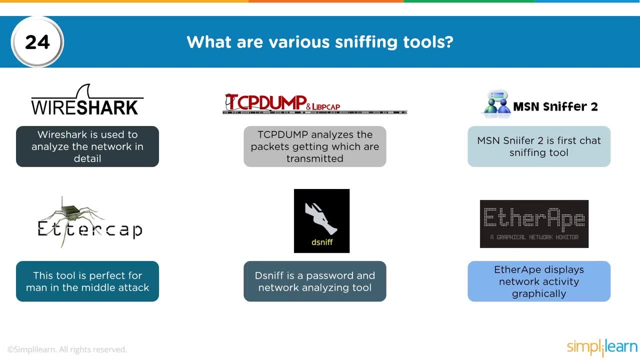 capturing tool which can help you capture data packets, prominently a Linux tool, Same with EtherApe. This is a graphical tool which will allow you to capture data, data traffic and map protocols and identify which IP addresses have been communicating with what. Essentially, all of the tools have similar functionality. 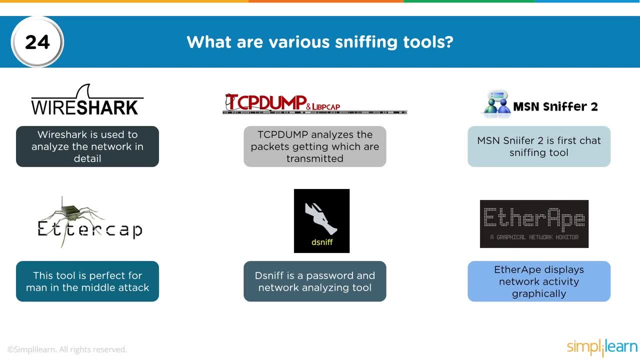 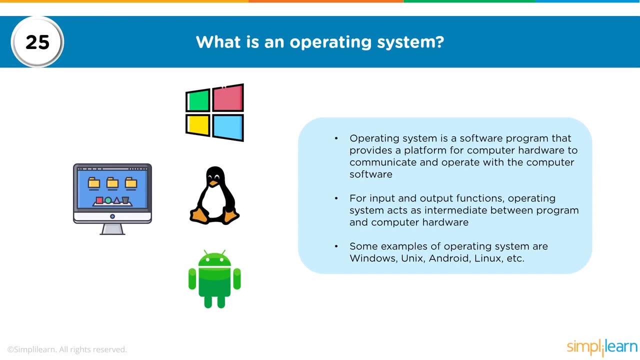 except that some have additional functionality, like launching man in the middle, attacks or capturing, or having specific filters. that will help you identify and troubleshoot some network issues that you may be facing. Moving on to the next question, What is an operating system? Now, this is a very difficult. 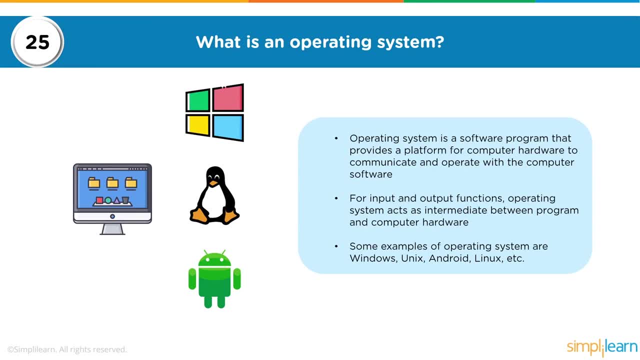 question to answer, because we normally, when we want to answer this question, we start off with the functionality of an operating system. We try to describe what Windows does or what Linux does or what MacOS does, and then we are trying to figure out what an operating system is in the first place. 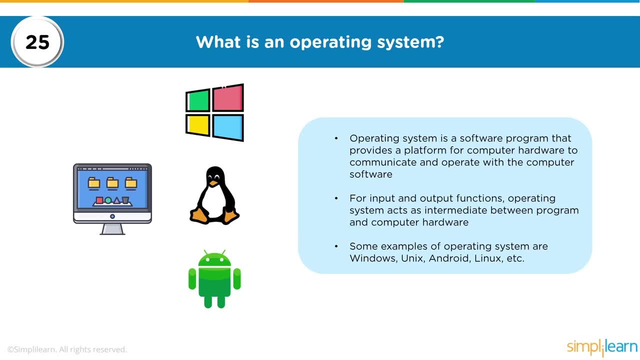 But an operating system essentially, as the slide says, is a software program that provides a platform for computer hardware to communicate and operate with the computer software. So it is basically an enabler for human interaction with the hardware that you have If you take the operating system out of the 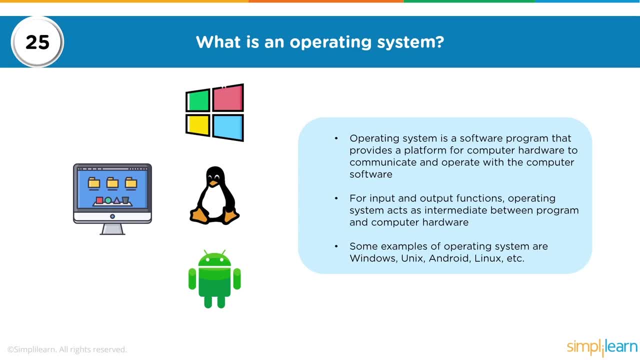 question. it's just some hardware which cannot interact with you. But essentially, when you have an operating system like Microsoft Windows or Linux or Mac, you are essentially installing an instruction set on that particular device which will allow you to interact and manipulate the hardware to do whatever you want. 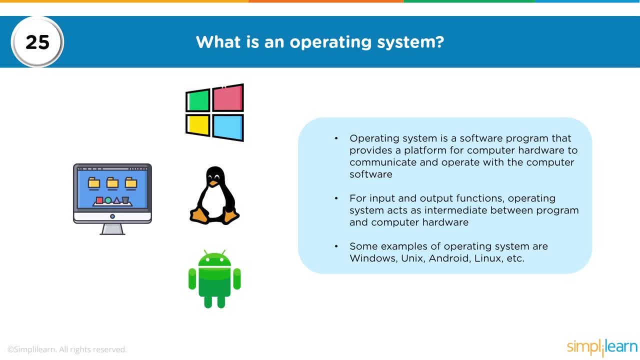 that hardware to do? Essentially, when we talk about drivers for your various devices, like a driver for your LAN card or for your sound card or for your graphics card, which allows you to tweak these cards for functionality. It allows us input and output functions, For example. 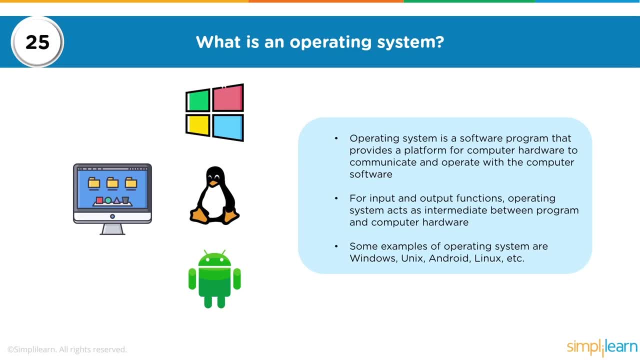 the basic example: you open up Microsoft Office products like Microsoft Word or Excel and you get a GUI on the screen which you can interact with. You got a keyboard and you type on that keyboard and the computer knows what you are typing and reflects those actions on the screen by. 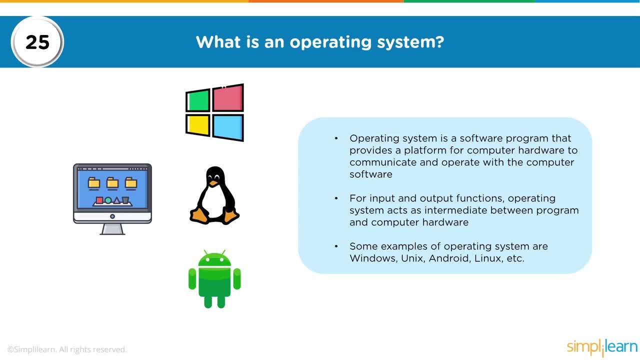 showcasing it on that particular Excel file or a Word file. So how does the computer know what to do, or what you are exactly intending to do at this point? It is all the operating system that is providing you all these services, analyzing what your inputs are and then based 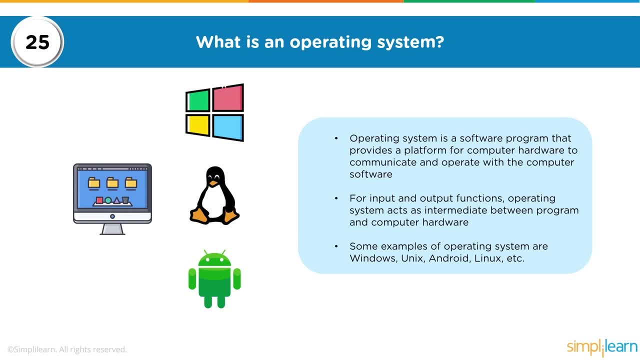 on the programming it is going to execute that and show it to you on the screen. Some of the most commonly used operating systems are Microsoft Windows- you have them in desktop as well as server variants. Unix, Linux- again, Linux has desktop and servers You got. 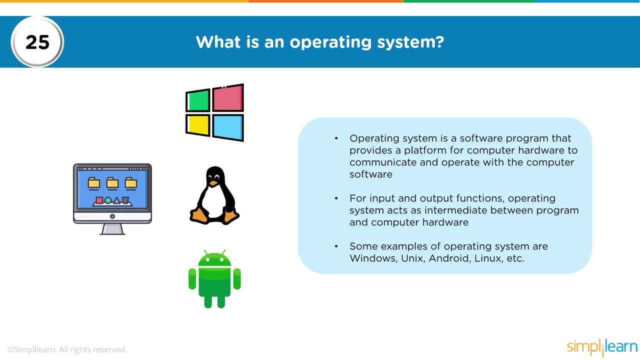 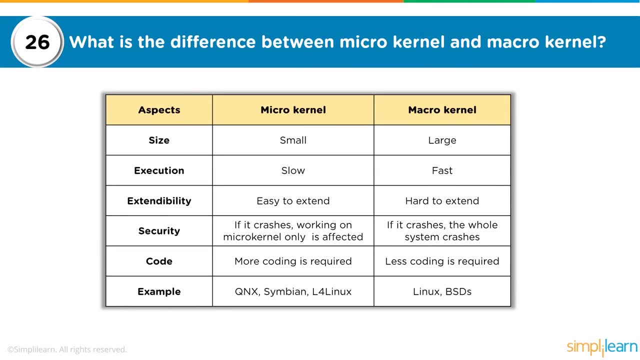 Ubuntu in Linux, Red Hat and so on and so forth. And then you got MacOS for Apple related components. The next question: what is the difference between micro kernel and macro kernel? The first thing we need to know is: what is a kernel? Kernel is the. 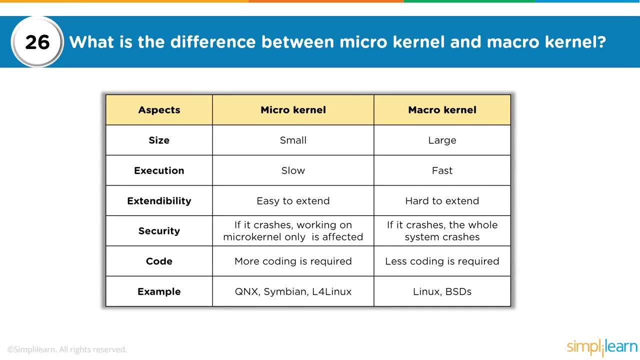 heart of the operating system that allows that input and output to happen. It allows those drivers to be set up so that the hardware can interact with the software and we can then instruct the software and the hardware both to function in a particular manner. So there are two types of 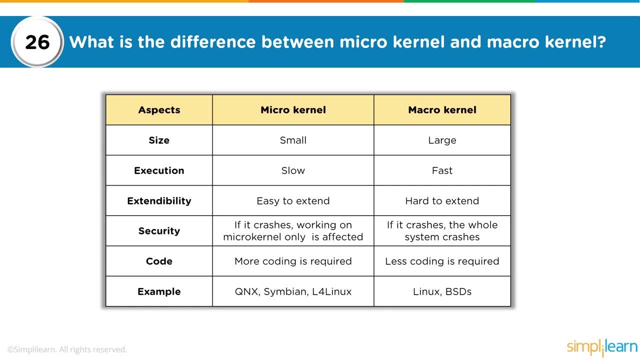 kernels, micro kernels and a macro kernel. Macro kernel is something that we normally use. Micro kernels are for operating systems that use processors directly handled by the processor. The micro kernel is very small in size. macro kernel is large because it basically is the entire image of the operating system. 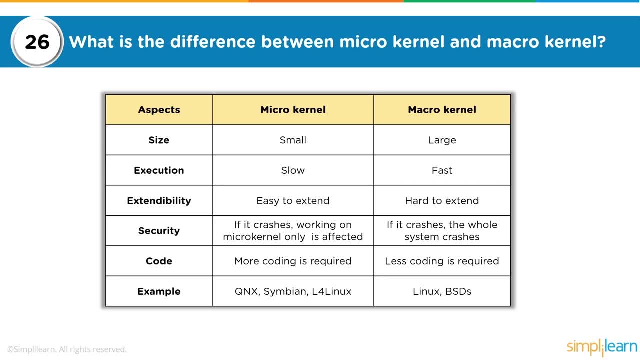 The execution for a micro kernel is slow. the macro kernel is going to be faster because it is more evolved. there is a lot of programming involved. Extendability: micro kernels are easy to extend. macro kernels are hard to extend. As far as security, 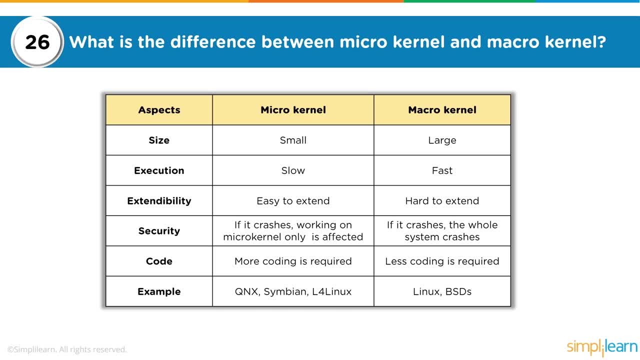 is concerned, if a macro kernel crashes, it takes everything down with it. the entire operating system is going to crash. But in case of a micro kernel, it is only that particular process that is going to get affected. Micro kernel: there is a lot of coding involved. 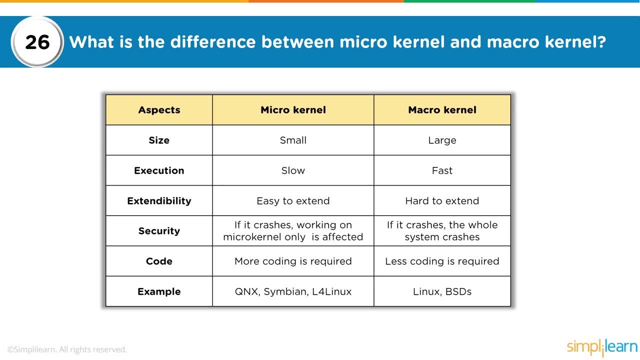 Macro kernel, less coding is involved. Examples of micro kernels would be Symbian OSS, most popularly used on yesteryear phones- Nokias, if you remember those- QNX, and so on so forth. Macro kernels, your Linux or VSD operating systems. 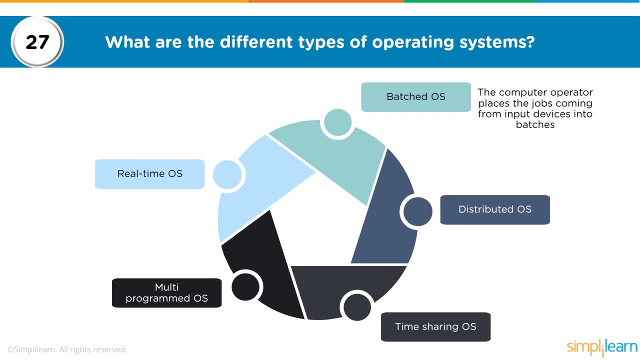 essentially use macro kernels. Next question: what are the different types of operating systems? So, as you can see on the screen, five types of operating systems: batched OS, distributed operating systems, time sharing, multi-program and real time. What are batched operating systems? 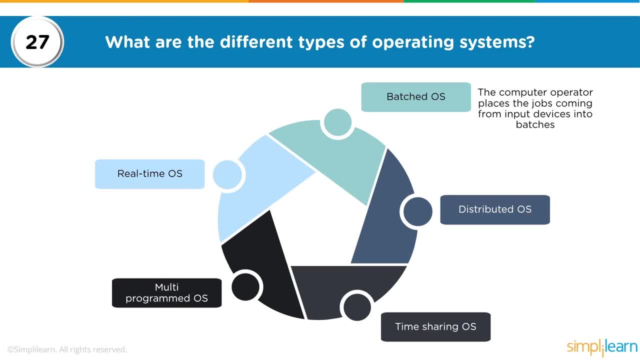 The computer operator places the jobs coming from input devices into batches. So consider this not from a desktop perspective, but from a server perspective, where these devices are used by organizations to compute and to crunch some processes. that is going to make some business sense out of it. 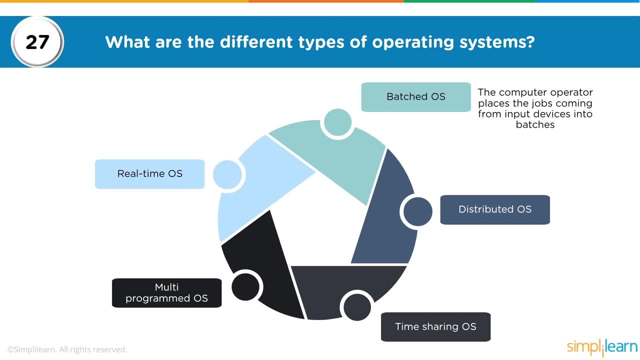 So when there are multiple processes coming in, multiple jobs that are going to be scheduled, a batched OS is going to place these jobs in batches and they are going to crunch those based on the inputs that have been given by these operators. Distributed OSS where there are multiple. 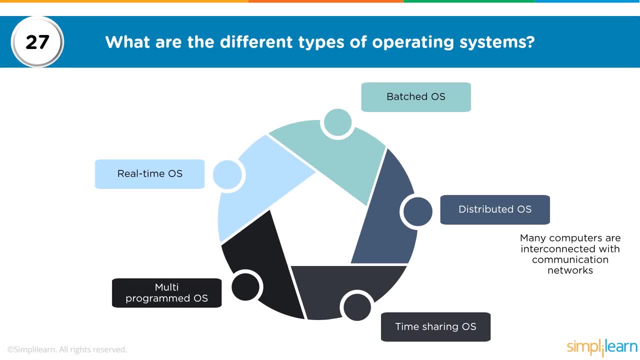 computers which are interconnected and are communicating through networks. So in a corporate environment you don't use one single computer to do everything. You've got a data center and the data center will have a cluster of servers where they are going to share some resources to crunch. 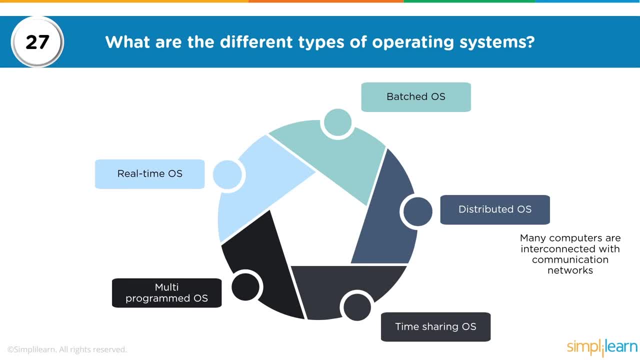 one particular task. So that's where your distributed OSS come into the picture. Then you have time sharing OSS where you are renting some time. So time sharing OSS minimizes the response time. Example: in today's world cloud. You go onto the. 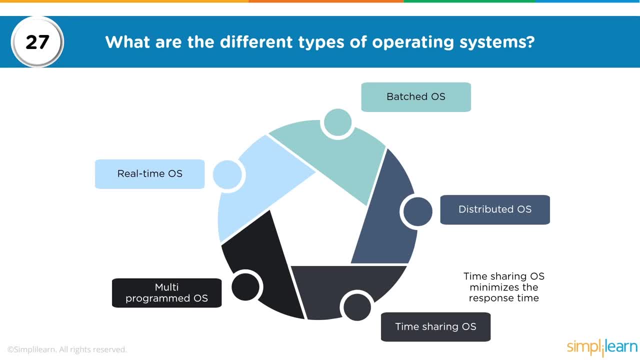 cloud. you have a virtual service over the. there you schedule something, you schedule a job over there it is executed and for that time being, that operating system services your particular request and provides you that particular job. Any application that you see online, that is executed, for example. 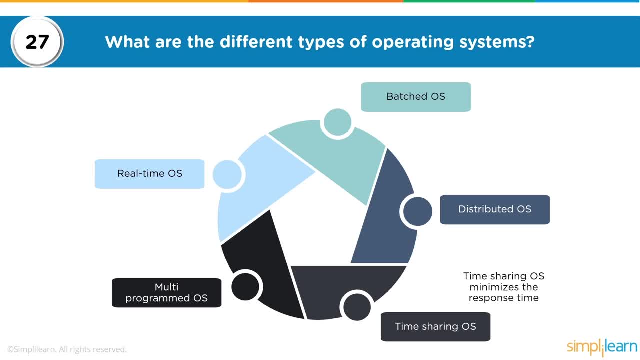 Facebook, from a consumer's perspective, could be a time shared experience. Then multi-programmed OSS: the operating system uses CPU scheduling to separate jobs. So you are scheduling the CPU to complete certain jobs in this particular manner and in real time. OSS. 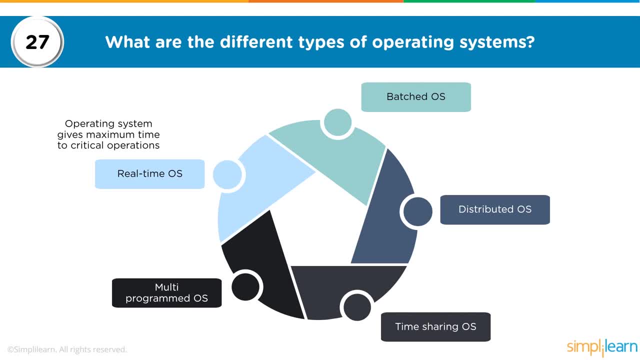 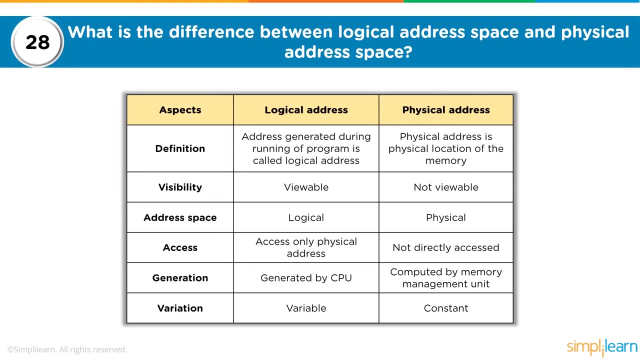 the operating system gives maximum time to critical operations. So it identifies the priority of these operations, it knows the high priority items, the medium low priority items and, based on that, it is going to execute these critical operations and get the job done. Moving on to the next question, what is? 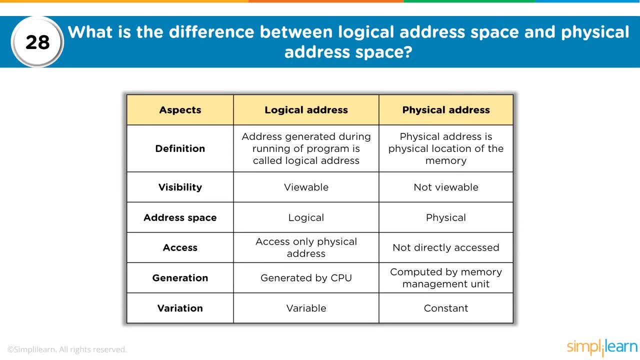 the difference between logical address space and physical address space. Now, when you are looking at address spaces, this is where applications come into the picture, and when you execute an application, it is going to create a particular address in the memory, where it is going to create a buffer. 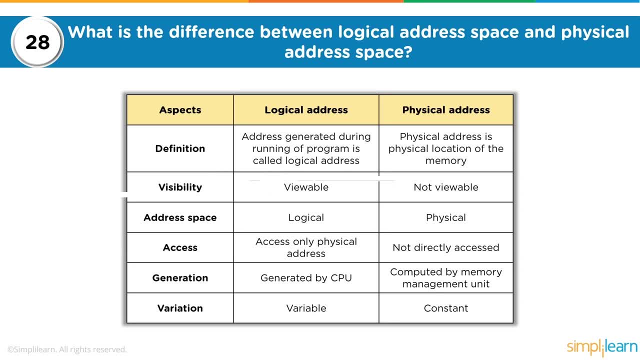 to store its own information so that it can be provided to the processor, processed and then can be returned back to the application as an output. So, as far as definitions are concerned, a logical address is generated during running of an application or a program, A physical address 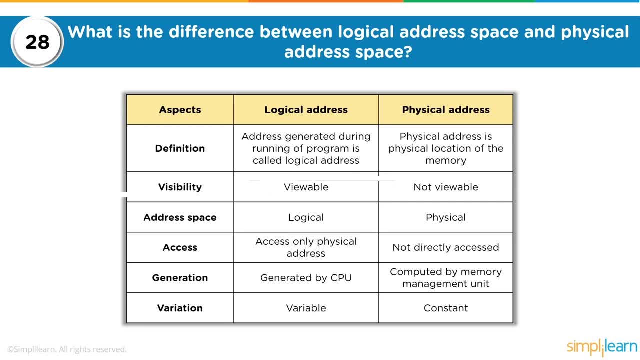 is a physical address or a physical location on the memory module itself. Right Visibility you can view a logical address because it is programmed into a computer. so if I am looking at C, C++ and I am using malloc or memory allocation, that is where the logical address is going to be. 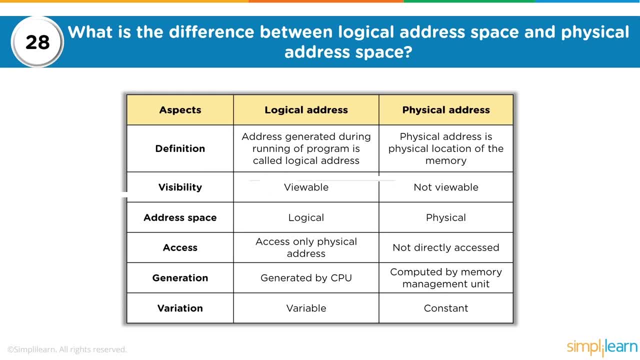 created where a buffer is going to be created for that program and whatever the user input is going to be, it is going to be stored in that buffer. But whereas physical address is concerned, this logical address will be created on a physical store or a physical memory module. 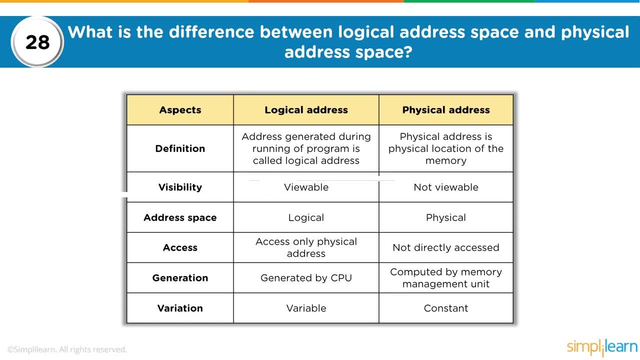 which will have its own addressing mechanism. Thus, you can see the memory module, but you cannot see the specific address on that particular memory module. But as far as a logical address is concerned, while you are programming or you are debugging the application, it will show. 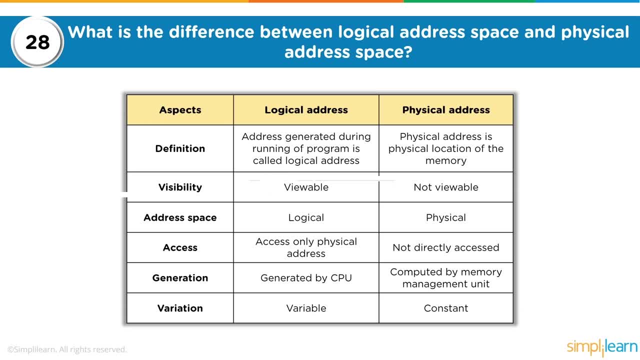 you the logical address that has been created, the start point and the end point of the logical address that has been created for that particular program, and it can be shown in a debugging environment. Address space, logical and physical address is physical, like I discussed, it is the memory. 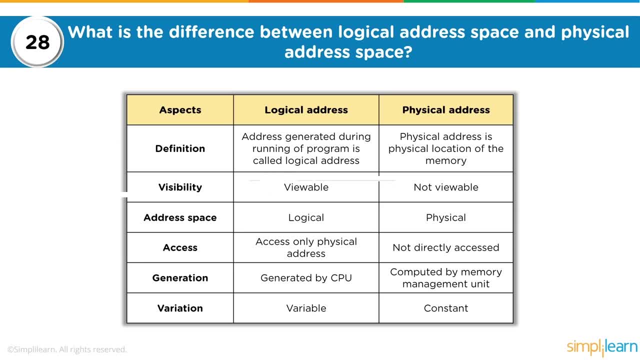 module itself. You can access only the physical address on that particular memory, because logical addresses can be viewed, but you cannot access them physically. Generation: the logical addresses are generated by the CPU during the processing time, whereas physical addresses are generated or computed by the memory management. 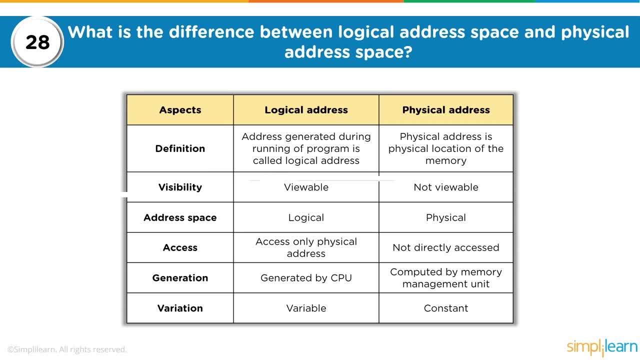 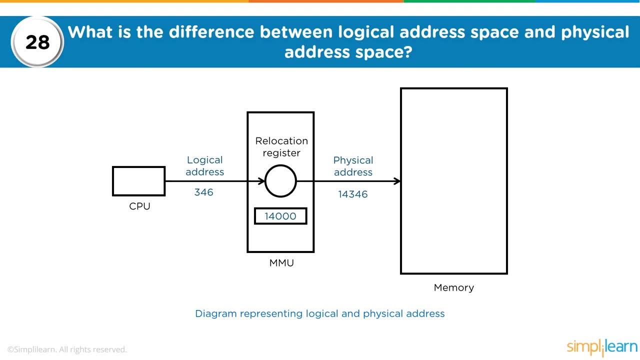 unit or the MMU that you have on your computers. And as far as logical addresses, they are variable, whereas the physical address is always going to be constant. Looking at the next question, what is the difference between logical address space and physical address space? So, moving on from the previous question to this, 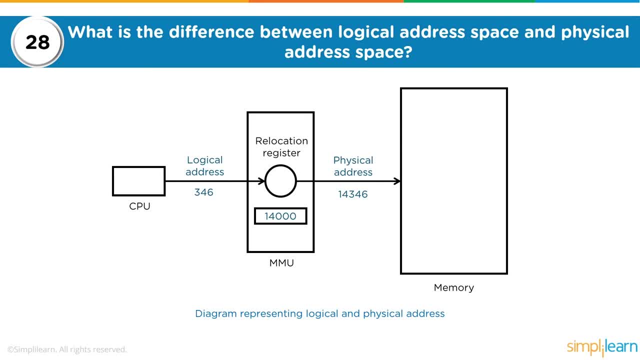 the logical address is an address created by the CPU for the processors that need to be addressed and that need to be stored as a buffer in the physical memory, Whereas the physical memory itself is going to be an address that is going to be there on the physical part of that memory. 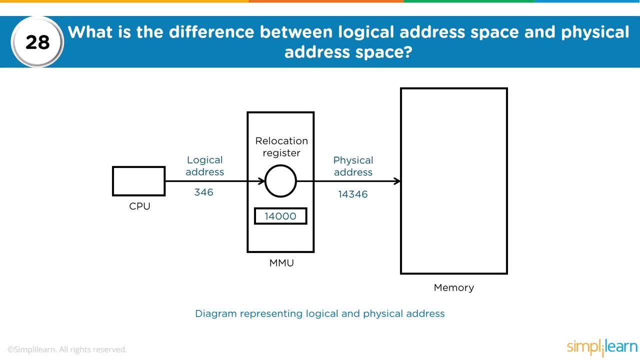 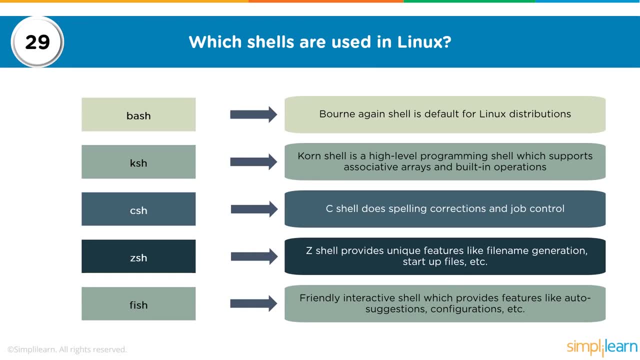 which is going to be assigned to it by the MMU. Then the next question discusses shells. So what shells are used in Linux? Now, what is a shell? Shell is the command line interface that we utilize on a Linux machine, So the terminal window, as we 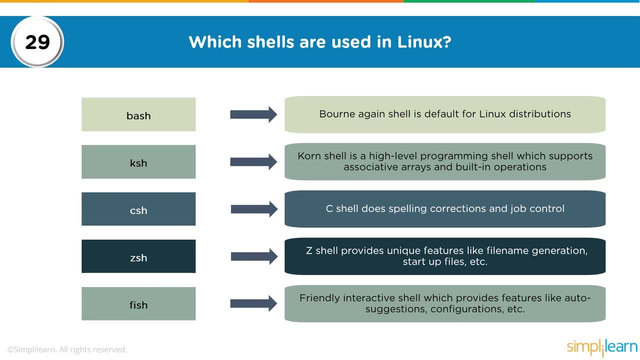 call. it is a shell And there are different variations of a shell based on what Linux operating systems you are using. The desktop operating systems that you use or the server operating systems in today's world that you are going to use normally, will always have a bash. 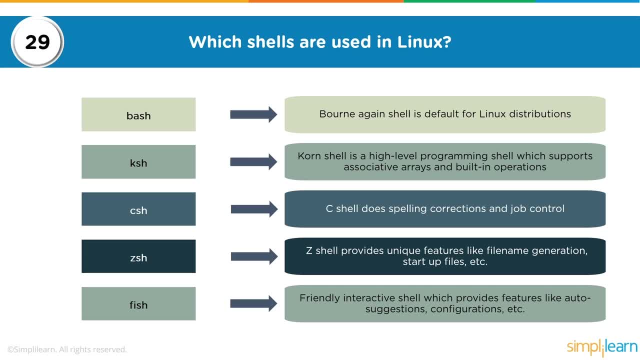 shell, which is the first shell that you see on the screen, Known as a born-again shell. it is a default for Linux distribution. So as far as end consumers- regular consumers- are concerned, it is always going to be a bash shell, a born-again shell. 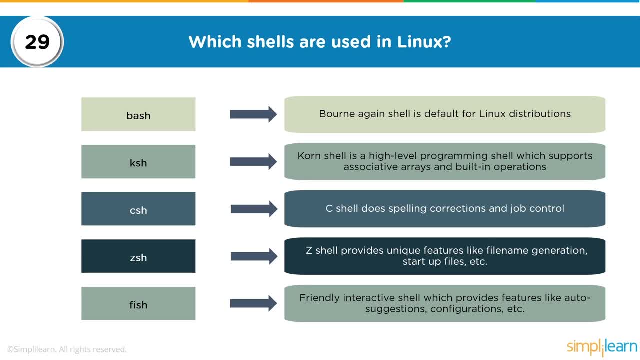 that you are going to utilize for scripting and to execute regular commands. But when it comes to high level programming or it comes to specialization tasks, then you got the rest of these shells that you can utilize, For example, the KSH, known as a con. 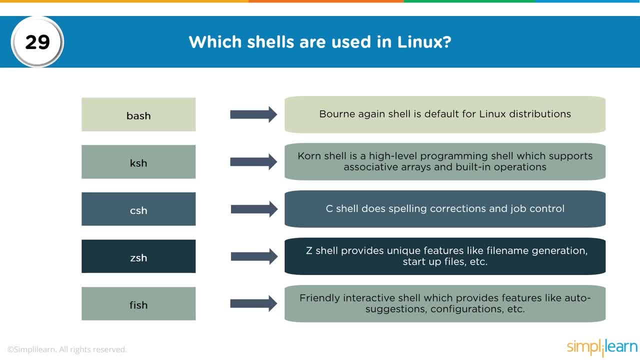 shell is used for high level programming which supports associative arrays and built-in operations. The CSH or the C shell has different functionality like spelling corrections and job controls. The ZSH or the Z shell provides unique features like file generation, startup files and FISH friendly. 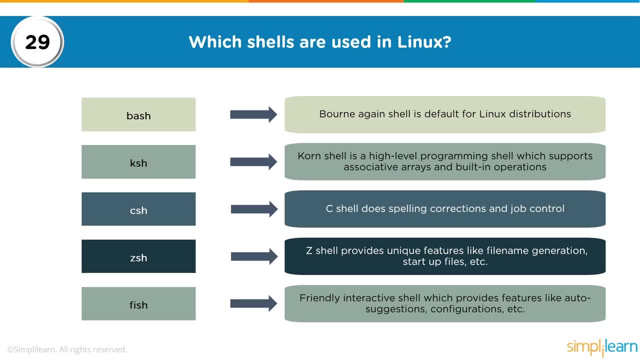 interactive shell which provides features like autosuggestions and configurations. So all of these have different functionalities depending on what usage that you have for that particular shell. The most common shell, like I stated, is the bash shell that you will always come across in your desktop Linux operating. 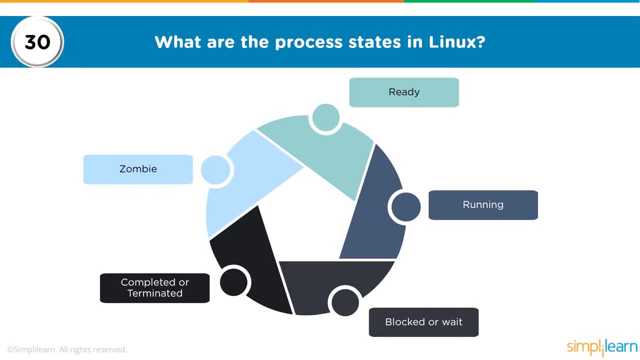 systems. Then, looking at the next question: what are the process states in Linux? Now, what is a process? Process is basically a service that is running for a particular application. for that application to function, This process is going to direct user input to the processor process. it. 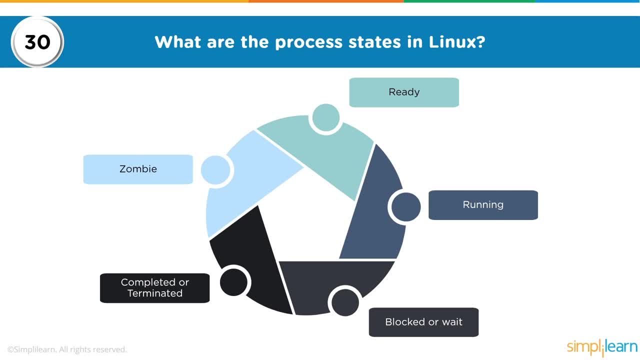 get that output back to the application, execute it and then show it onto the graphical user interface for the user. So in Linux there are five states for a process. First is the ready space. Now in ready. in this state the process is created. 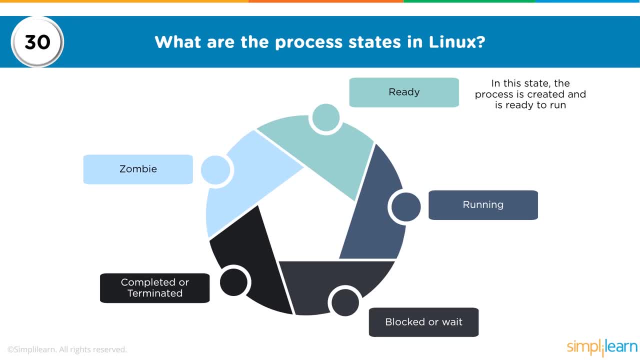 and it is ready to run, So it is waiting for input. It's ready, the application is executed. The running is when the process is being executed itself. Blocked or wait is when user input is being looked upon. So it's waiting for user input so that it can. 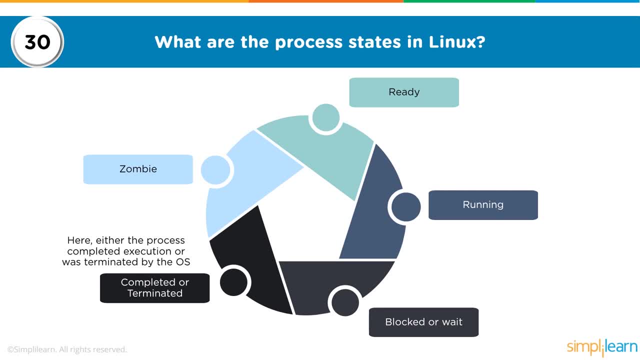 do the processing Completed or terminated? it has completed its execution or was terminated by the operating system for some reason or the other. So this is where things have: the processing has been completed And the last state is zombie, where the process is terminated. but 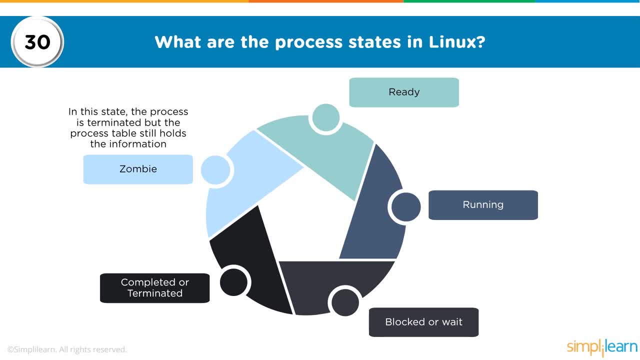 the process table still holds the information, or maybe it is waiting for the kill request before it gets terminated. So these are the five states for a Linux process to be in. And that brings us to the 10 questions in the operating system and application space In the next. 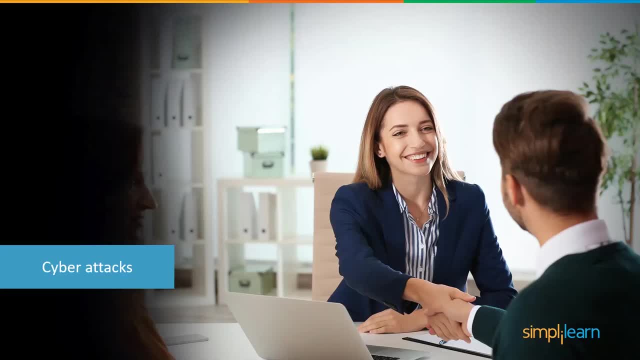 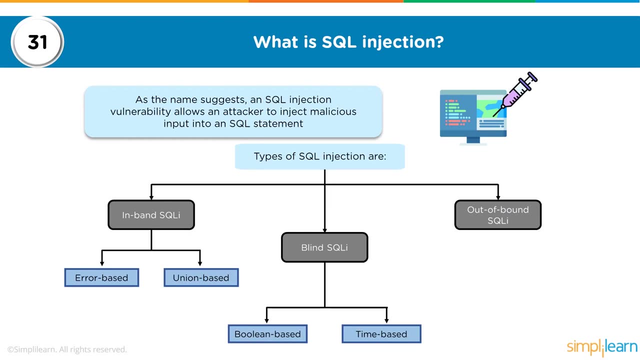 video. we'll be looking at 10 more questions on cyber attacks. Interview questions based on cyber attacks. Let's start off with the first one. The first question is: what is SQL injection? SQL stands for structured query language, which is a language that is. 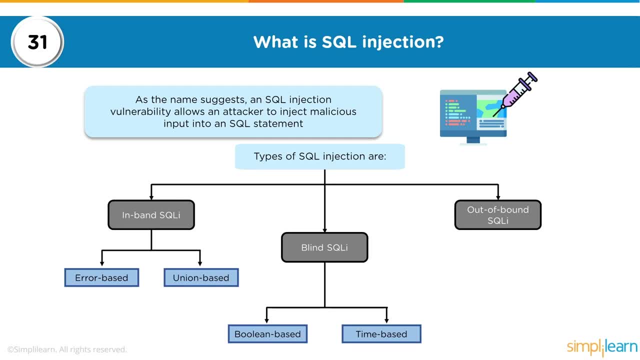 used by most of your databases or your relational databases. The variations of your database would be MySQL, Microsoft SQL, Oracle SQL. You'll have IBM databases. All of these databases utilize the structured query languages to interact with the applications. Now, all of these, 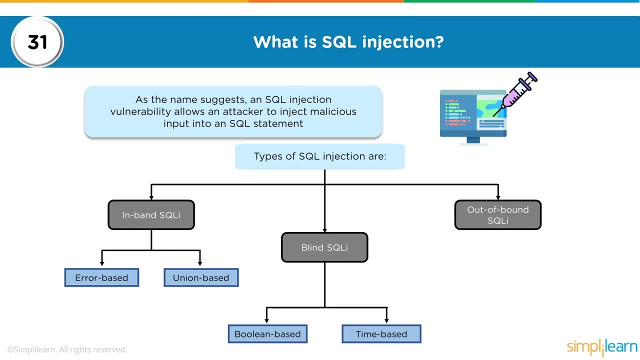 databases have their own syntax, so you'll have to study most of these databases based on which applications and which databases you want to provide security for. But, as the name suggests, SQL injection vulnerability or structured query language injection vulnerability is where a user can maliciously inject. 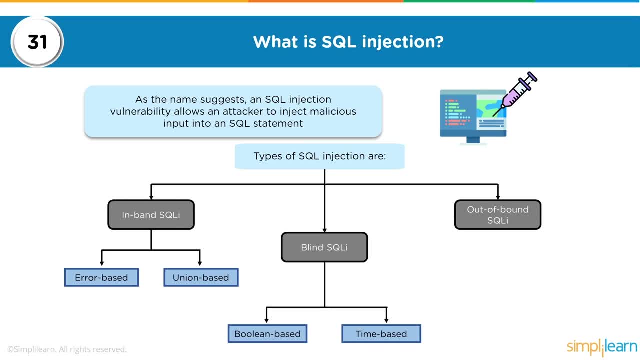 a SQL input or a SQL statement in a query and send it to the database and evoke a response out of it. So this vulnerability is not specifically to the database. The vulnerability lies more in the application and the coding of that application. So when the application receives a query, 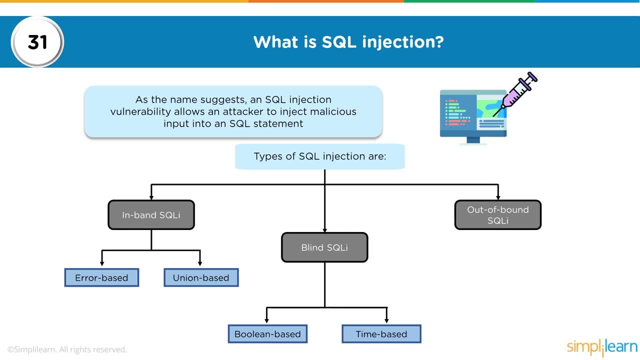 which it needs to be forwarded to the SQL database. we need to configure and the application needs to know at what level of what queries are allowed and what queries are not allowed. So there are different, various aspects of how to manage a SQL injection vulnerability. 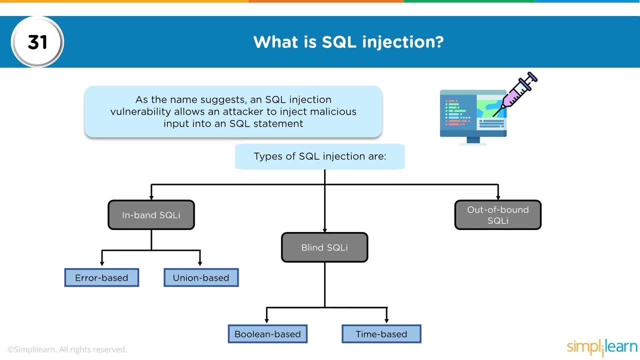 But the basic flaw lies in the application, where invalidated input is accepted and sent forward to the database, where the database might confuse it into an executable statement and thus create a response that was not warranted. There are various types of SQL injections, As shown on the screen: in-band SQL injection. 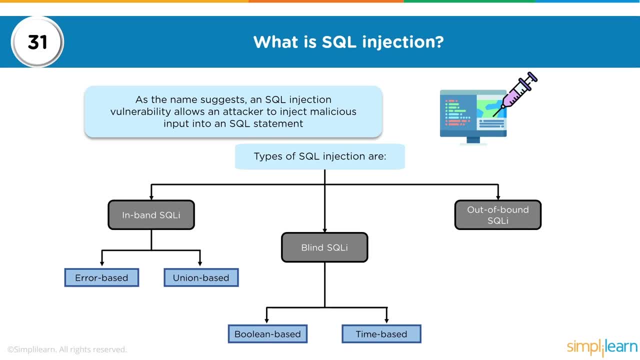 where you can look at an error-based or a union-based injection, a blind SQL injection where it is either Boolean-based or a time-based attack, and then an out-of-bound SQL injection. Essentially, you're looking at databases and you're looking at application security where you want to. 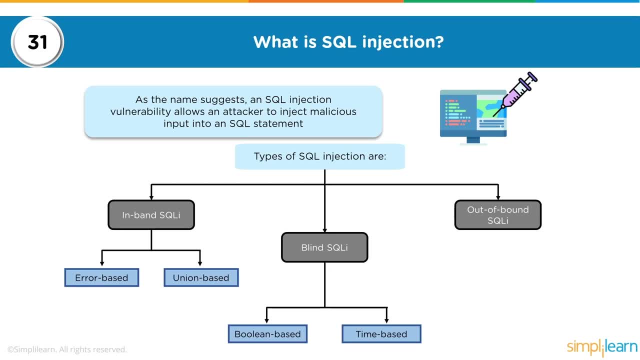 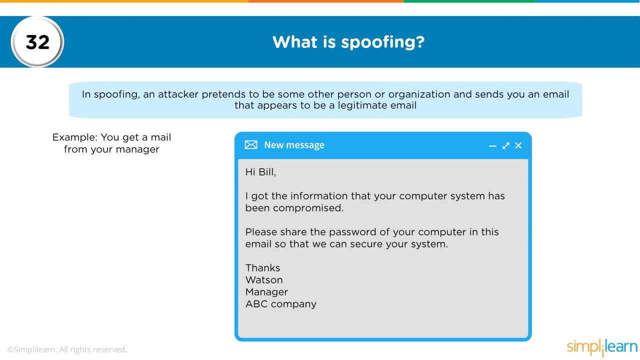 encourage secure coding practices so an unvalidated input is mitigated. The next question is: what is spoofing? Now, in spoofing, you're basically assuming the identity of another person. So here the attacker pretends to be some other person or an organization and sends you an. 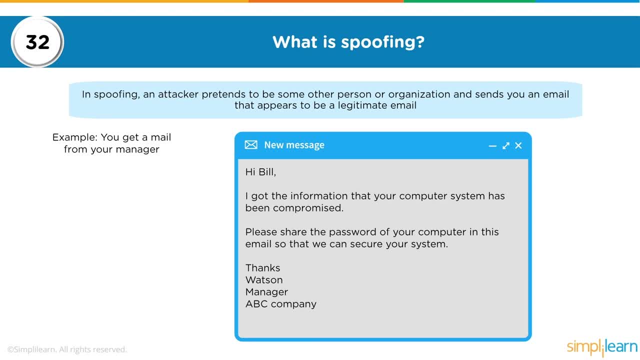 email that appears to be a legitimate email. It looks almost genuine. It has been constructed to replicate what a genuine email would have been, and it is very difficult to spot a fake one. There are different ways to identify whether an email is genuine or not. 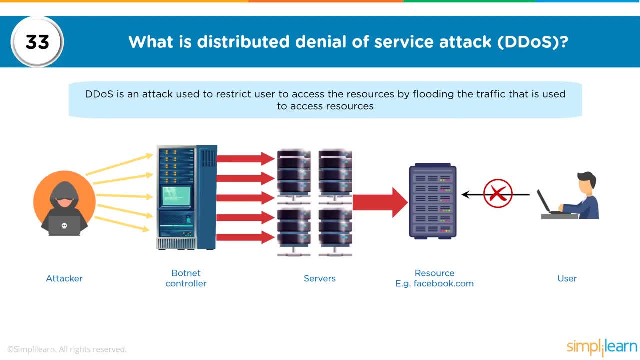 but that's for a different video. Moving on to the next question, what is a distributed denial of service attack or a DDoS attack? Now, generally, a denial of service attack is an attack where legitimate users are prevented access to the resources that they legitimately can access. 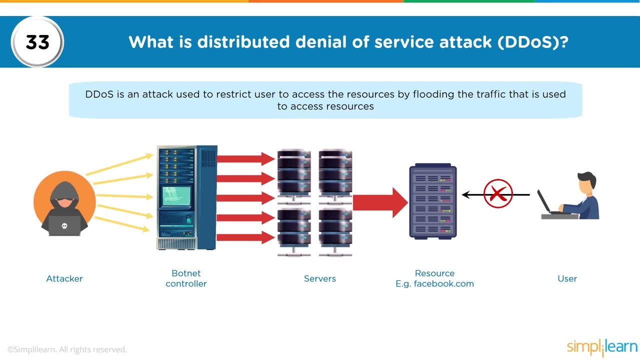 So, for example, if it is a bandwidth-based attack, the attacker consumes the bandwidth of the network in such a way that there is no more bandwidth left for legitimate users to access the network. Now, a single device may not be able to generate that much amount of. 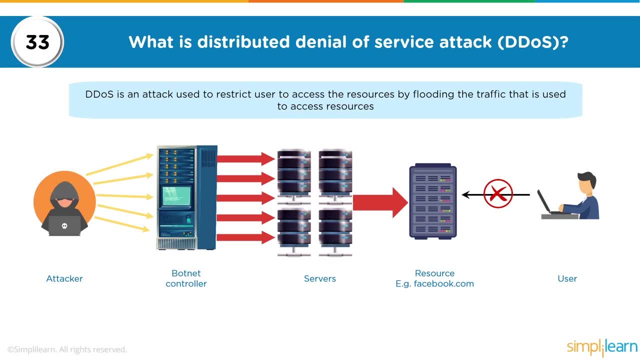 traffic to consume the bandwidth of a huge server. Thus the attacker will construct a botnet and through that botnet they will launch a distributed denial of service attack to the target victim. So a botnet. there are two terms that we want to look at over here. The first term: 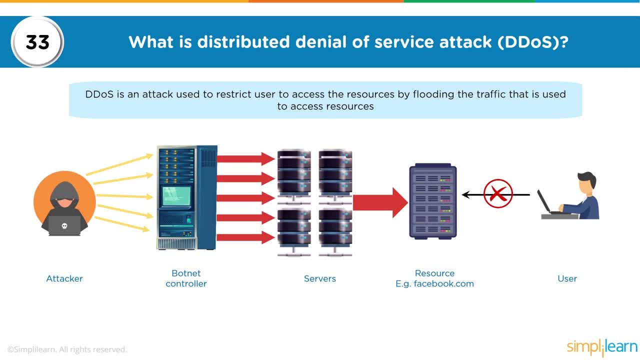 is a bot, and the second one being the botnet itself. Bot is a software that, once installed on a victim's machine, allows the hacker to send remote commands to that machine. that will make it generate some activity Once we have enough machines on which such bots. 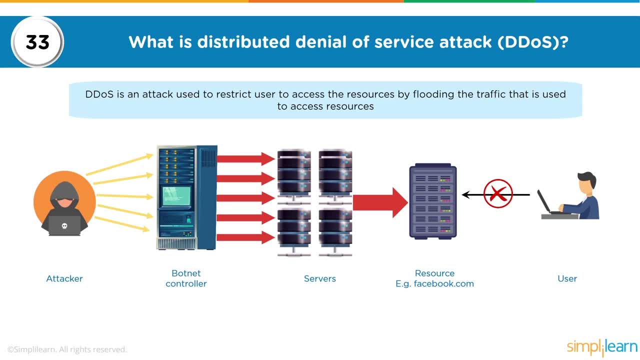 have been implemented. the collection of these machines would be known as a botnet, So an attacker would then instruct this entire botnet to start generating data traffic to be sent to the targeted network or to the targeted server, which will then bog down the server, thus crashing. 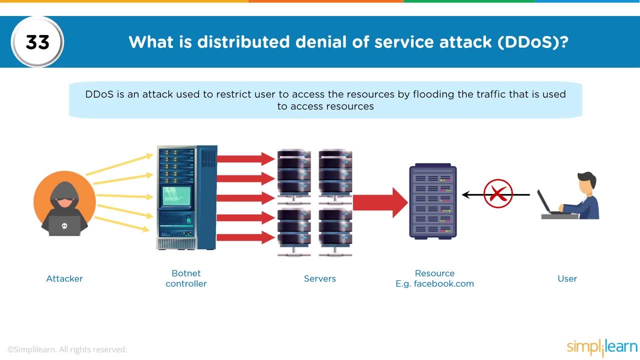 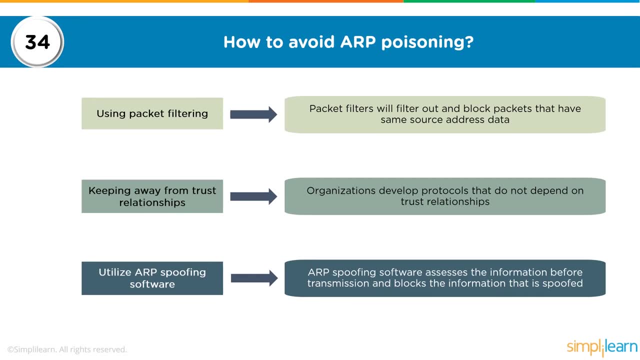 it and preventing users from accessing that particular resource. The next question is how to avoid ARP poisoning, or ARP. Now, first let's understand what ARP is. ARP stands for address resolution protocol, which is a protocol used by computers to communicate over the network Once your computer boots up. 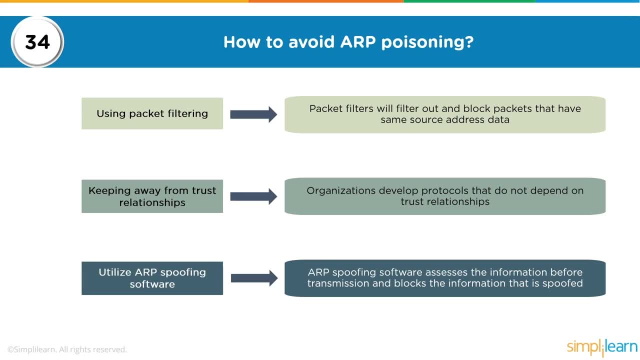 it starts a discovery process of identifying its neighbors. So if I am in a particular subnet, my machine will proactively send out ARP requests and address resolution protocol to find out which other machines are within the same network and which are live. Once it sends out a query, a live machine will respond. 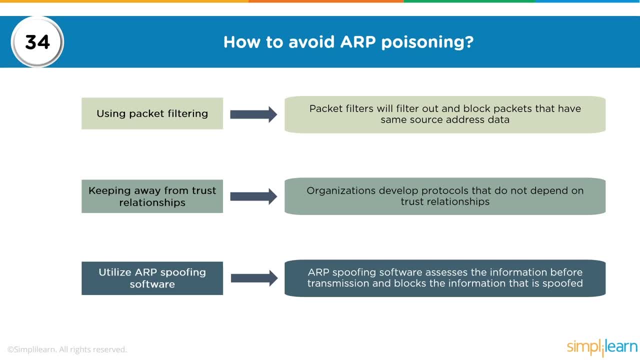 to that query, along with its MAC address. This information is then stored in what is known as an ARP table, or an ARP table, on the machine's cache. So whenever my machine now wants to send out a packet to this particular machine, it will go to the ARP table. it will identify. 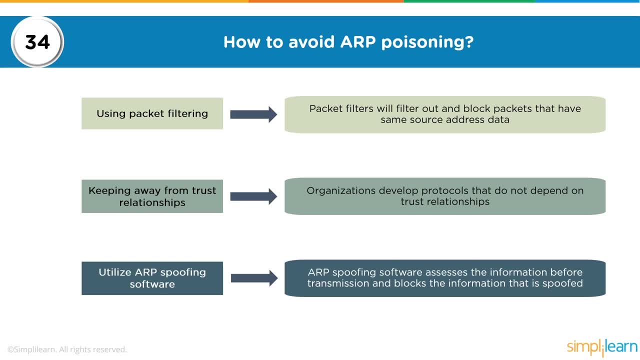 the IP address and the associated MAC address. It will print that onto the data packet as a destination IP and destination MAC and send that packet across to the switch. The switch will then identify the MAC address and send the packet to the relevant machine that is connected to that particular switch. 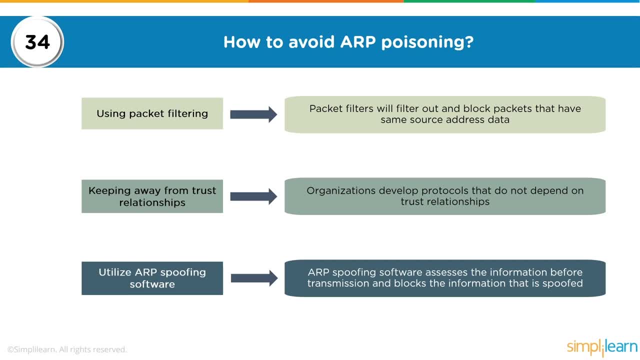 Now to confuse this switch into sending it to a different machine, our poisoning attack is created. This attack is generally launched to create a man in the middle attack. Now, to prevent this ARP poisoning from happening in the first place, there are three different aspects that we can utilize. First, we can 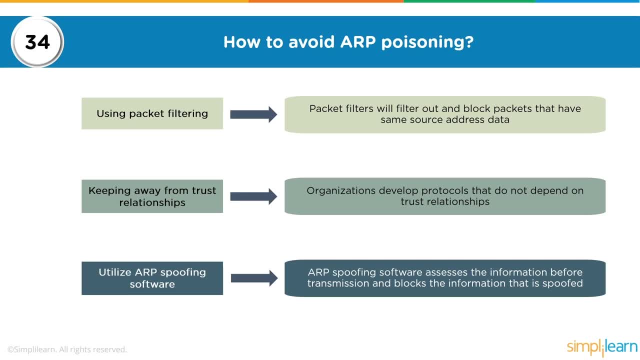 use packet filtering, which will filter out and block packets that are the same source address data. so you have identified some malicious IP addresses and you want to block out some IP addresses. so you are using a packet filter firewall, where you have instructed the firewall to filter out certain packets. 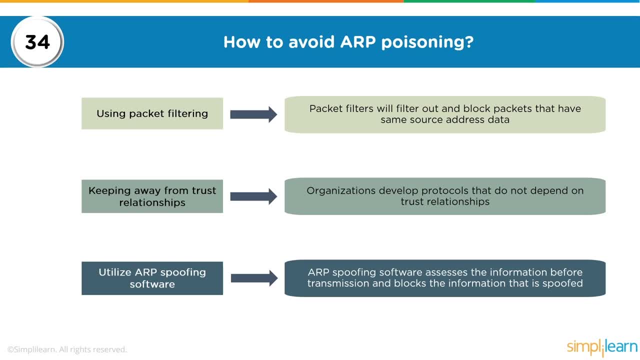 originating from particular range of IP addresses. This firewall and this technique will then block those kind of packets coming in. Second, keeping away from trust relationships. Organizations will develop protocols that do not depend on trust relationships, and thus you want to keep this protocol away from that Once you. 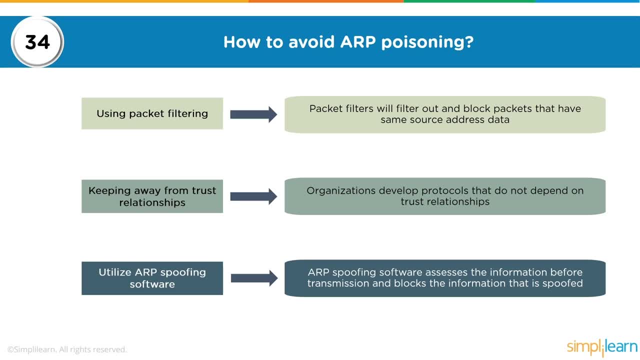 have created a trust relationship, these machines should not be sending out ARP requests to other machines in the first place. since the trust relationship has been defined and these machines know whom to communicate with, such kind of protocols should then be disabled, Or you can use ARP spoofing. 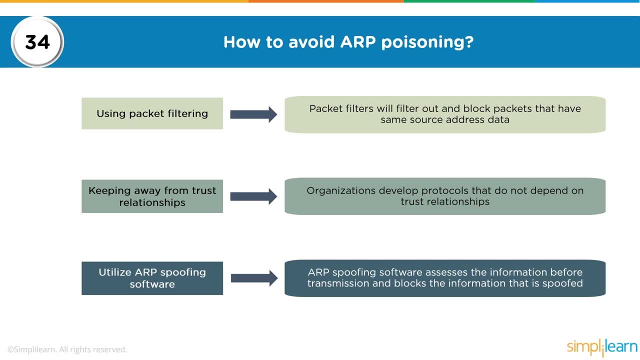 software. So there are some softwares out there that will look for ARP spoofing and prevent that from happening in the first place. So if somebody has sent out a spoofed ARP packet, that packet will be picked up by this software and it will be mitigated. 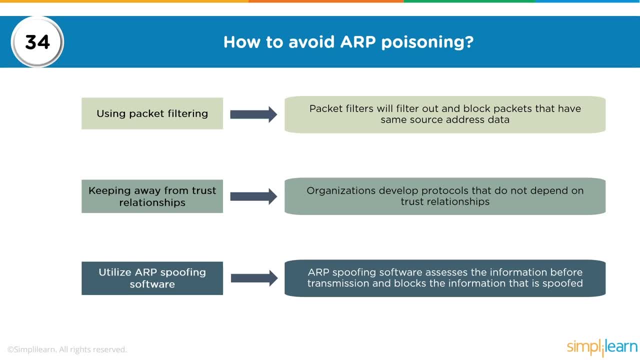 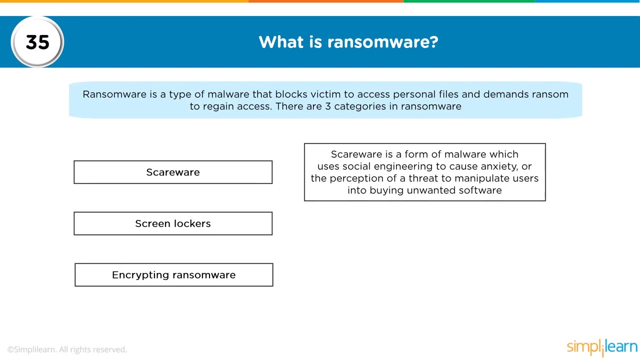 Network visualizers like GlassWire, antiviruses like Sophos. they have inbuilt capabilities of identifying ARP spoofing attacks and mitigate them in the first place. In the next question, we are going to discuss what is ransomware? Now, ransomware is a type of malware. 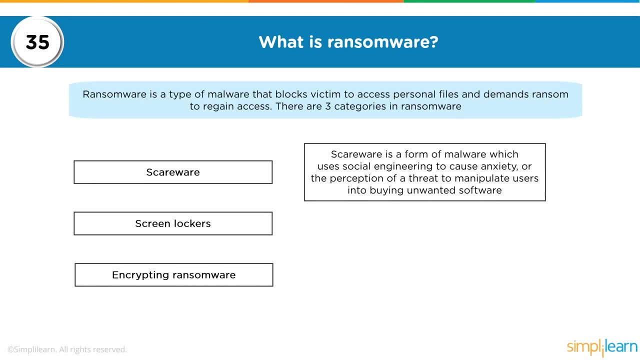 that blocks victims to access personal files and demands ransom to regain access. There are three categories. Before we go into the categories, let's just revisit what ransomware is. Let's start with the word malware. Malware is a malicious software that poses as a legitimate software. 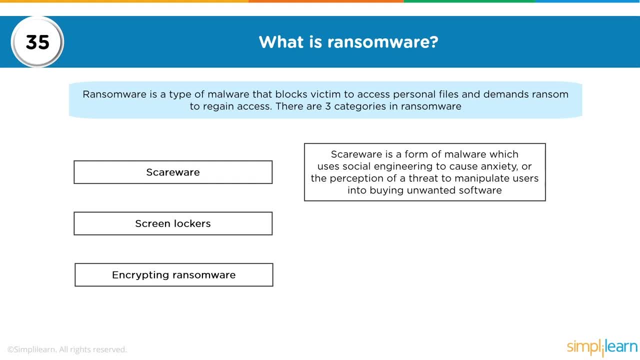 but has a payload that will have a security impact on your machine. So in this instance, viruses, trojans- all of these can be classified under malwares. So can ransomwares. A trojan is a software that will give you a backdoor. 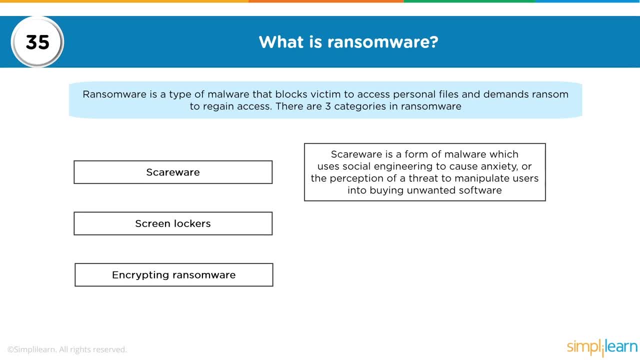 access to a particular device, A virus will do some destructive activity on that device. A ransomware will basically encrypt the data of that particular user on that particular machine, thus rendering that data inaccessible to the users themselves, And in turn will demand a ransomware. 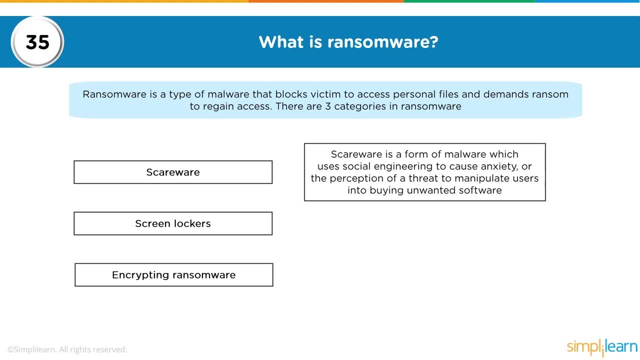 to provide access to that particular data. So the three types of ransomwares: the first one is scareware, which uses social engineering to cause anxiety or the perception of a threat to manipulate users into buying unwanted software. So this preys on the gullibility of humans. 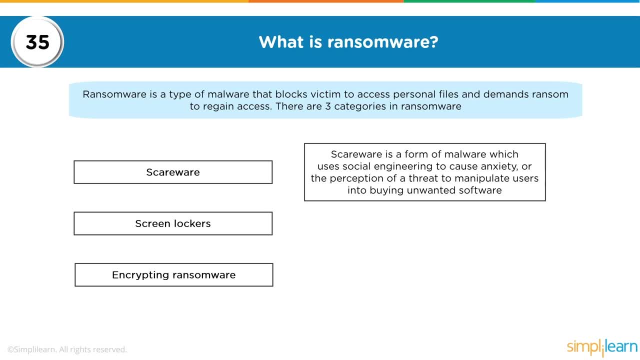 where you can see a pop-up appearing on your screen which can scare you into believing that you may have been attacked or there is a virus on your machine and then instructs you to download a particular software to mitigate that particular virus. Now the malware will be. 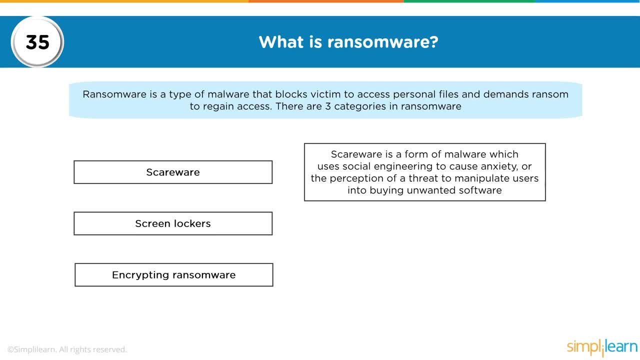 in this software that you will be downloading and then a ransomware will be installed and your data will be encrypted. Screen lockers: where locking users' computers by preventing them from logging in and displaying an official looking message. You will see a screen saver once you boot up. 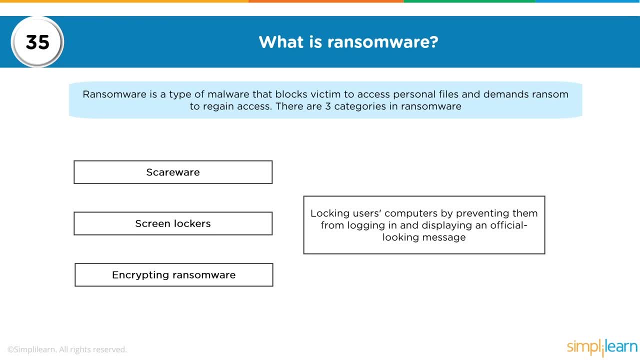 which prevents you from accessing the login page. so it will not allow you to log in to your own machine, but it will give you a warning that your data has been encrypted and you need to connect to a particular email address and send bitcoins over there to get a. 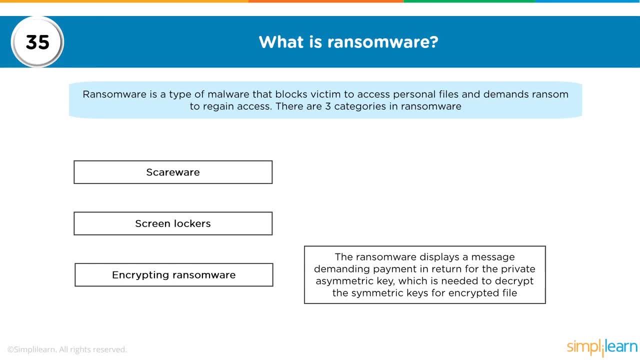 decryption key to access your own data, And then the encrypting ransomware displays a message demanding payment in return for the private asymmetric key which is needed to decrypt the asymmetric keys for encrypted file. So once your files have been encrypted, you might just have a blank screen. 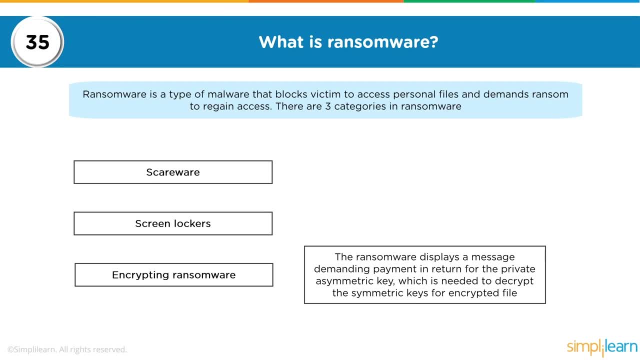 in front of you where you will receive a warning message where it instructs you to pay up a ransom in bitcoins or in some crypto currency to some particular digital e-wallet which is not traceable, and once you make that payment, they will send you the decryption key. 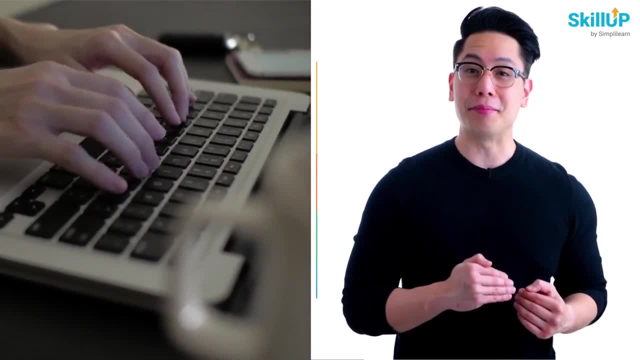 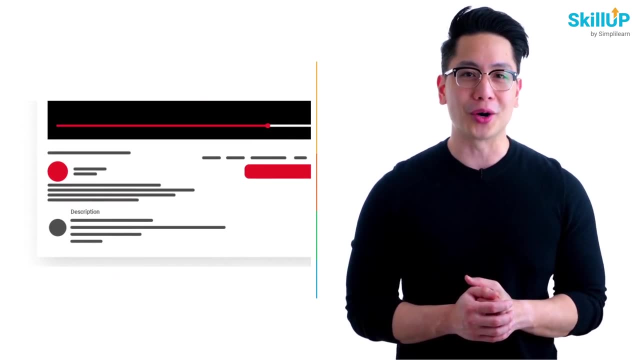 and then you can access your data. If getting your learning started is half the battle, what if you could do that for free? Visit SkillUp by SimplyLearn. click on the link in the description to know more. Then talking about the next question: what is the difference between an active 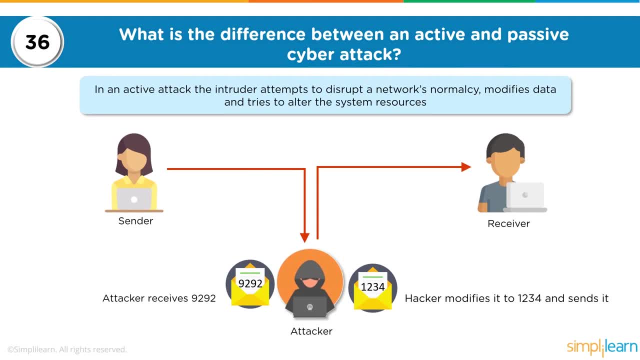 and a passive cyber attack. Now, when we talk about cyber attacks, cyber attack is activity that is caused by a malicious user who wants to try to get access or do some security incidents on the victim's devices. So there are two ways that can happen. It's either in an active 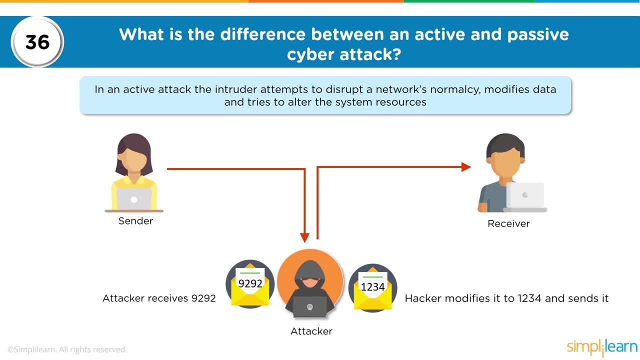 manner or a passive manner. In an active manner, they include an attempt to disrupt a network's normalcy, modifies data and tries to alter the system's resources. So this is more active, where the attacker will proactively try to destroy the network so that communications fail. 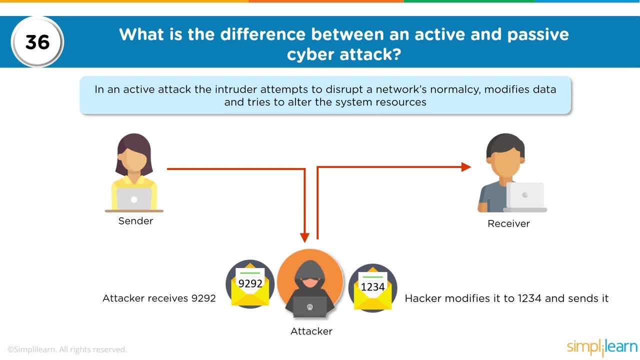 or they might try to modify the data where, using a ransomware, they can encrypt it, or they might delete that data using a virus, or steal that data using a trojan, or they might even alter the data so that it is no longer trustworthy, Whereas in a 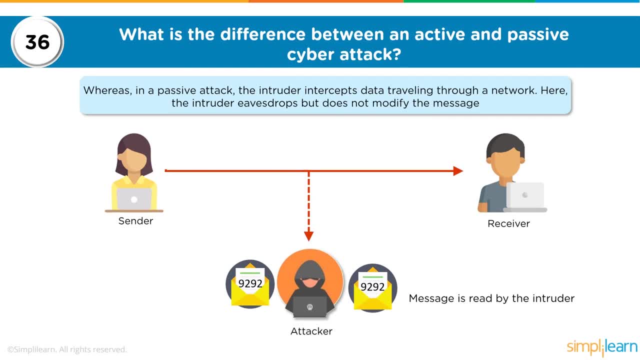 passive attack. the intruder intercepts data travelling through a network. Here the intruder eavesdrops but does not modify the message. So they're just listening in. they're just observing what is going on. they're not manipulating the data, they're not stealing. 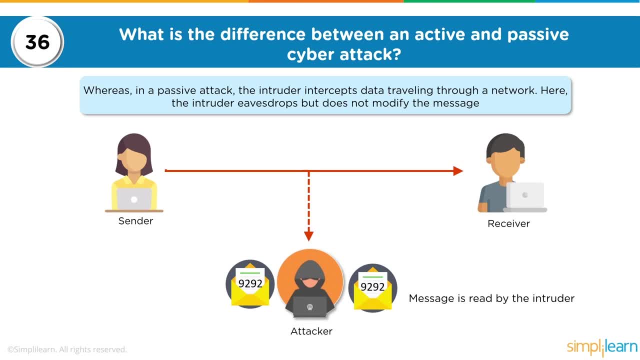 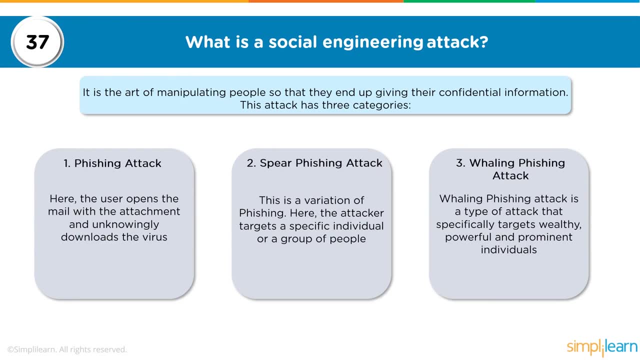 anything. It's just that they are monitoring the activity that's going on. Then the next question: what is a social engineering attack? Now, social engineering attack is a people based attack. The victim here is the human by itself. The vulnerability also lies in the human It. 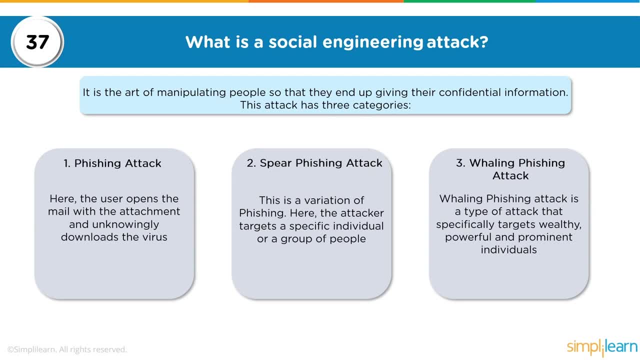 may be executed through a computer, but end of the day, the gullibility is of the human. So it is the art of manipulating people so that they end up giving up confidential information. Now we always read in the papers where somebody got manipulated: their passwords got hacked. 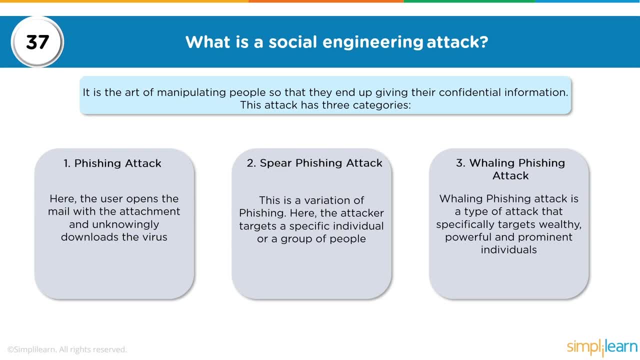 and somebody's life savings got wiped out right because they shared the OTP with someone or they shared the password with someone. Now creating a scenario where these people will fall prey to this attack and share this kind of personal information to unknown people- that is where the social engineering attack comes in. 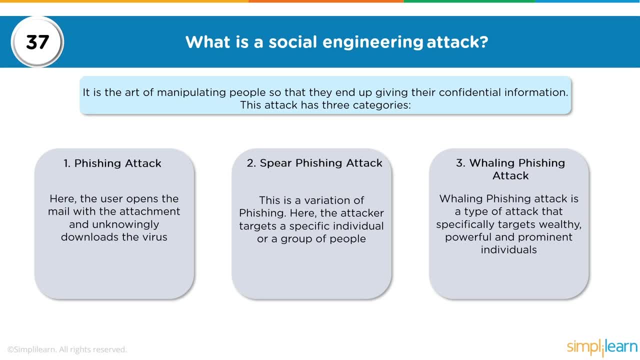 Creating that scenario which will ensure that these people give out this confidential information. Now, there are three categories in this attack. The first one is a phishing attack, second is a spear phishing attack and a third is a railing attack. Now, phishing attack is basically a generic attack. 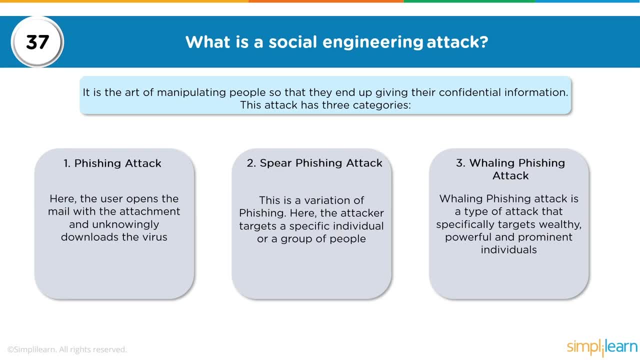 It is targeted to the world at large. Whoever falls prey to that attack will be a victim, Whereas a spear phishing attack is a targeted attack towards a specific individual or a group of individuals or towards an organization. So there is a lot more research that goes into spear phishing. 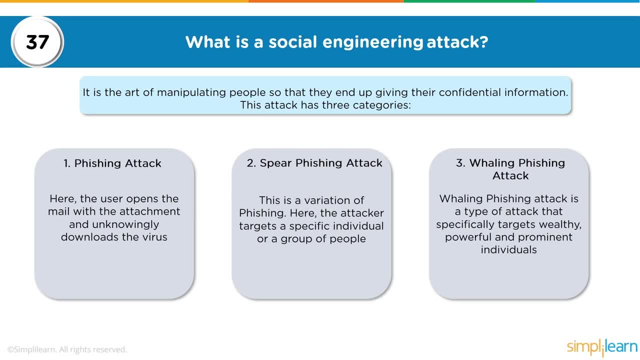 where you analyze the victim, you try to figure out what their vulnerabilities are and you tailor, make or you customize the attack to that particular vulnerability. Once you have that attack, you launch it against those people. Those people will then fall prey to this attack And a railing attack. 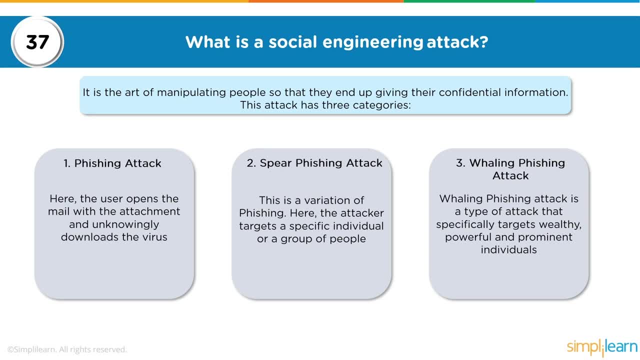 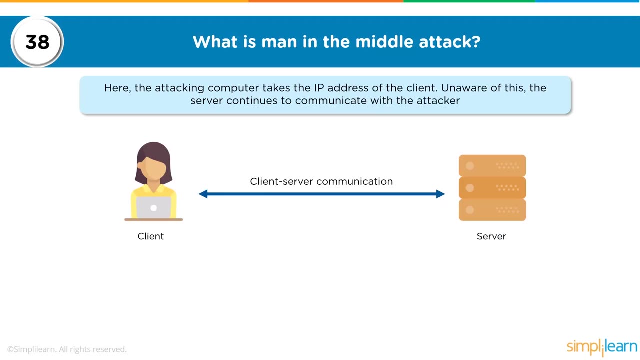 is where you are attacking top level executives, So the C level executives of an organization, politicians, movie stars, wealthy and powerful people. So any of these people, when they are attacked, it will be known as a railing attack. Next question: what is man in the 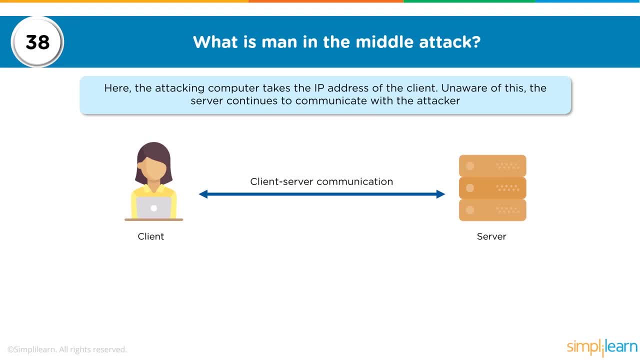 middle attack. Now, this is something that we had touched base when we talked about ARP, where the ARP poisoning attack needs to be executed to leverage a man in the middle attack. Now, in the man in the middle attack, the attacker attacking computer takes the IP address of the client. 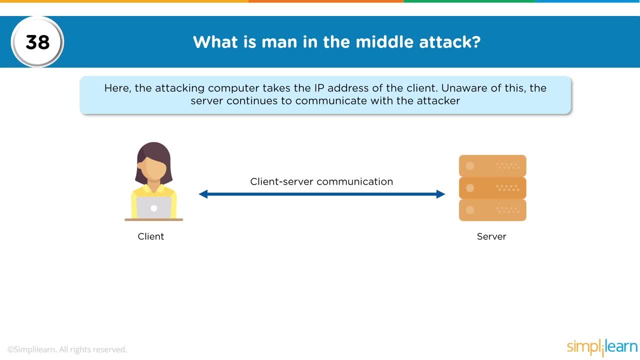 unaware of this, the server continues to communicate with the attacker. Now, if you remember, in a previous question we have also talked about spoofing. So in this scenario, attacker has spoofed their IP address to replicate themselves as a genuine client and now, with that spoofing in mind, they might 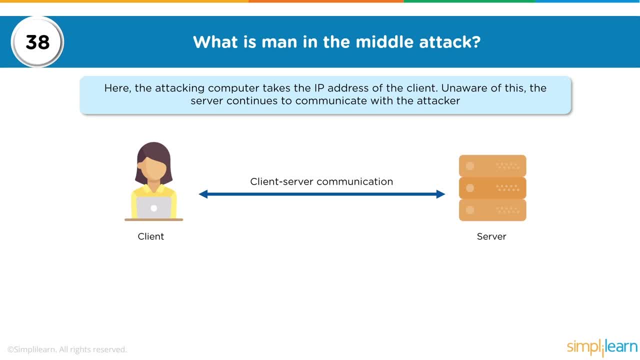 either through an ARP poisoning attack or just because of the spoofed IP address, become a man in the middle. That means that they are now eavesdropping on the conversation between the actual client and the server by posing themselves as a server In this scenario. 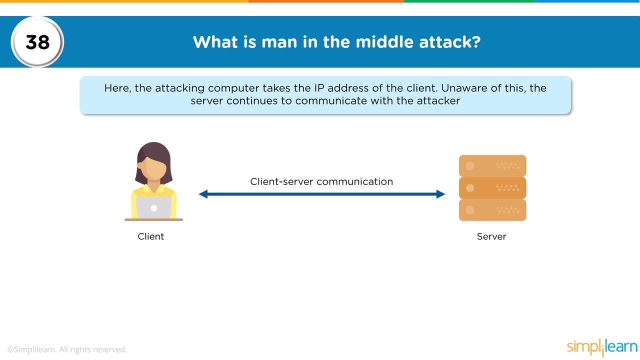 the attacker is now a go between between the client and the server and can eavesdrop and can copy the data if they want, and they can modify the data as well. So, as you can see on the screen, the attacker becomes man in the middle, which means that they are now. 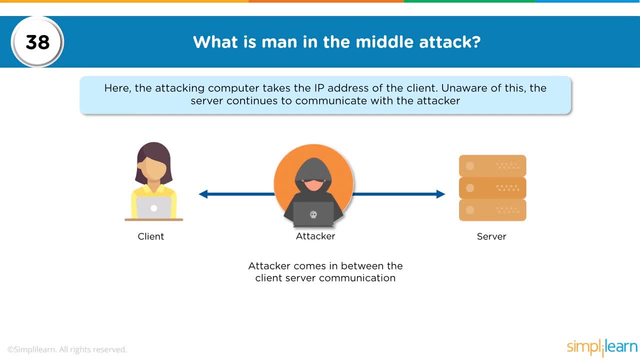 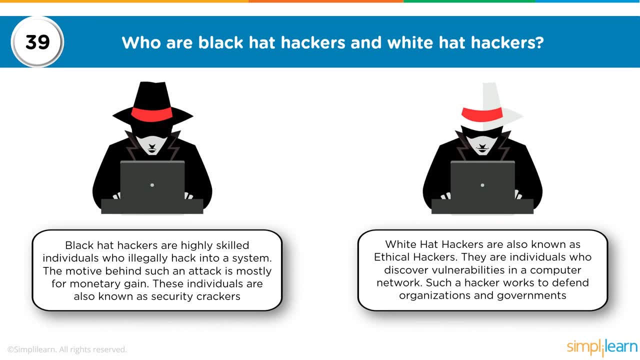 eavesdropping on the conversation that is happening between the client and the server. The next question: who are black hat hackers and white hat hackers? The main thing is the differentiation between a black hat hacker and a white hat hacker. Now, black hat hackers are skilled individuals. 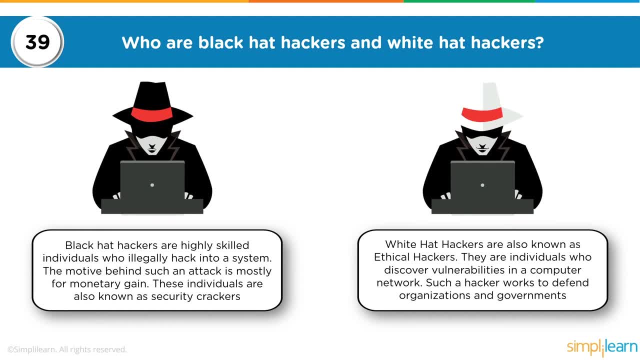 who illegally hack into a system. The motive behind such an attack is mostly for monetary gain. These individuals are also known as security crackers. Now, if you look at your criminal hackers- those who have malicious intent, those who do hacking for the intent of 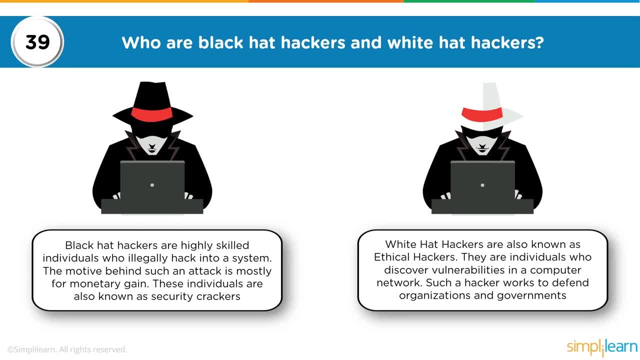 personal gain or for the matter of disruption. The main thing that black hat hackers lack is authorization. They are not authorized to do the activity that they are about to do, and they are going to get unauthorized access to devices or to data, which is going to cause losses to the organization. 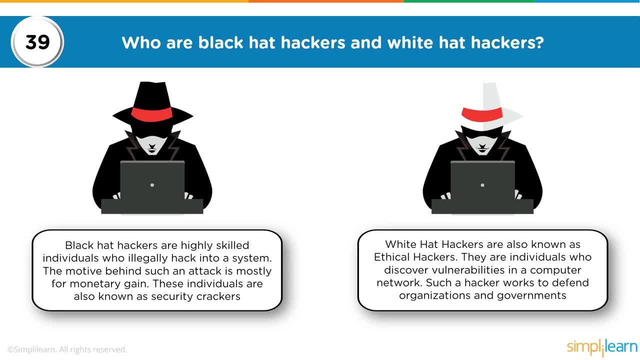 involved, Whereas on the other side, a white hat hacker are also known as ethical hackers. These are the individuals who discover vulnerabilities in a computer network and they help the organizations mitigate these vulnerabilities. They help the organizations defend themselves from black hat hackers. So the main difference between these two. 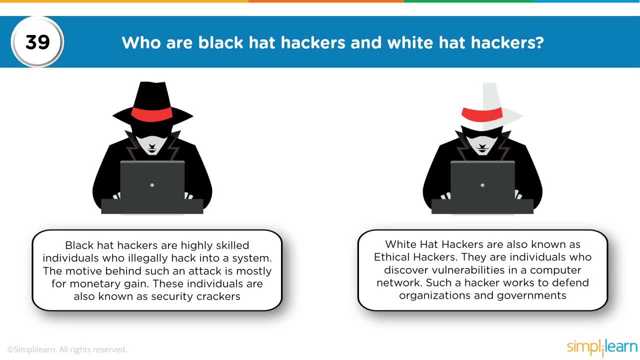 types of hackers. a black hat and a white hat is the intent and the authorization. So black hat hackers will have malicious intent. They will try to personally gain from that attack by finding out vulnerabilities. They also will not have authorization to conduct whatever activity they are doing. 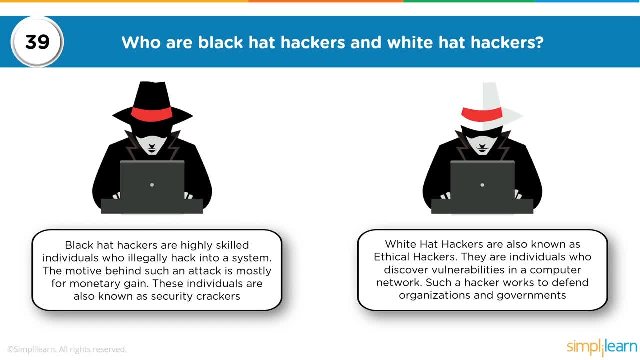 Whereas on the other side, white hat hackers will be hired by organizations. They will provide authorization for certain activity that the white hat hacker can do to find out those vulnerabilities. Once those vulnerabilities have been found out by the white hat hacker, they will report it. 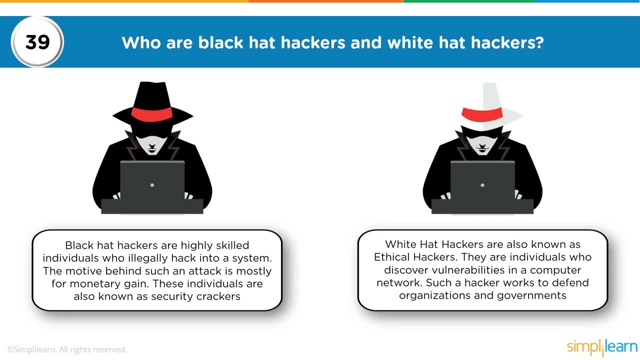 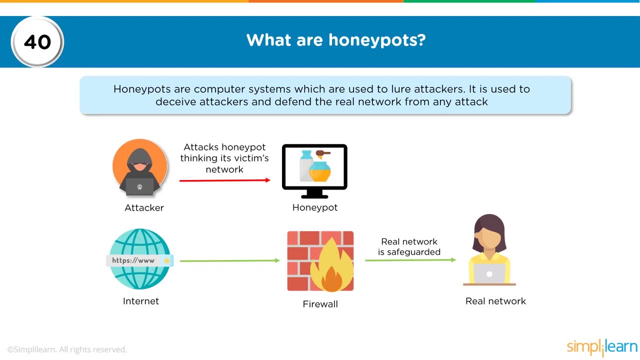 to the management and guide them in implementing security controls to mitigate those vulnerabilities. The main difference between a black hat and a white hat is the authorization and the intent. Next question: what are honeypots? Now, honeypots are a very interesting device that can be introduced in a network. 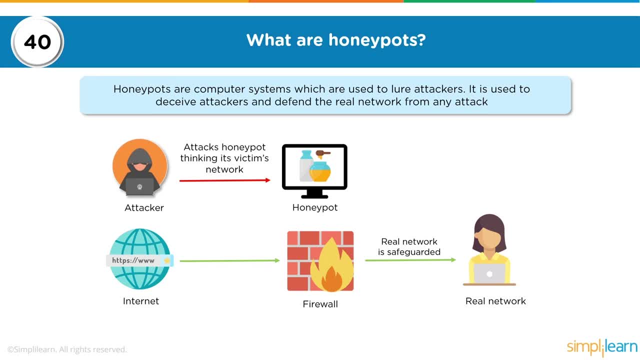 These, basically, are decoy servers that are implemented in a network to attract the attention of an attacker. It is there to lure an attacker into attacking that particular device, thus creating a security blanket for the rest of the devices. So if an attacker has been able to 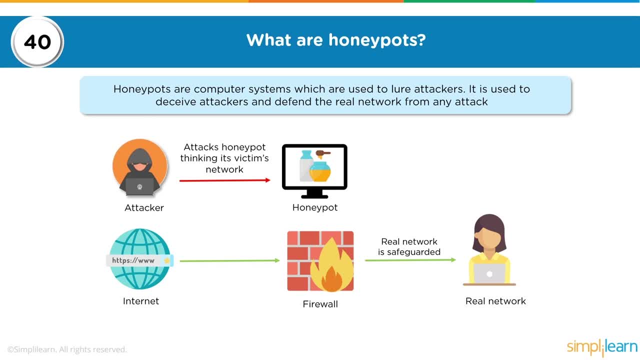 bypass a firewall and is now trying to scan a particular network. when they scan, they will come across various devices that are there in the network. They will then proceed to do a vulnerability scan on these devices- The honeypot- at that point in time. 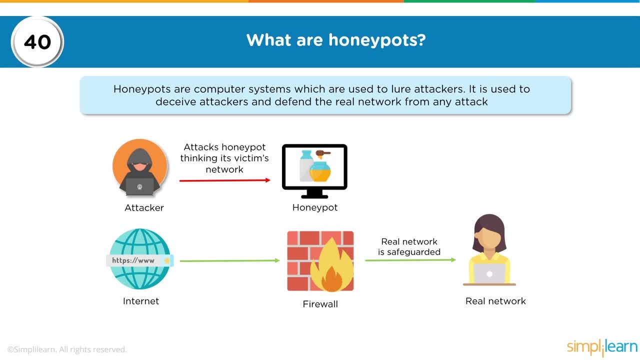 will prove as an attraction to these attackers, because it will demonstrate some vulnerabilities to the hacker which will divert their attention. So these vulnerabilities are simulated on these devices. These actually do not exist, But the moment the attacker then starts interacting with the honeypot, the honeypot will identify that. 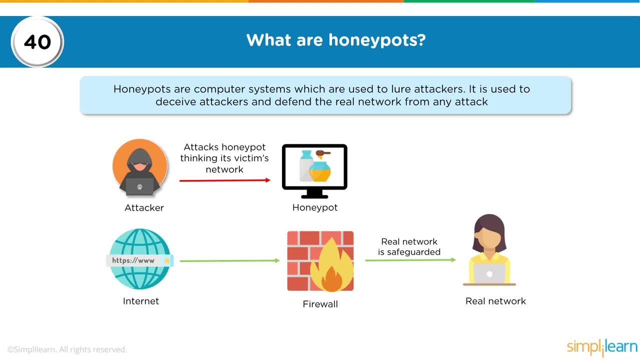 as a malicious traffic and will warn the administrator about a possible attack that is going on. The administrator will then investigate through the honeypot of what activity is going on and then reconfigure their security controls to block the attacker or mitigate the attack itself. 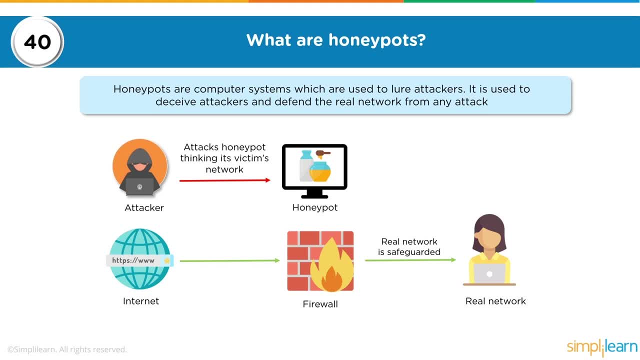 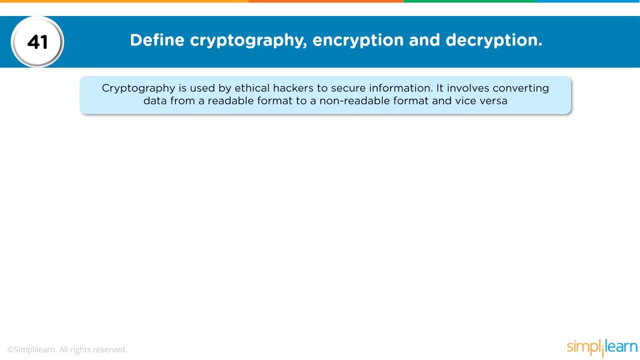 So it is more of a decoy server that will showcase or simulate some vulnerabilities to an attacker, thus to lure them and save the attacker. These are the 10 questions for cybersecurity. In the next video we will be talking about cryptography. The first question: define cryptography. 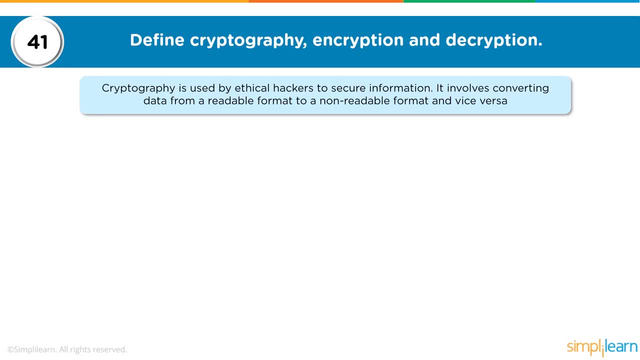 encryption and decryption. Now cryptography is used by security professionals to scramble data into non-readable format, which is used in securing that information. So it involves converting data from a readable format into a non-readable format and then reversing it back to readable format again, For example, the word computer. 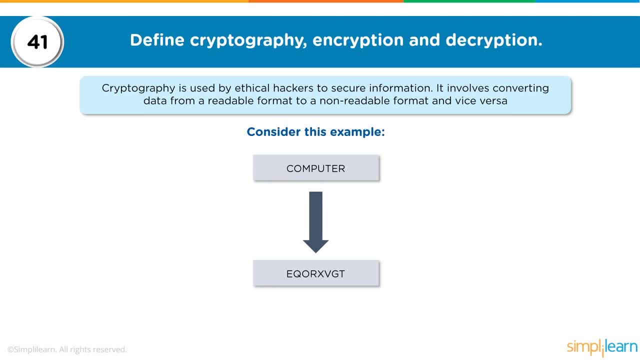 is now scrambled into looking like an unreadable format. Now, if you look at this word that it has been scrambled into, it would be very difficult for a human to figure out what the actual word was. Now, in this scenario, we have taken an algorithm where we have 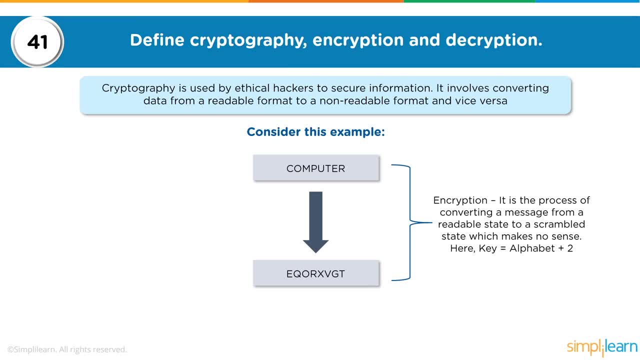 made a shift of the alphabet, where we have added two alphabets to the current one. so C plus 2 becomes E, O plus 2 becomes Q, M plus 2 becomes O. So we have done a shift of 2 and thus 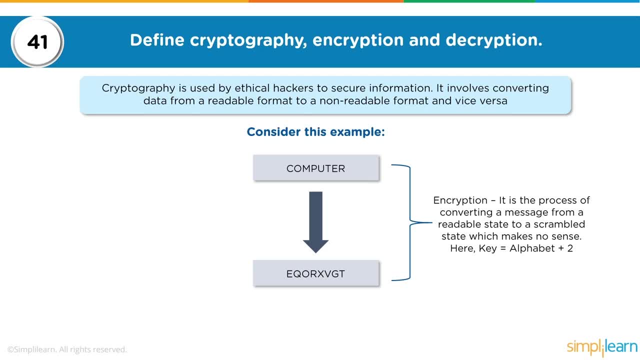 the key over here for this algorithm is the alphabet plus 2. So any person who figures that out will be able to unscramble this and convert this back into readable text. The fact of scrambling a readable text data into something that is unreadable by using 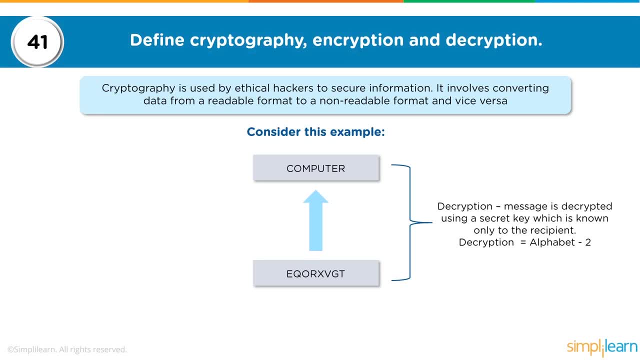 a particular key is what cryptography is all about. Now, as we discussed, the decryption again is replacing the alphabet and taking it further back by two characters. so E minus 2 becomes C, Q minus 2 becomes O, O minus 2 becomes M, and so on, so forth. So anybody who knows this key. 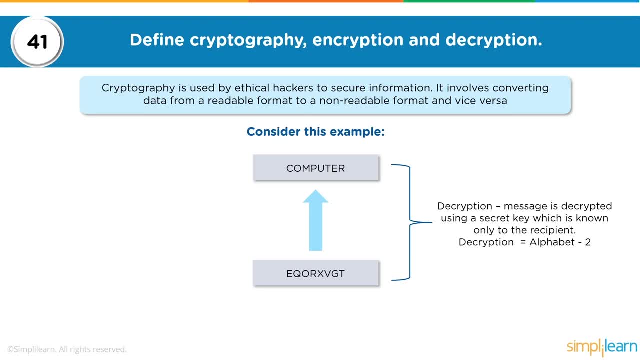 the shift key, anybody will be able to decrypt this particular character, So this depends on the user. If I want to utilize alphabet plus 5, then the spacing, the shifting of that character will be the fifth character from that particular character, and so on, so forth. 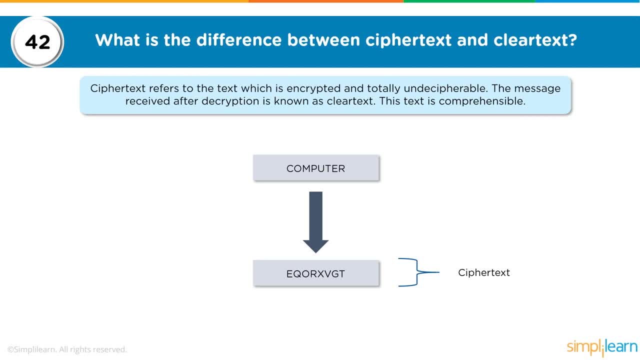 The next question: What is the difference between ciphertext and cleartext? Ciphertext refers to the text which is encrypted and totally undesirable. The message received after decryption is known as cleartext. This text is comprehensible. So the word computer is cleartext. That means that it has 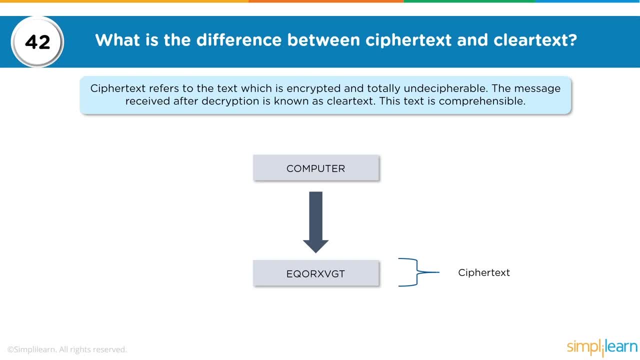 not been treated to any cryptographic measures. It does what it is intended to be. However, if the moment we encrypted, that means we scramble it into unreadable text by using any of the algorithms that we will be looking at, that text is known as a ciphertext. 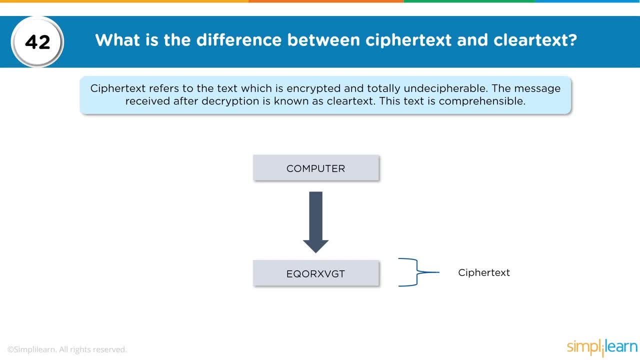 and without the key, this becomes unreadable. The cleartext as discussed is the plain word that we have utilized. We are using the English language in this instance, So the plain word computer is the cleartext Once we add the encryption layer to it. 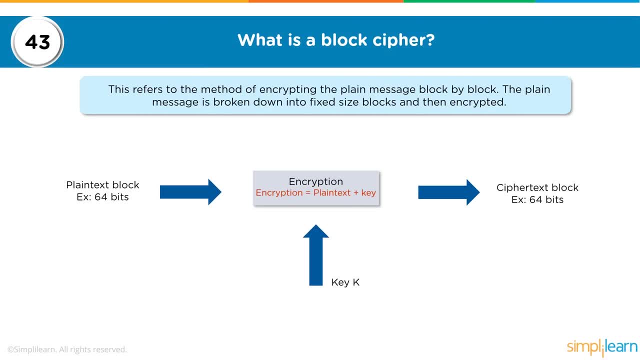 we get the ciphertext to it. Moving on to the next question, what is a block cipher? This refers to the method of encrypting the plain message. block by block, The plain message is broken down into fixed size blocks and then encrypted. Now, a block cipher is normally used for 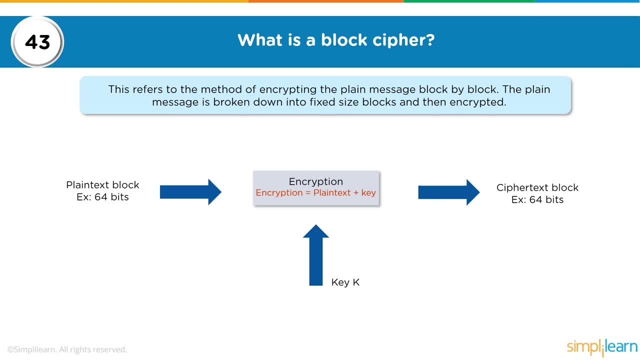 data that is stored, So a data that is stored on a hard disk and we want to encrypt that data. that is known as block encryption or a block cipher. So a block cipher is an algorithm that will allow you to encrypt data that is stored onto a hard disk. 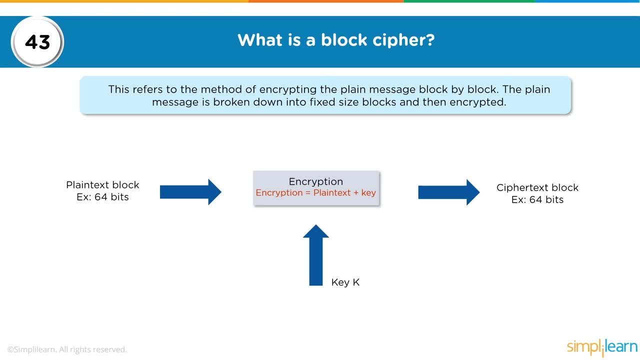 So in this example we have got plain text, which is 64 bits in size, and we have added a layer of encryption to it. So plain text plus the key that we have studied in the previous questions, and then the scrambled data out of it, which is 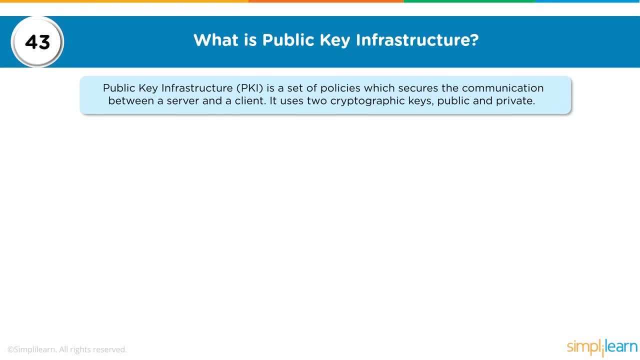 unreadable and thus encrypted. Then the next question: what is public key infrastructure? Now, the public key infrastructure is a set of policies which secures the communication between a server and a client. It uses two cryptographic keys, public and private. So the infrastructure itself is 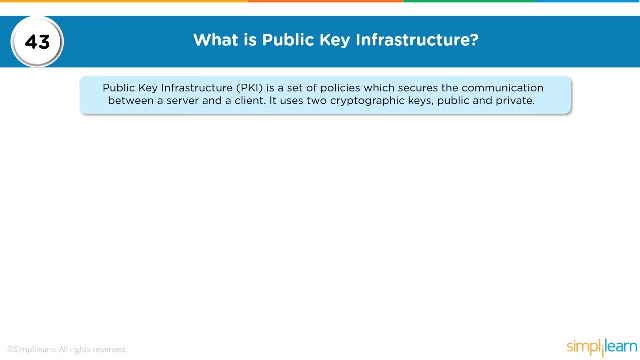 a set of policies, people, procedures and techniques which are standardized in nature and are globally accepted, which allow us to use digital certificates to encrypt data and decrypt the data. at the other end. We use asymmetric encryption over here, which means that we use two keys. one is a. 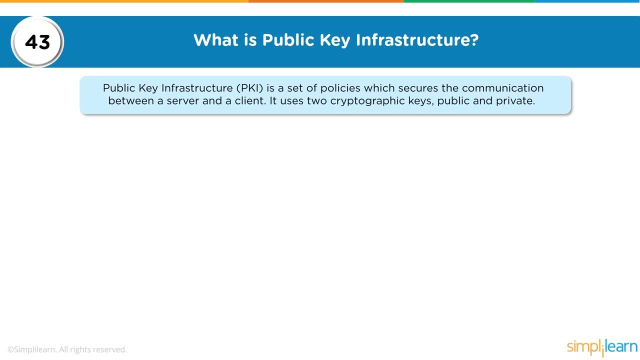 public key to encrypt and the private key to decrypt. The other part of encryption is asymmetric encryption, where the same key is used to encrypt and the same key is used to decrypt. Now, in a public key infrastructure, like I said, we have standardized that. so in the standardizing part, 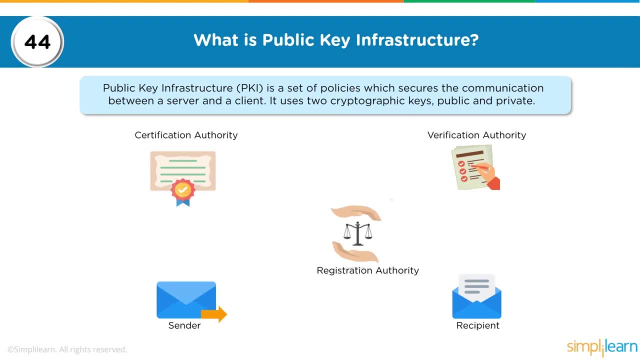 of it. these are the various players that have been defined in the public key infrastructure. The first is the user or the sender, in this scenario, the one who requires this digital signature to digitally sign a particular transaction or a communication, A registration authority with whom they are going to register for that. 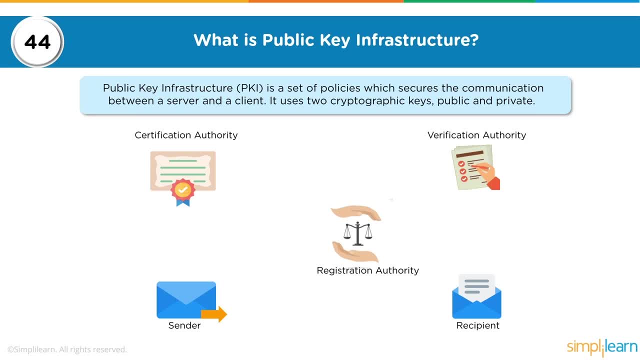 particular key, The certification authority who issues that key and the verification authority who validates the key itself and the recipient, who is going to be the other party of that particular transaction. So how is this utilized? A sender or the user who requires this digital signature will request. 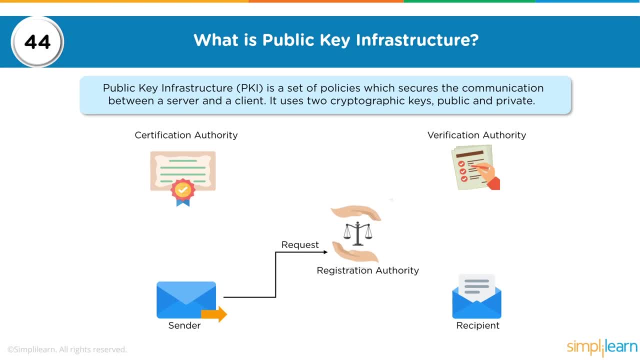 or apply for a digital signature with the registration authority. The registration authority would validate the genuity of the user so they might do some identity verification or proof of residence or something like that. once they have identified the person and they have validated the information, they will then send the request. 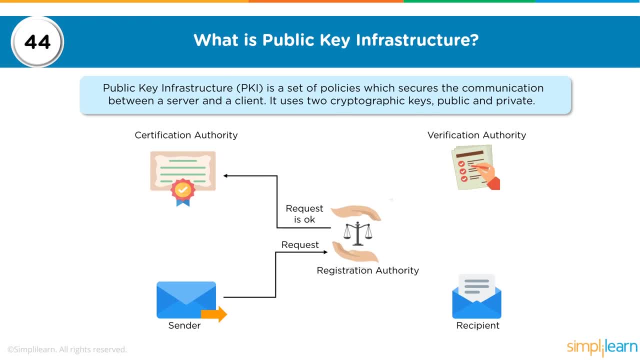 to the certification authority stating that the sender has been validated and the certification authority can issue the digital certificate to the particular user. They will send the public key to the sender, which will be utilized by the sender for further transactions. So when the sender is going to sign some, 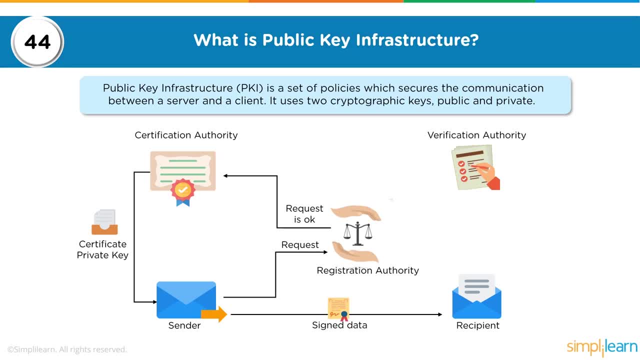 data and wants to send it across to the recipient, they will use the public key to sign it and send it across. The recipient will then validate with the verification authority to see if the data, the signed data, is correct or not. Now, while the certification authority sends the public. 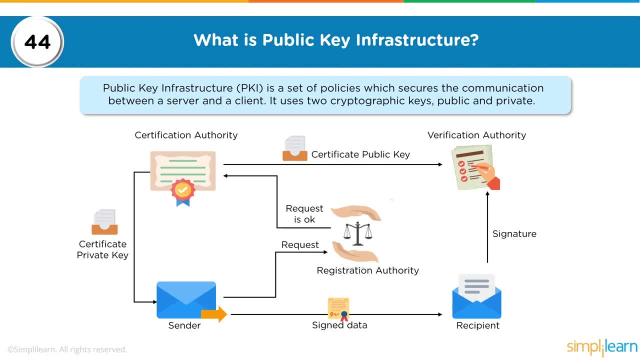 key to the sender. the certification authority updates the private key with the verification authority. So whatever is signed by the sender, received by the recipient and they want to validate it, they will send it back to the verification authority. The verification authority will validate using the private. 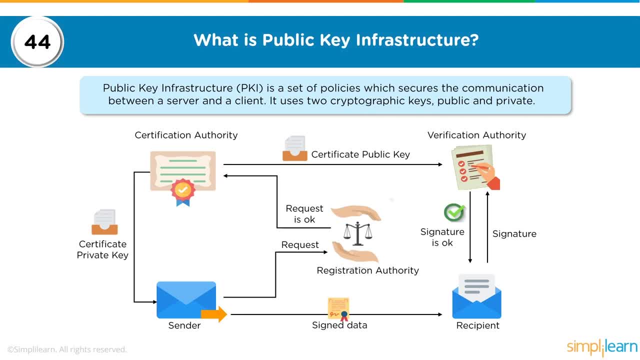 key. Once the private key is validated, it will then send the okay signal back to the recipient, thus allowing the validation of that particular transaction. If the signature is tampered with or is not, the verification authority is not able to validate the signature. it will then send. 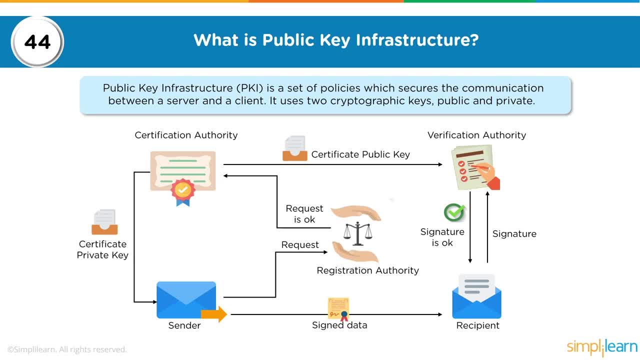 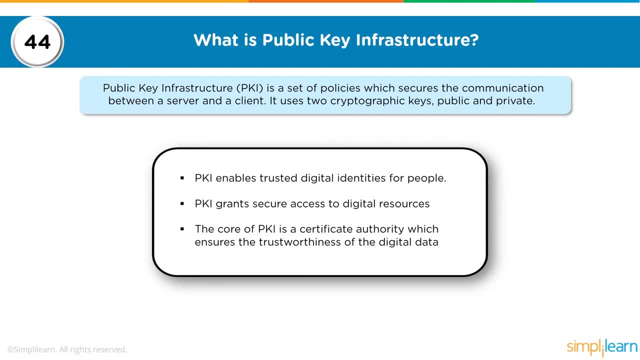 a denial message back to the recipient and the transaction will not go through. So the PKI enables trusted digital identities for people. So the PKI grants secure access to digital resources based on the infrastructure that has been created, and the core of the PKI is a certification. 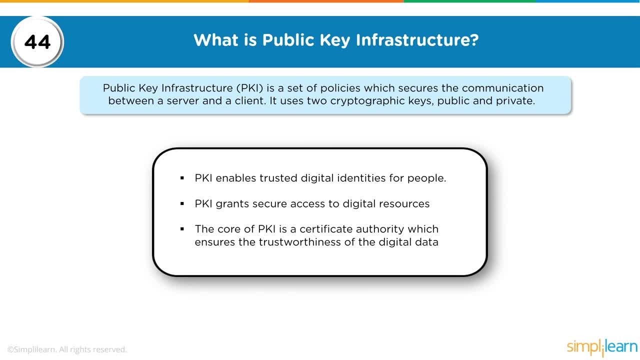 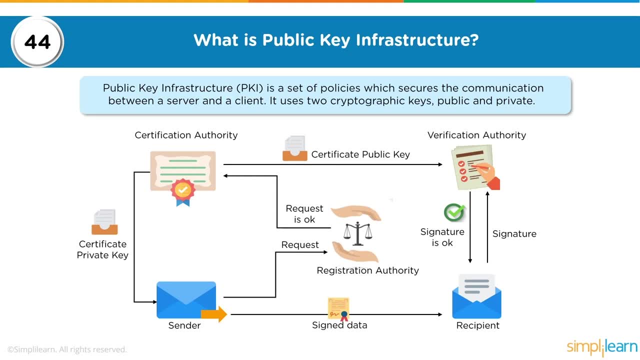 authority which ensures that the trustworthiness of the digital data is ensured. So, going back to the previous slide, these are the key players that have been standardized in the public key infrastructure. The certification authority is the authority that issues the digital certificates, The validation. 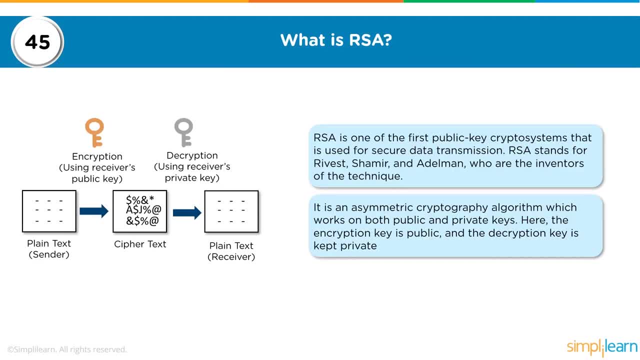 authority is the one who validates that digital certificate. Now let's focus on what is RSA. RSA is one of the first public key crypto systems that is used for secure data transmission. It stands for Rivest, Shamir and Edelman. Now, these are the. 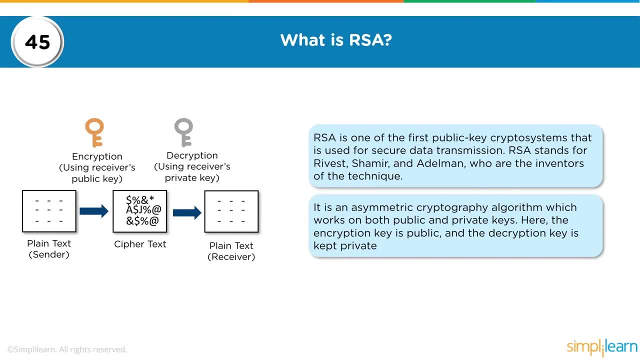 three people who have created this algorithm: Ron Rivest, Adi Shamir and Leonard Edelman, who are the inventors of this technique. It is an asymmetric cryptography algorithm which works on both public and private keys. Hence, the encryption key is public and the decryption key is kept. 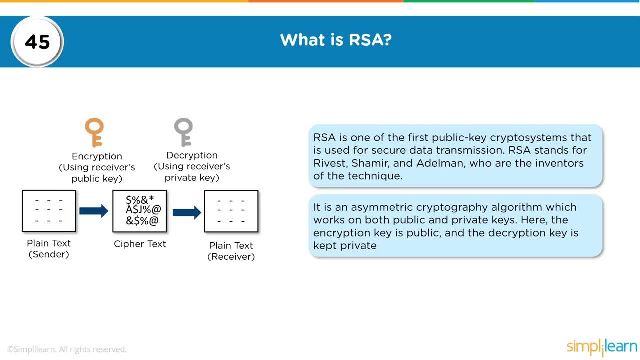 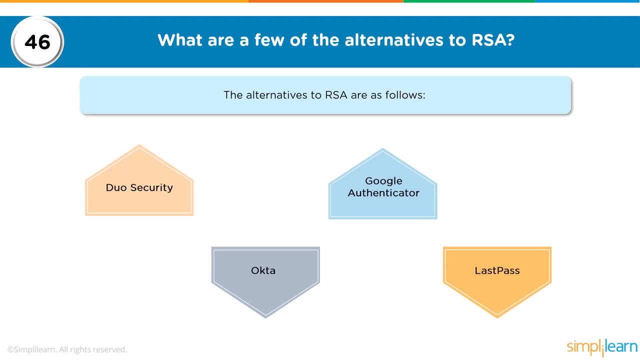 private. Now, as we have discussed earlier symmetric and asymmetric cryptography. Symmetric cryptography is where the same key is used to encrypt and decrypt, whereas asymmetric cryptography is where there are two keys to encrypt and decrypt the algorithm. What are the few alternatives to RSA? Now? RSA is: 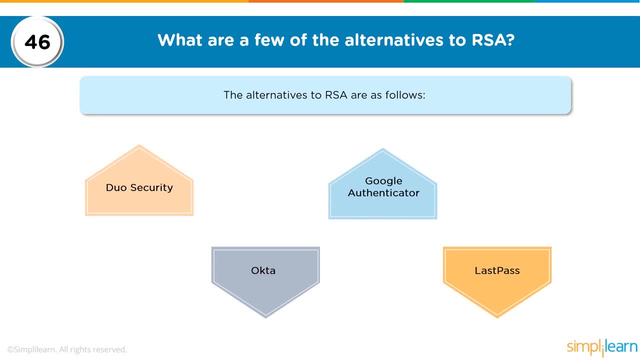 an algorithm that is used for encryption. There are a lot of other algorithms that can be utilized to alter or to scramble data, depending on your requirements. So in the previous question we have studied and we have talked about what RSA is. It stands for Rivest, Shamir and Edelman- the three 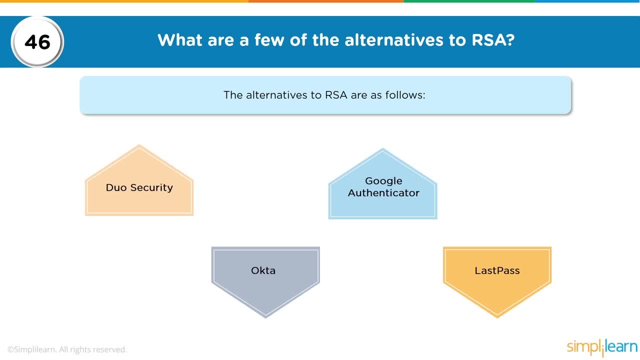 creators of that particular algorithm. But there are a lot of alternatives to this algorithm, depending on how secure you want that data to be, And some of them are listed here on your screen: DuoSecurity, Okta, Google Authenticator and LastPass. 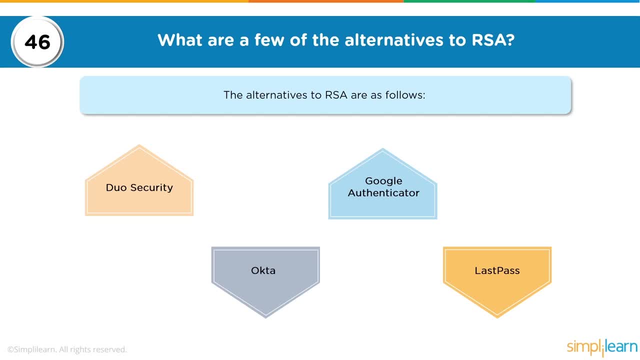 LastPass is a password manager, so is DuoSecurity. Google Authenticator is something that we all utilize. It is an application that you can download and store on our mobile device, and we can set that up to authenticate ourselves with certain portals, So it issues a unique 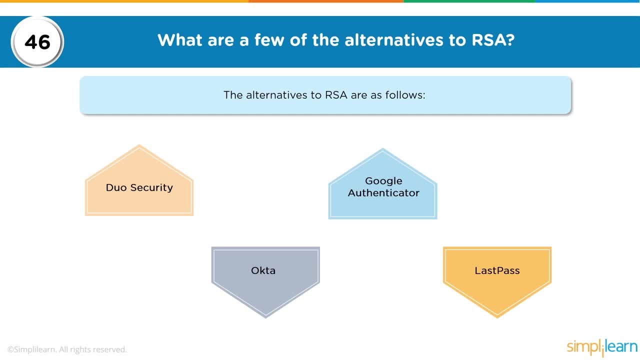 ID to us which, once utilized, will allow us access to those particular portals. Okta is an identity manager where you have created different digital identities and you have assigned them certain permissions and, based on your authentication mechanisms, Okta will allow or disallow access to those different. 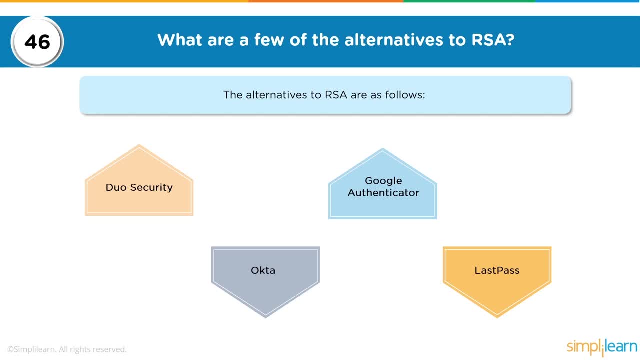 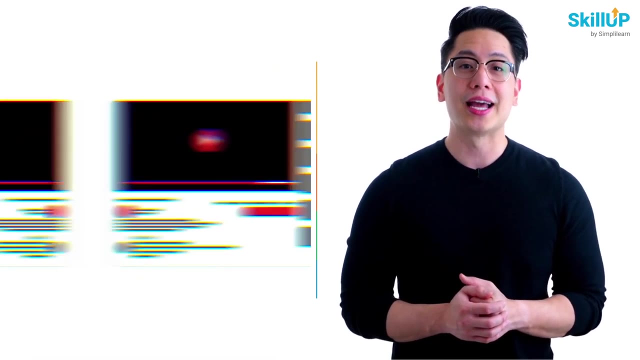 applications or different portals as you have configured it. So all four are authorization and authentication mechanisms which can be used as alternatives to RSA. If getting your learning started is half the battle, what if you could do that for free? Visit SkillUp by SimplyLearn. 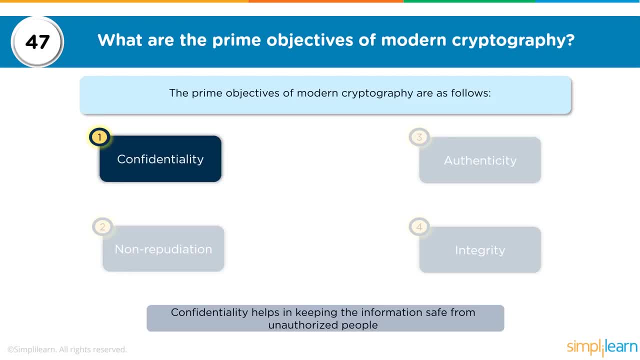 Click on the link in the description to know more. Next question: What are the prime objectives of modern cryptography? And this is a very important question, because we have so far looked at what cryptography is and what public infrastructure is, But what is the achievement out of it? 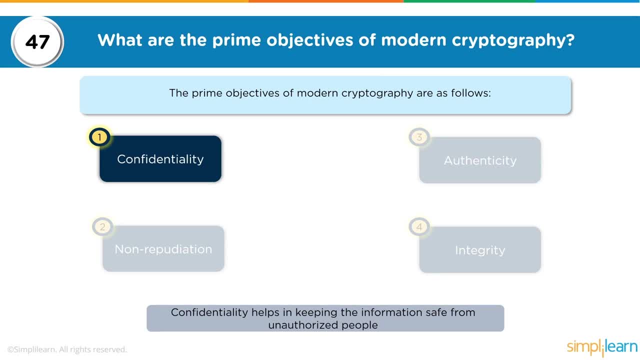 Why are we utilizing it And what do we want to gain out of it? So the main and the prime objectives of modern cryptography are as follows, mentioned on your screen. The first one is confidentiality, The second one is non-repudiation. 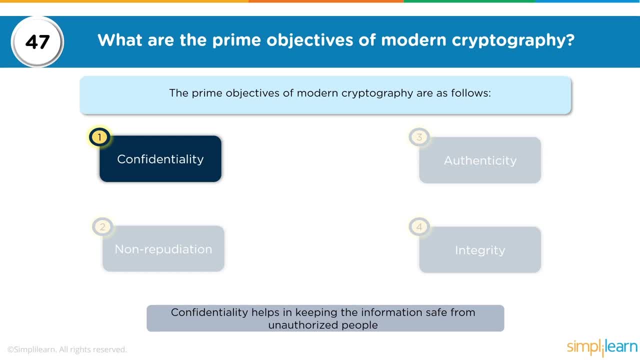 Third one is authenticity, And the fourth one is integrity. Now, if I go back to the first one, confidentiality. that is where I want to keep data confidential. That means it will only be visible to authorized users. So here I have created a list of 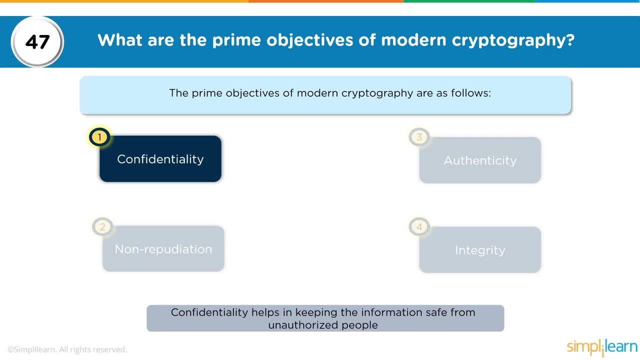 people who I have deemed as authorized users and I have created a digital identity to them and I have given access controls to those people. Now, that is how confidentiality is ensured. So when we want to keep data confidential, we create a list of users who we are. 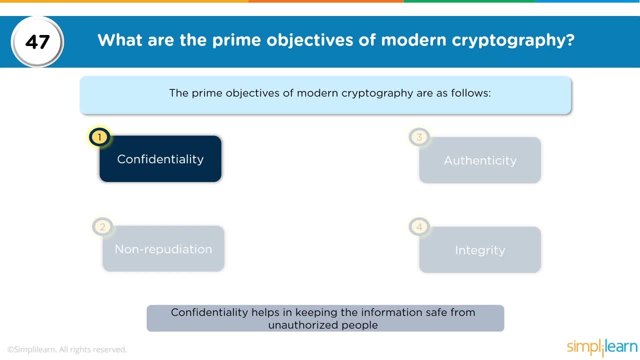 going to allow access to certain resources and we are going to define what access controls are to be utilized, what access are allowed, whether they've got administrative access or user level access- and only those authorized users are going to be able to access these resources. 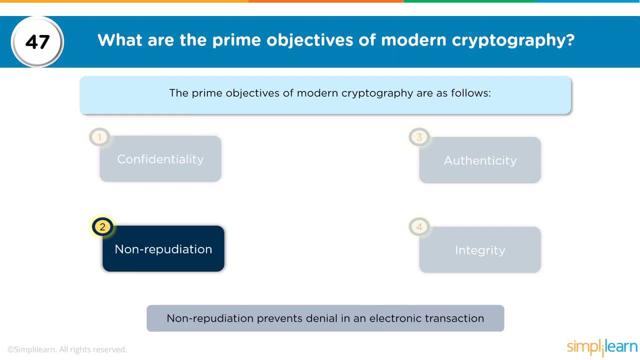 That is how we maintain confidentiality. The next one is non-repudiation. Non-repudiation is the prevention of denial of having been a part of a particular transaction. So in the public key infrastructure that we discussed, where a digital signature was utilized to sign, 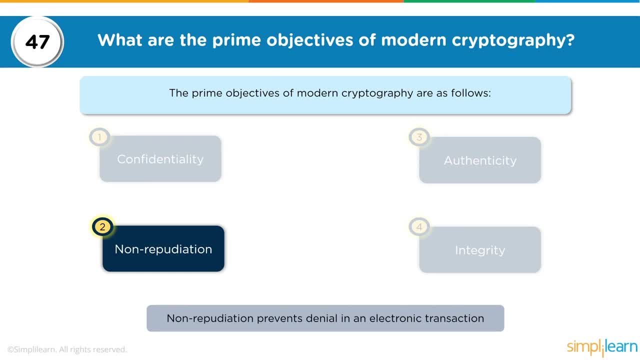 a particular transaction and then sent to the recipient. the sender would not be able to deny of having originated that transaction because it was using their digital certificate. Thus non-repudiation comes into the picture. One more example that we can have here is on our mobile. 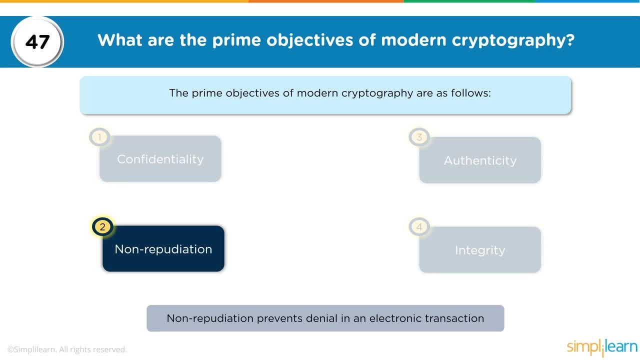 phones. when we use SMS short messaging service and we send a message to another person, the person- when they receive a message, the number is validated by the service operator and thus the sender cannot deny having sent that message. The sender at the same. 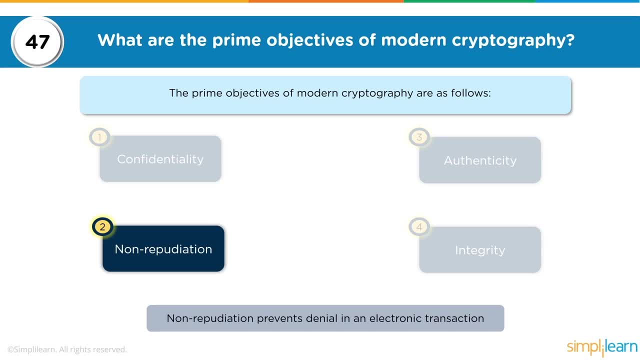 time can have a delivery report sent to them that the message was delivered to the inbox of the recipient, and thus if the recipient denies having received that message, the delivery report becomes proof of having that message being delivered to their inbox. Thus, both the parties cannot deny of. 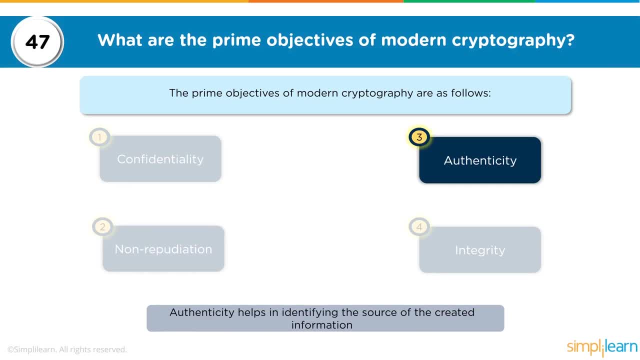 being a part of that particular transaction. Then comes the part of authenticity. Now, in confidentiality, we have created a digital identity, assigned it to a particular person and we have given them digital signatures where they cannot deny having been a part of that transaction. But authenticity is the part where 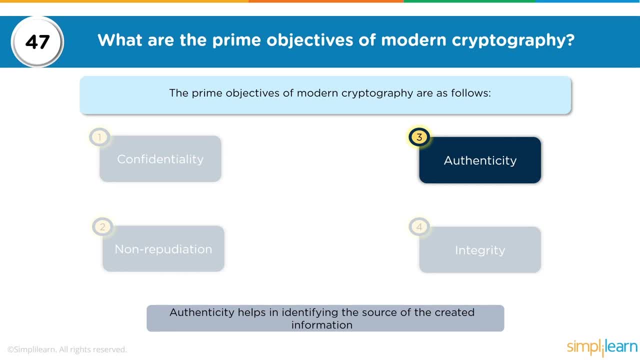 they try to prove that they are who they claim to be. So if I am claiming a digital identity, I have to prove that I am that person who I am trying to claim to be. An example to that is when we go to our gmailcom websites. 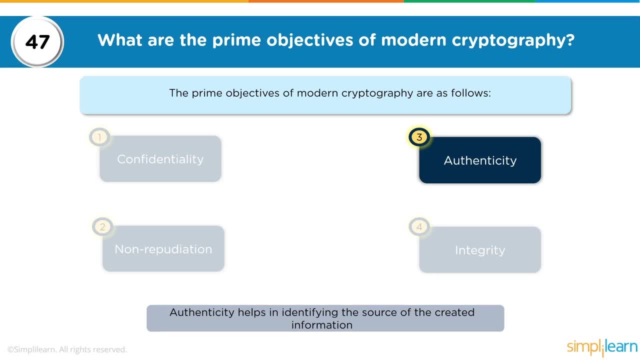 it first asks us: what is our username? Our username is normally our email address, which identifies the account that we are trying to access. So this account is confidential because it is only authorized for a particular person, and once they identify themselves by identifying the email address, that is when the authentication part 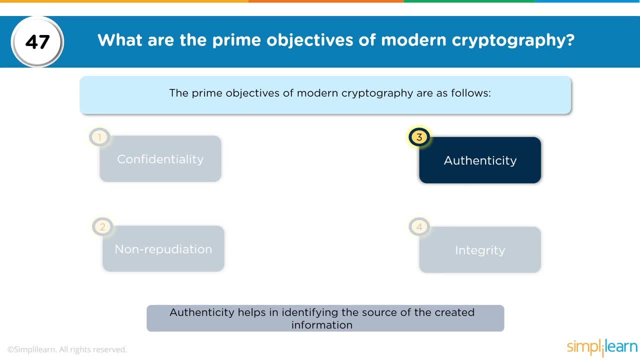 comes into the picture where it asks for the password. Now, it has never, ever happened that we just go on to gmailcom, type in a password and then it figures out which account we are talking about. So the first step is always the confidentiality part, where we identify which account. 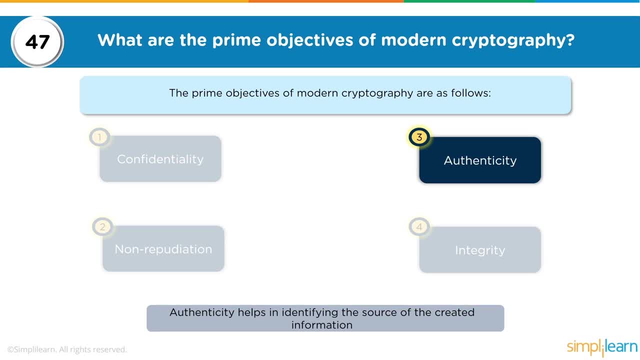 we are talking about, and then we try to authenticate as the owner of that particular account by providing the appropriate password to that account. If both of these match, only then do we get access to that account and we are able to make whatever transactions we want to make Now, when we are making. 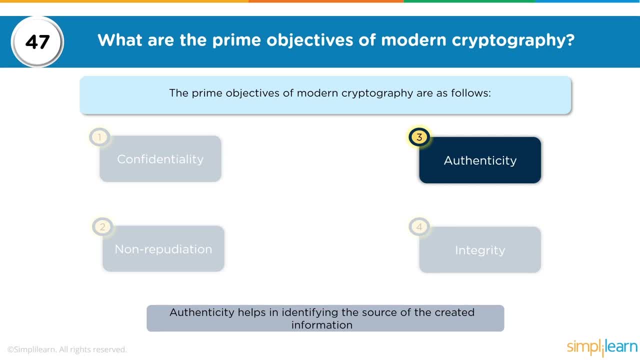 those transactions. non-repudiation comes into the place where all our activity is also being logged. So we have identified our account, we have authenticated ourselves by providing the password, so the proof is there that it is us who are trying to access it. and then 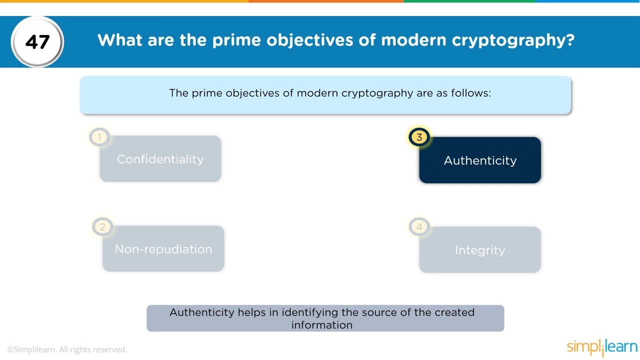 whatever activity we do- send an email, receive an email, delete something, attach something- all of those activities are logged and stored as proof of what actions have been done. So tomorrow, if we deny having sent that email, gmail can still prove to us through. 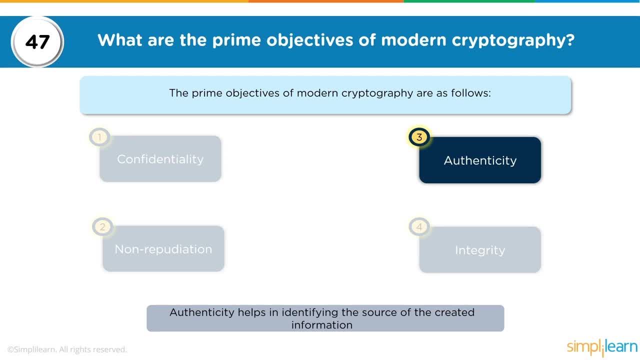 those logs that that activity was done by us. And the fourth part is integrity, which ensures that the data received and sent by the sender and received by the recipient has not been modified, while in So the integrity part is the trustworthiness of that data. 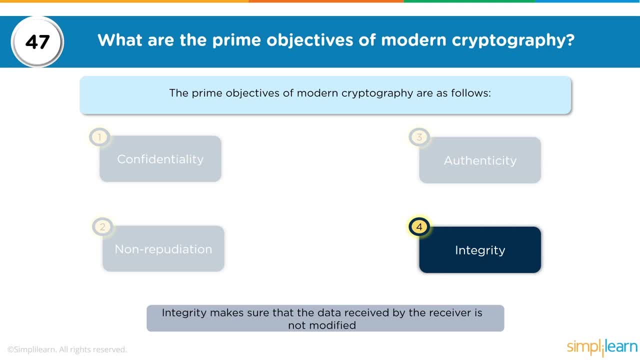 that the data has not been modified by any hacker or any other entity and is still trustworthy. So these are the four prime objectives of modern cryptography. Once I have scrambled that data using my public signature, it is only my private signature that is going to decrypt it. 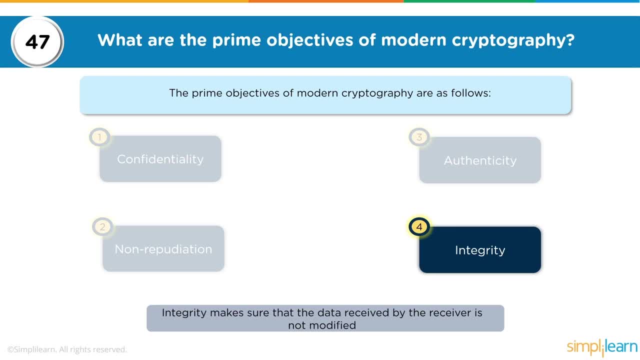 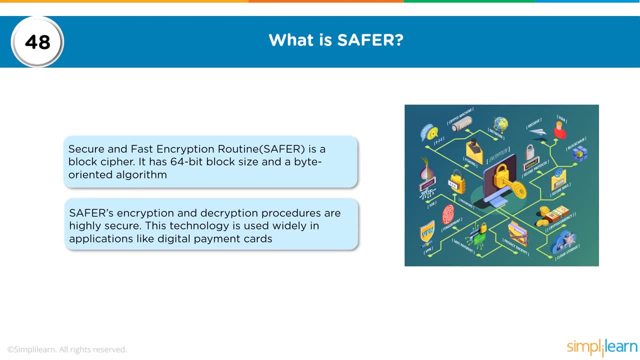 Using these mechanisms, I will be able to achieve all these four aspects of cryptography and security. Next question: what is SAFER Now? SAFER stands for secure and fast encryption routine, which is also a block cipher, As we have discussed previously. block cipher is a 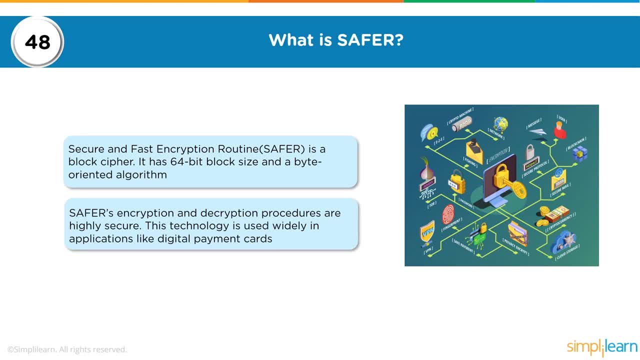 cipher that is used to encrypt data that is stored, So it has a 64 bit block size and byte oriented algorithm. SAFER's encryption and decryption procedures are highly secure. This technology is widely used in applications like digital payment cards. So when you are using 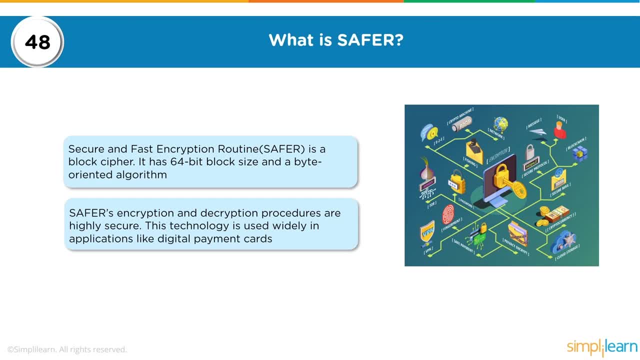 a digital payment gateway to make transactions. you have gone onto an online portal, you want to purchase a particular item, and then it takes you to another payment gateway where you have to fill in your credit card information, sensitive information like your expiry date, CVV information. 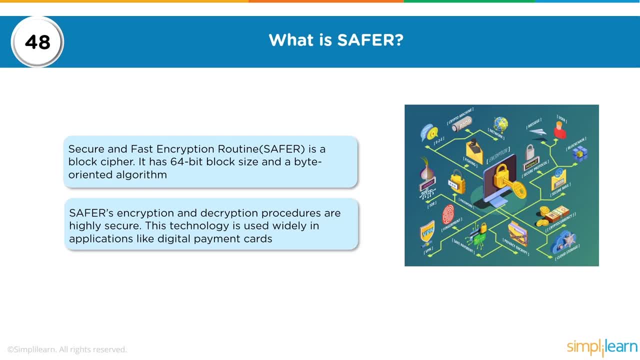 and then the OTP, or the password that you have created for your particular account. Now all of these need to be secured or highly secured, based on PCI DSS, which is the payment card industry data security standard. So these standards ensure that certain protocols are utilized. 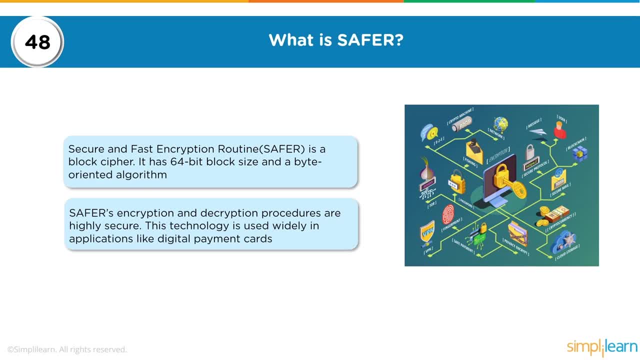 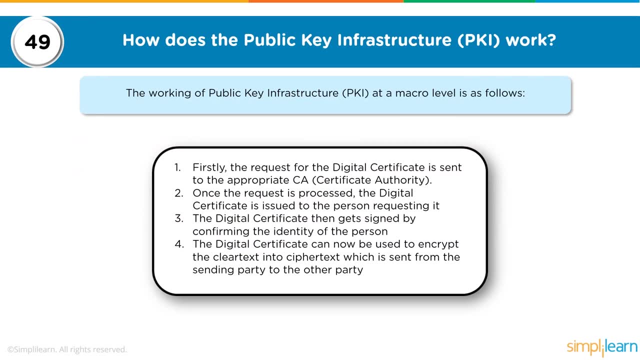 to attain that level of security. SAFER is one of those block ciphers that is used under the digital payment gateway infrastructure. Next question: how does the public infrastructure, public key infrastructure- work? Now, we have already discussed this in the previous diagrams We have identified. 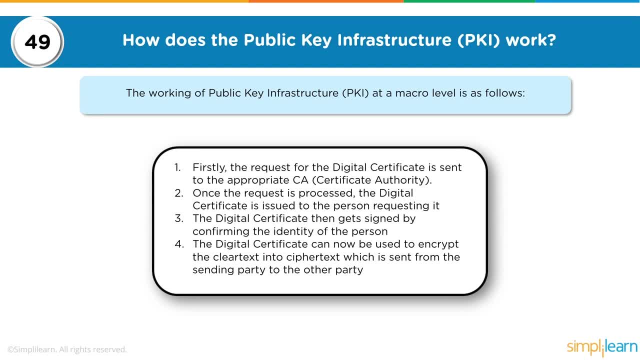 the key players: the certification authority, the registration authority, the end user who requires the digital certificate, the validation authority who is going to validate it, and then the recipient, the end user with whom the transaction is going to be conducted. So the first point here is: